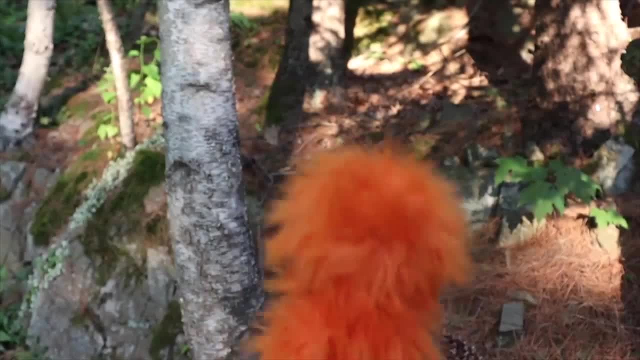 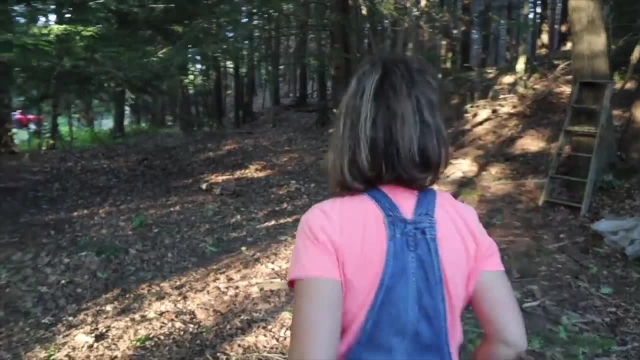 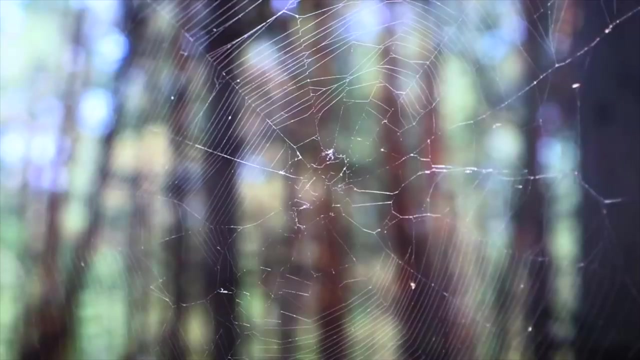 Look what I found. There's so many of them here. It's a tree Tree, Miss Rachel. I found a spider web and a bug. Wow, Herbie, Two things on our list we could to check off. Great job, Yeah, come see. 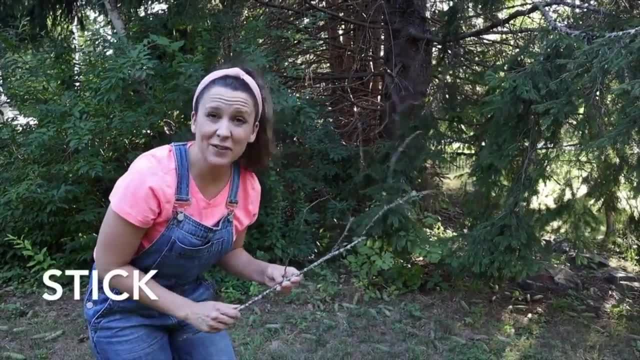 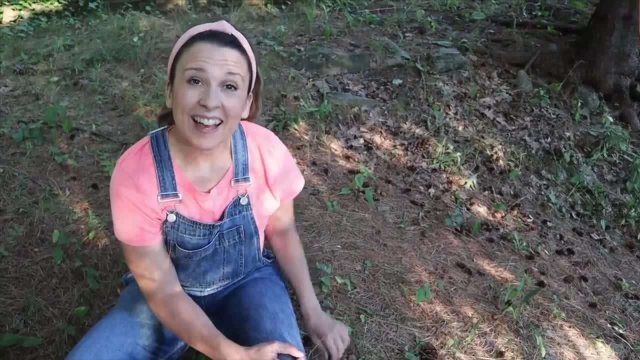 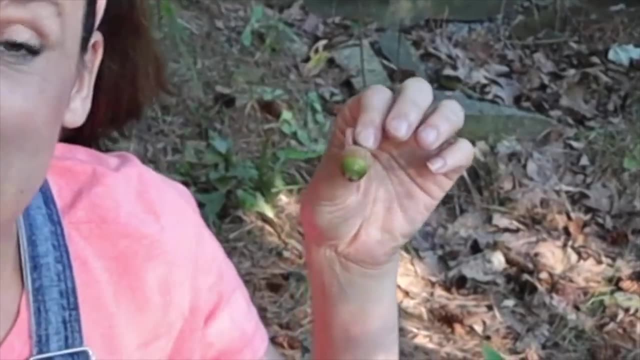 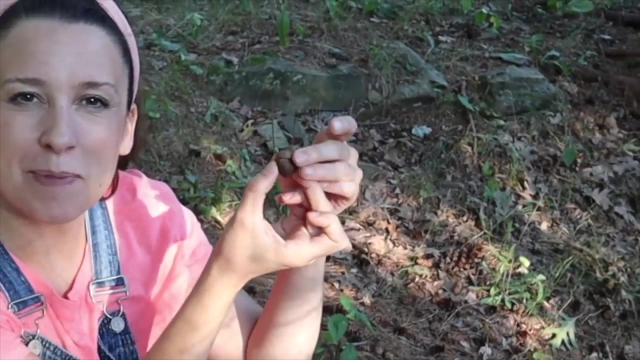 It's a stick. Wow, I found a big stick. Look what I found: It's an acorn. Wow, The acorn was hanging on an oak tree. Yeah, acorns come from oak trees. Acorns have a little cap on them. 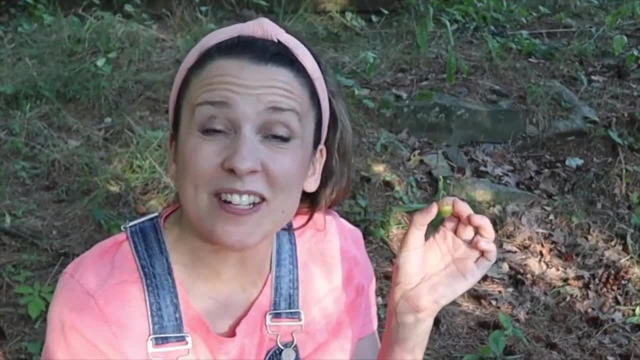 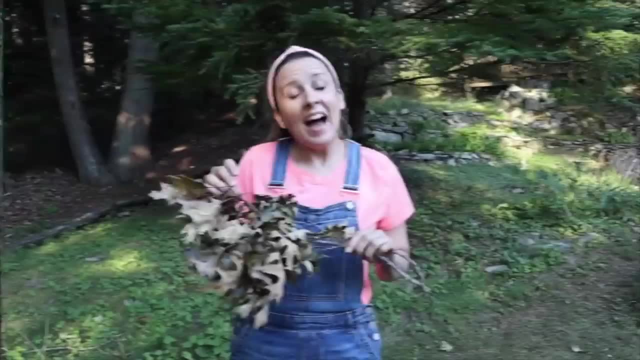 This one fell off. An acorn is on our list, so we can check it off. Great job, We found an acorn. Yay, I found this branch on the ground And guess what? There's still an acorn attached. 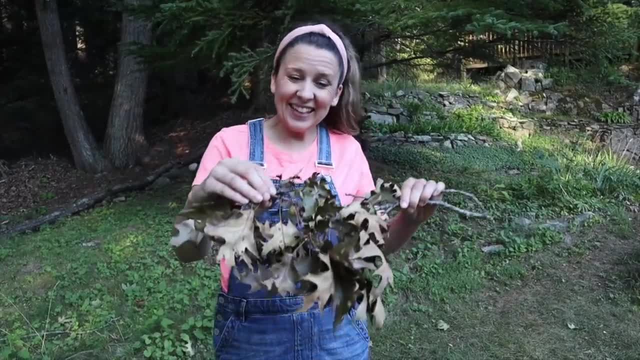 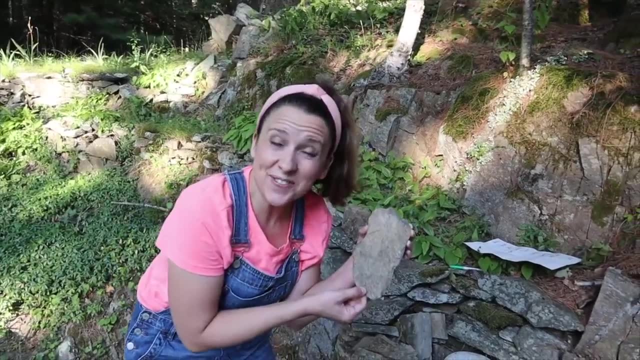 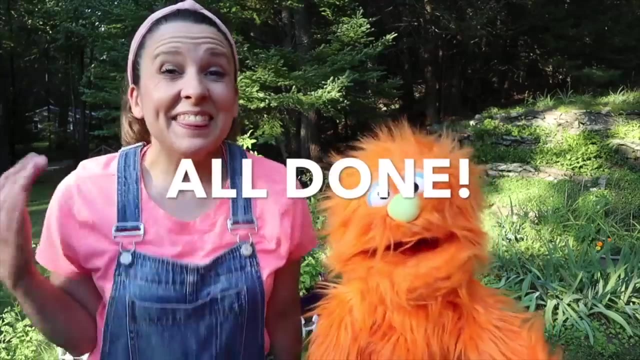 Would you like to see what it looks like? Okay, I found a rock which is on our list. I can check it off. That was so much fun. Yeah, We found so many great things. Yeah, we did Great job. 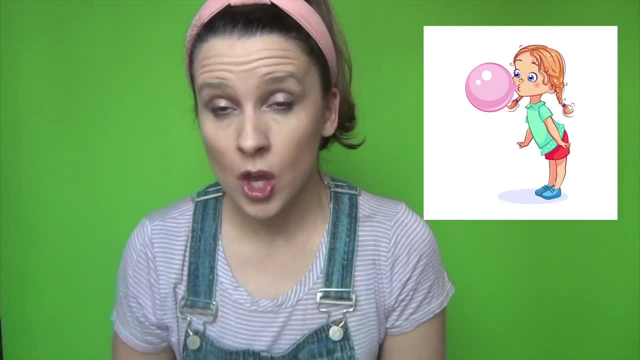 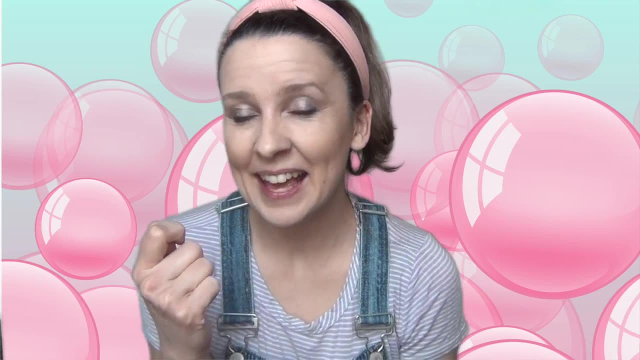 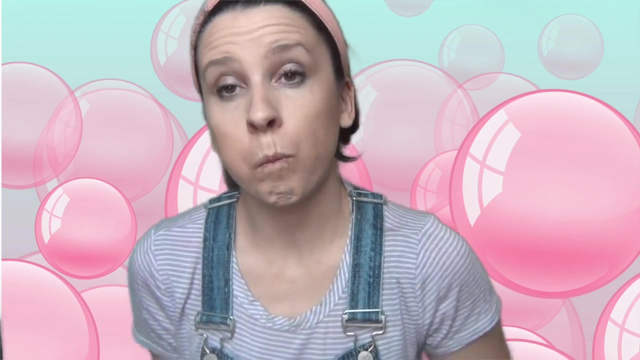 We're going to get out some pretend bubble gum. Okay, so get out some pretend bubble gum. What color is yours? Mine's pink. Put it in your mouth and we're going to chew it. Are you chewing your gum? Okay, now we're going to blow a really big bubble. Are you ready? 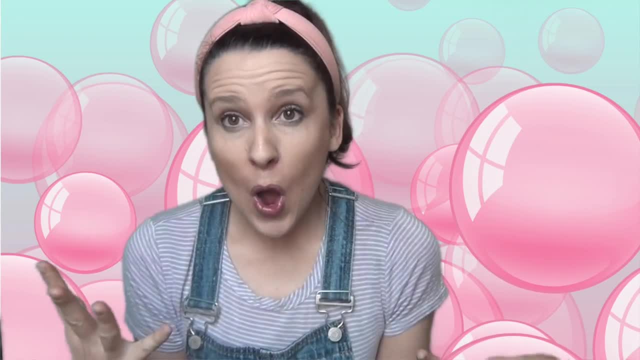 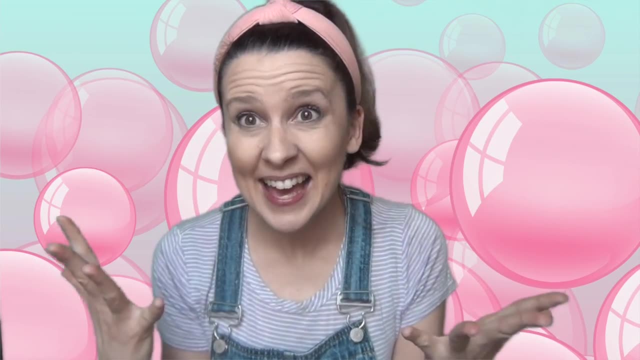 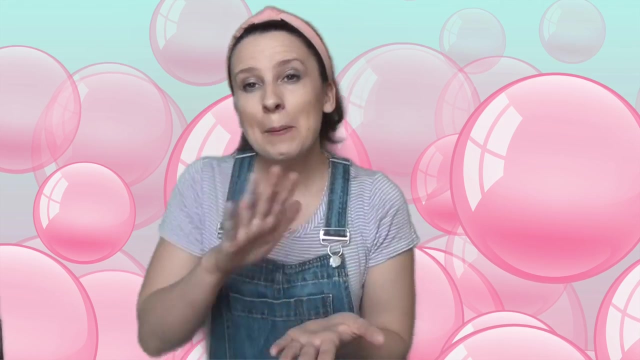 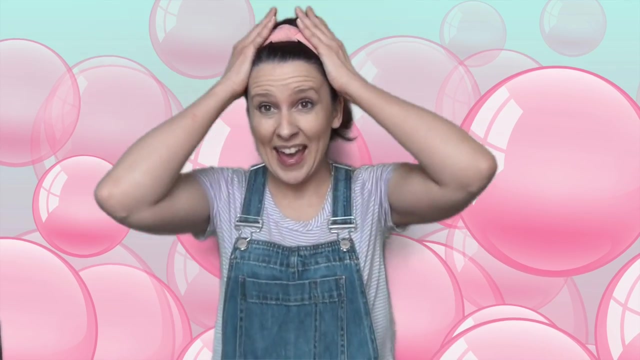 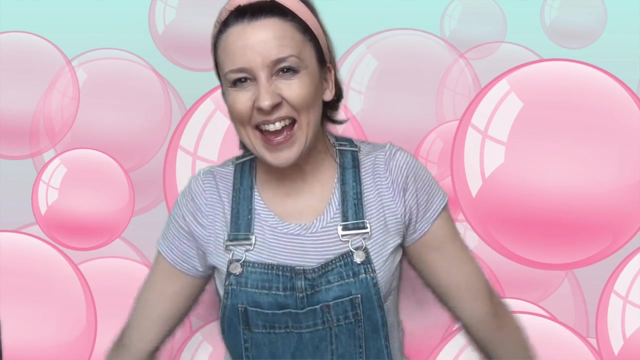 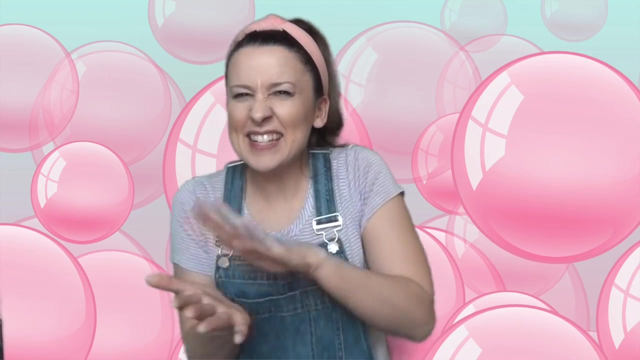 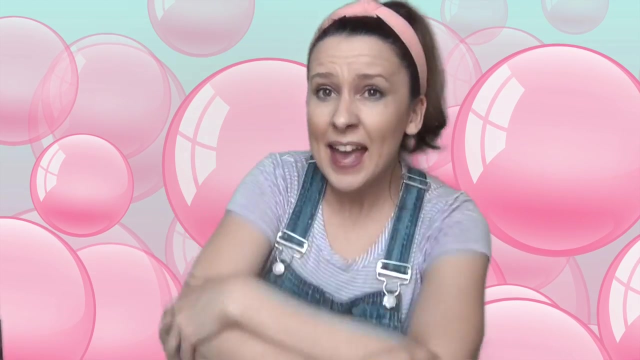 Wow Pop, Oh no, Our bubble popped and the sticky bubble gum is all over our hands. February, Oh my goodness. Okay, so what is it? Are you telling the story right now? No, And you pull them, and you pull them, and you pull them away. 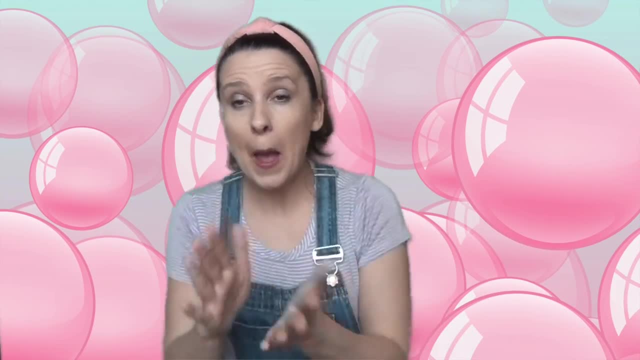 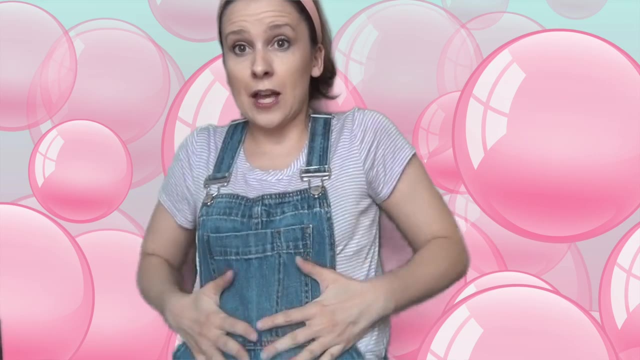 Icky, sicky, sicky, sicky bubblegum, bubblegum, bubblegum. Icky, sicky, sicky, sicky bubblegum makes your hands stick to your tummy And you pull them, and you pull them, and you pull them away. 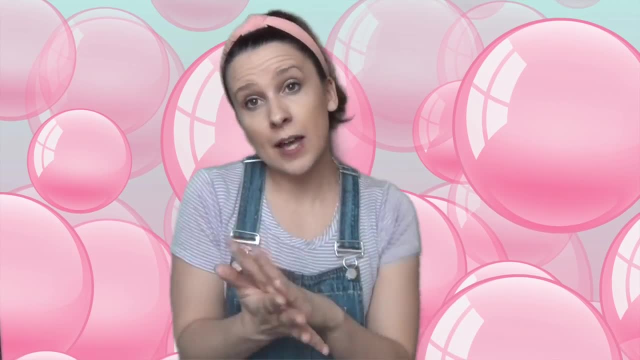 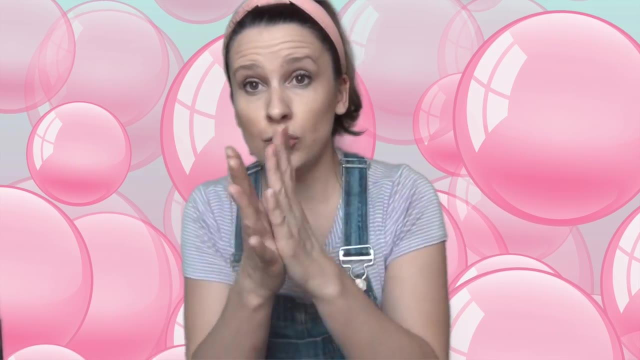 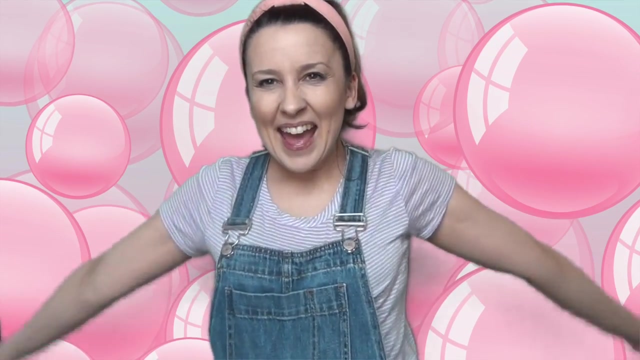 Icky, sicky, sicky, sicky bubblegum, bubblegum, bubblegum. Icky, sicky, sicky, sicky bubblegum makes your hands stick to your ears And you pull them, and you pull them, and you pull them away. 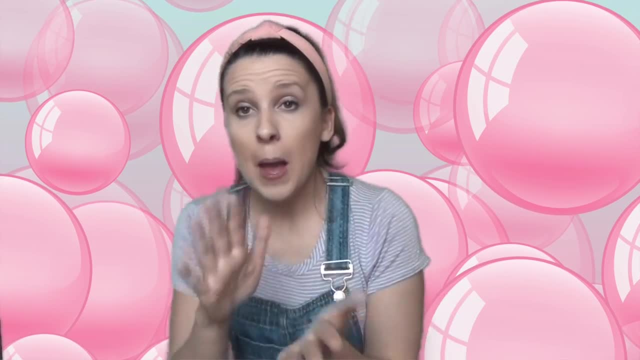 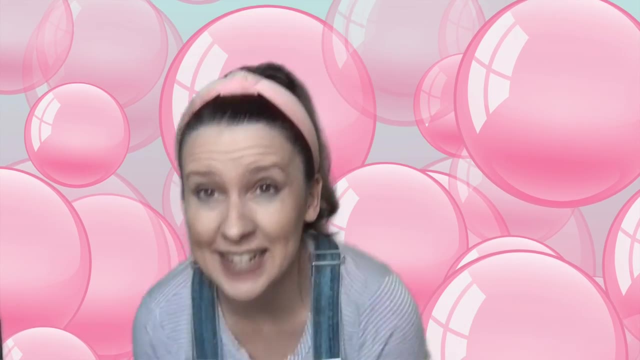 Icky, sicky, sicky, sicky bubblegum, bubblegum bubblegum. Icky, sicky, sicky, sicky bubblegum makes your hands stick to your knees. Are they on your knees? And you pull them, and you pull them, and you pull them away. 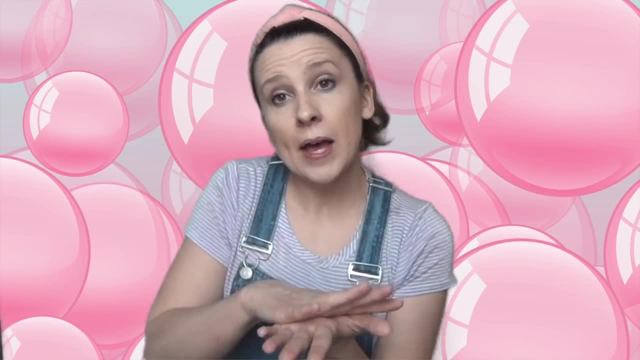 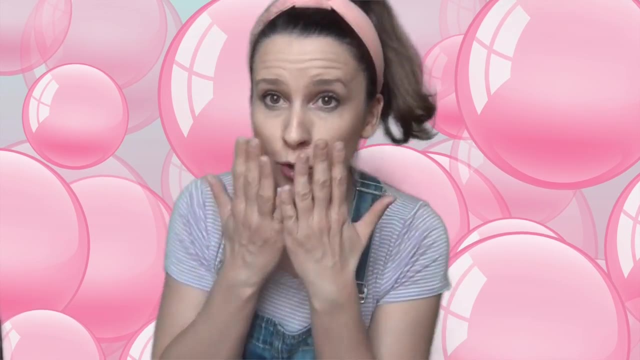 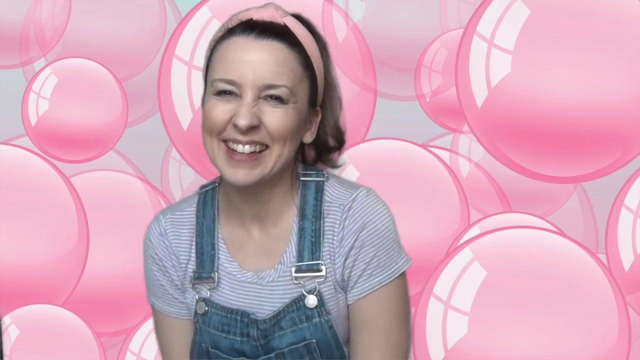 Icky, sicky, sicky, sicky bubblegum, Bubblegum bubblegum. Icky, sicky, sicky, sicky bubblegum Makes your hands stick to your mouth. Ba-do-ba-ba, Wa-ba-ba-ba, Da-ba-do-ba-ba-ba. 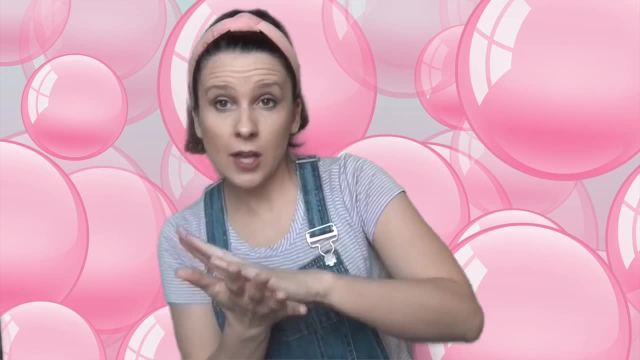 Icky, sicky, sicky, sicky bubblegum, Bubblegum bubblegum. Icky, sicky, sicky, sicky bubblegum Makes your hands stick to your grownup. 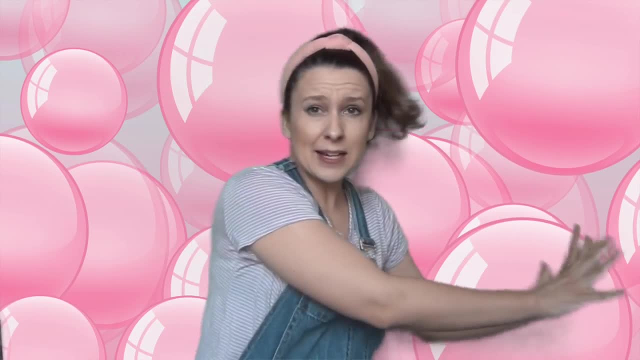 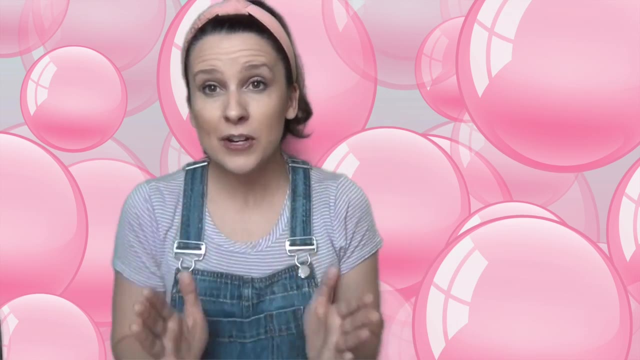 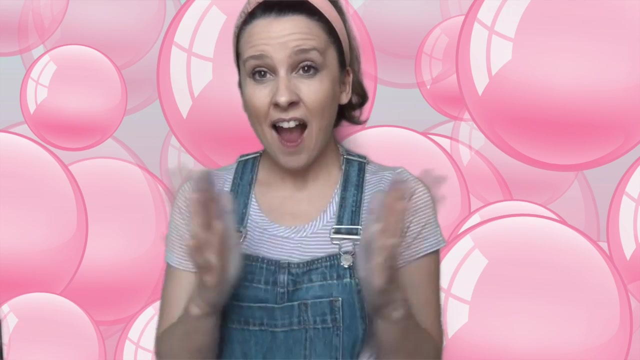 Put them on your grownup And you pull them, And you pull them, And you pull them away. That was so fun. One more time. Icky, sicky, sicky, sicky bubblegum Makes your hands stick to your. 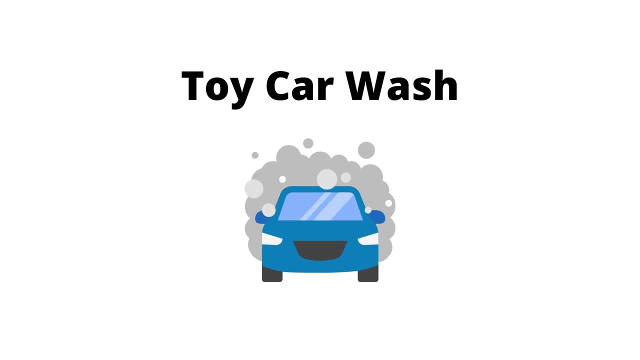 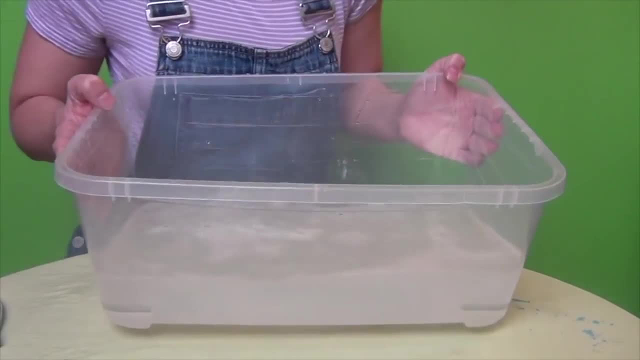 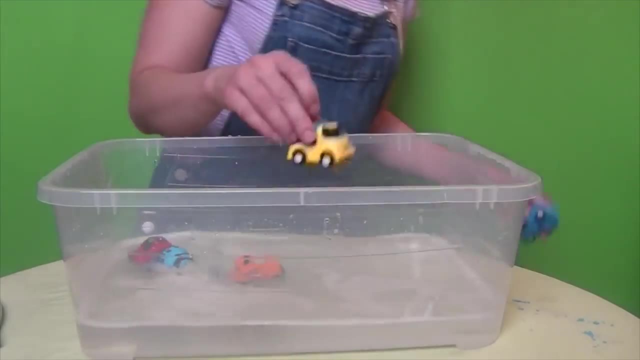 Yay, That was so much fun. Let's fill this tub of water so we can give the cars a bath. Let's put the cars in the warm water, And I put in some soap too. Putting the cars in the water, In In. 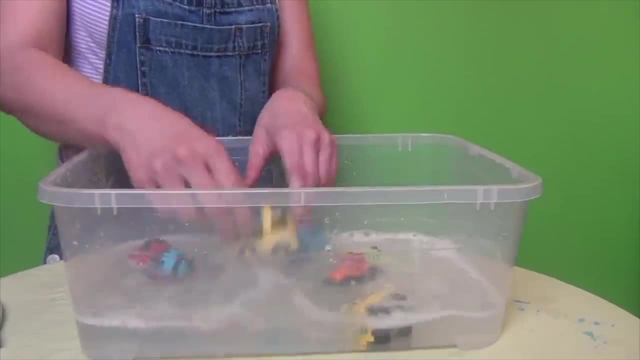 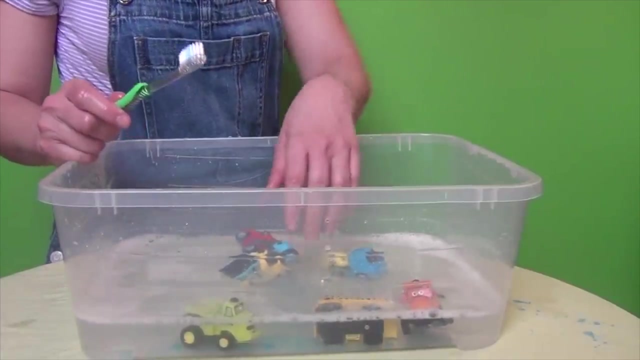 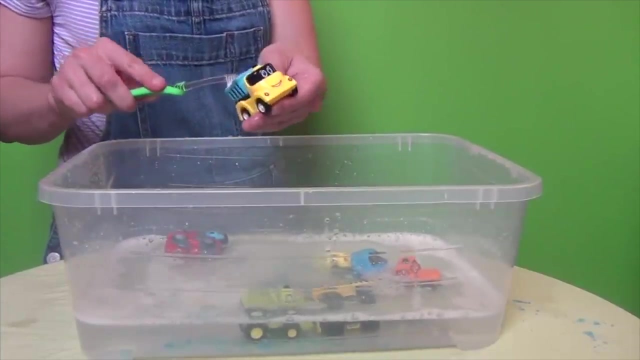 Ooh, they like the bath. You're right, This was so much fun. Ooh, Now I'm going to take a toothbrush and clean the cars. Oh, that tickles. I want to get you all clean, so I'm brushing you with a toothbrush. 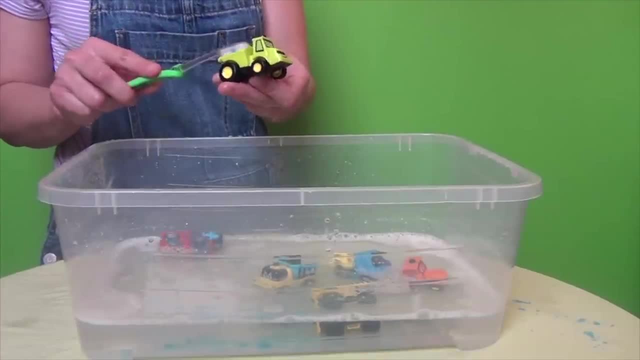 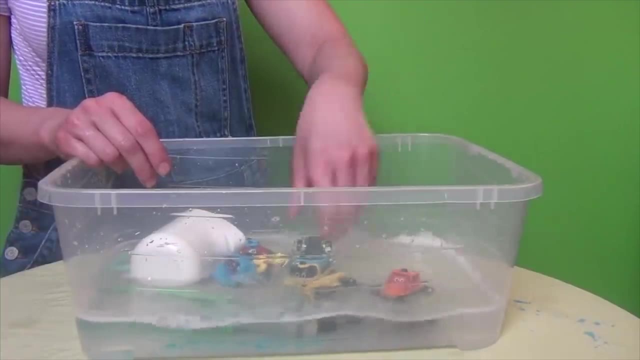 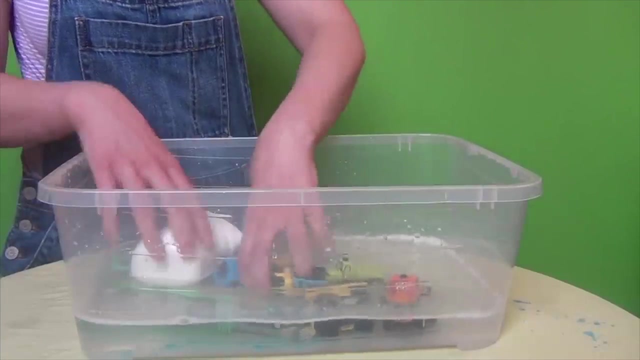 So silly That tickles. Thank you for cleaning me. We're having so much fun in the bath. Kaboom, Ooh, that's fun. I'm going to try that Kaboom. Okay, now it's time to rinse you off. 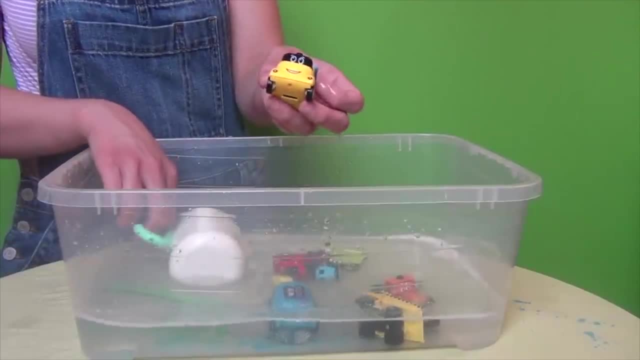 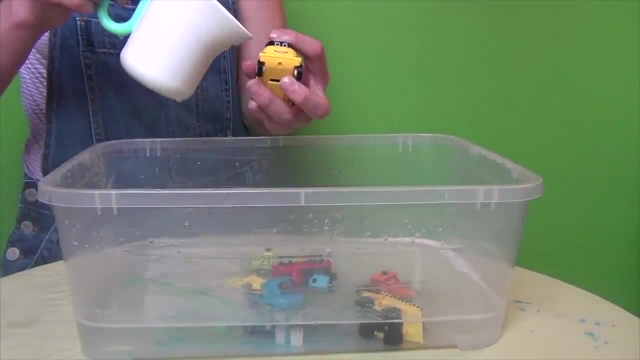 I'm scared. I don't want to be rinsed off. Oh, don't worry, It's not scary. I'm going to put my hand right here so I don't get any soap in your eyes. See, Okay, Ooh, that feels good Yeah. 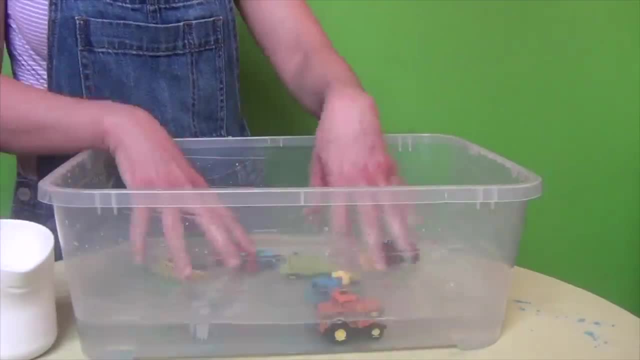 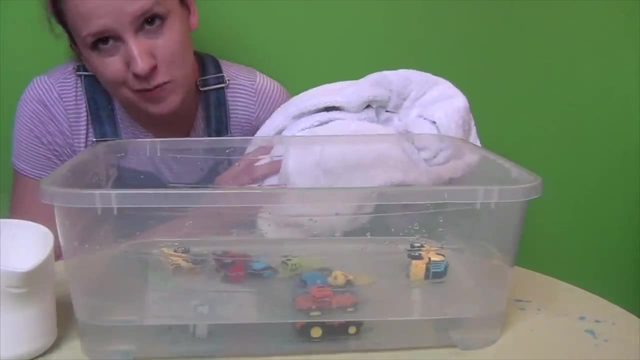 It's not scary. Baths are really fun. The cars are having fun in the water, but it's time to get out. I got a towel to dry off the cars and then we'll put them to bed, Taking the cars out. 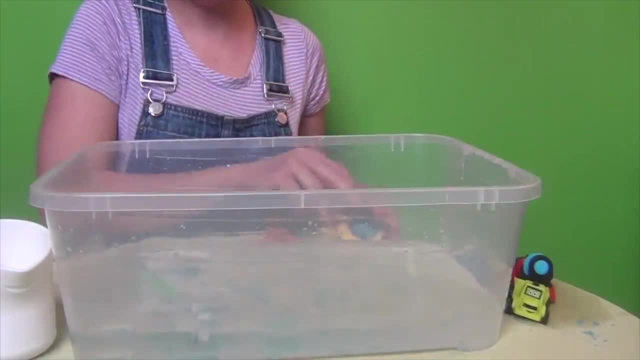 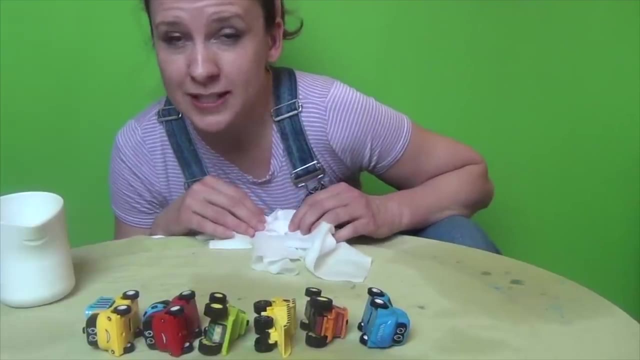 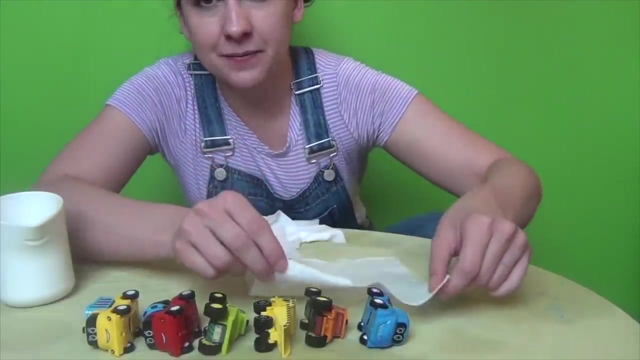 Out, Out. They're all done the bath All done, the bath All done. Now it's time for the cars to go to sleep. They're so tired. Good night, cars Shh. I'm going to give them a blanket. 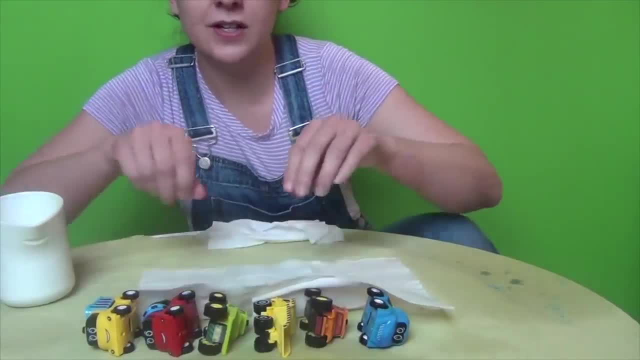 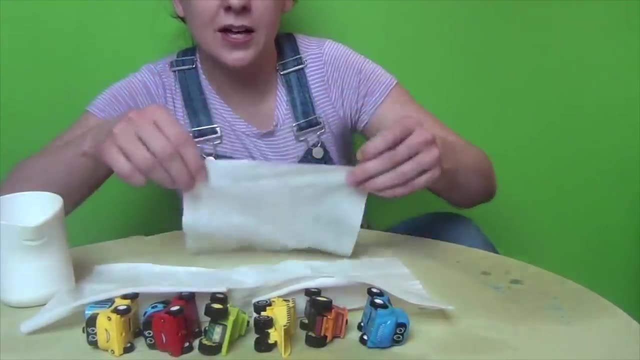 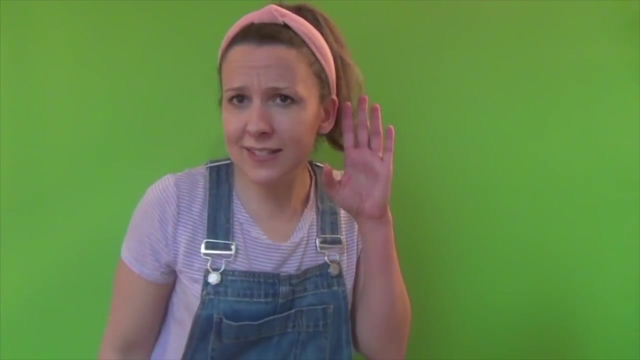 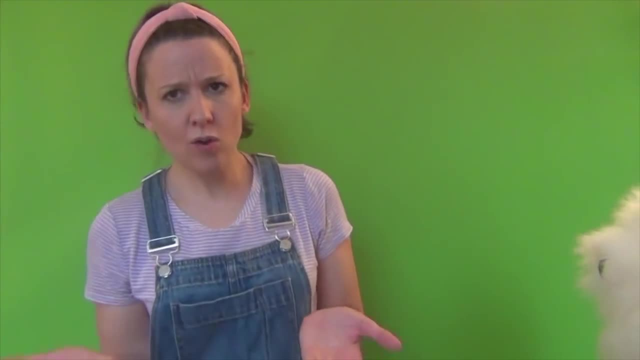 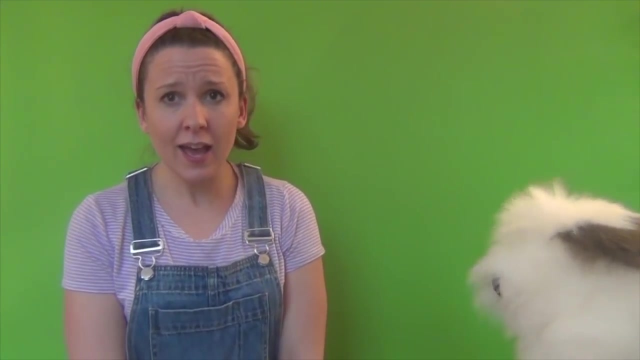 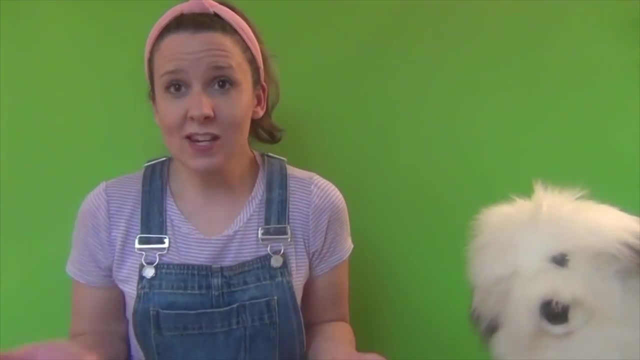 You're right, a dog. Oh, hi, It's our friend Bingo. Hi, Bingo, what's wrong? You look sad. I'm sad because I forgot how to spell my name. Oh, We can help you. Do you guys at home think you can help Bingo remember how to spell his name? 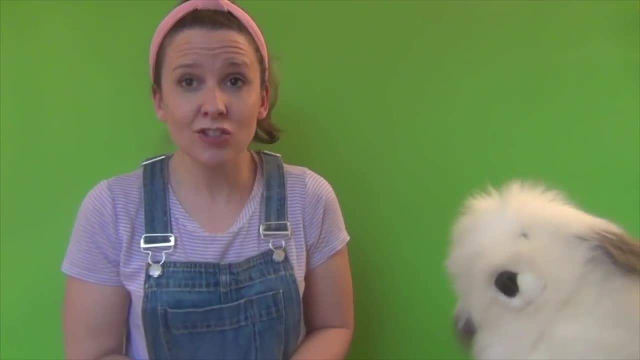 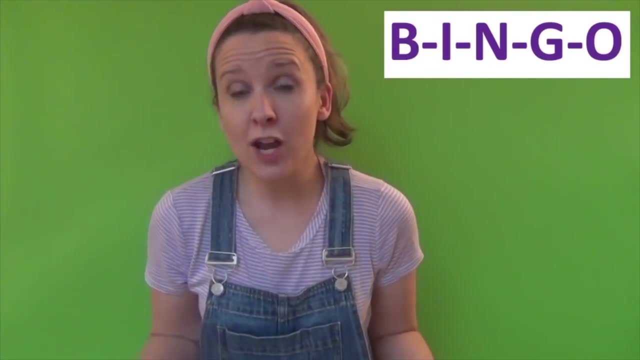 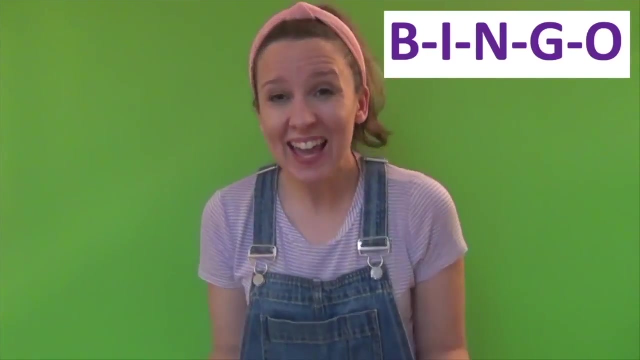 Can you help? Yeah, I bet if we sing the song Bingo, you'll remember. Okay, There was a farmer had a dog and Bingo was his name-o. B-I-N-G-O, B-I-N-G-O, B-I-N-G-O, and Bingo was his name-o. 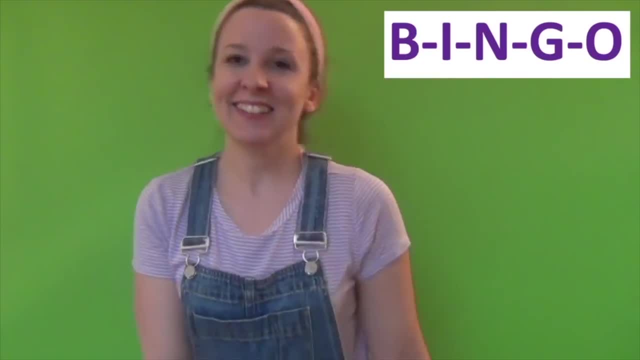 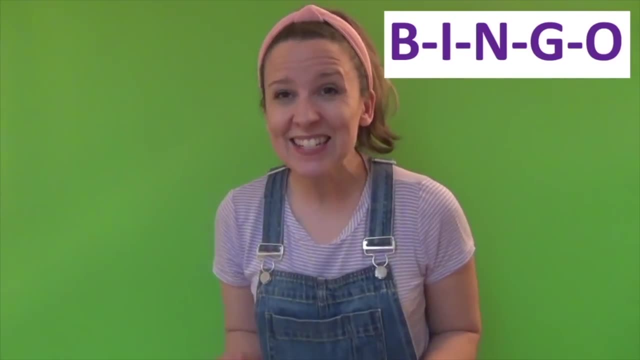 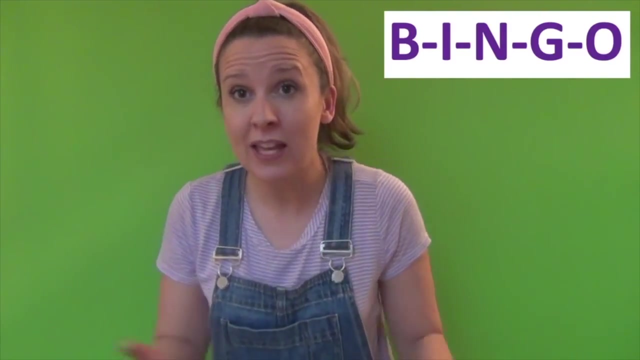 This time let's clap for the B. There was a farmer had a dog and Bingo was his name-o. I-N-G-O, I-N-G-O, I-N-G-O, and Bingo was his name-o. Now we clap for the B and the I. 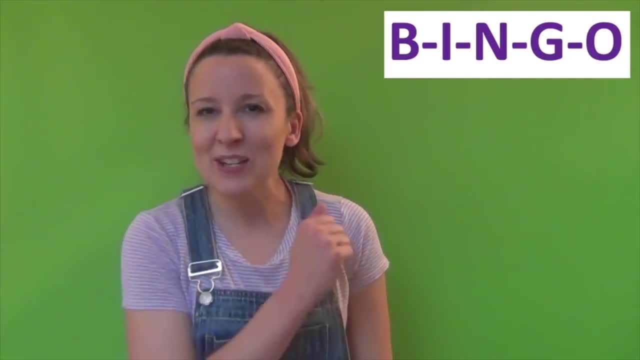 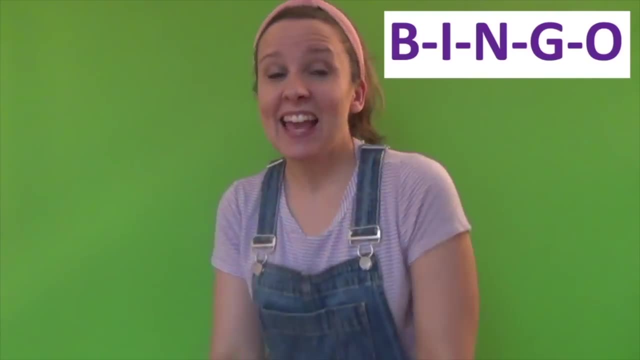 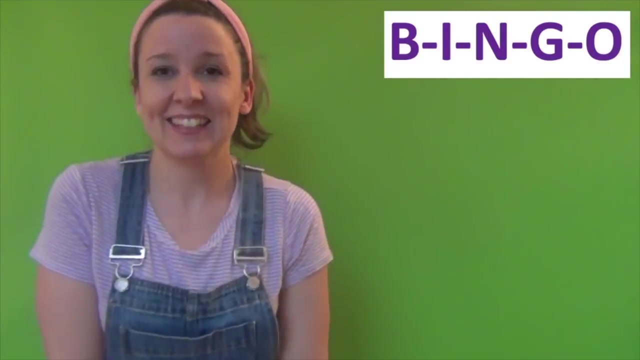 There was a farmer had a dog and Bingo was his name-o. N-G-O, N-G-O, N-G-O and Bingo was his name-o. Now for the B-I-N You ready. There was a farmer had a dog and Bingo was his name-o. 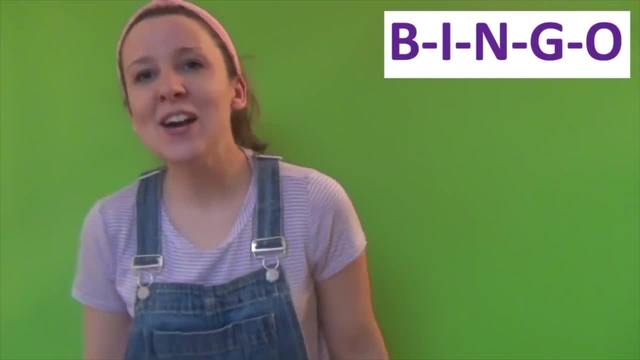 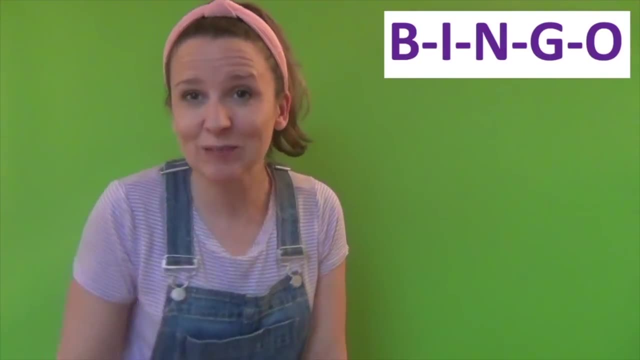 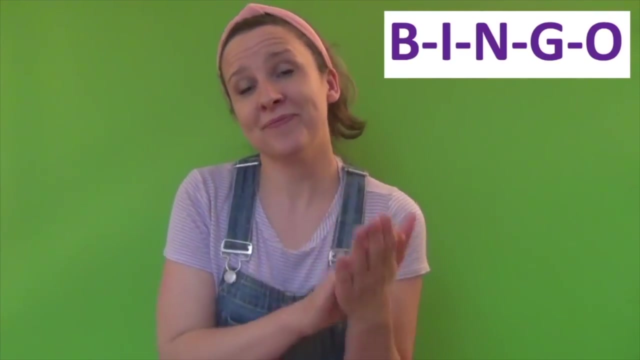 G-O, G-O, G-O, and Bingo was his name-o. Now for the B-I-N-G, There was a farmer had a dog and Bingo was his name-o. O, O, O and Bingo was his name-o. 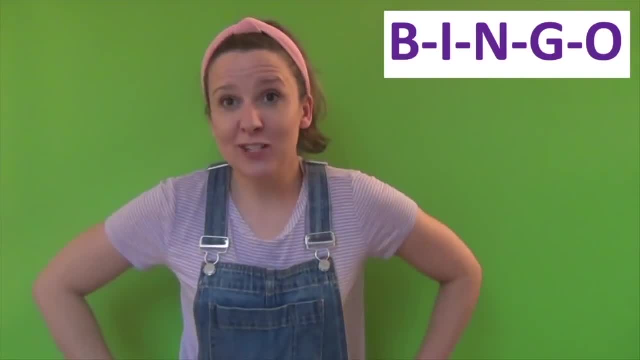 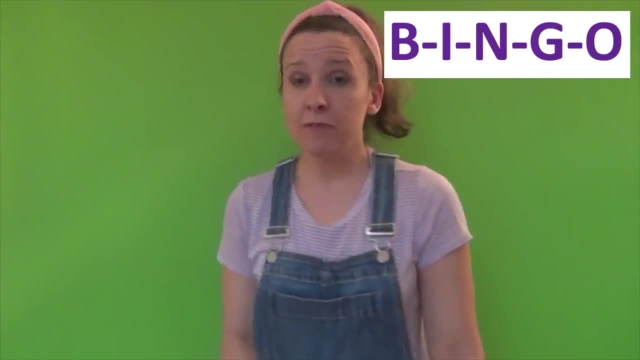 And Bingo was his name-o. Now we're going to do it for all the letters. It's going to be so tricky. Do you think you can do it? I know you can. There was a farmer, had a dog and Bingo was his name-o. 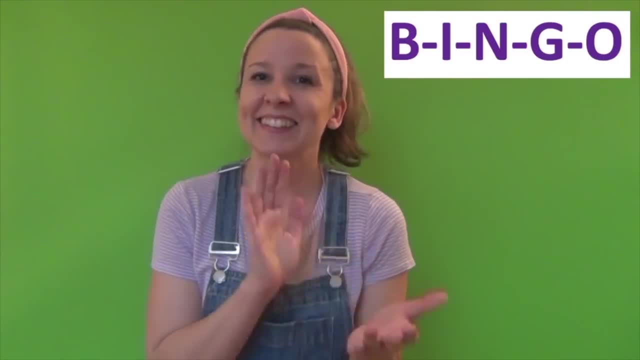 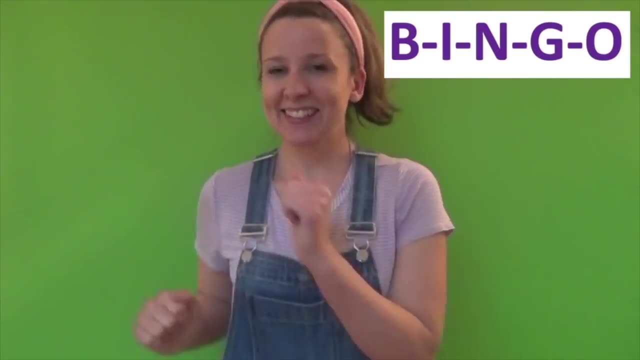 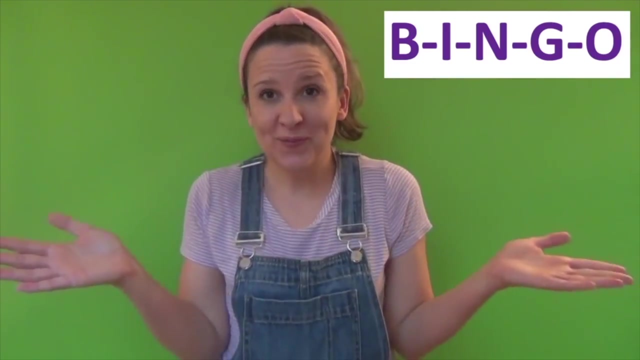 O O O and Bingo was his name-o. O O O and Bingo was his name-o And Bingo was his name-o. Yay, You guys did an amazing job, Thank you. Thank you so much. 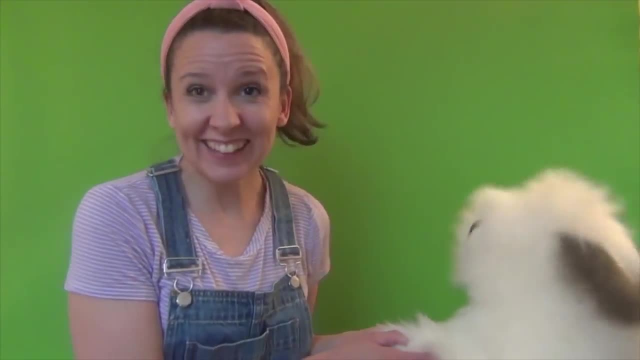 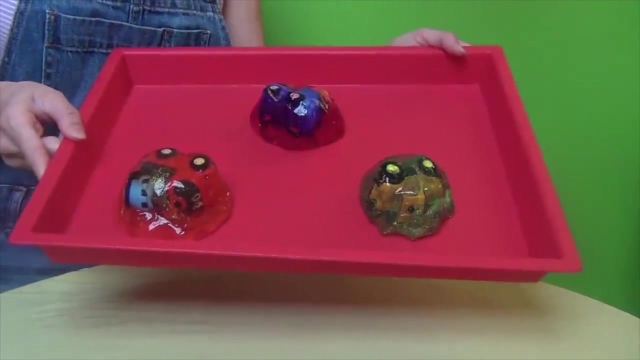 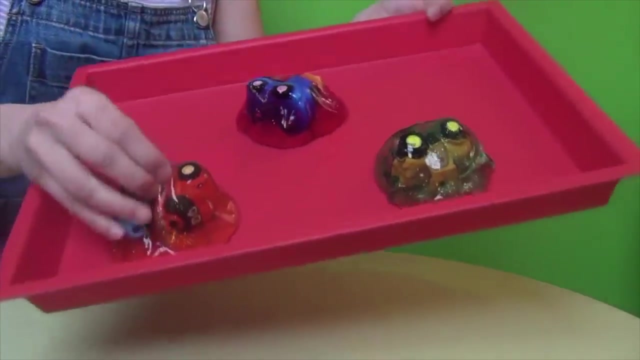 Do you remember how to spell your name? well, Now I know. Yay, Thank you, Thank you. Thank you so much, Thank you. Oh no, These cars have been slimed. They're covered in icky, sticky slime. 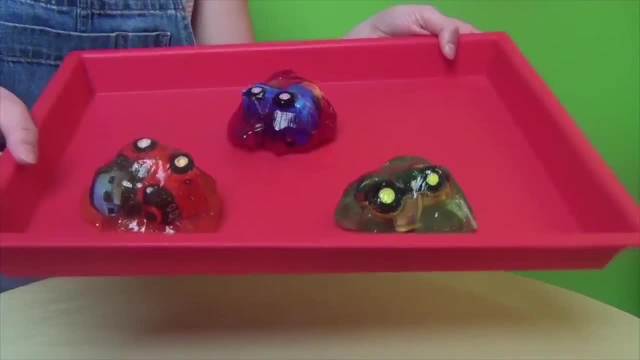 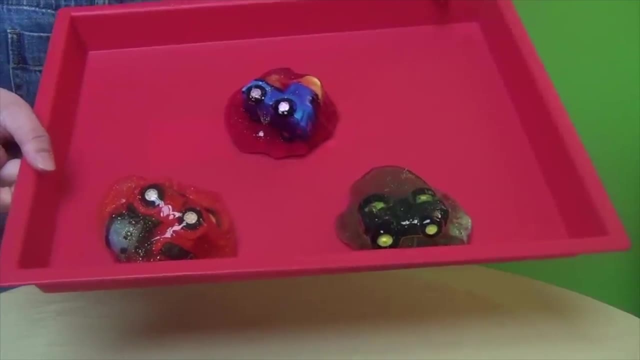 Can you help me get them out? Help us get out of the slime. Can you help us? Yeah, we can help. Let's say out, and that will get them out of the slime. Wow, They're really covered in slime. 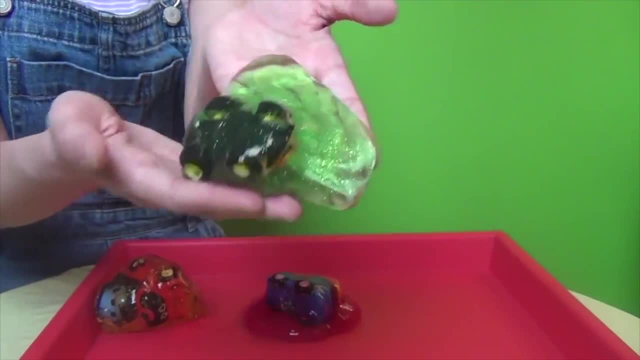 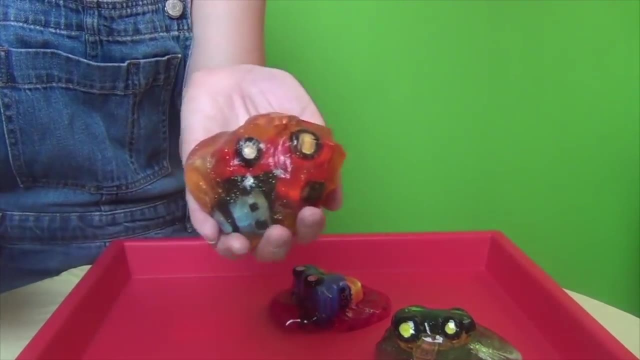 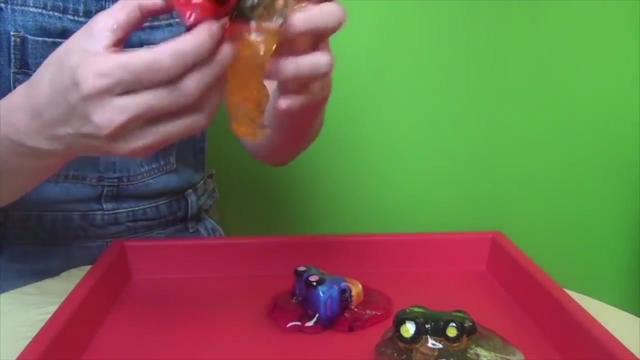 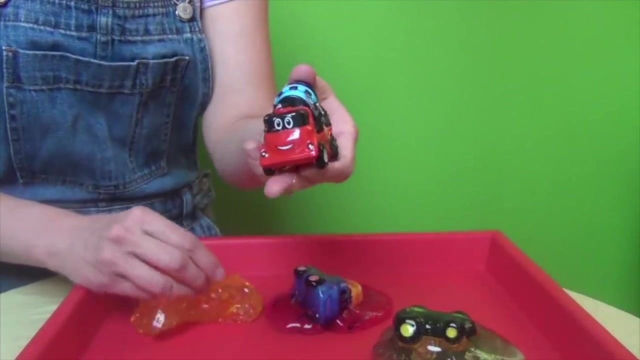 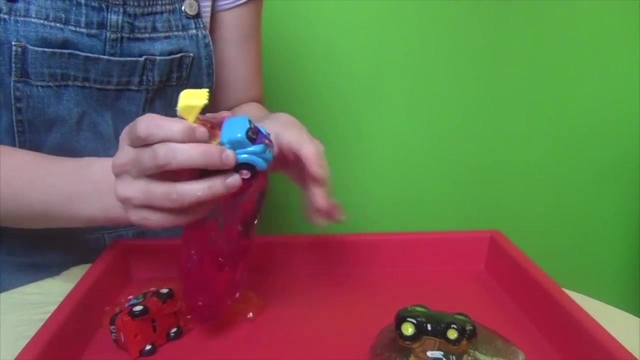 Covered in slime And covered in slime. Say out, Out, Out. It's coming out. Thank you so much. I'm so happy to be out of that slime. Say out Out. Wow, Thank you, I'm so happy to be out of the slime. 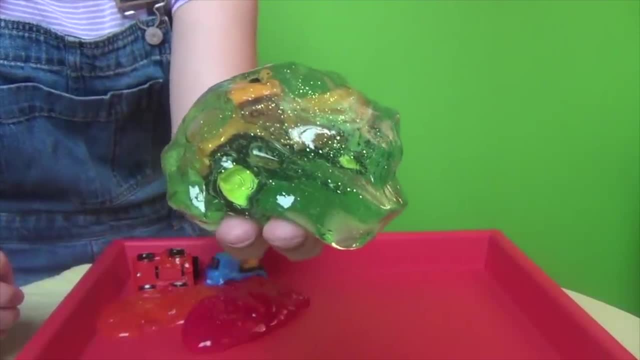 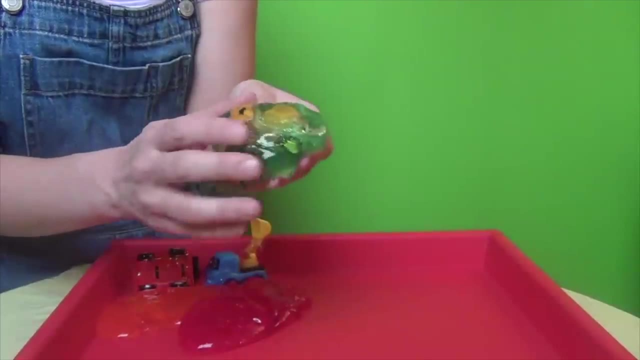 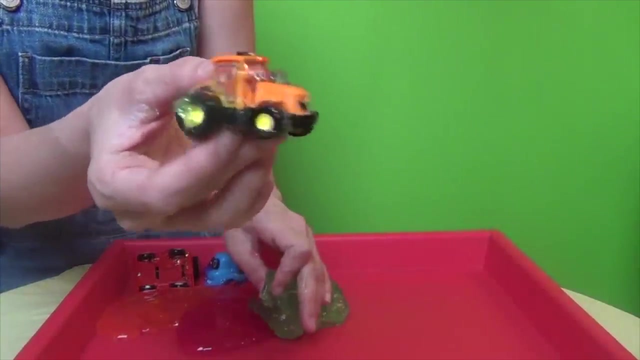 Thank you so much. Can you get me out of the slime? Yes, we can Say out One, two, three Out. He's getting out of the slime. Oh, thank you so much. You did such a good job saying out. 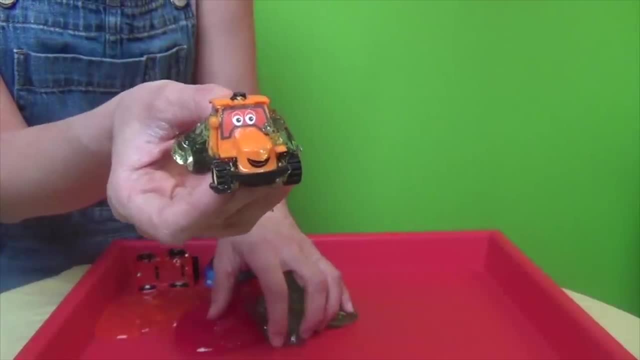 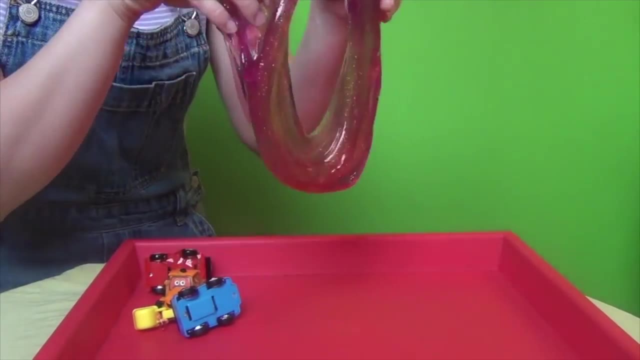 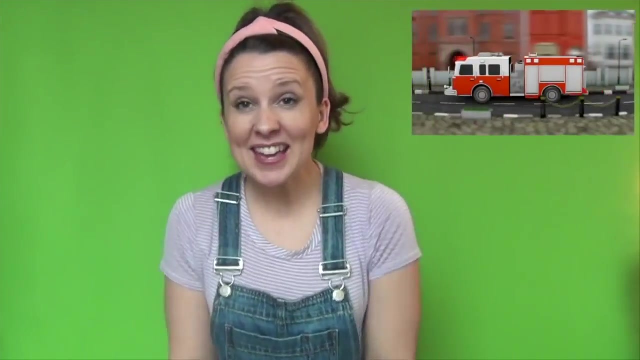 I feel better, but I think I need a bath. Ew, Look at all this slime. You saved the cars from all this icky, sticky slime. Great job. Okay, let's get into our fire truck. Are you ready? 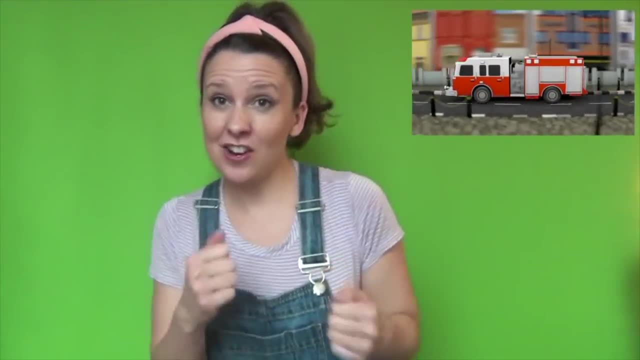 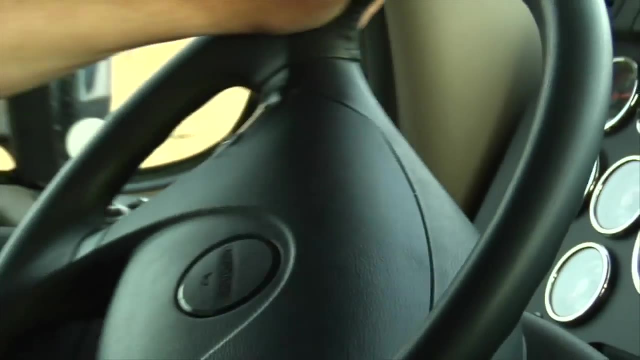 Hurry, hurry, drive the fire truck. Hurry, hurry, drive the fire truck. Hurry, hurry, drive the fire truck. Ding, ding, ding, ding ding. Now it's time to turn the corner. Hurry, hurry, turn the corner. 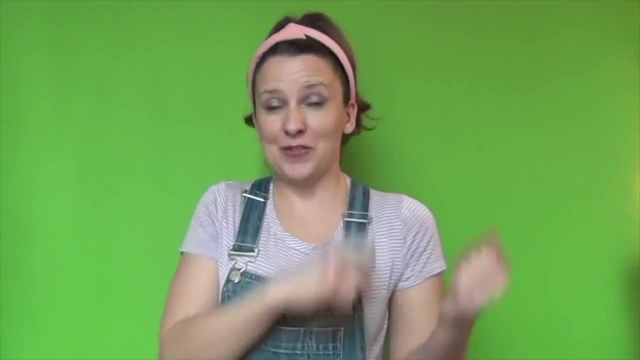 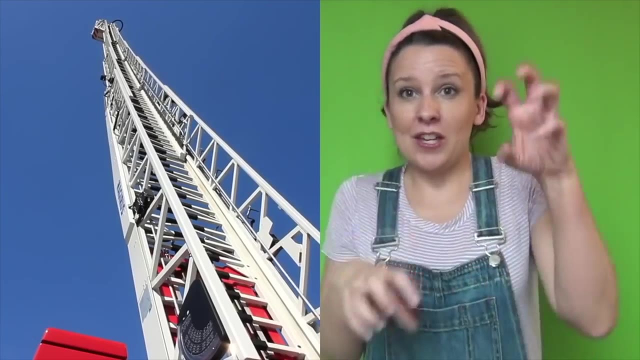 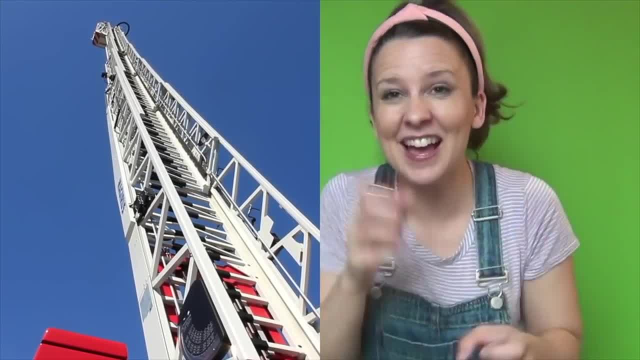 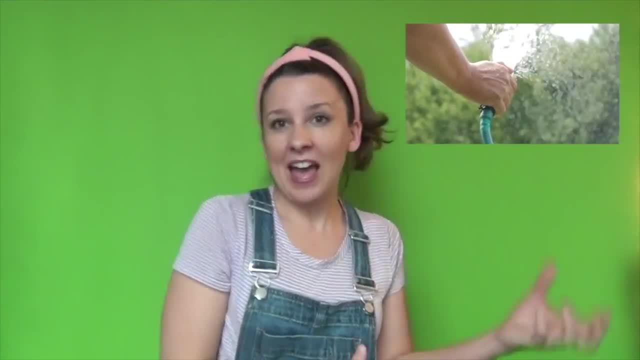 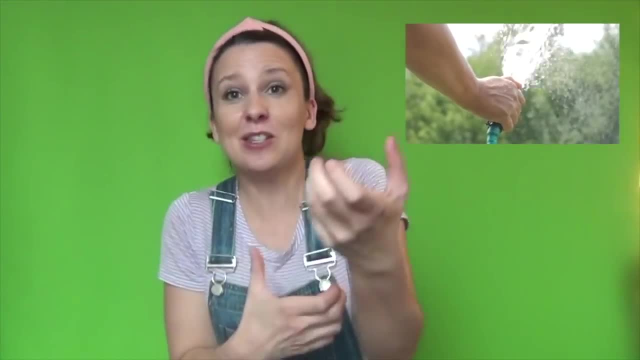 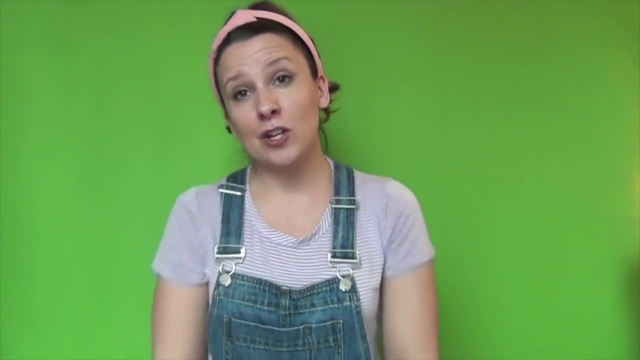 Hurry, hurry squirt the water. Hurry, hurry squirt the water. Ding ding, ding, ding ding. We did it. We put out the fire. Great job. Now we're gonna go back to the station slowly. 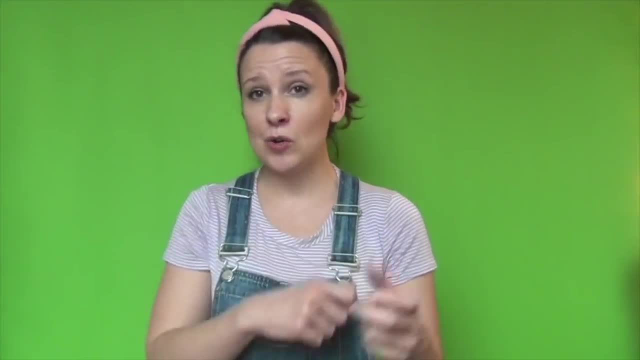 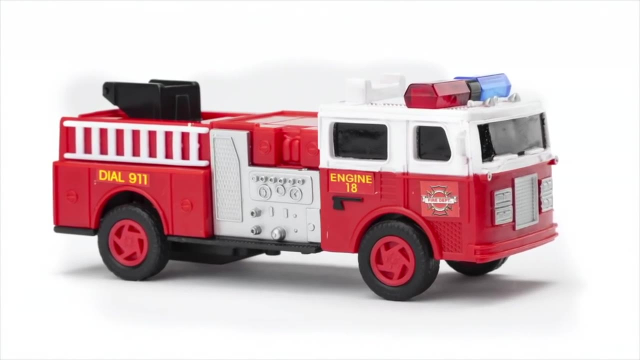 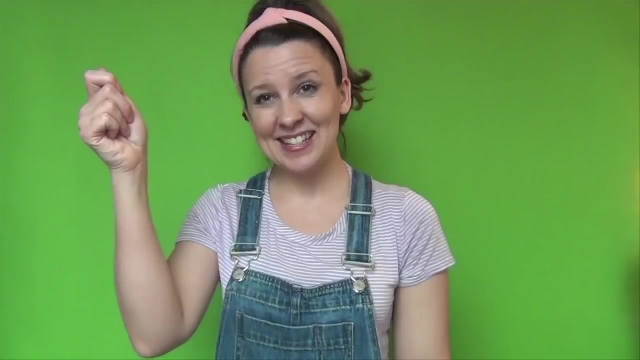 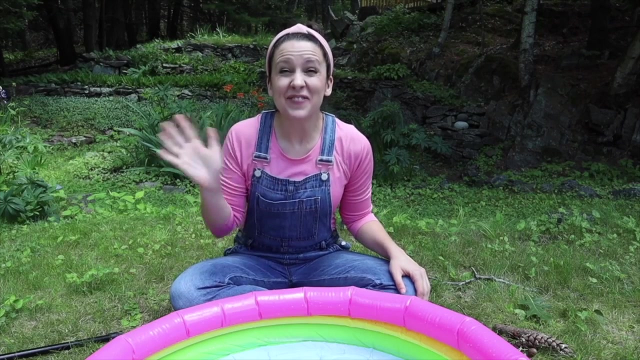 Slowly, slowly back to the station. Slowly, slowly back to the station. Slowly, slowly back to the station. Ding, ding, ding, ding ding. Great job, firefighters. High five, Hi friends, I'm so excited. 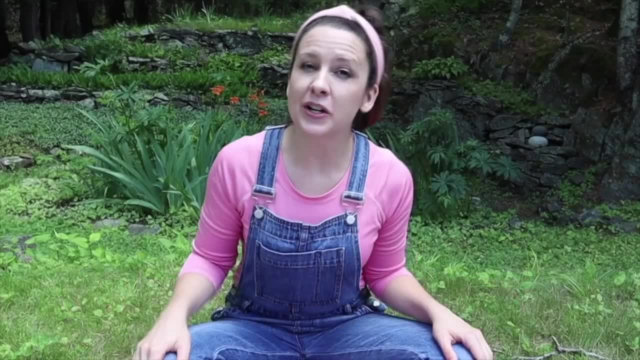 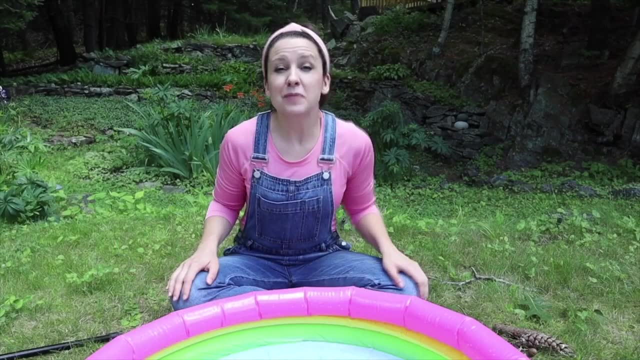 We're going to do a science experiment. We're going to see what sinks and what floats. I can't wait to try it. I found some things in the yard outside And I found some things in my house inside. Okay, let's do the experiment. 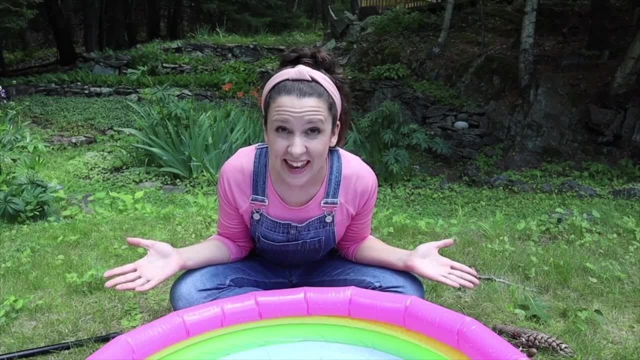 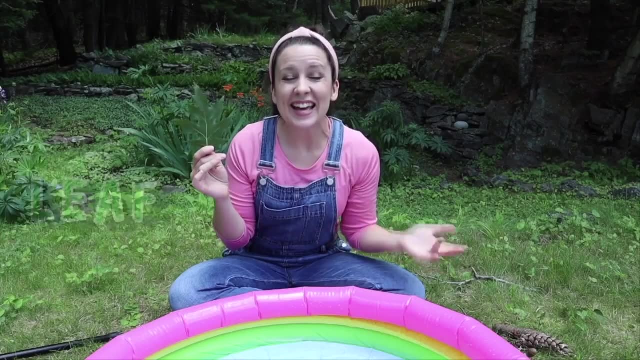 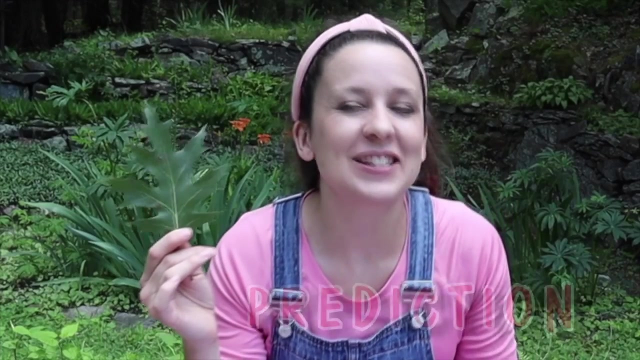 I need your help. Can you help? Let's start with this. What is this? Yeah, it's a leaf. Do you think it's going to sink or float? What is your prediction? Sink or float? Hmm, Let's try it and see. 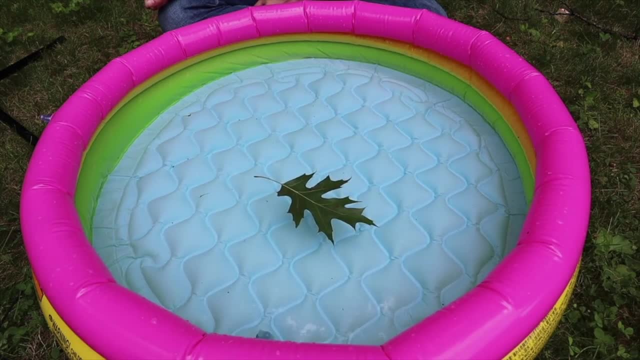 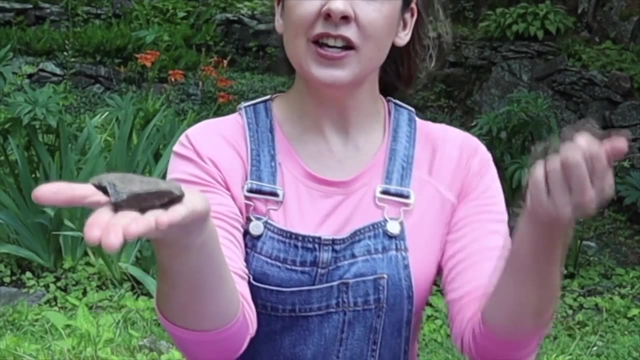 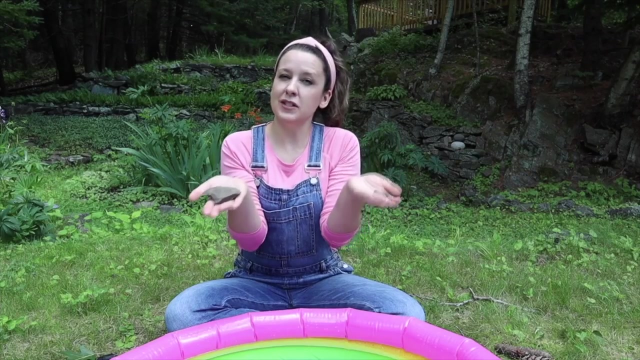 It's floating, Wow. Next we have two rocks, And two is the number of the day. One, two. I have a big rock and a small rock. Do you think these rocks will sink or float? What is your prediction? 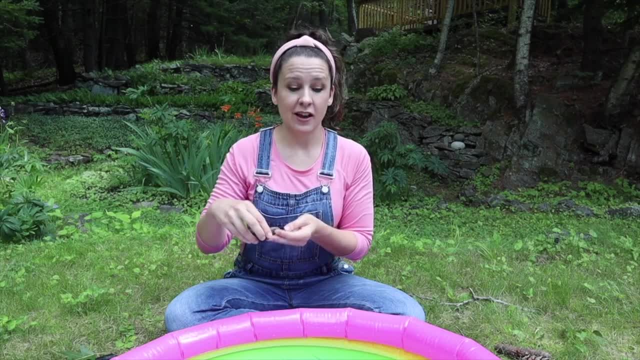 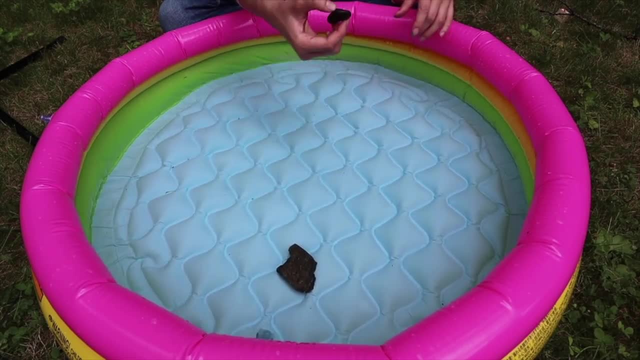 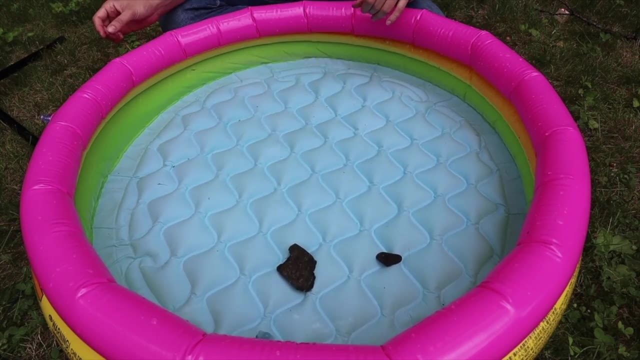 Okay, let's try the big rock first, Ready, set, go. It sunk to the bottom really fast. What do you think will happen with the little rock? Will it sink too? It sunk really fast too. The big and the small rock both sunk. 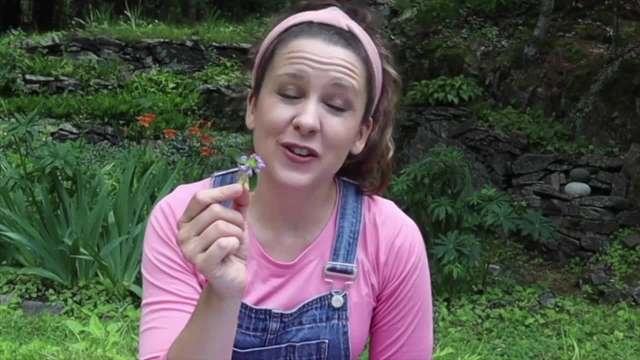 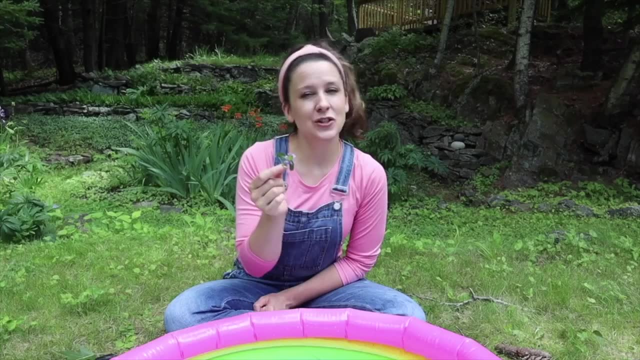 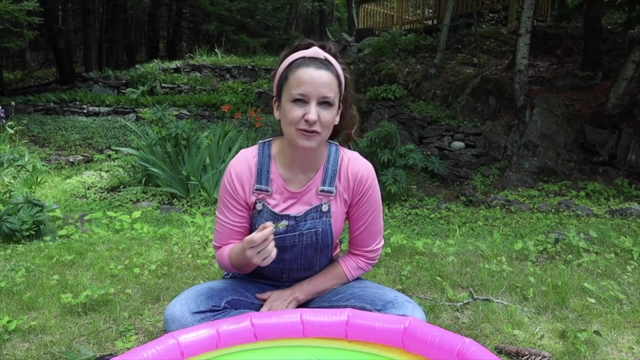 Guess what I found in my yard: A beautiful flower. Yeah, What color is this? It's purple. Do you think it's going to sink or float? Hmm, What's your prediction? I think it's going to float. Let's try. 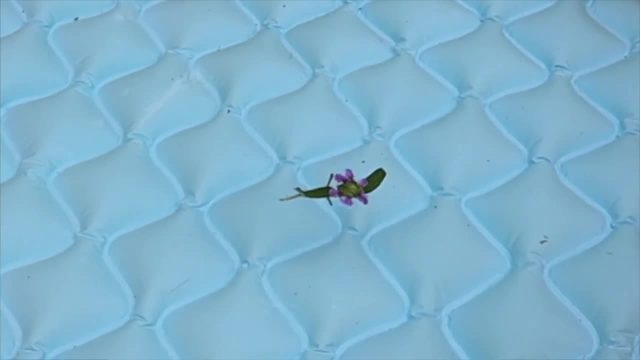 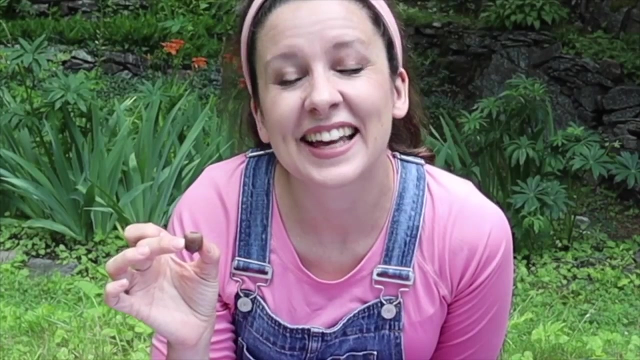 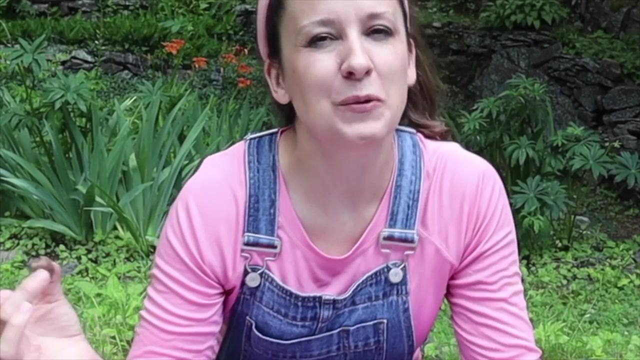 It's floating. Wow, We were right. Next, I found this. Do you know what this is? Yeah, It's an acorn. Let's put it in and see if it sinks or floats. What's your prediction? What do you think is going to happen? 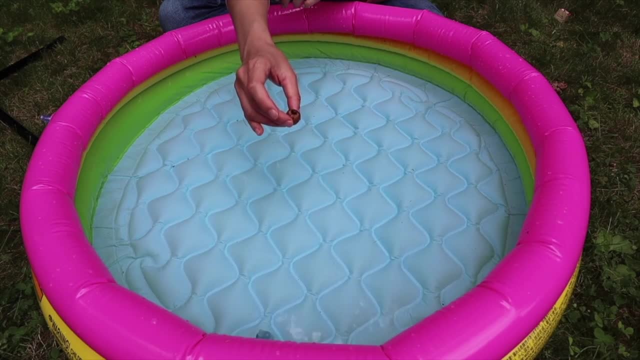 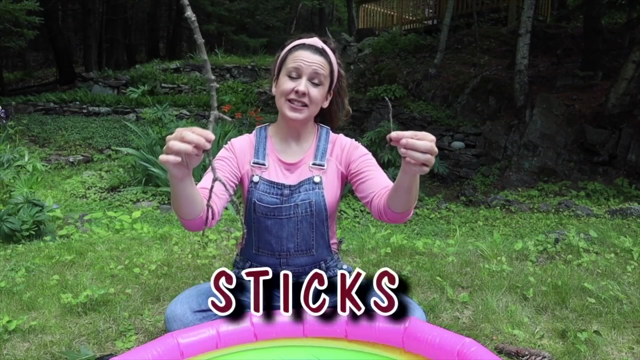 Okay, Let's try it. Ready set go. Wow, It's floating. I thought it was going to sink. The acorn is floating, Wow, Look what I found. How many sticks do I have? One, two, 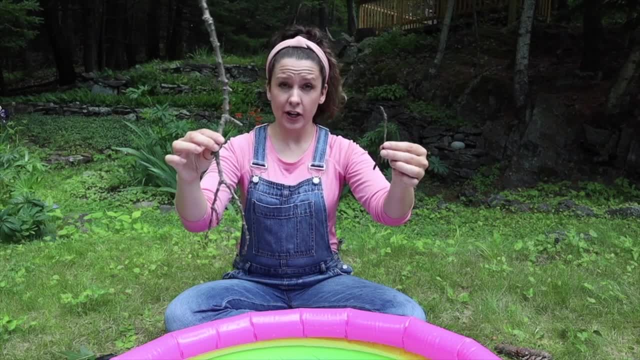 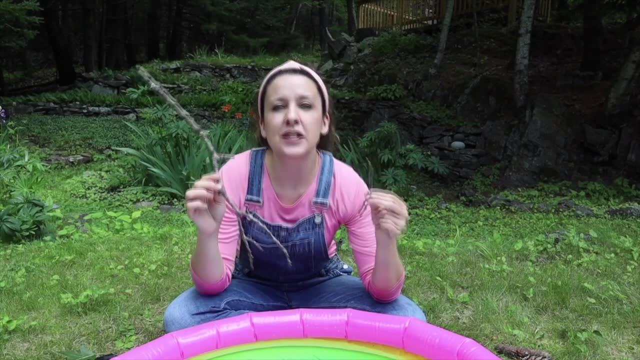 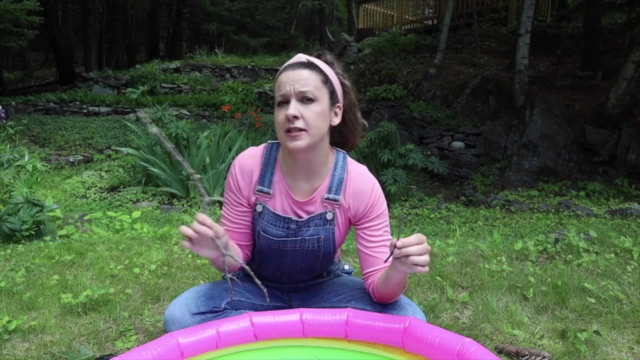 Two sticks. Which stick is bigger? Yeah, This stick is bigger and this stick is smaller. Do you think they'll both sink or both float? Hmm, I think the big stick will sink and the little stick will float. That's my prediction. 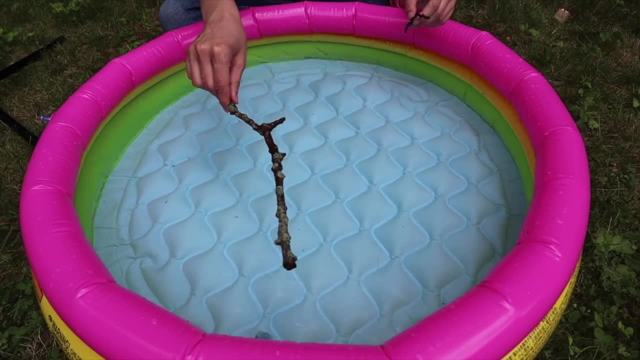 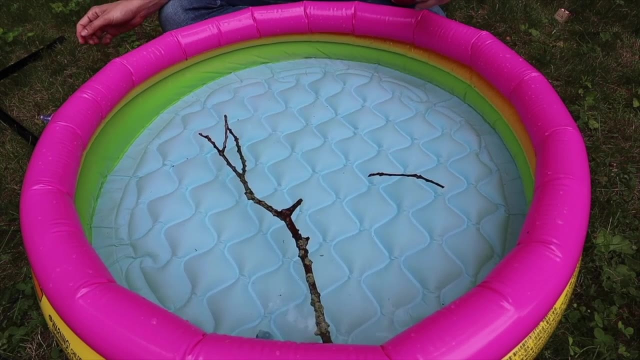 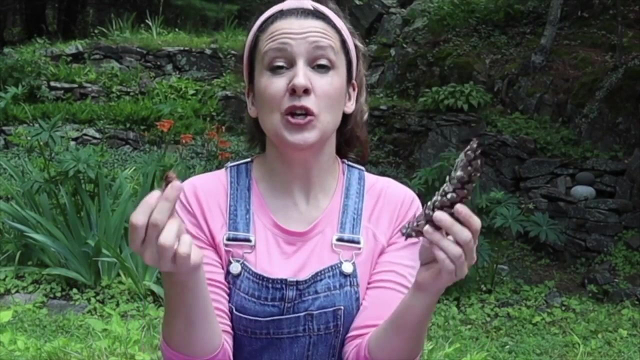 Let's see what happens. The big stick is floating. Wow, The little stick is also floating. I was wrong. Since the number of the day is two, I have two pine cones: A big pine cone and a little pine cone- So cute. 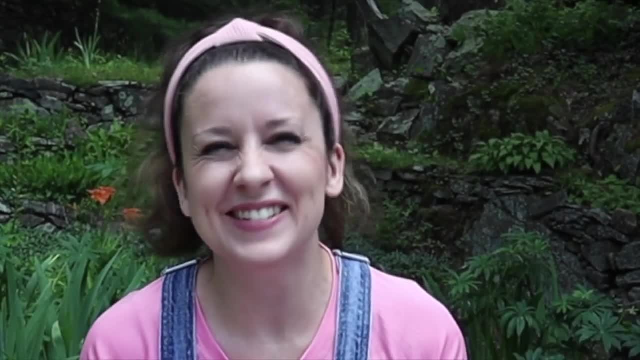 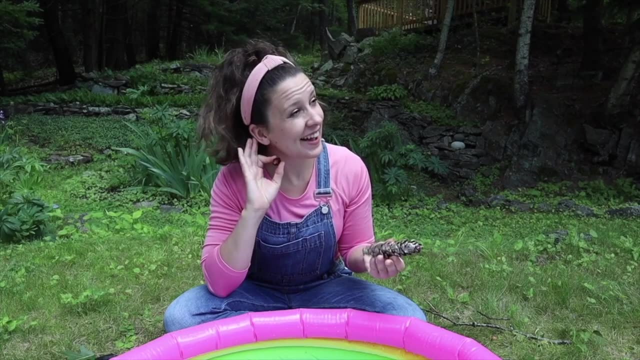 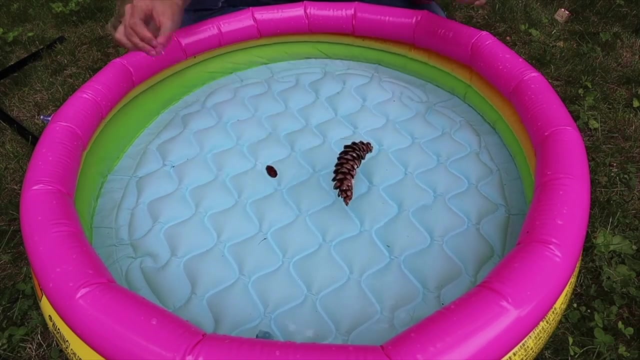 Is it a little nose? No, So silly. Okay, Do you think these pine cones will sink or float? Yes, Okay, Let's see what happens. I'm going to put them in, at the same time Putting them in the water. 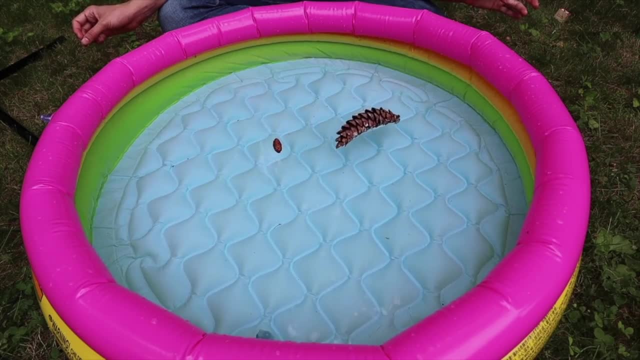 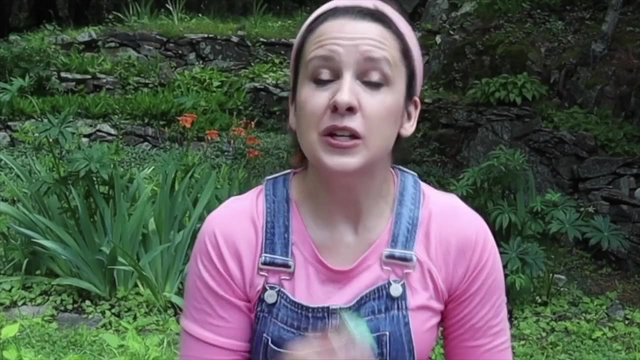 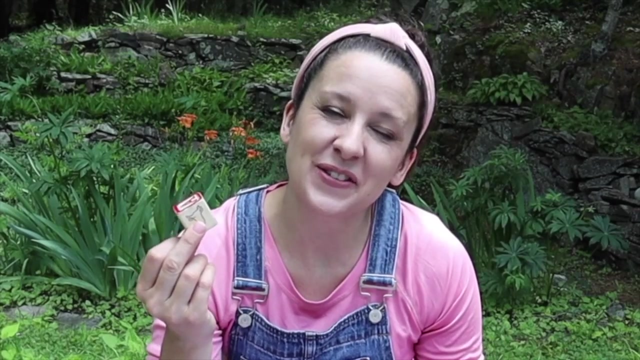 They're both floating. Wow, Now let's try things from inside my house. Are you ready? Do you know what this is? Yeah, It's a block. Do you think it's going to sink or float? What's your prediction? 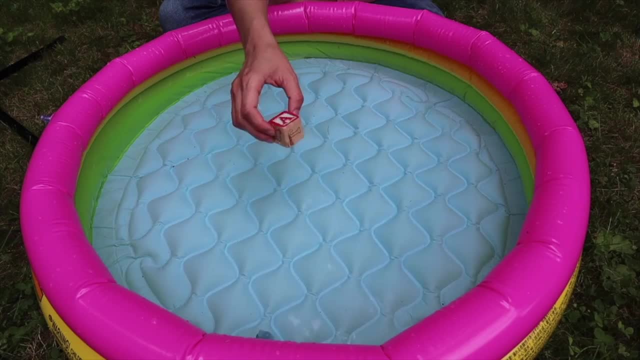 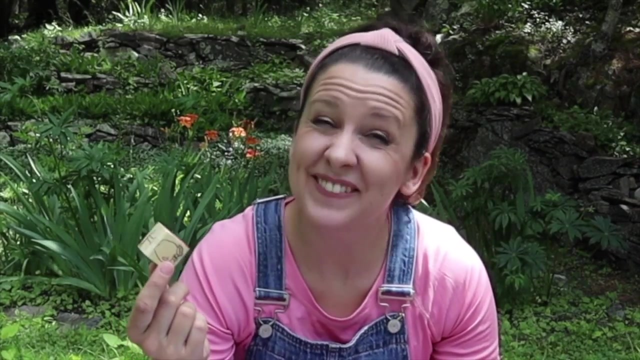 Hmm, Let's try it. Ready set go. Wow, The block floats. Wow, That's cool. Do you know what this is made out of? The block is made out of wood. Wow, This penny is really small. 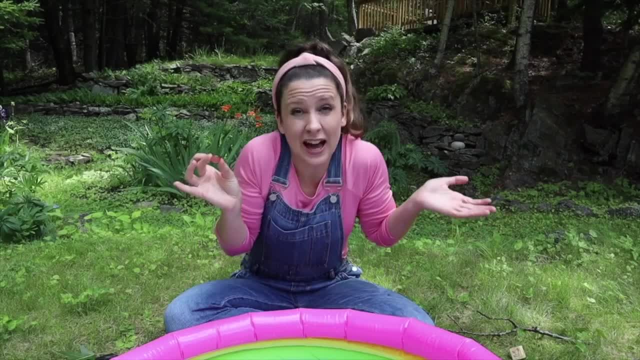 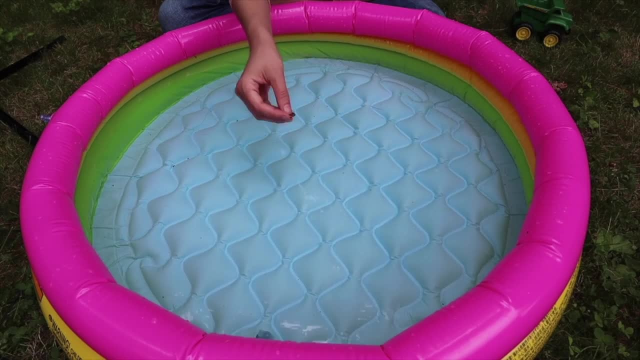 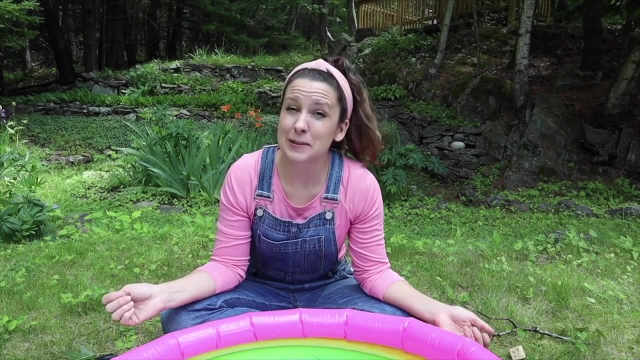 Do you think it will sink or float? I don't know. Let's try it and see Ready set go. The penny sunk. Wow, The penny is now on the bottom of the pool. The penny must be pretty dense. 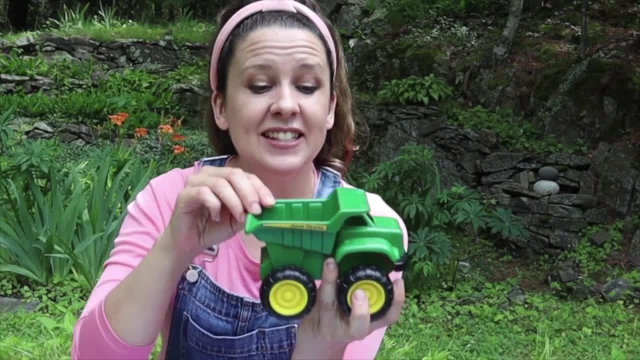 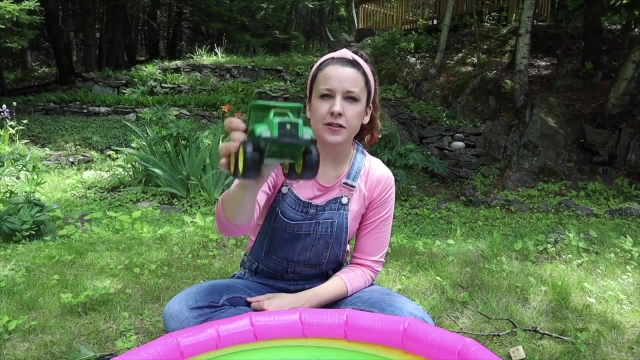 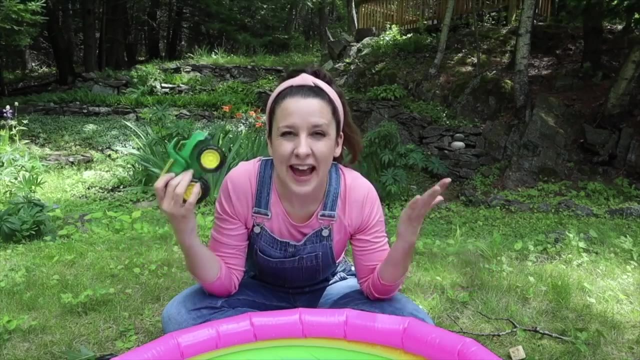 Do you know what this is? It's a dump truck. It's green. I like it. Do you think it will sink or float? Hmm, I don't know. Mrs Dump Truck, Let's see what happens. Put me in the water. 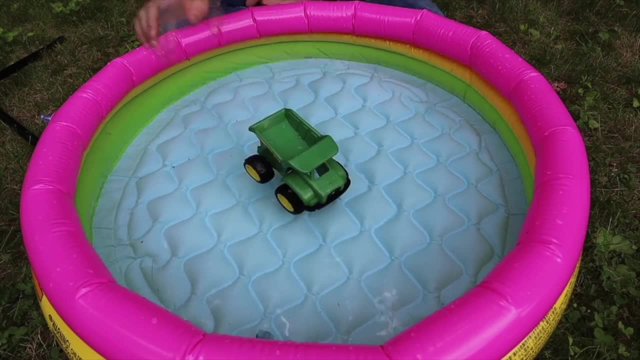 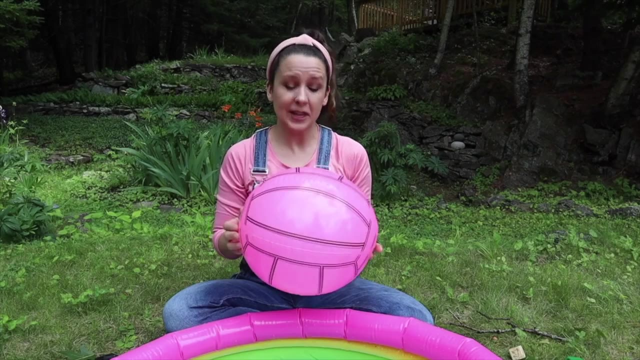 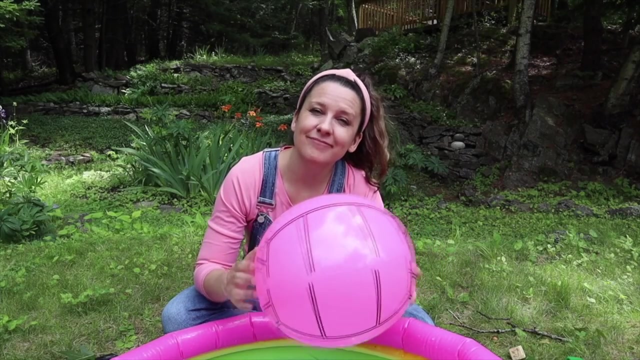 The water is cold. I like it. Wow, I am floating. Look what I found: A beach ball. It's pink. Do you think this beach ball will sink or float? Hmm, Let's try it. Wow, It's floating. 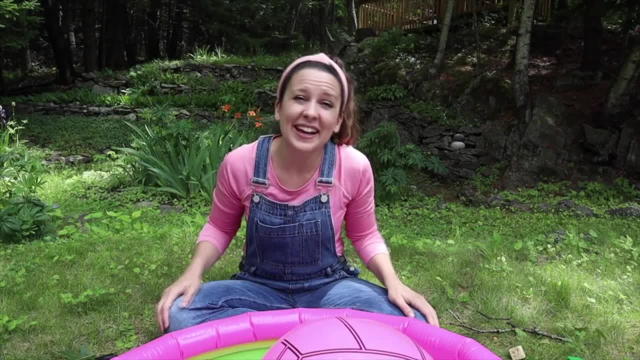 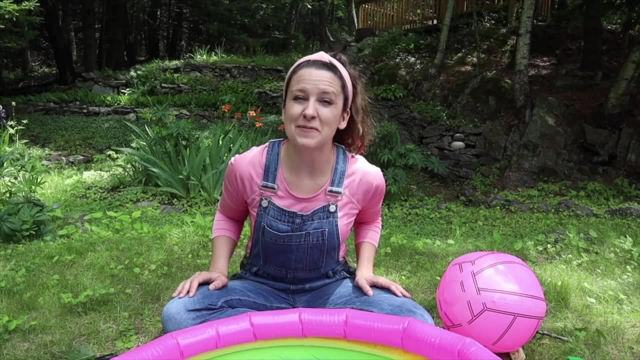 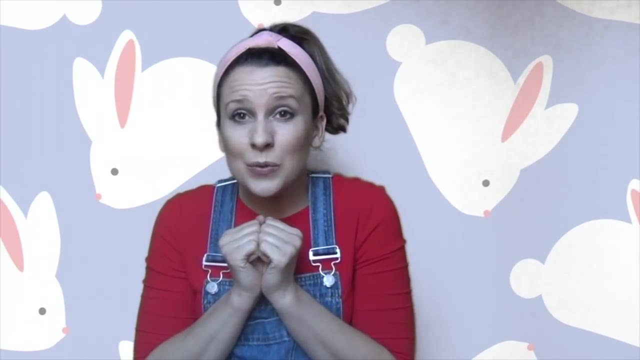 Wow, It's really big, but it's floating Cool. It must not be that dense. That was a really fun science experiment, Great job. See the bunnies sleeping till it's nearly noon. Shall we wake them with a merry tune. 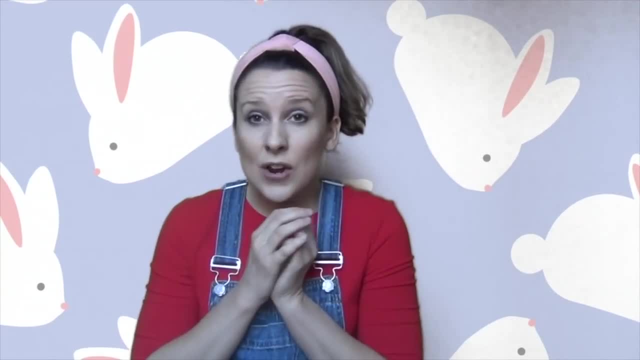 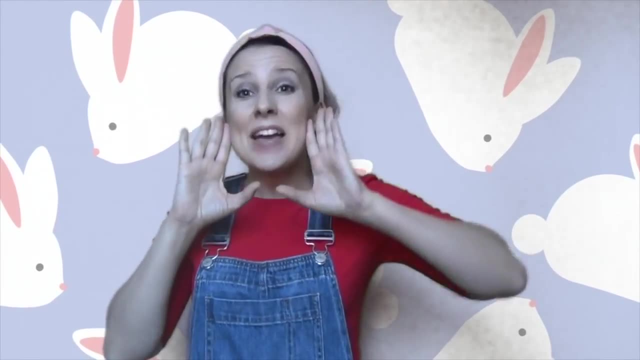 They're so still, Are they ill? Wake up soon. This is the loud part. Wake up. little bunnies Hop. little bunnies, Hop, hop, hop, Hop. little bunnies, Hop, hop hop. 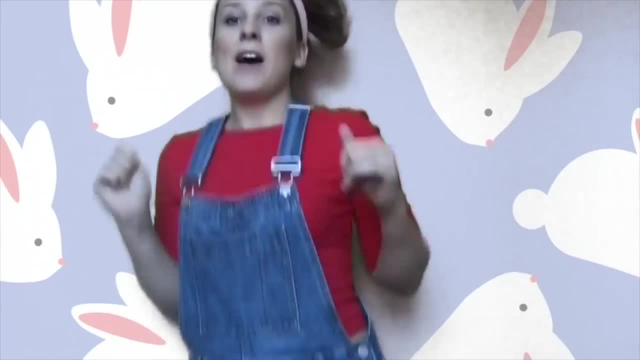 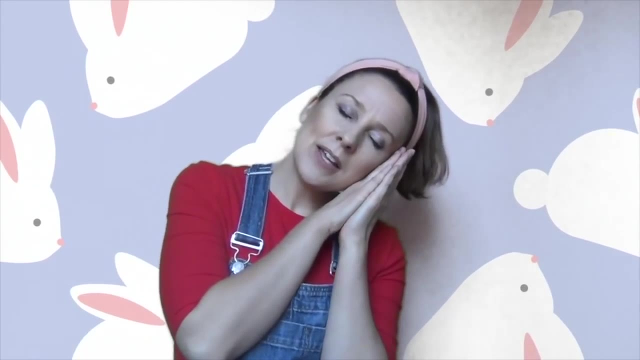 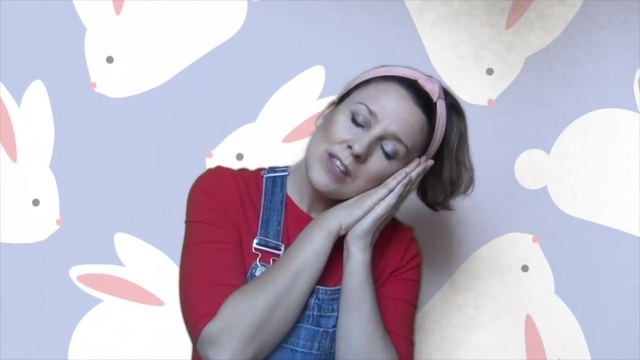 Hop, little bunnies, Hop, hop, hop, Hop, hop, hop and stop. Now we're going to be quiet again. See the bunnies sleeping till it's nearly noon. Shall we wake them with a merry tune. 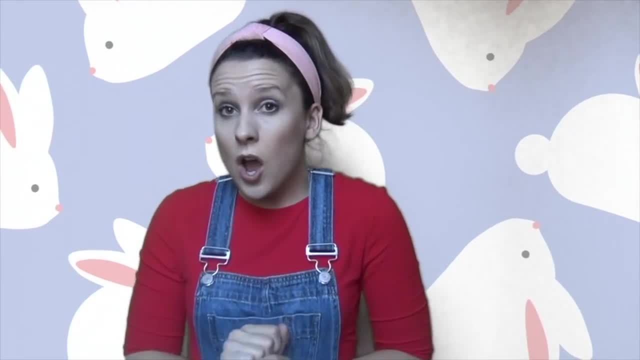 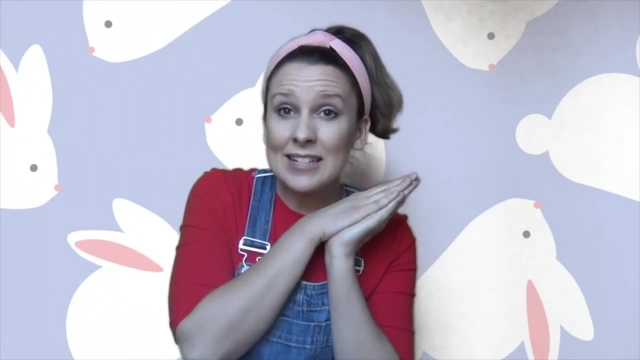 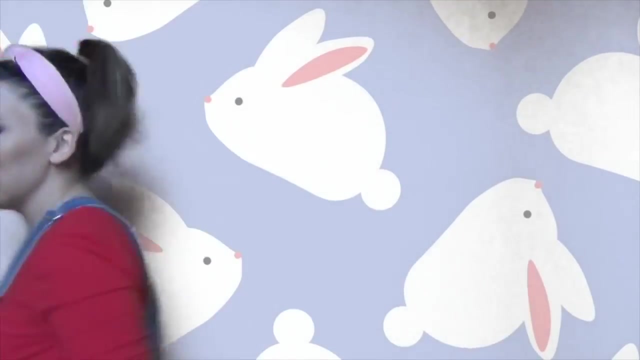 They're so still Are they ill? Wake up soon. Ding ding, ding, ding ding. That's the alarm clock. Wake up. little bunnies, Skip, little bunnies, Skip, skip, skip, Skip, little bunnies, Skip, skip, skip. 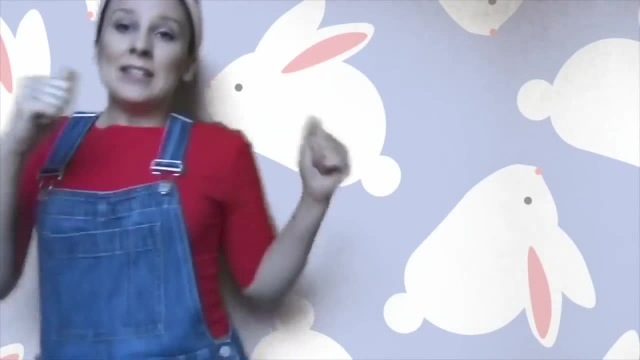 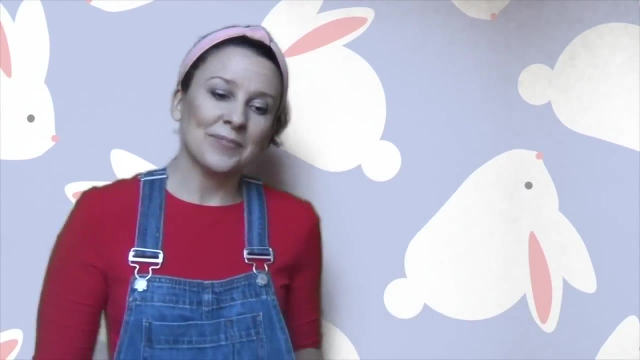 Skip little bunnies, Skip, skip, skip, Skip, skip, skip and stop. Should we hop again? Let's do it. Are you ready? Time to hop? Hop little bunnies, Hop, hop, hop. 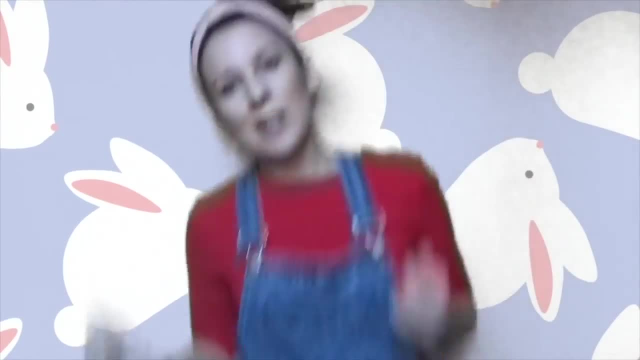 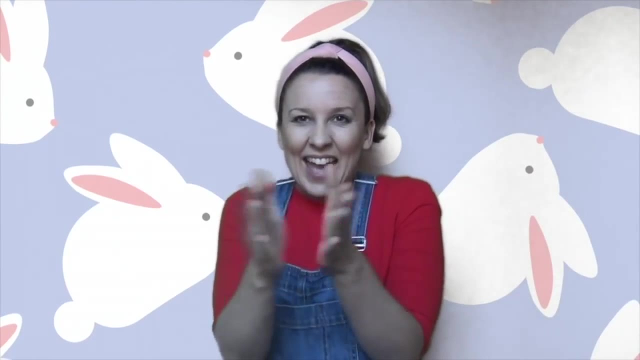 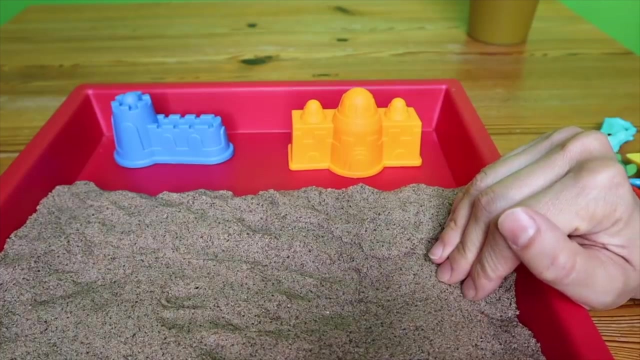 Hop little bunnies: Hop, hop, hop, Hop little bunnies: Hop, hop, hop, Hop, hop, hop and stop. Yay, Great job. Okay, friends, For our sensory activity today we have kinetic sand. 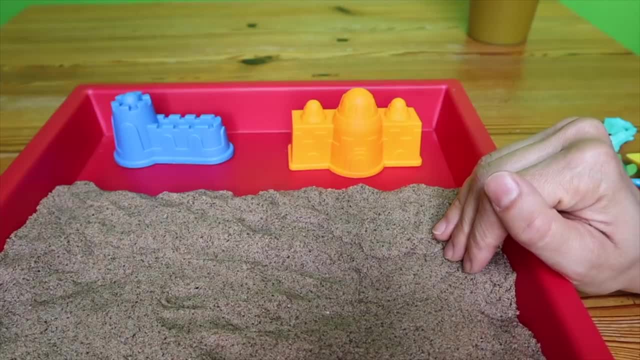 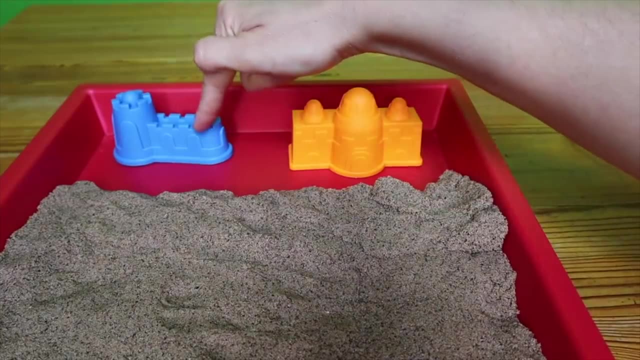 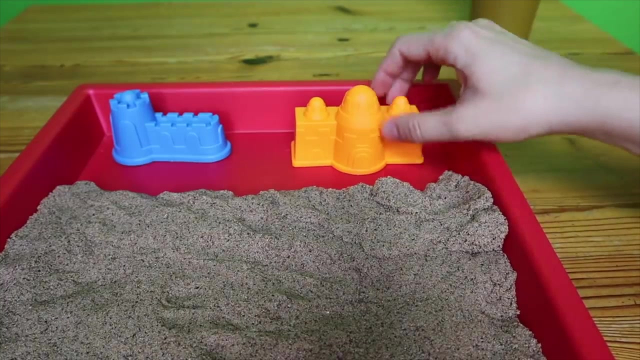 It's going to be so much fun to play with. We're going to make sand castles. Let's see how many sand castle molds we have: One, two, Two sand castle molds, and that's the number of the day. Okay, so to make the sand castle, we have to put the sand into the mold. 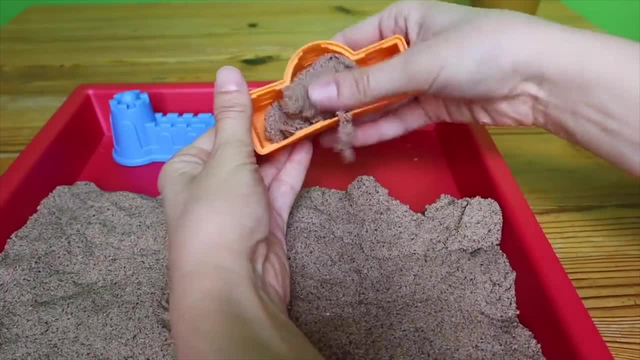 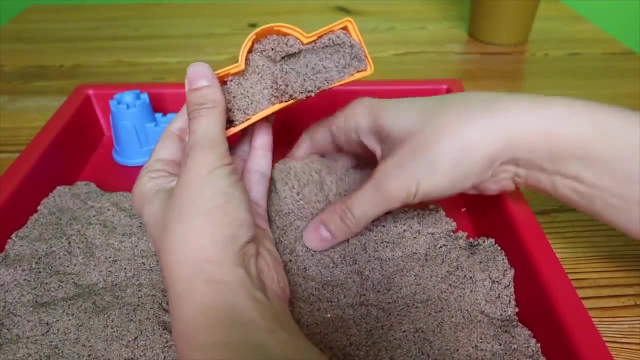 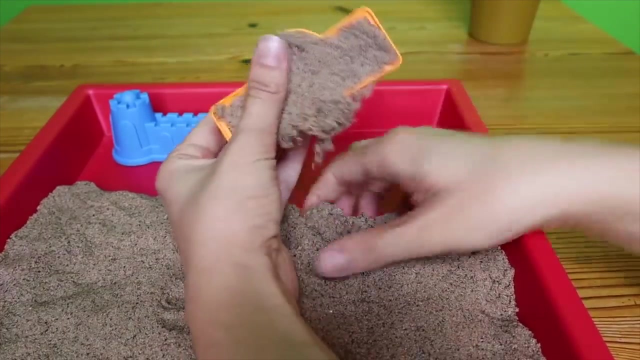 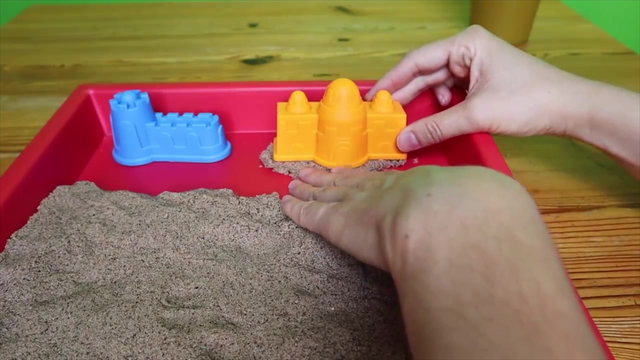 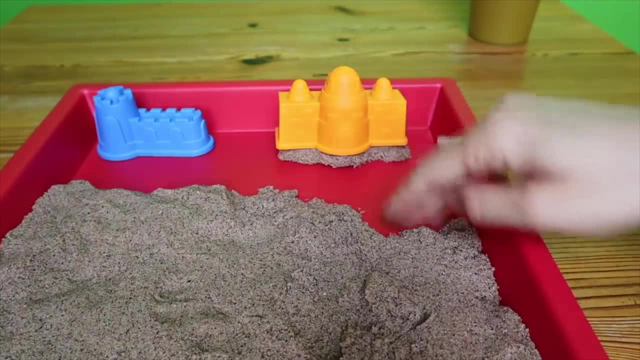 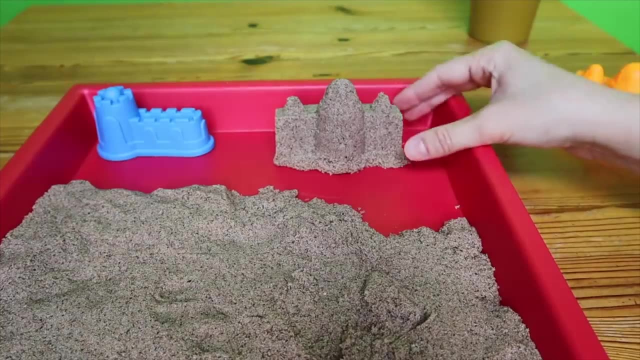 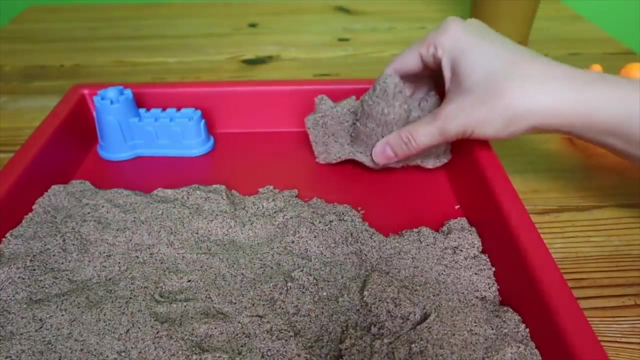 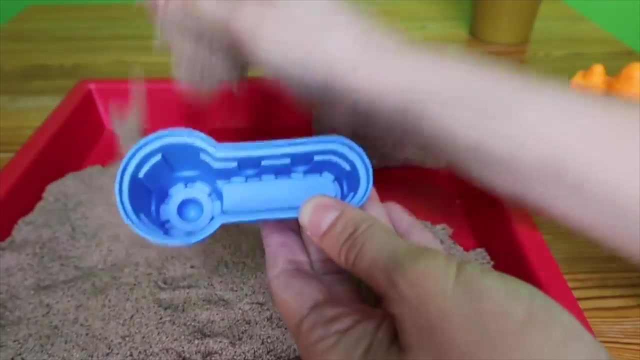 Are you ready? Yay, Ready set, say go, Go. Oh, it worked. We made a beautiful sand castle, So fun, Let's make the other one. So we're going to put the sand in again. Put it in. 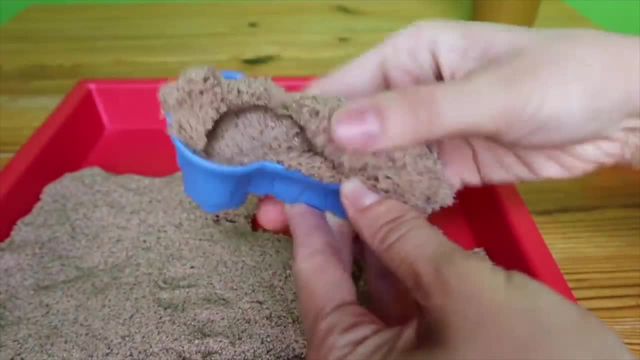 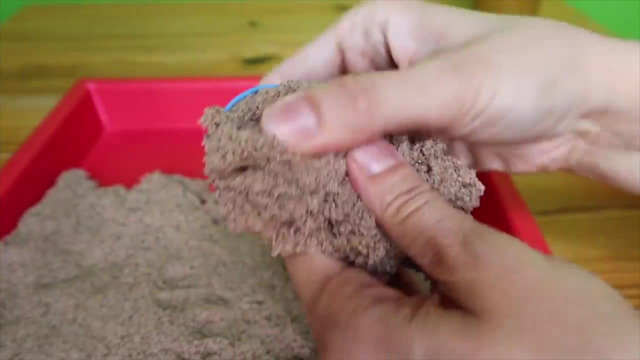 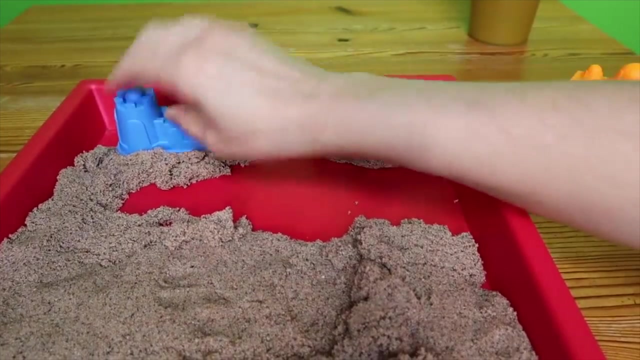 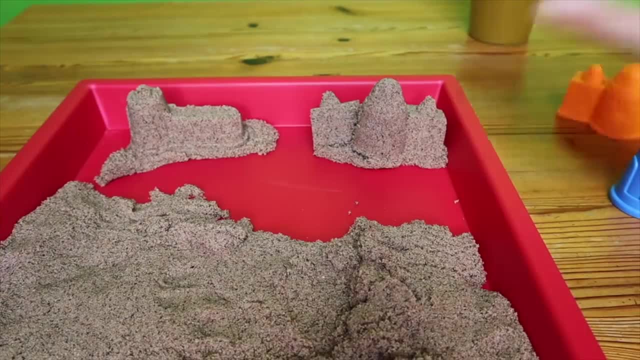 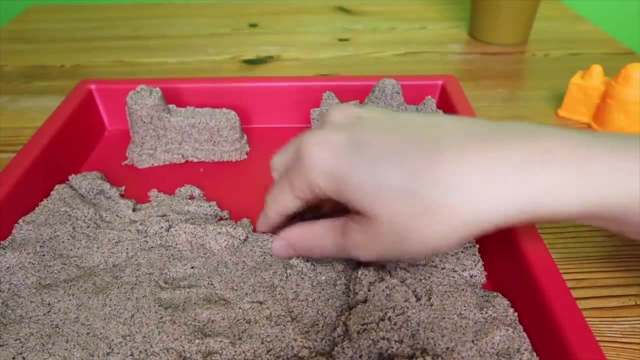 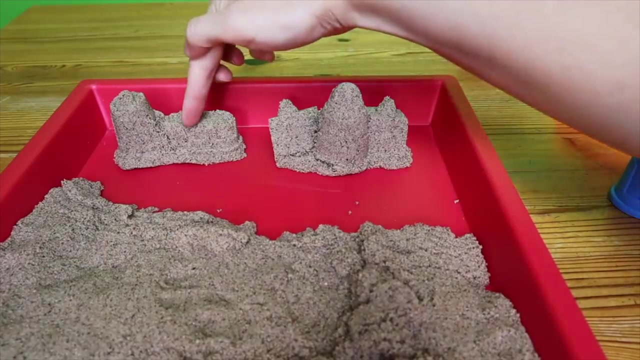 Oh, another castle, So nice, I'm going to trim the edges, Trim, trim the edges. Wow, this is a really cool castle. Now, how many sand castles do we have? One, two, Two sand castles. 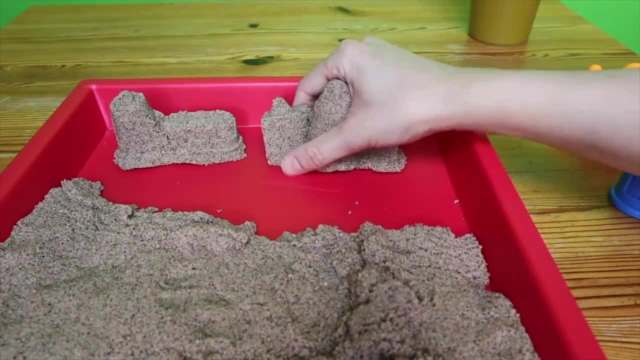 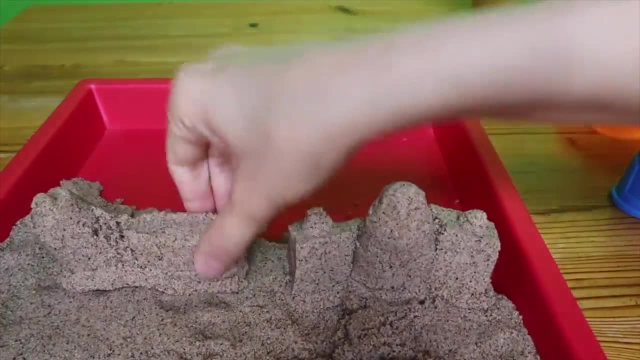 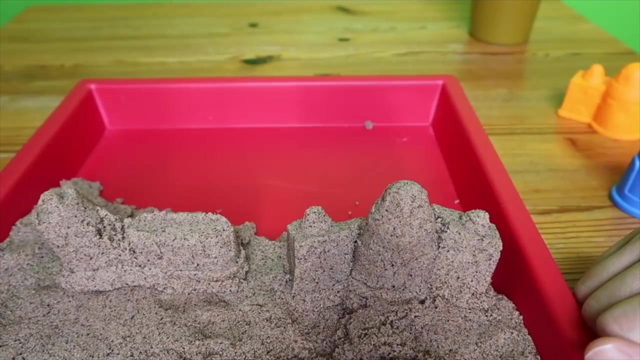 Yeah, Let's put them on the sand. On the sand. Fix it a little bit. Put this one on the sand. Wow, Have you ever made a sand castle? That's awesome. This sand is really cool. You can even make it into a b-b-ball. 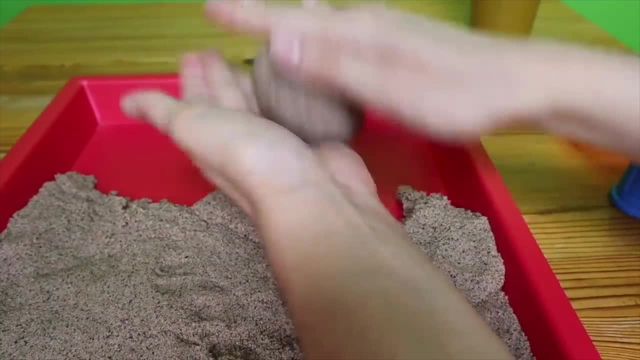 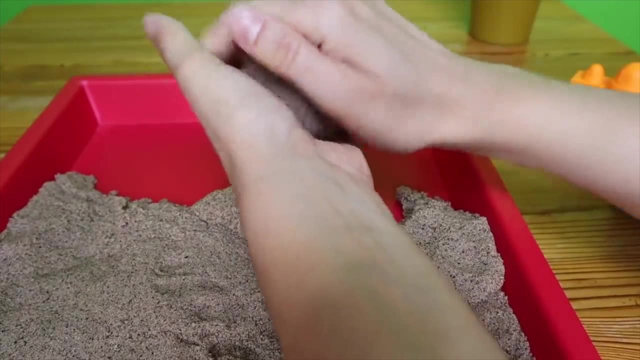 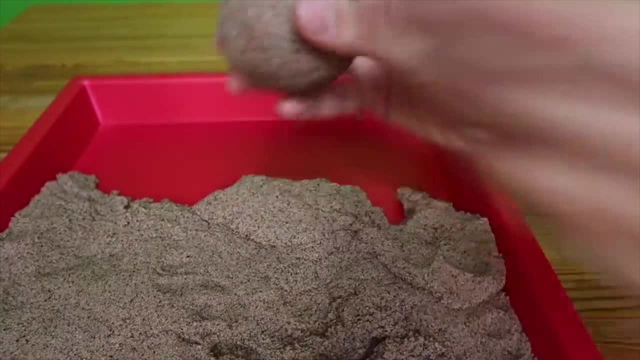 Let me show you: Roll, roll, roll the sand, Roll, roll, roll the sand, Roll, roll, roll the sand. We are rolling sand. Whoa, The sand is now a b-b-ball which starts with the letter B. 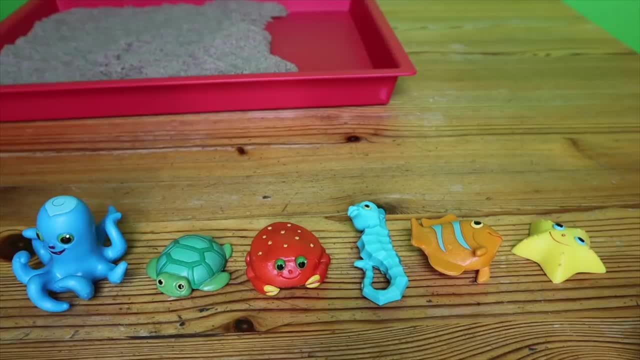 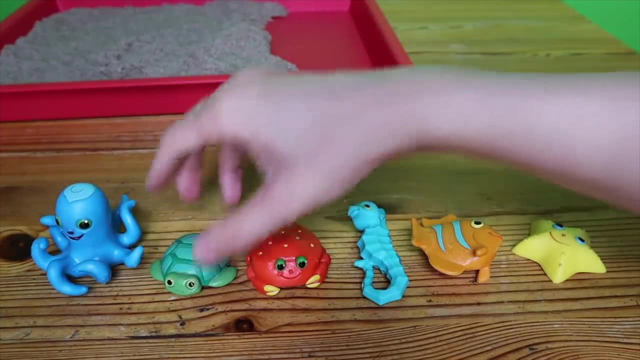 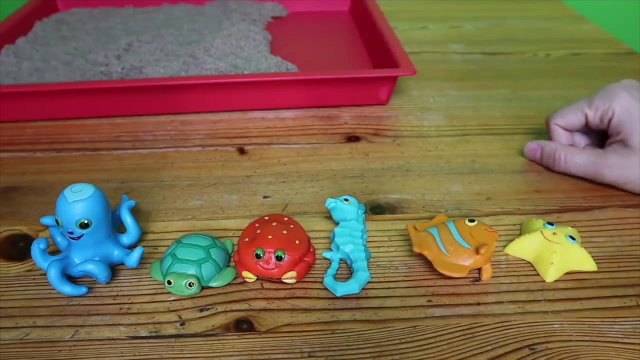 Yeah, That's cool, right. Next, I'd like to show you our little ocean animals. So we have an octopus, a little sea turtle, a crab, a sea horse, a fish and a star. Now look at them very closely, because I'm going to play a game with them. 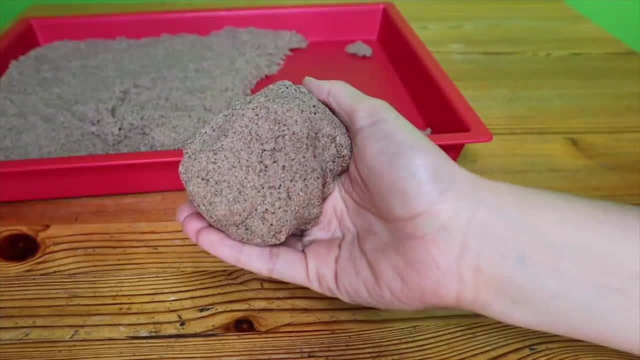 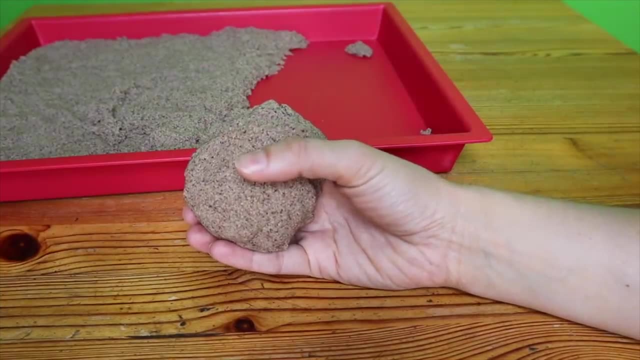 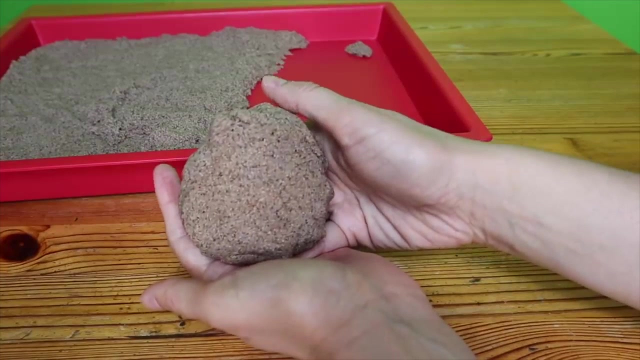 And I'm going to try and trick you. Which animal do you think is hiding in the sand? Peek-a-boo, I showed you a clue. Peek-a-boo, Oh, it was the color red. Hmm, Do you know which one it is? 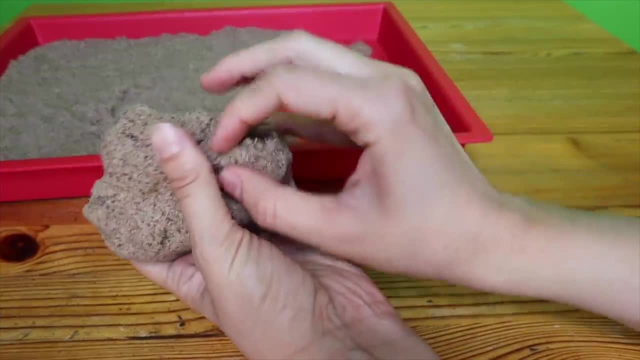 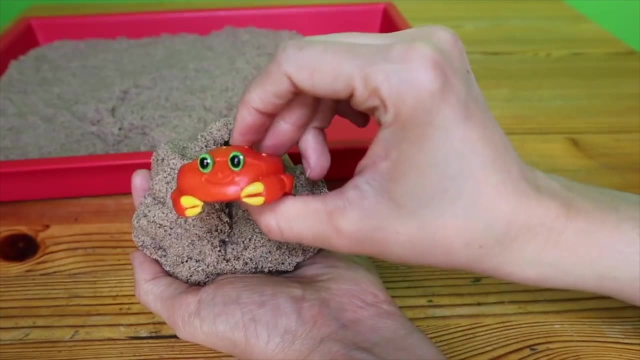 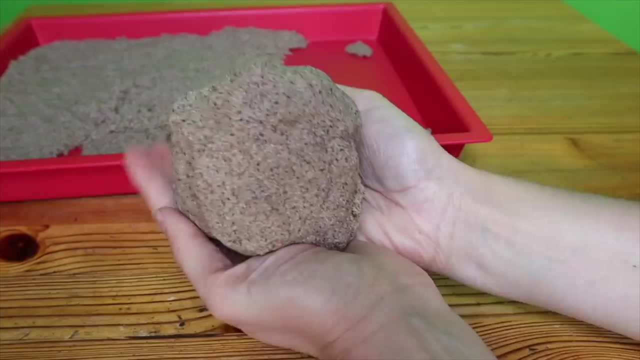 Yeah, It's the. Let's take it out The crab. Good job. I was hiding in the sand. Did I trick you? You didn't trick us. We knew it was you. Who do you think is hiding in this sand ball? 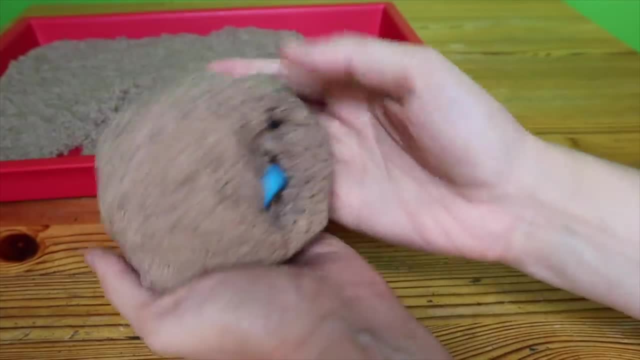 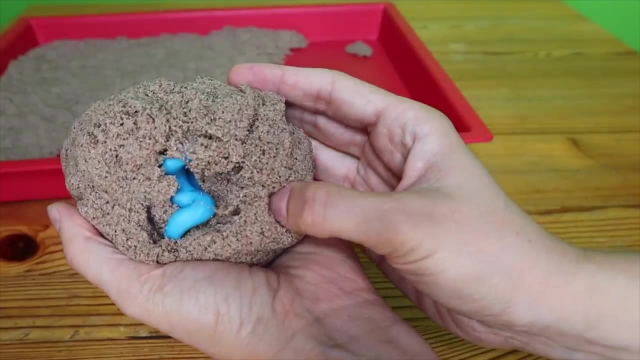 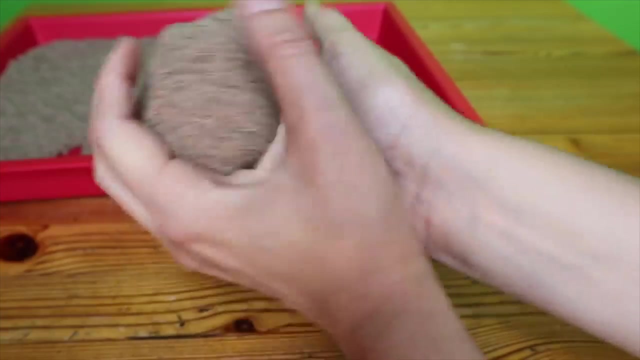 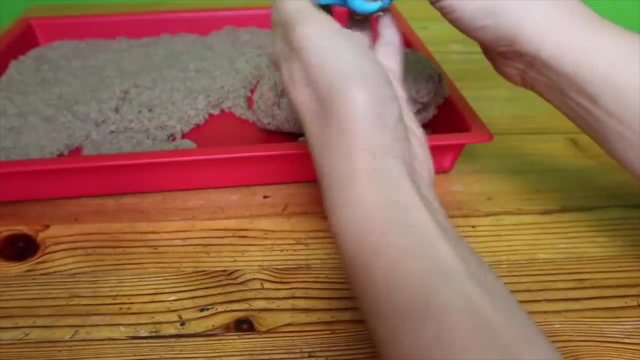 I'll give you a clue. Peek-a-boo, What did that look like? Peek-a-boo, Peek-a-boo, What do you think? it is An octopus. What a silly octopus. There he is, You found me. 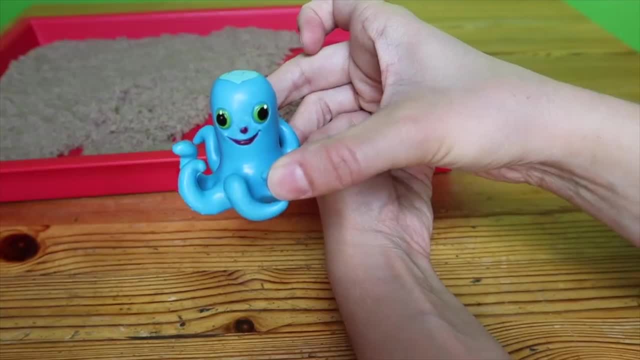 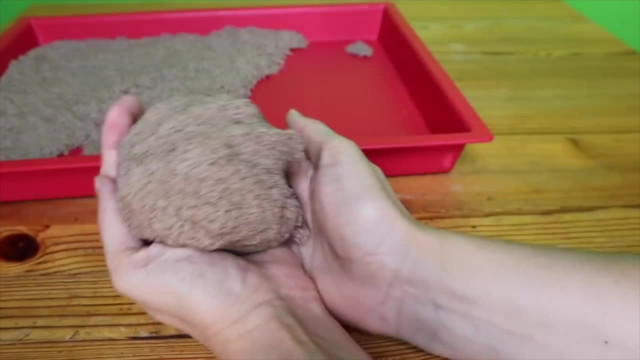 I was hiding in the sand. Did I trick you? No, You didn't trick us. We knew it was you. Good job playing the game. Who do you think is hiding in this sand ball? Peek-a-boo? Who was that? 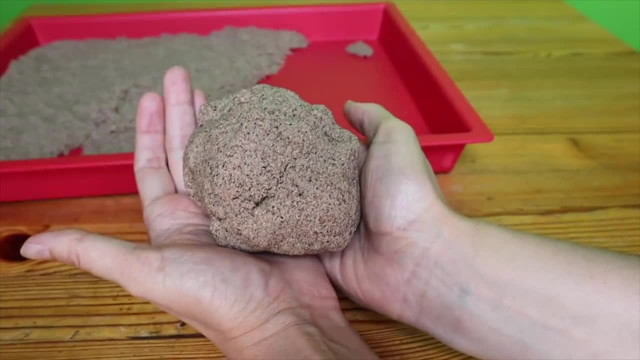 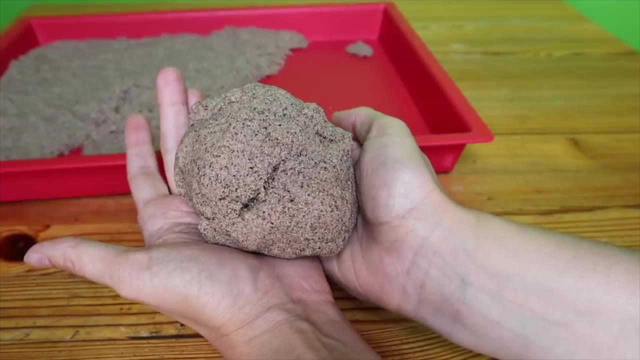 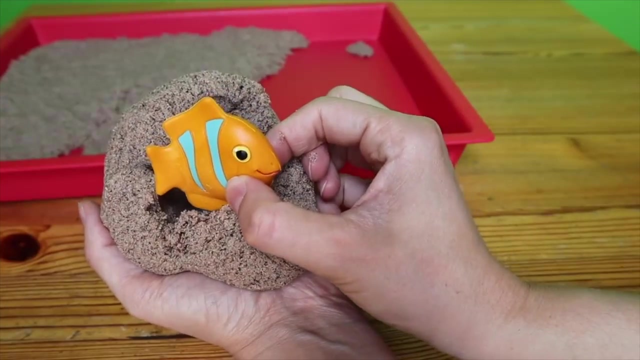 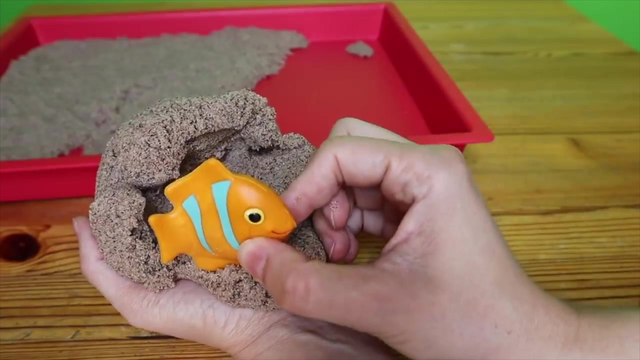 Peek-a-boo. It starts with the letter F. What do you think? It's a fish? It was a fishy. Did I trick you? Swim, swim, swim. You didn't trick us, Mrs Fish. We knew it was you. 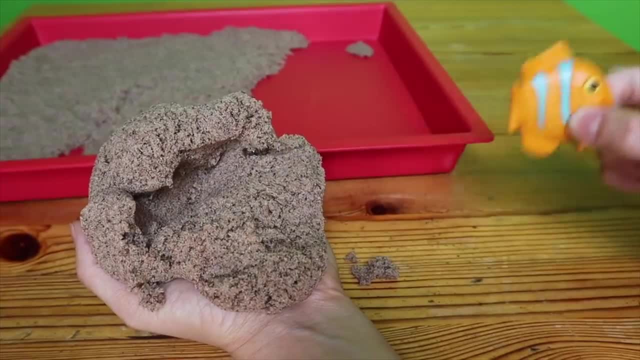 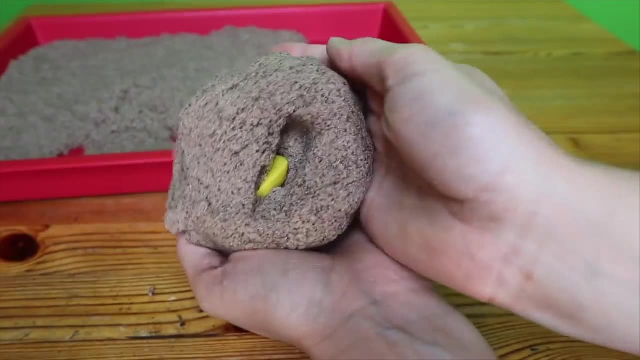 Thanks for playing. Swim, swim, swim, Bye-bye. Hmm, I wonder who's in this sand ball. Who's hiding? Here's your clue: Boop, It's yellow. Do you remember what one of our ocean animals was? yellow? 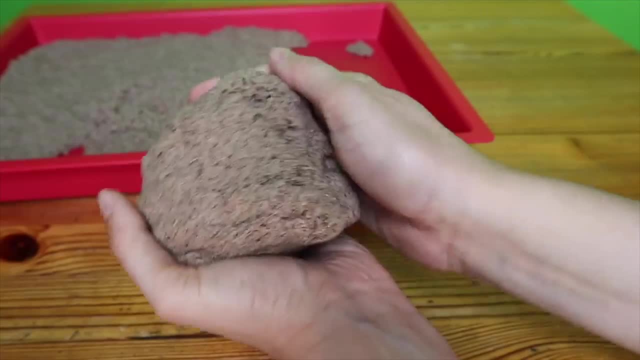 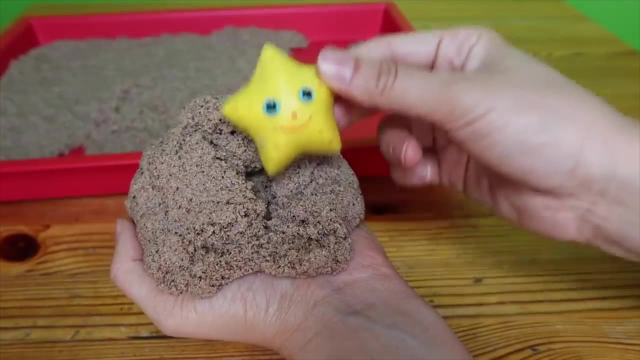 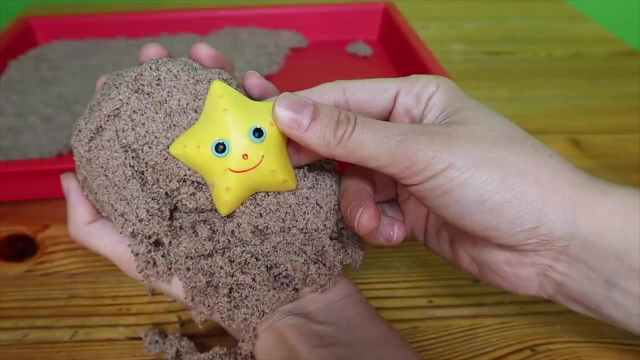 Hmm, It's the s-s-s-starfish. Oh, you found me. I was hiding. Did you know it was me? when you saw the color yellow, We did. You didn't fool us, starfish. Who do you think is hiding in this ball? 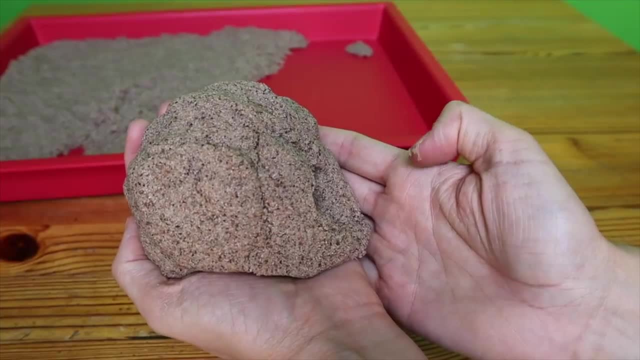 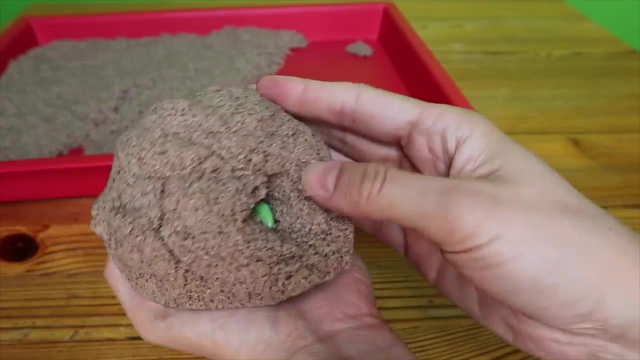 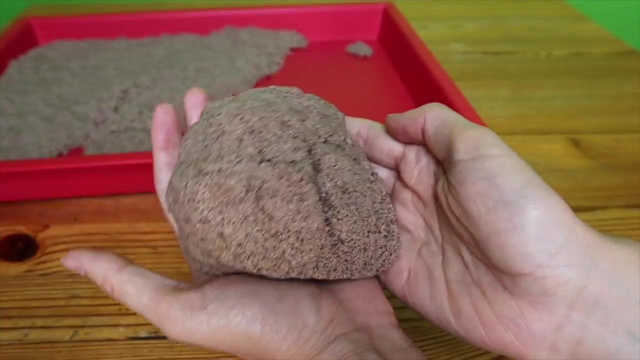 I'll give you a clue. It begins with the letter T, T-t-t, T-t-t. And here's a little clue: We can see him peeking out. Oh, did you see that? Did you see that It's a? 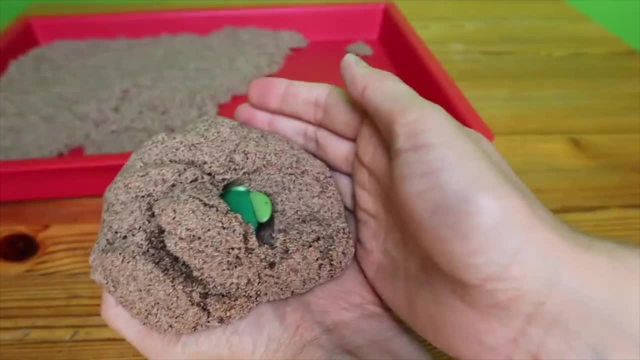 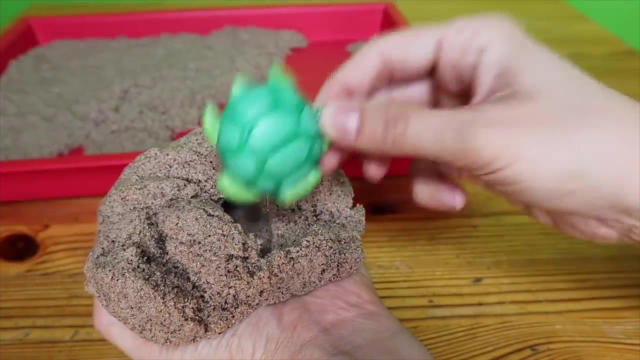 Turtle. Oh no, It's stuck. Say out and we'll get him out Out. Oh, Thank you so much. I was stuck. You're so nice. Did you know it was me a turtle? We did because we saw the green and we knew that it started with a T. 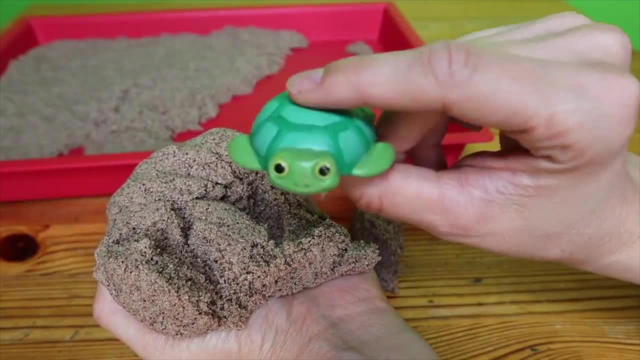 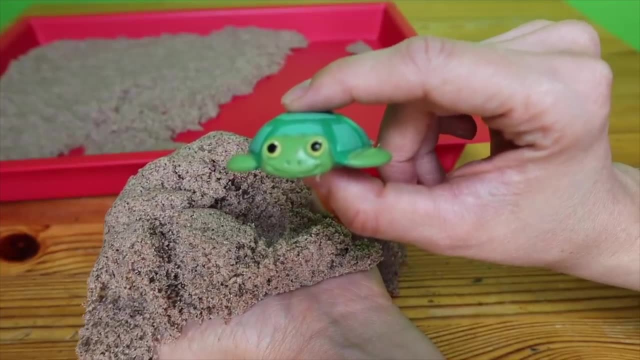 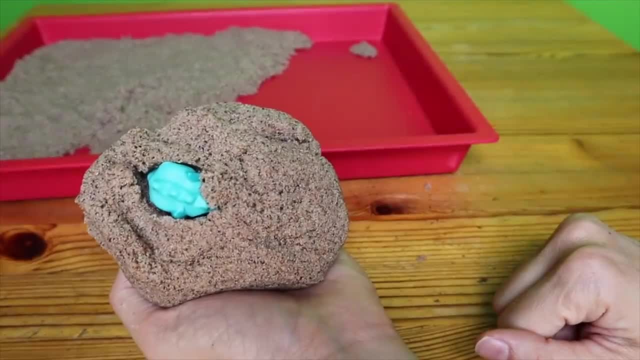 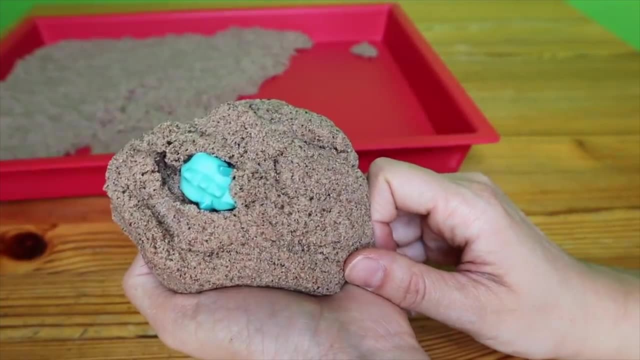 Oh my, She is peeking. Oh my, She is peeking. Oh my, Oh my, Oh my She is peeking out. Hmm, Well, the octopus was blue, but we already found the octopus. 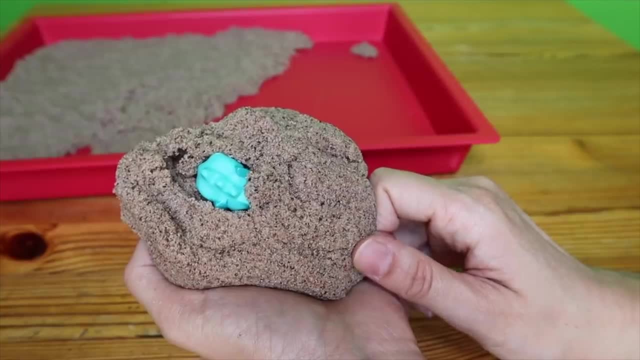 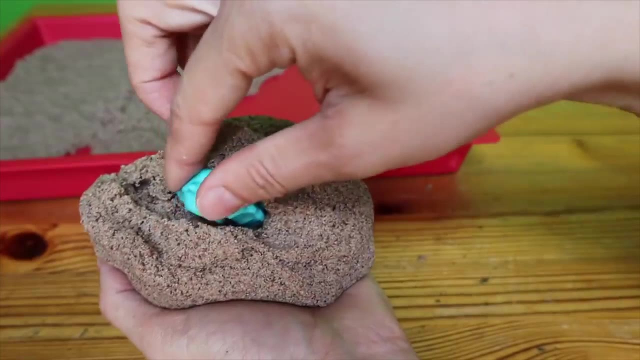 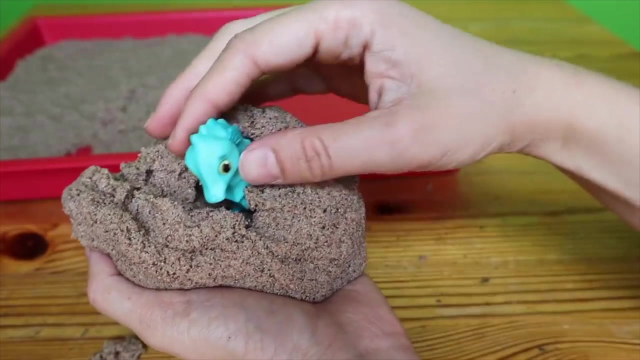 Do you think it's another octopus? What other animals did we have? Hmm, Let's get out a little more and see what we think. Out out out. Do you recognize this little animal? It's a seahorse. 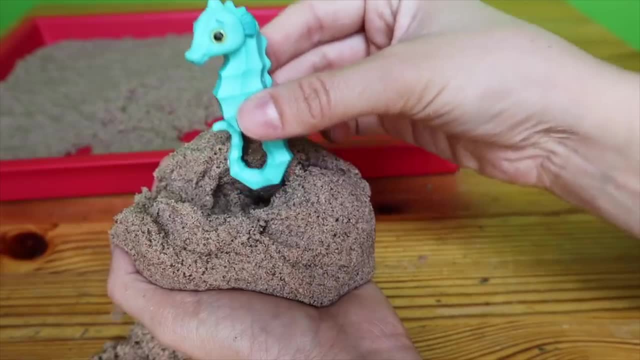 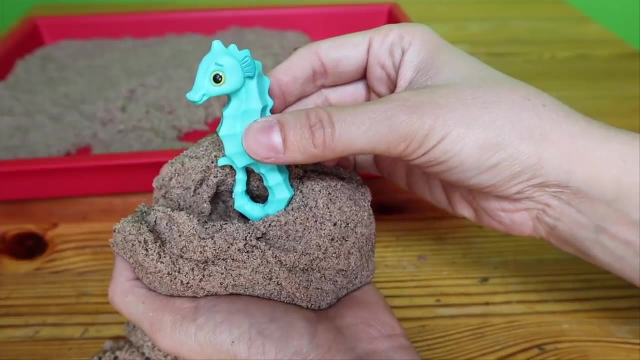 Wow, Hello, I'm a seahorse. Did you know it was me or did you think it was the octopus? We thought it might be an octopus because it was blue like the octopus, but we knew it was you. 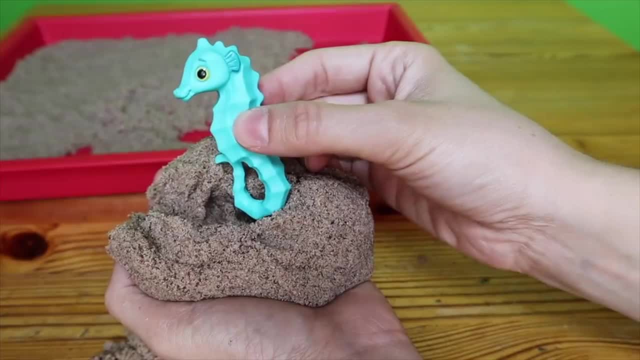 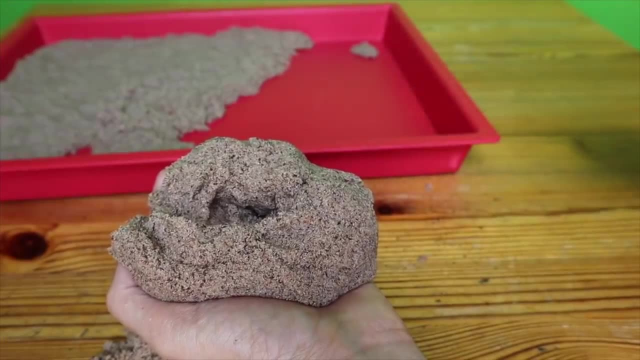 Thank you for finding me. Oh, she gave us a kiss. That's so nice, Swimming away, Swimming, Bye-bye. Can you say bye-bye? Good job. It's fun to play in the sand with the cars Vroom. 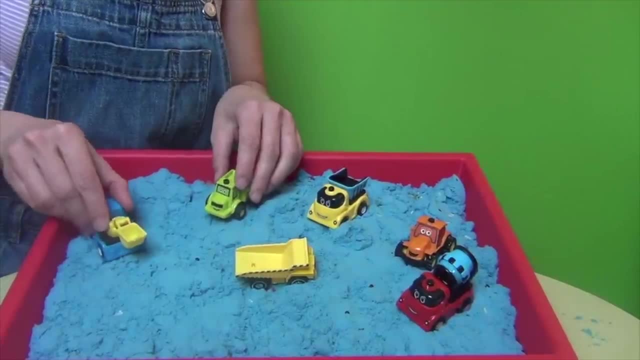 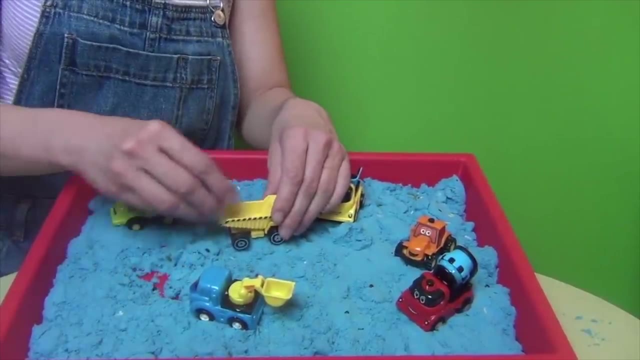 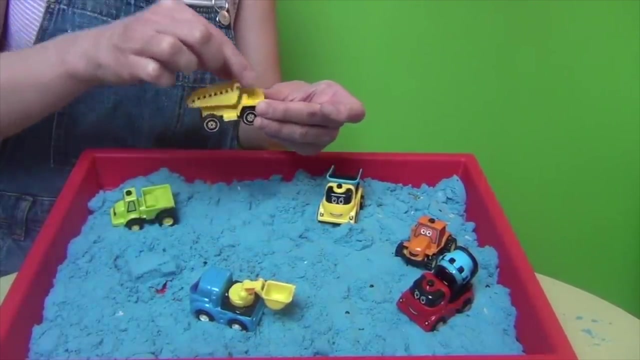 Vroom, Vroom, Vroom, Vroom, Vroom. Beep, Beep, Beep, Beep. Let's fill this car with sand, Put the sand in in and he dumps it out. Wow, that was fun. 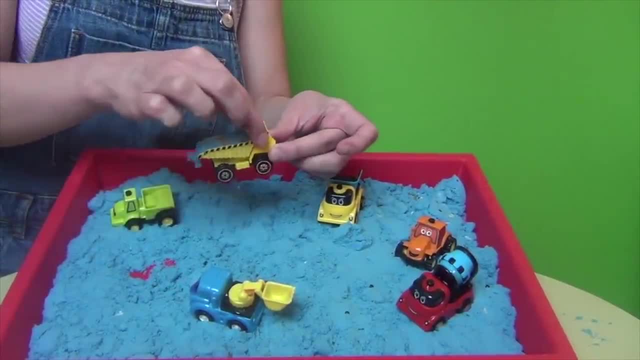 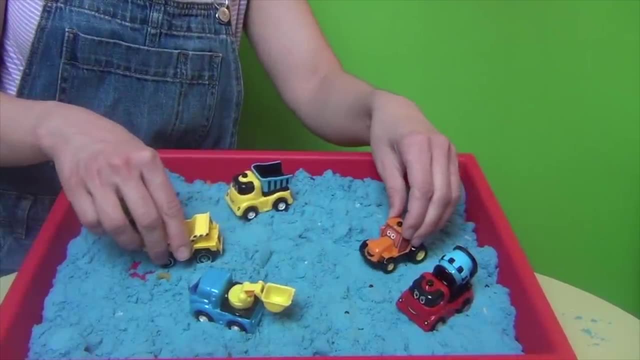 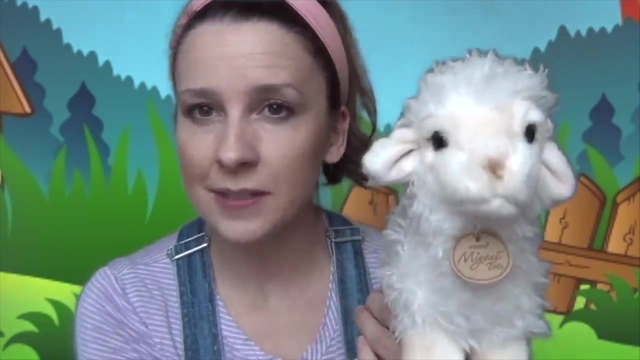 Let's try it again. We put the sand in and then the truck dumps it out. Wow, Vroom, Vroom, Vroom, Beep, Beep, beep. I have a little stuffed animal. do you know what this is? it's a lamb. 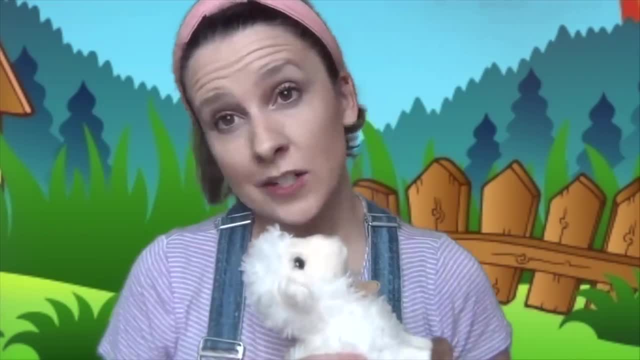 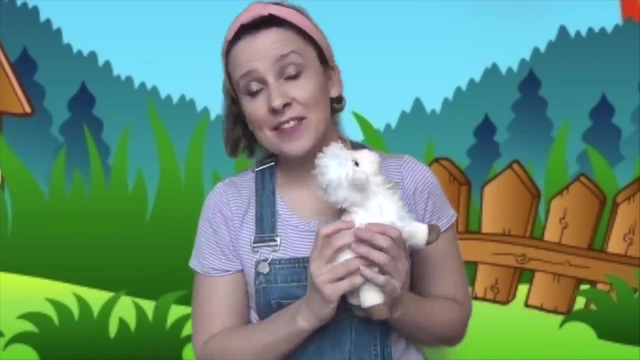 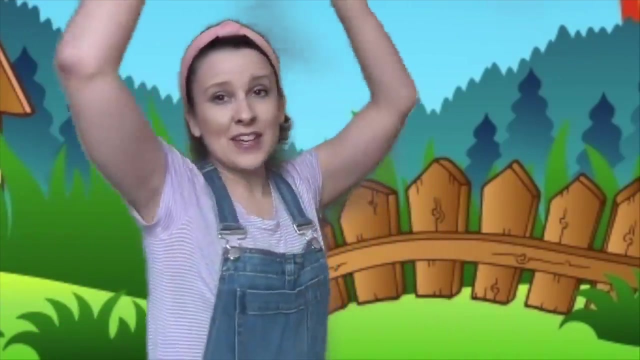 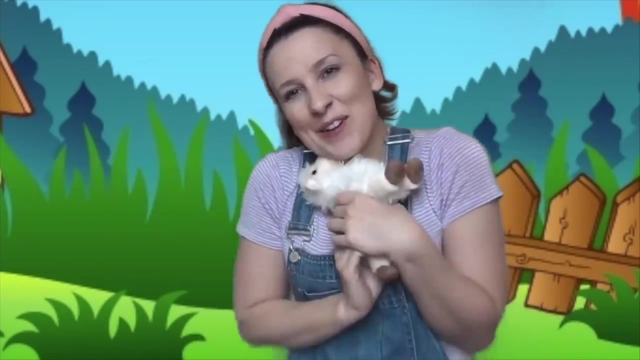 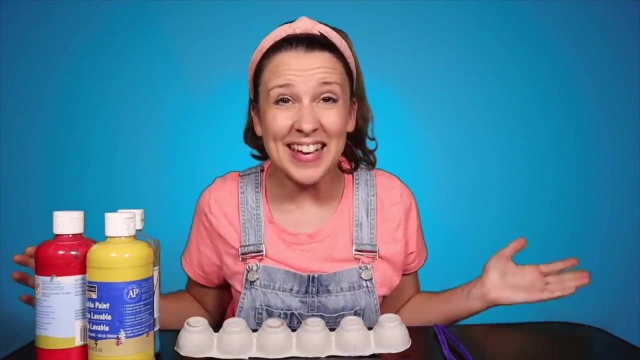 can you get a stuffed animal or an action figure to dance with, and then we'll do a dance together. that was so fun. I'm so excited to make an egg carton caterpillar with you. I can't wait. let's get started. okay, first I'm going to 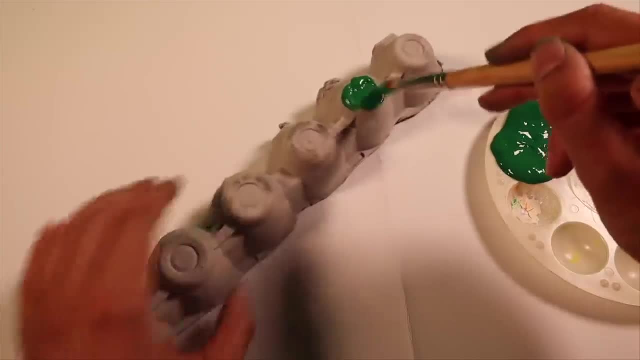 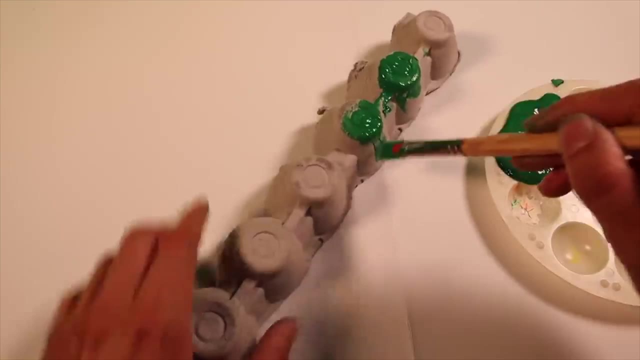 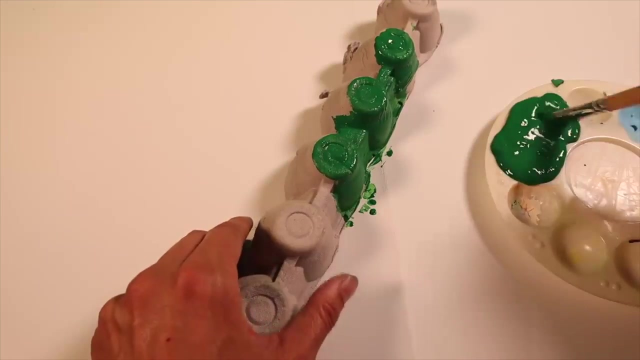 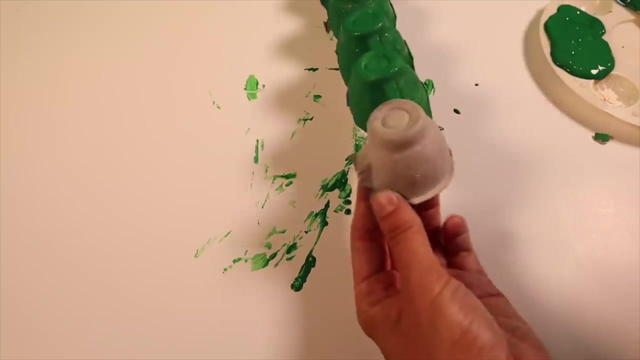 do a little egg carton caterpillar. dip my paintbrush in the green paint and paint the egg carton green, green, caterpillar. what color are you going to paint yours? you could do any color you want. do you like painting me too? I love it. now I'm going to paint the head red. wow, this is so. 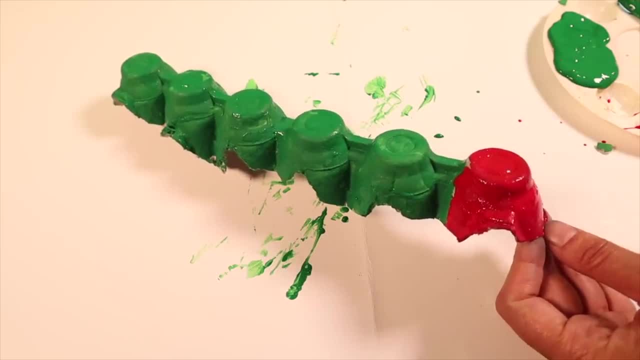 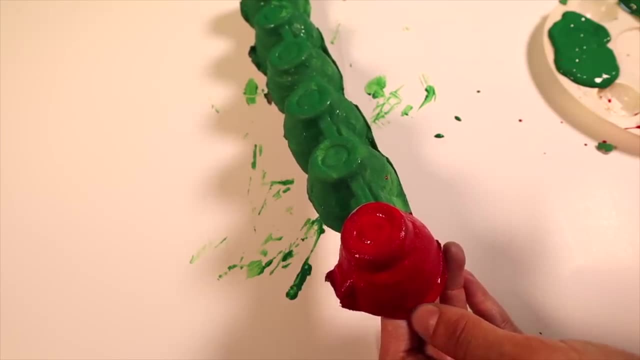 fun. I'm going to paint the head green. fun. wow, that looks really cool. thanks for helping me. now I'm going to let it dry for a little while and then we'll paint the face and put in the antennas. do you remember how we learned about ovals? 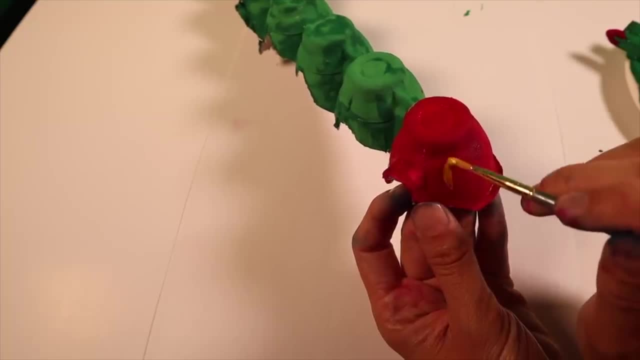 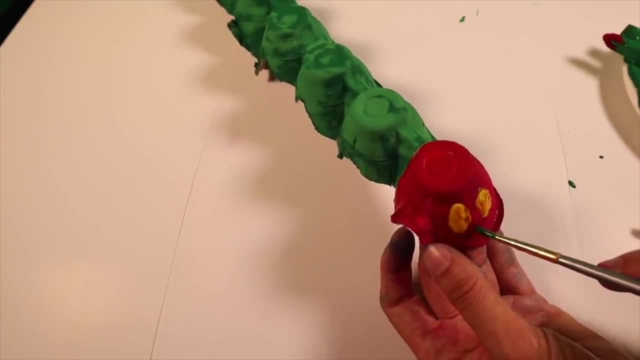 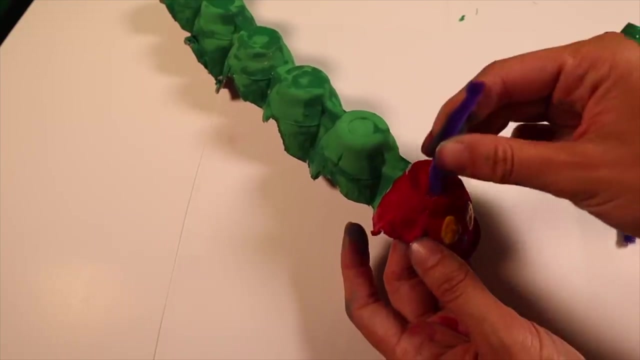 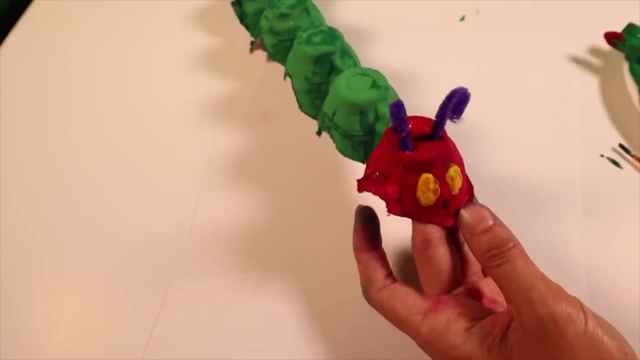 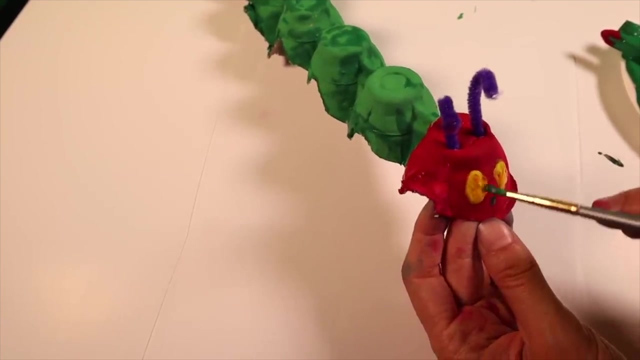 I'm going to make some ovals for the eyes. next I think I'll make a little nose. oh so cute. there's a little tiny nose. next I'll put in the antennas. it looks so cute. it's starting to look like a caterpillar. now let's try the inside of the eyes. 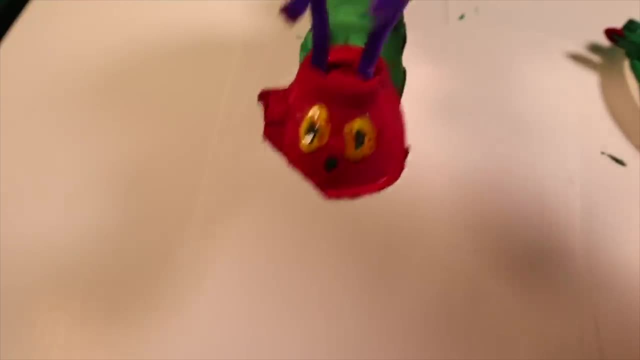 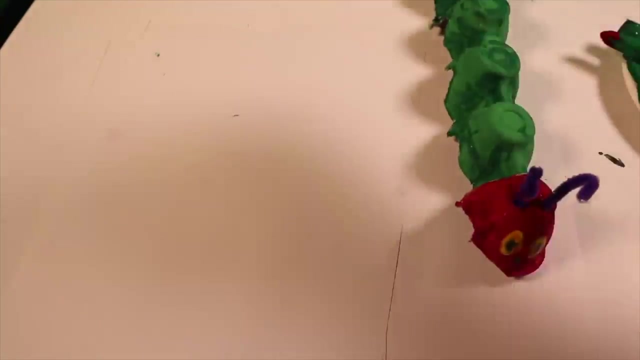 and he's all done. hello, thank you for making me miss Rachel. I'm gonna go eat. I'm so hungry. you could draw him something like this. you could draw him something like this. you could draw him something like this. hmm, what's the thing in the book he ate? I think he ate an apple. 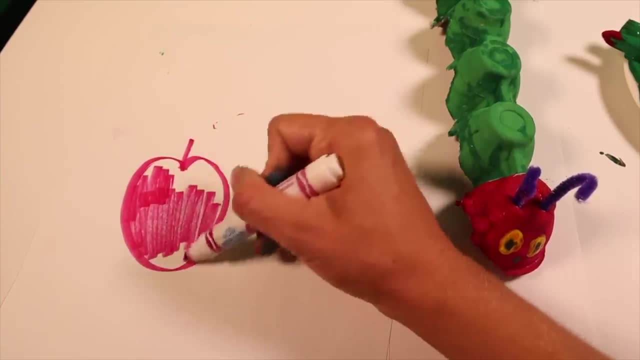 hmm, what's the thing in the book he ate? I think he ate an apple. hmm, what's the thing in the book he ate? I think he ate an apple. so you could draw an apple, so you could draw an apple, so you could draw an apple and then, if your grown-up has a, 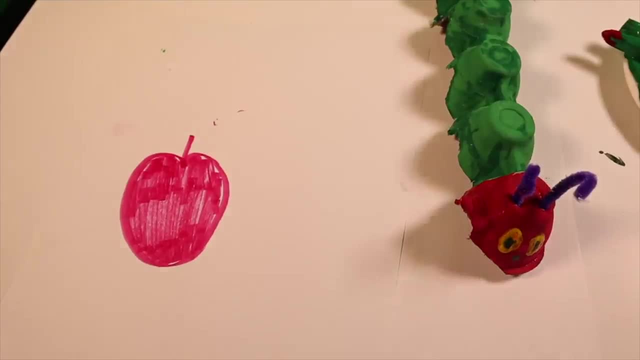 and then if your grown-up has a, and then if your grown-up has a hole puncher, you could punch a hole in the hole puncher. you could punch a hole in the hole puncher. you could punch a hole in the apple. apple, apple, you made me an apple. thank you so much. 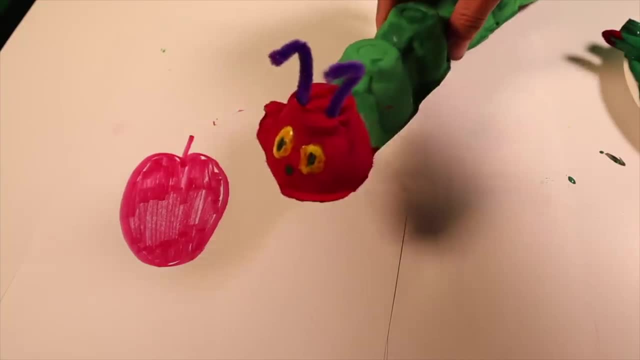 you made me an apple. thank you so much. you made me an apple. thank you so much. you could cut that out too with a. you could cut that out too with a. you could cut that out too with a grown-up's help. can you make me more food? okay, what else? 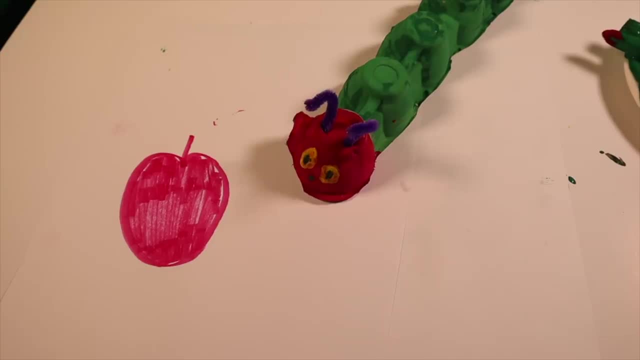 can you make me more food? okay. what else can you make me more food? okay, what else could I make him? I think I'll do a. could I make him? I think I'll do a. could I make him? I think I'll do a banana, banana, banana. 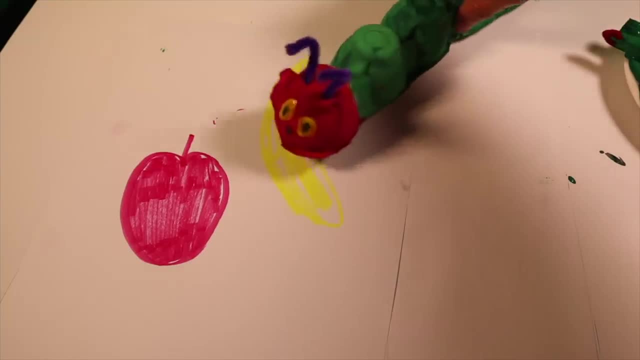 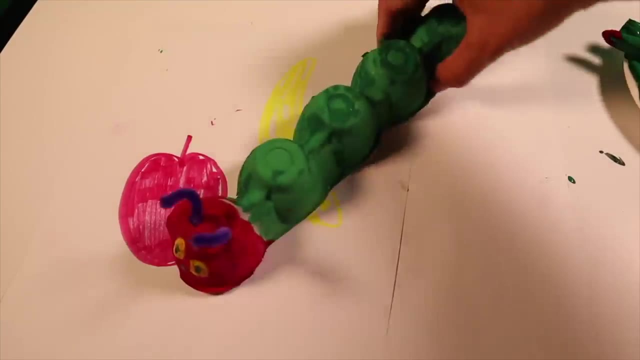 oh, thank you, I love fruit. it's so yummy. oh, thank you, I love fruit. it's so yummy. oh, thank you, I love fruit. it's so yummy. wow, that was such a fun craft. thanks for wow, that was such a fun craft. thanks for wow, that was such a fun craft. thanks for help. do you have a teddy bear? Wow, if you. help. do you have a teddy bear? Wow, if you help. do you have a teddy bear? Wow, if you want, you can get out your teddy bear. want you can get out your teddy bear. want you can get out your teddy bear for, for. 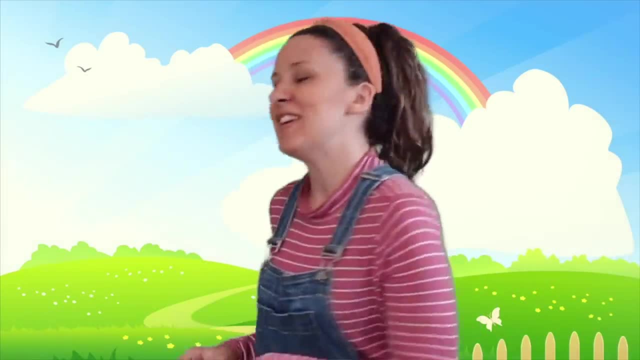 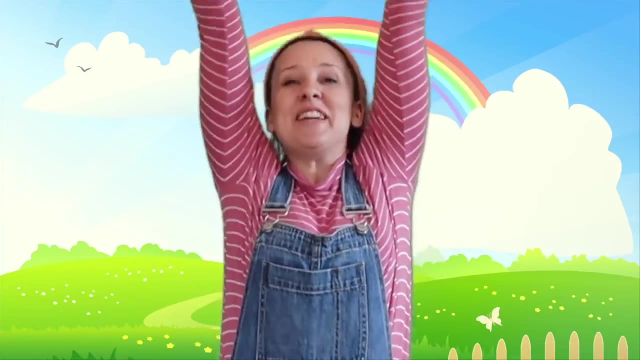 for this rhyme. teddy bear, teddy bear, turn this rhyme. teddy bear, teddy bear, turn this rhyme. teddy bear, teddy bear, turn around. teddy bear, teddy bear touch the around. teddy bear, teddy bear, touch the around. teddy bear, teddy bear touch the ground. teddy bear, teddy bear, reach up. 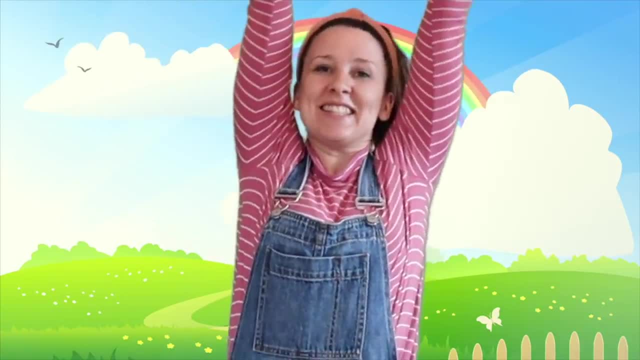 ground. teddy bear. teddy bear. reach up ground. teddy bear. teddy bear. reach up behind teddy bear. teddy bear. touch the behind. teddy bear. teddy bear. touch the behind. teddy bear. teddy bear. touch the sky. teddy bear. teddy bear. bed down low. 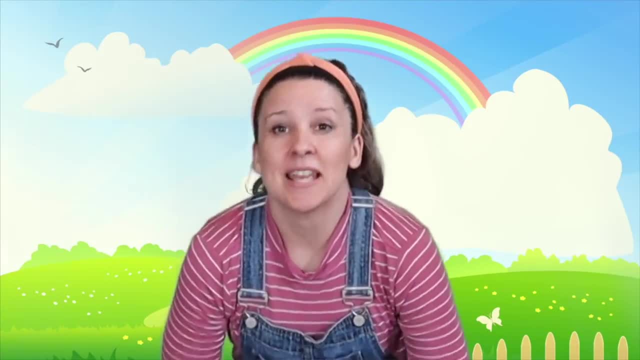 sky teddy bear. teddy bear bed down low sky teddy bear. teddy bear bed down low. teddy bear. teddy bear. touch your toes. teddy bear. teddy bear. touch your toes, teddy bear. teddy bear. touch your toes, teddy bear. teddy bear. go to bed, Oh teddy. 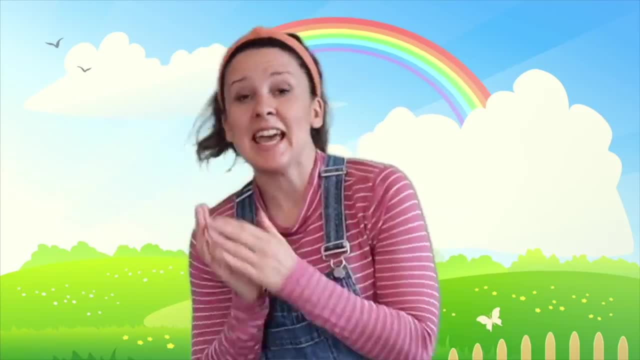 teddy bear, teddy bear, go to bed. Oh, teddy, teddy bear, teddy bear go to bed. Oh, teddy bear, teddy bear. rest your head, bear, teddy bear. rest your head, bear, teddy bear. rest your head, bear, teddy bear, teddy bear, rest your head, teddy bear, teddy bear. turn off the light. 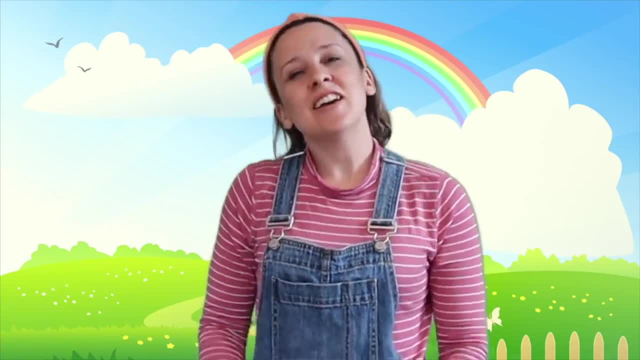 teddy bear- teddy bear. turn off the light. teddy bear- teddy bear- turn off the light. click teddy bear. teddy bear say good night. click teddy bear. teddy bear say good night. click teddy bear. teddy bear say good night. oh, the teddy bear is so tired pretend to. 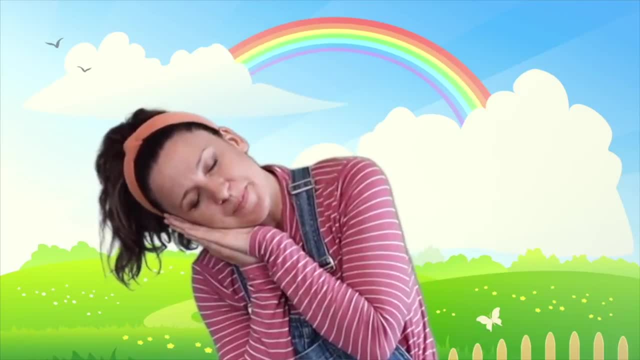 oh, the teddy bear is so tired, pretend to. oh, the teddy bear is so tired. pretend to go to sleep, or put your teddy bear to go to sleep, or put your teddy bear to go to sleep. or put your teddy bear to bed. ding, ding, ding, ding, ding. that's our. 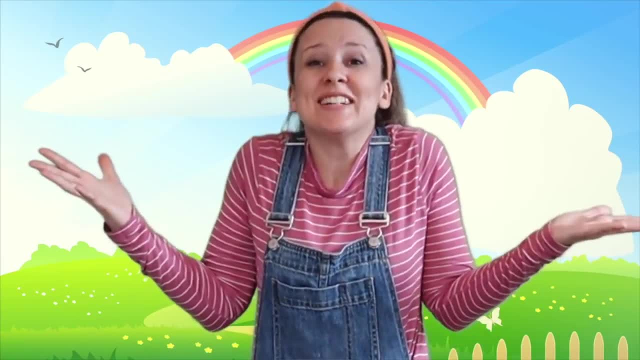 bed. ding, ding, ding, ding ding. that's our bed. ding, ding, ding, ding, ding ding. that's our alarm clock. we have to get up and alarm clock. we have to get up and alarm clock. we have to get up and sing more songs. teddy bear, teddy bear find. 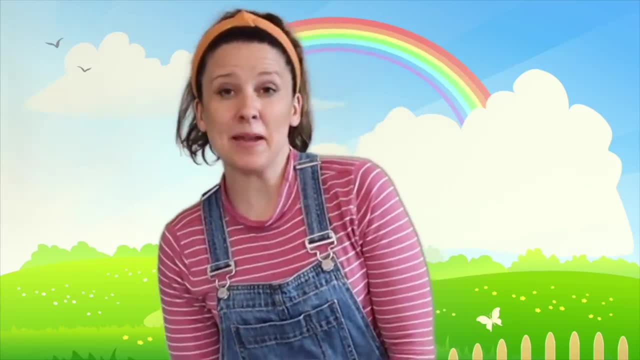 sing more songs. teddy bear, teddy bear, find. sing more songs. teddy bear. teddy bear, find your nose boink, teddy bear. teddy bear, your nose boink, teddy bear. teddy bear, your nose boink, teddy bear. teddy bear, touch your toes. oh, touch your toes, teddy. 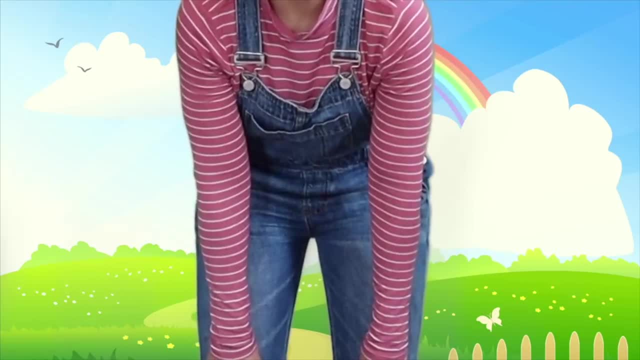 touch your toes. oh, touch your toes, teddy. touch your toes. oh, touch your toes, teddy bear. teddy bear. touch your knees. are bear, teddy bear. teddy bear. touch your knees. are bear, teddy bear. teddy bear. touch your knees. are you touching your knees, teddy bear? 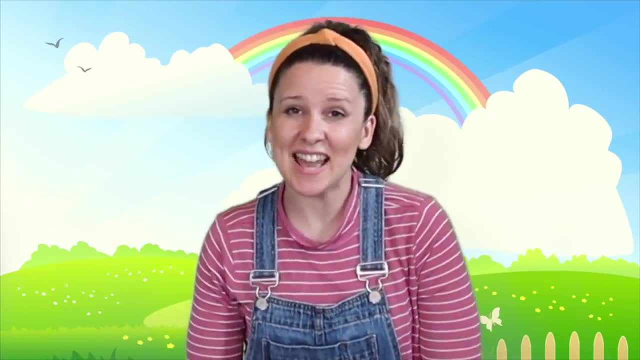 you touching your knees, teddy bear. you touching your knees, teddy bear. teddy bear sit down. please are you sitting? teddy bear, sit down. please are you sitting. teddy bear, sit down. please are you sitting down. good job down, good job down, good job. our friend Georgie's doing an art project. 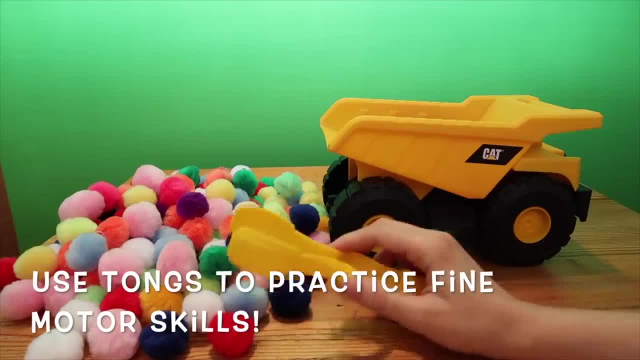 our friend Georgie's doing an art project. our friend Georgie's doing an art project with red puff balls. let's fill up the with red puff balls. let's fill up the with red puff balls. let's fill up the truck and bring the puff balls to Georgie. 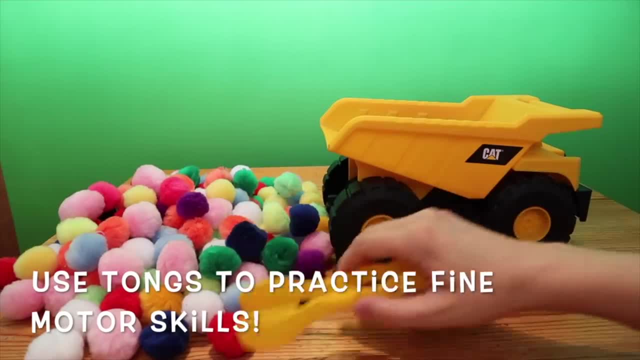 truck and bring the puff balls to Georgie. truck and bring the puff balls to Georgie. he needs red puff balls cuz he's he needs red puff balls cuz he's he needs red puff balls cuz he's making an Apple project. should this one making an Apple project? should this one? 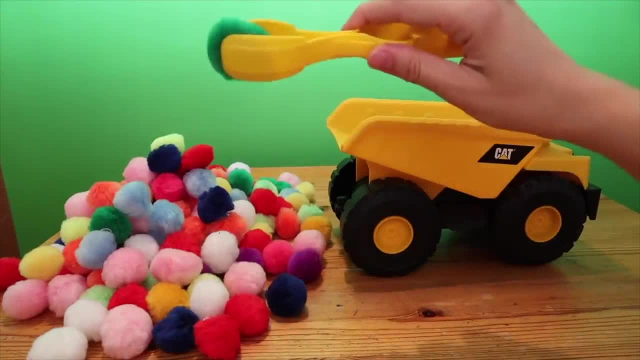 making an Apple project. should this one go in? yeah, it's red. does this go in? no, go in. yeah, it's red. does this go in? no, go in. yeah, it's red. does this go in? no, we want the red puff balls. does this go? we want the red puff balls. does this go? 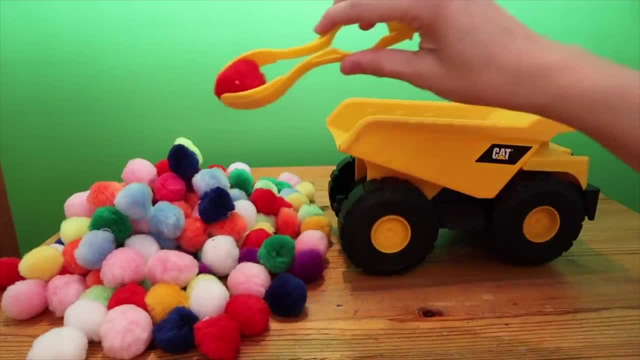 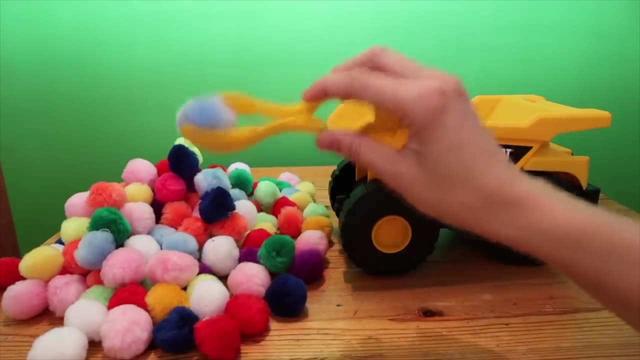 we want the red puff balls. does this go in? yeah, this is red. this is red. does in? yeah, this is red. this is red. does in. yeah, this is red. this is red. does this go in? no, it's blue. does this go this go in? no, it's blue. does this go? 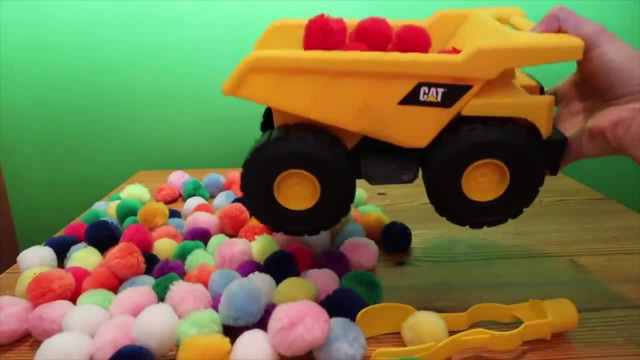 this go in? no, it's blue. does this go in? no, it's green. we filled up the truck in. no, it's green. we filled up the truck in. no, it's green. we filled up the truck with red puff balls. yay, awesome job now with red puff balls. yay, awesome job now. 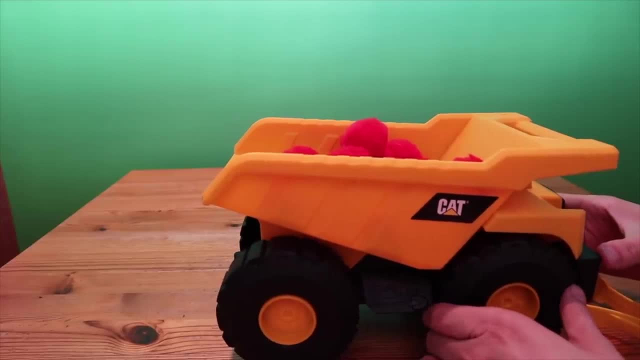 with red puff balls. yay, awesome job. now we can bring them to Georgie. can you? we can bring them to Georgie. can you? we can bring them to Georgie. can you help me dump out the puff balls? huh say, help me dump out the puff balls, huh say. 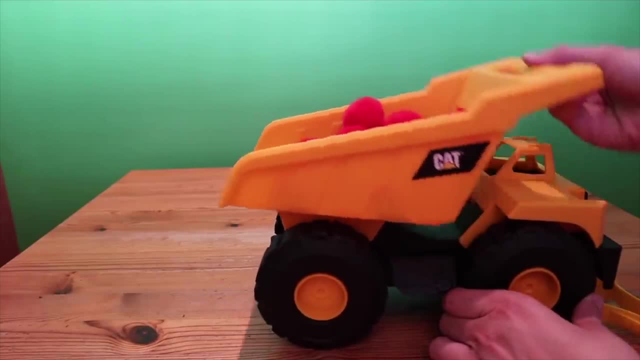 help me dump out the puff balls. huh say, out, and I'll dump them out. one, two out, and I'll dump them out. one, two out, and I'll dump them out. one, two, three out- yay, oh, we dumped him out great. three out, yay, oh, we dumped him out great. 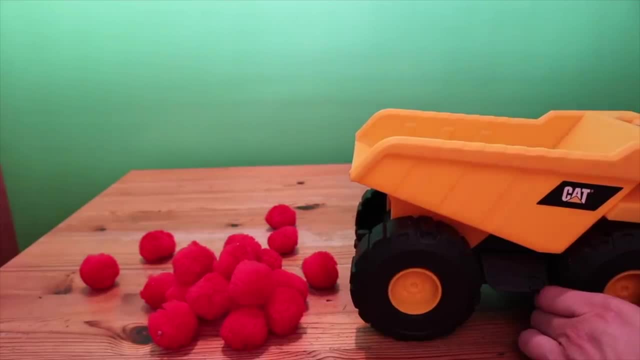 three out. yay, oh, we dumped him out. great job. so many puff balls for Georgie's job. so many puff balls for Georgie's job. so many puff balls for Georgie's Apple project. this song is called the Apple project. this song is called the Apple project. this song is called the hokey pokey. I bet you already know it are. 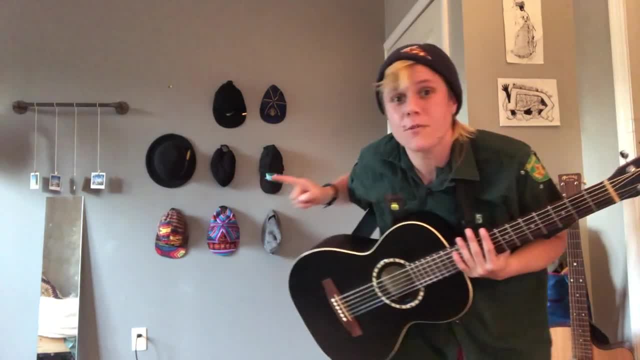 hokey pokey. I bet you already know it are hokey pokey. I bet you already know it are y'all ready? okay, let's go, you can y'all ready. okay, let's go, you can y'all ready. okay, let's go. you can follow along with me right here. 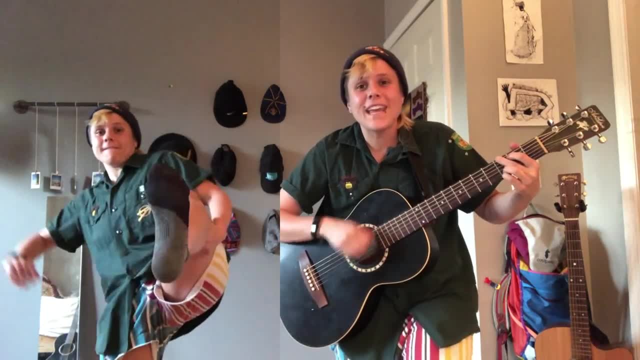 follow along with me right here. follow along with me right here. you put your left foot in. you put your. you put your left foot in. you put your. you put your left foot in. you put your left foot out. you put your left foot in. left foot out. you put your left foot in. 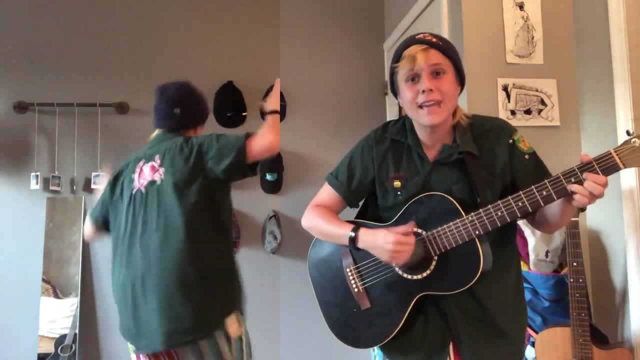 left foot out, you put your left foot in and you shake it all about. you do the and you shake it all about. you do the and you shake it all about. you do the. hokey pokey and you turn yourself around. hokey pokey and you turn yourself around. 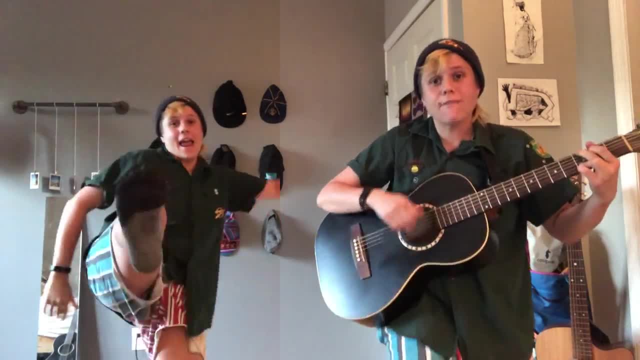 hokey pokey and you turn yourself around. that's what it's all about. that's what it's all about. that's what it's all about. you put your right foot in. you put your. you put your right foot in. you put your. you put your right foot in. you put your right foot out. you put your right foot. 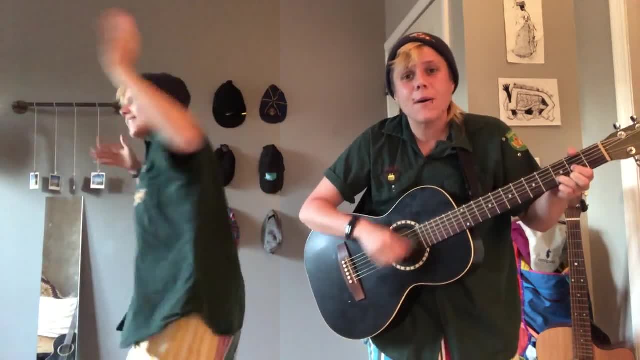 right foot out, you put your right foot in and you shake it all about right foot in, and you shake it all about right foot in and you shake it all about. you do the hokey pokey and you turn. you do the hokey pokey and you turn. 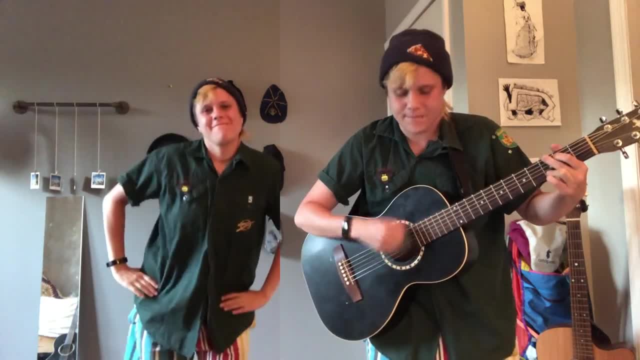 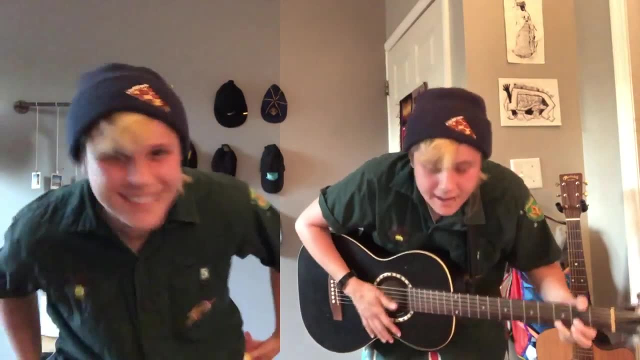 you do the hokey pokey and you turn yourself around yourself, around yourself around. that's what it's all about. that's what it's all about. You put your head in, you put your head out, You put your head in and you shake it all about. 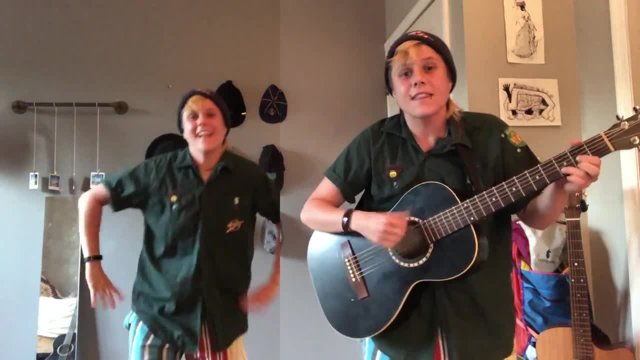 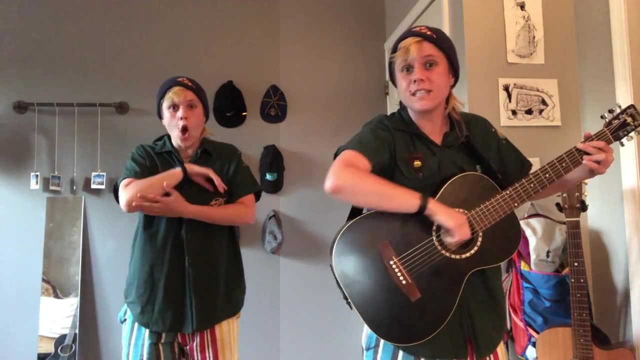 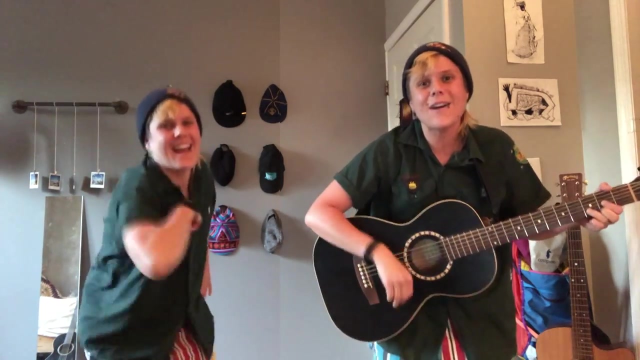 You do the Hokey Pokey and you turn yourself around. That's what it's all about. What else should we put in this circle? How about our elbows? Yeah, You put your right elbow in, you put your right elbow out, You put your right elbow in and you shake it all about. 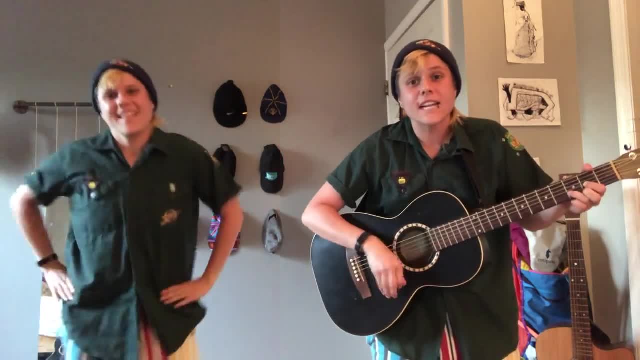 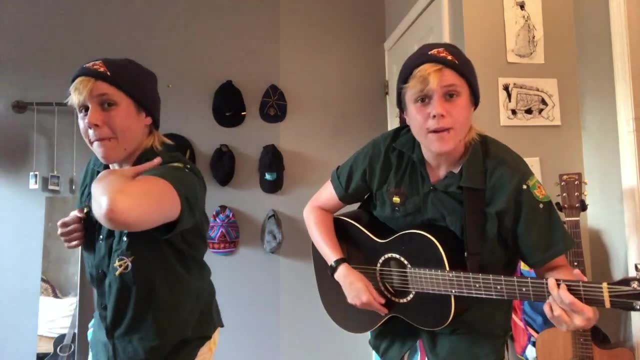 You do the Hokey Pokey and you turn yourself around. That's what it's all about. Let's do the left elbow Ready. You put your left elbow in, you put your left elbow out, You put your left elbow in and you shake it all about. 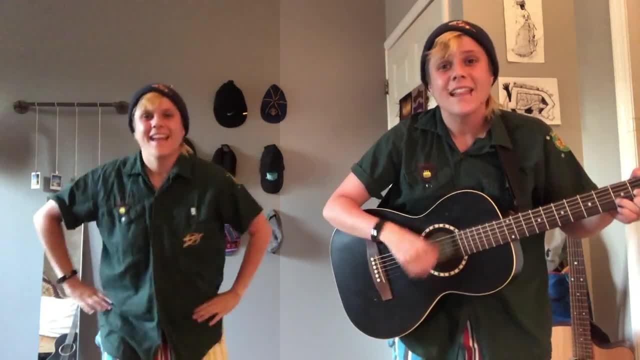 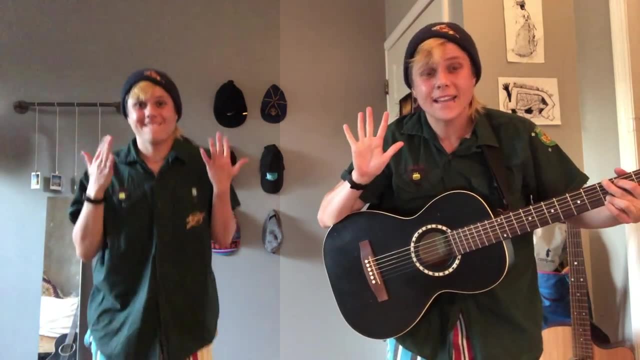 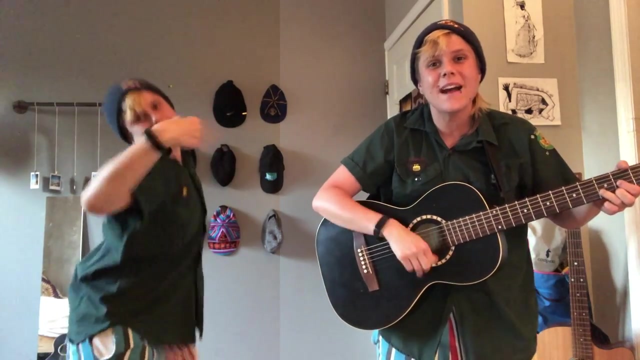 You do the Hokey Pokey and you turn yourself around. That's what it's all about. Alright, let's do our hands Ready. We put our right hand in, we put our right hand out, We put our right hand in and we shake it all about. 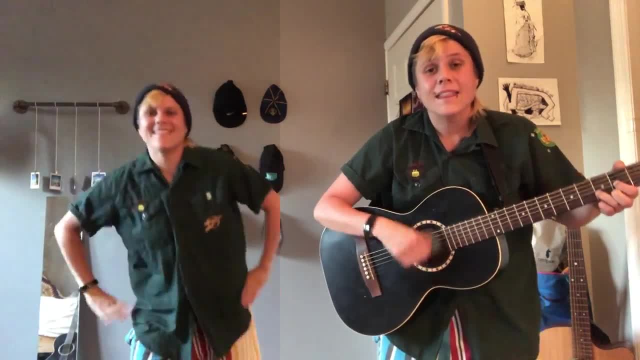 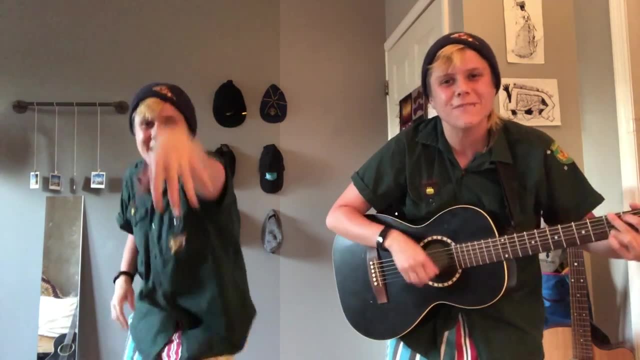 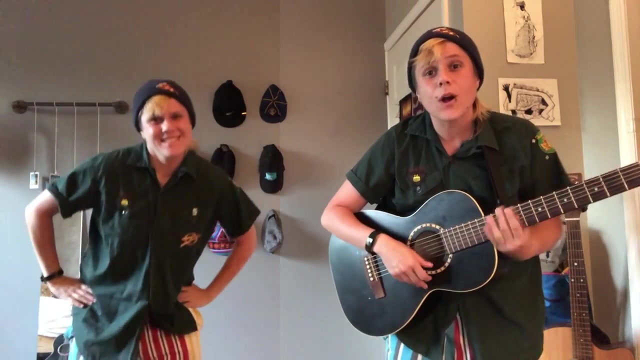 You do the Hokey Pokey and you turn yourself around. That's what it's all about. You put your left hand in, you put your left hand out, You put your left hand in and you shake it all about. You do the Hokey Pokey and you turn yourself around. That's what it's all about. 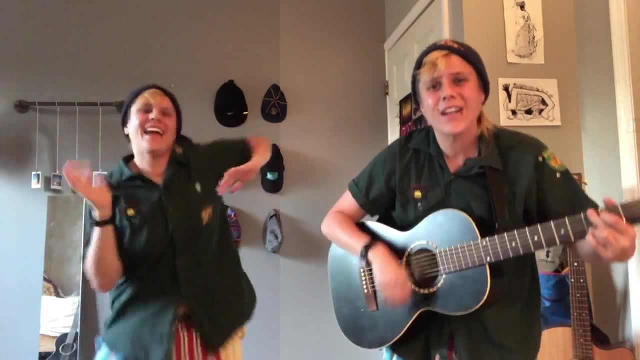 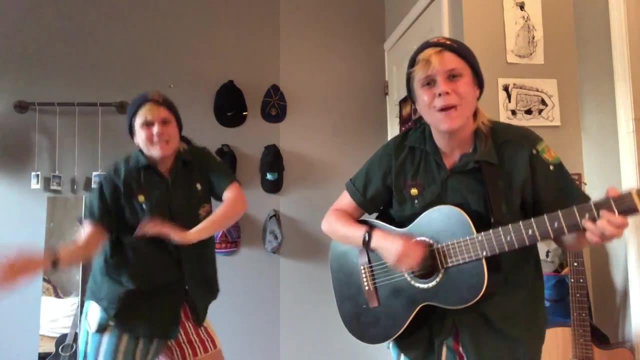 Free dance. You do the Hokey Pokey. Woo, You do the Hokey Pokey and you turn yourself around. That's what it's all about: Free dance, You do the Hokey Pokey and you do the Hokey Pokey. 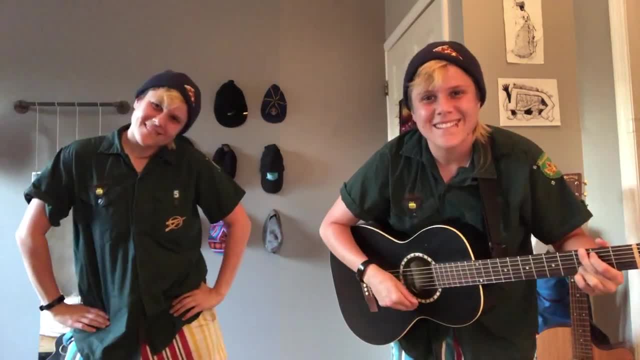 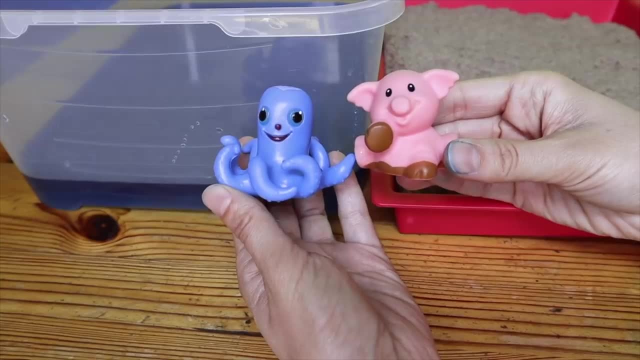 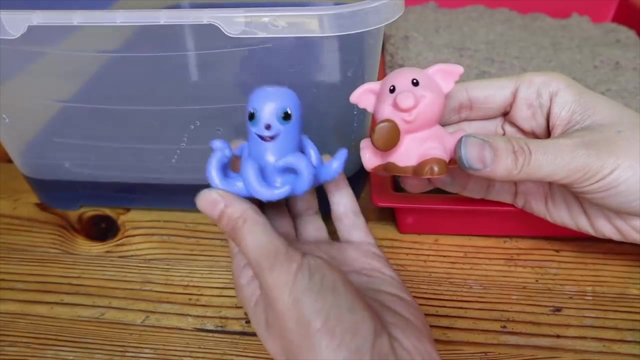 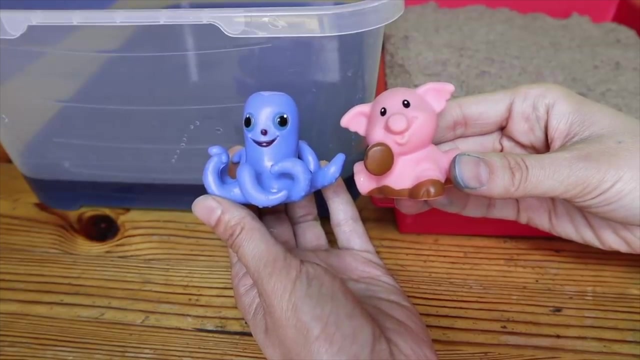 That's what it's all about. Yay, Can you help these animals get back to their homes? Thank you. Who belongs in the ocean, The octopus or the pig? Yeah, the octopus. Let's let the pig go back to the farm. 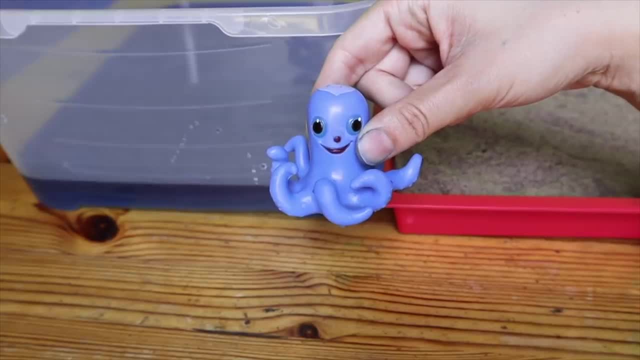 Thank you for finding my home. I swim in the ocean. Okay, you say in and I'll put the octopus in. Put it in, put it in. put it. You said in and the octopus went back in the ocean. 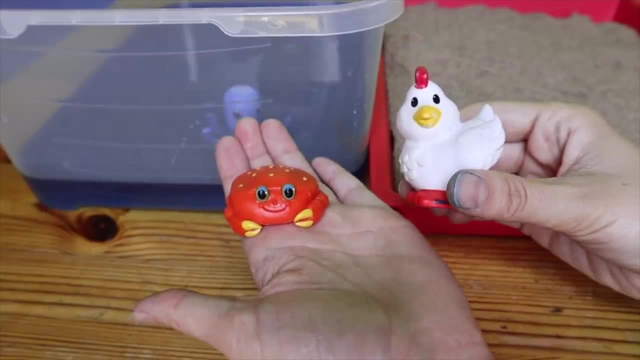 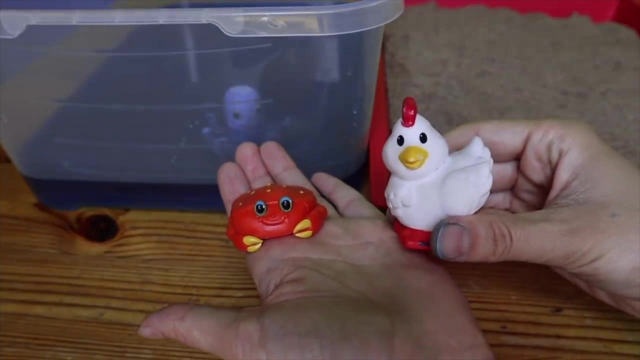 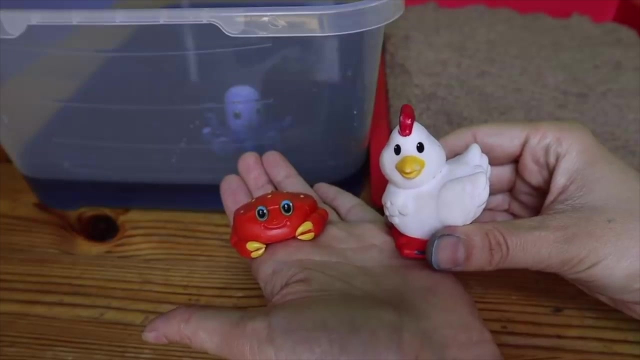 I'm so happy in the ocean. Can you help these animals find their home? Who belongs in the sand, The crab or the chicken? Yeah, the crab. The chicken should go back to the farm. The chicken lives on the farm. so let's say: 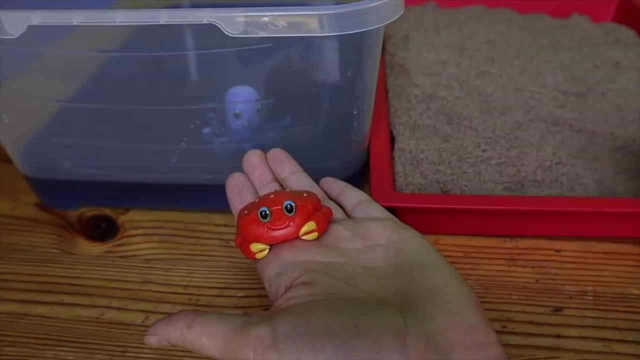 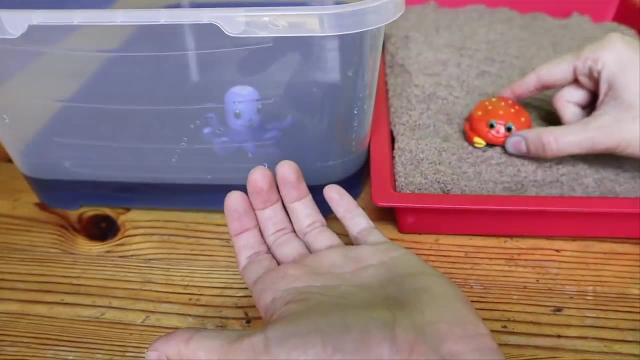 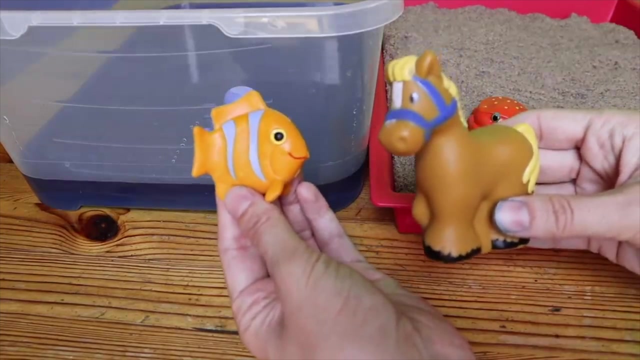 Bye-bye chicken. Bye-bye chicken, Bye-bye. Let's put the crab on the sand, Put it on, put it on, put it on. Thank you so much. I love the sand. Can you help us find our homes? 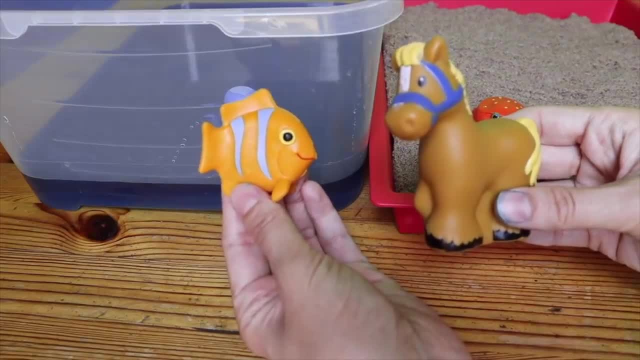 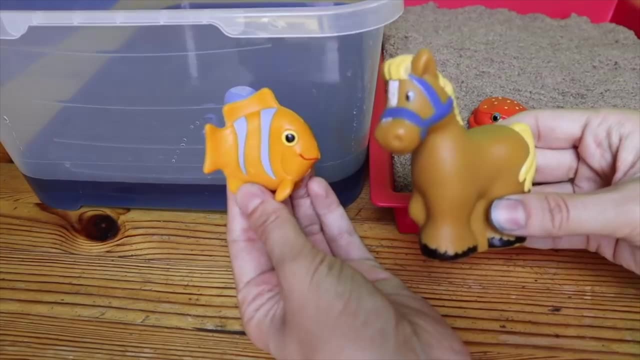 Can you help them? Awesome, Okay, who belongs in the ocean, The fish or the horse? Yeah, the fish. Let's let the horse go back to the farm. You belong on the farm, Mr Horse. Oh, thank you, Bye-bye. 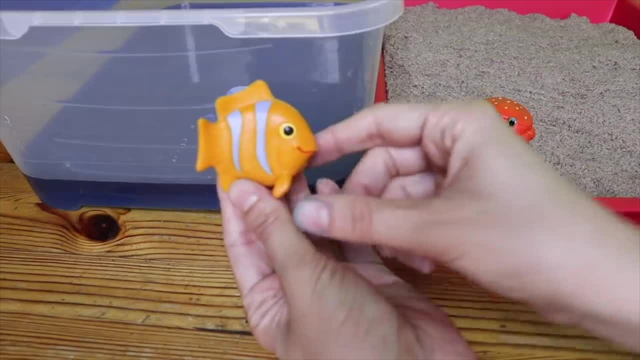 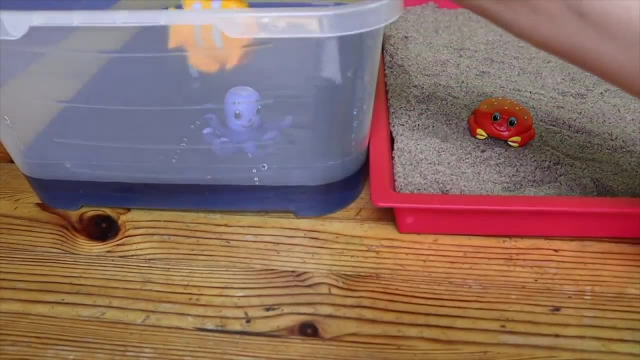 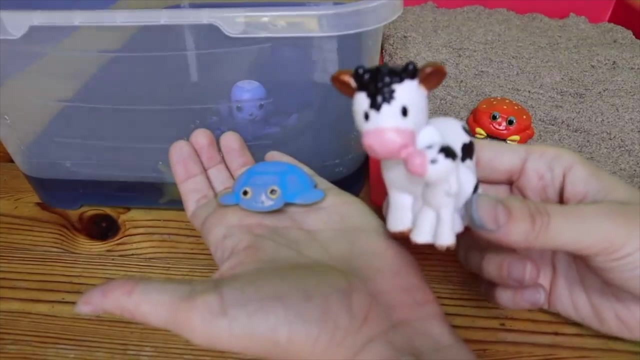 Say bye-bye, horse Bye-bye. Thank you so much. Can you put me in the water, Sure, Put her in. put her in. put her in the water. She's so happy swimming. Can you help us find our homes? 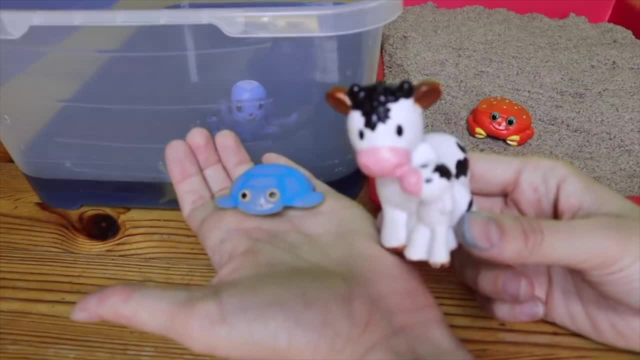 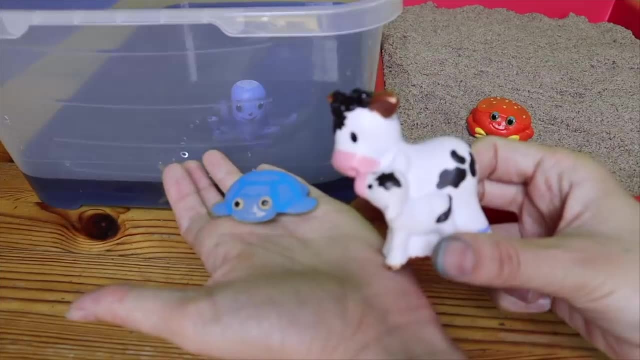 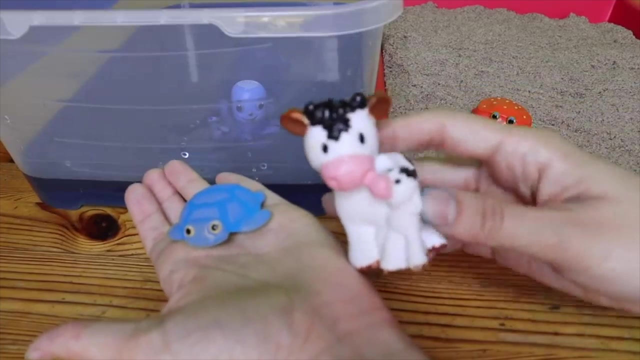 Sure, Hmm, Who would like to go on the sand with the crab, The sea turtle or the cow? Yeah, the sea turtle, The cow is going to go back to the farm. Moo, Moo, Thank you, Bye-bye. 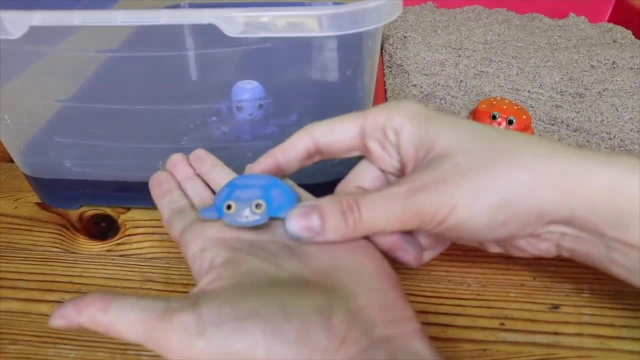 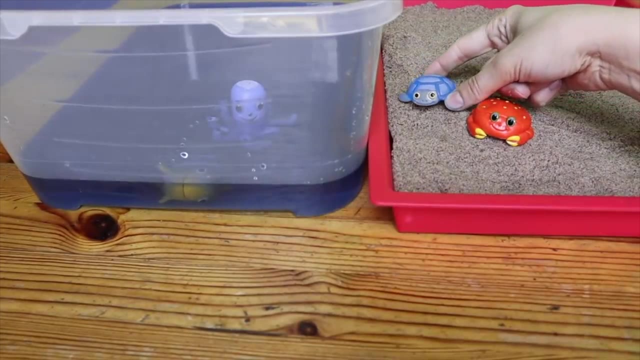 And we'll put the sea turtle in the sand. They also like the water. Thank you so much. I love the sand. Put him on, put him on, put him on. Oh, he's already crawling around. This is fun. 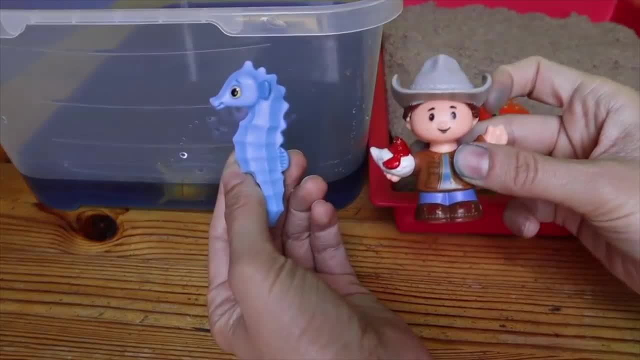 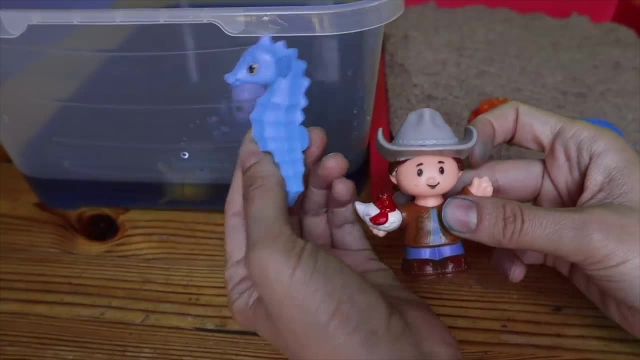 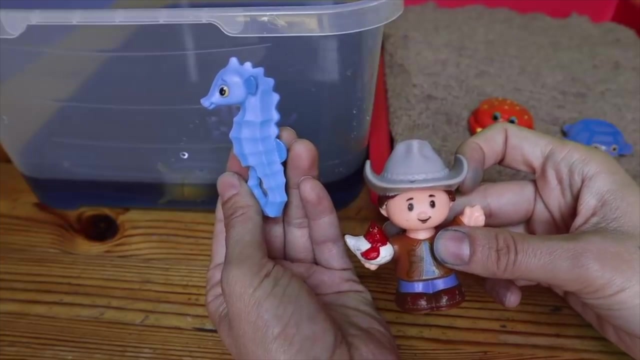 Who should we put in the water, The farmer or the seahorse? This one's kind of tricky, because seahorse has the word horse in its name, But a seahorse actually belongs in the water or the ocean. It swims, And the farmer belongs on the farm. 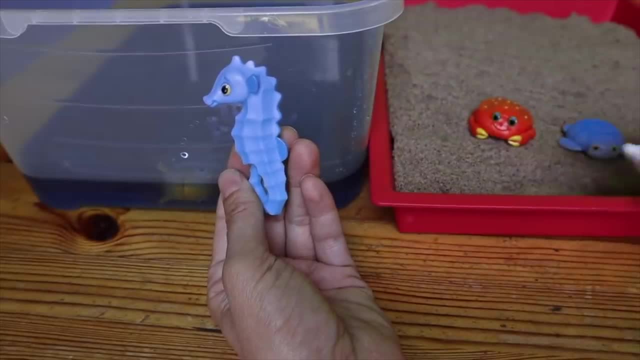 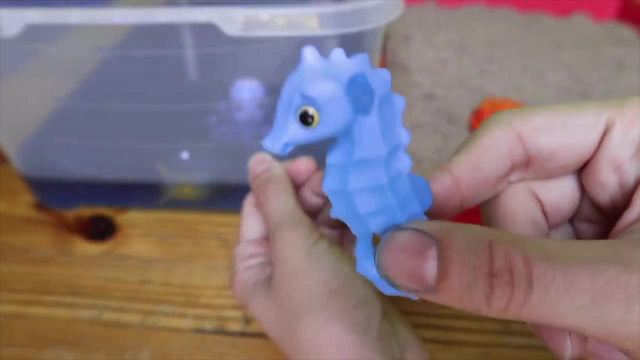 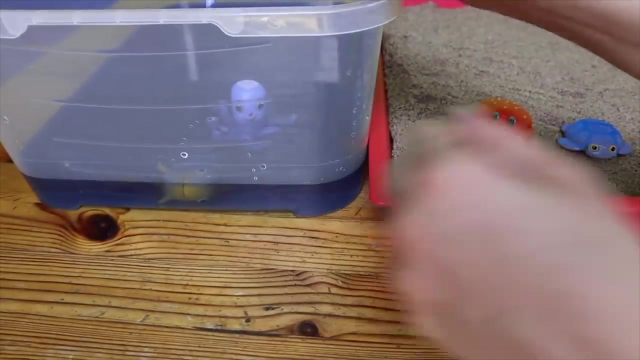 Okay, I'm going back to the farm. Bye-bye, Good job. Thank you so much. You helped me find my home, which is in the water on the beach. Put her in, put her in, put her, Say in and she'll dive in. 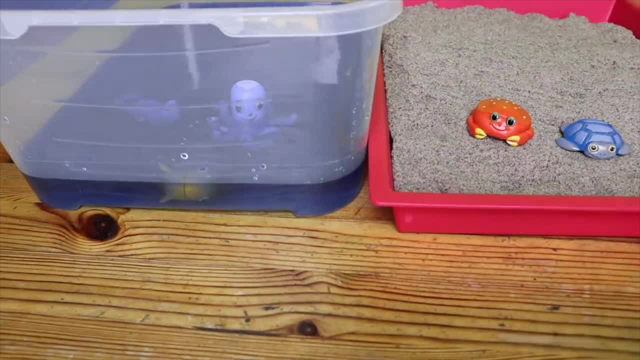 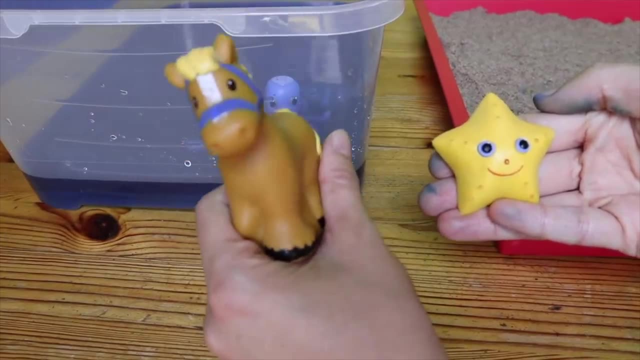 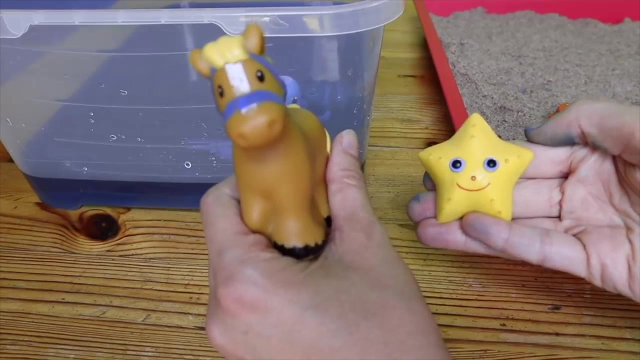 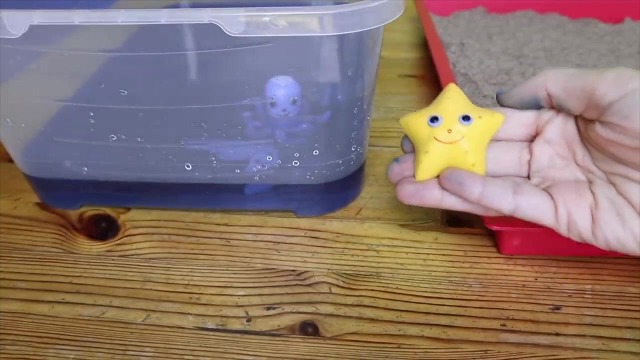 In Yay, Here's our last one. Who belongs on the sand or in the ocean? The horse Nay, Or the starfish? Hello, The starfish. The horse lives on the farm. Nay, Oh, bye, Let's put the starfish in the sand. 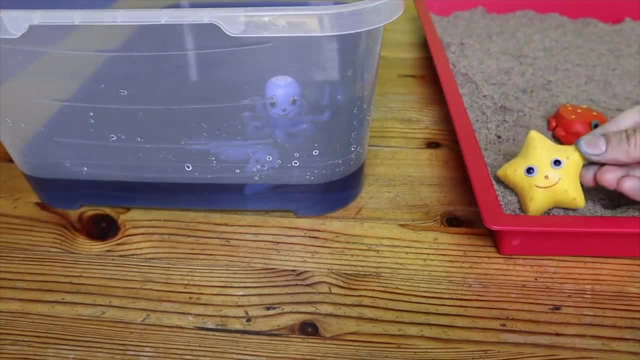 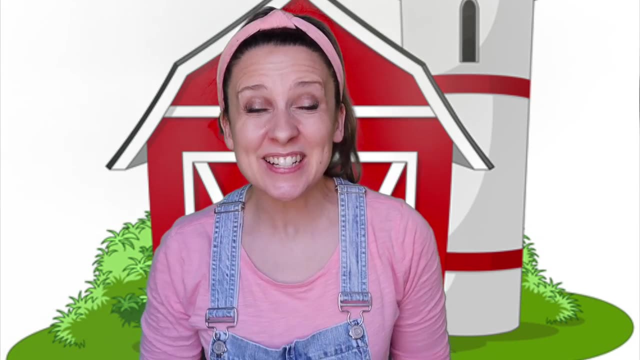 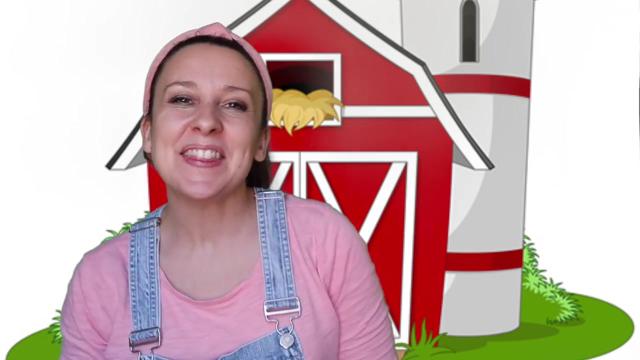 Thank you so much. I love the sand. Ah, I love that. It's so nice. Let's sing: Old MacDonald Had a Farm. Old MacDonald had a farm, E-I-E-I-O, And on that farm he had a horse E-I-E-I-O. 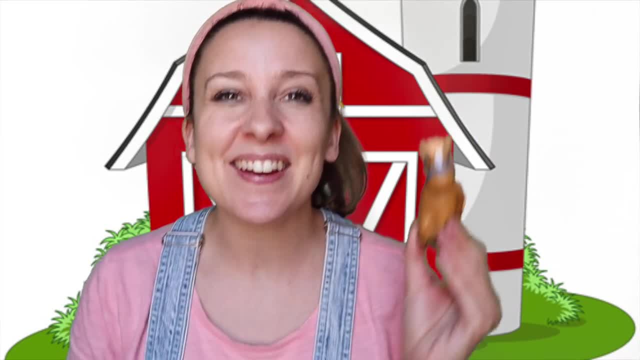 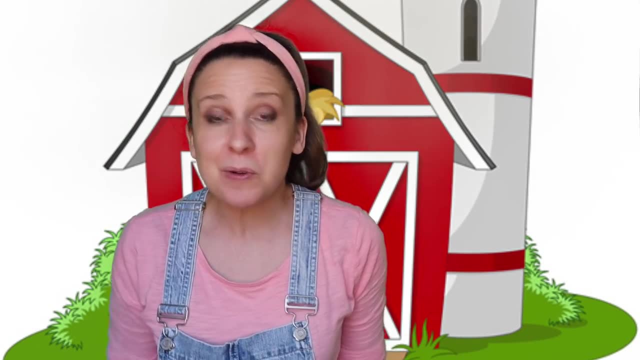 With a nay-nay here and a nay-nay there. Here a nay, there a nay, everywhere a nay-nay. Old MacDonald had a farm, E-I-E-I-O. I wonder what animal will be next. 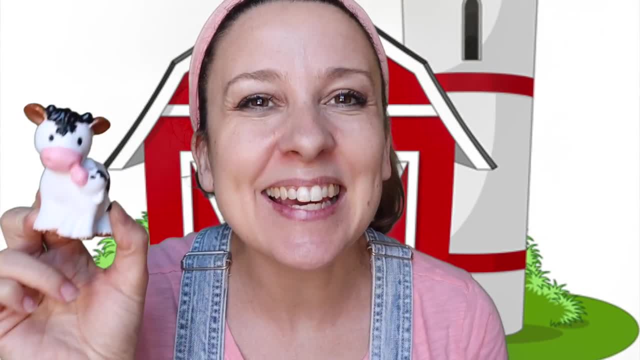 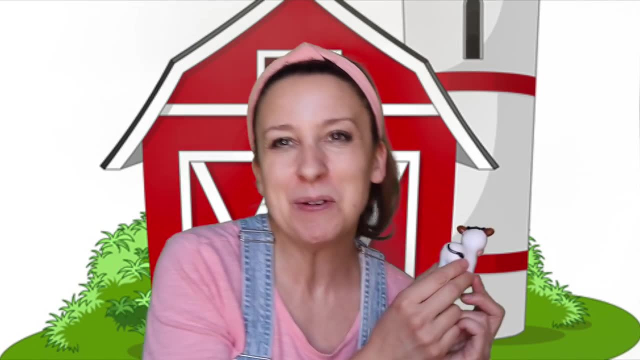 Old MacDonald had a farm E-I-E-I-O And on that farm he had a cow E-I-E-I-O With a moo-moo here and a moo-moo there. Here a moo, there a moo, everywhere a moo-moo. 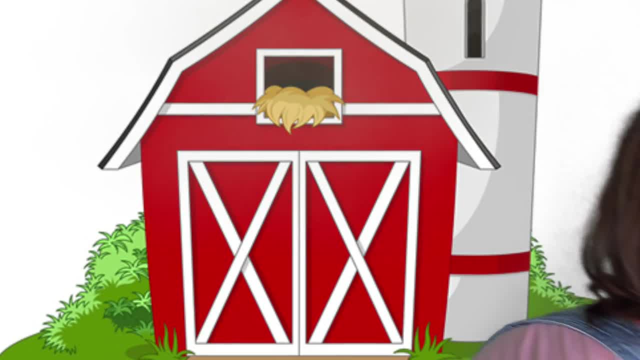 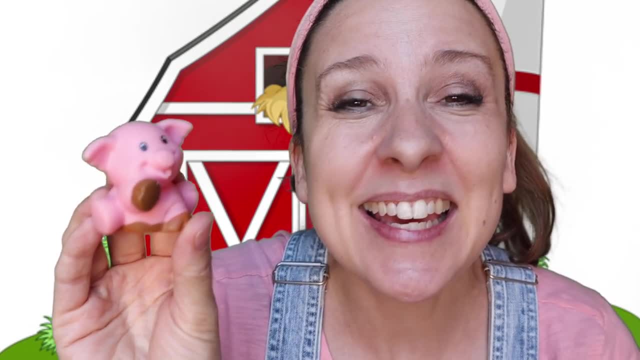 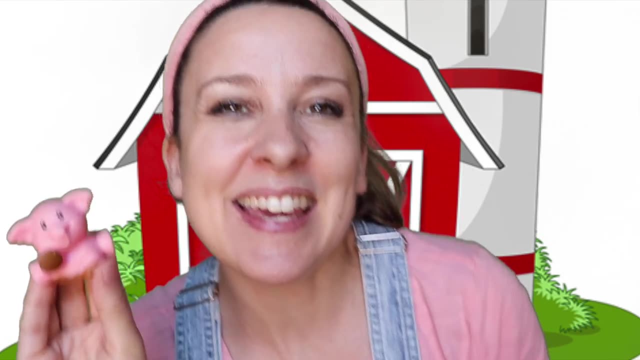 Old MacDonald had a farm E-I-E-I-O. What's next? It's a pig. Old MacDonald had a farm E-I-E-I-O And on that farm he had a pig E-I-E-I-O With an oink-oink here and an oink-oink there. 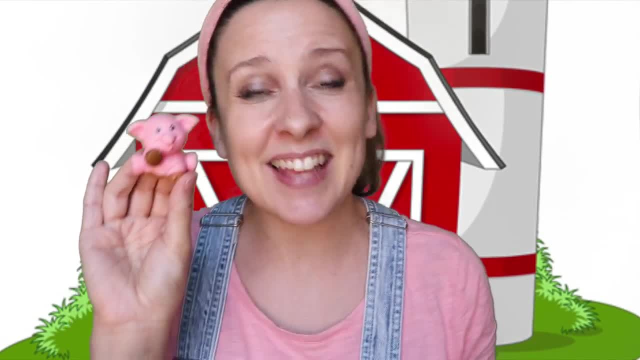 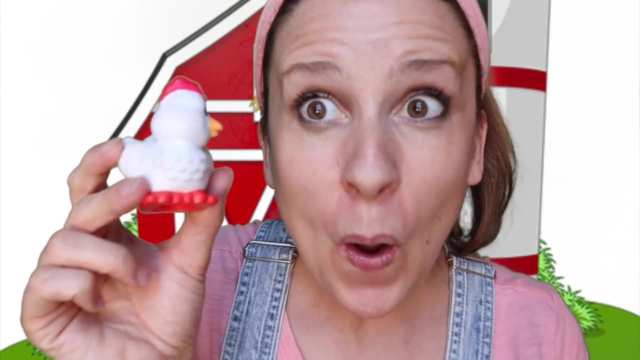 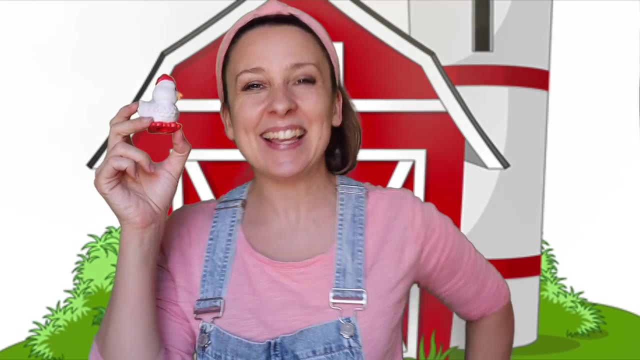 Here an oink, there an oink, everywhere an oink-oink. Old MacDonald had a farm E-I-E-I-O. I hear a chicken. Old MacDonald had a farm E-I-E-I-O And on that farm he had a chicken E-I-E-I-O. 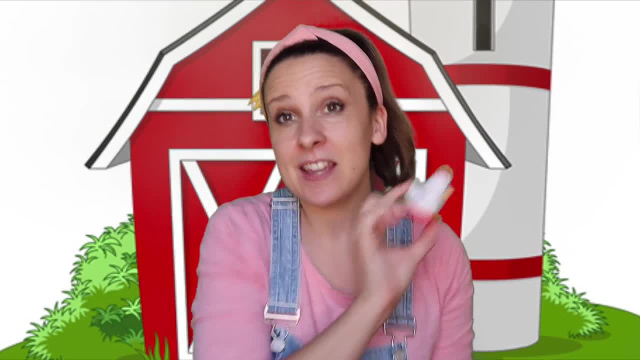 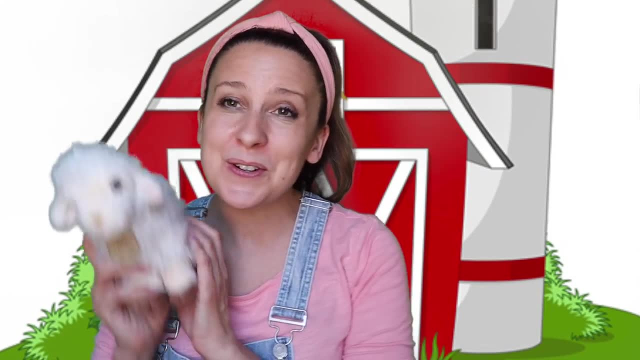 With a cluck-cluck here and a cluck-cluck there. Here a cluck, there a cluck, everywhere a cluck-cluck. Old MacDonald had a farm E-I-E-I-O. Aww, how cute A little sheep. 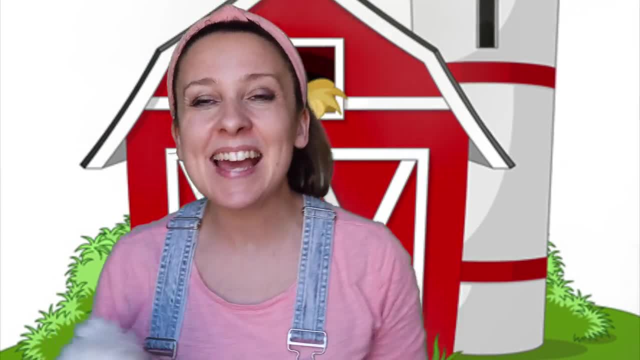 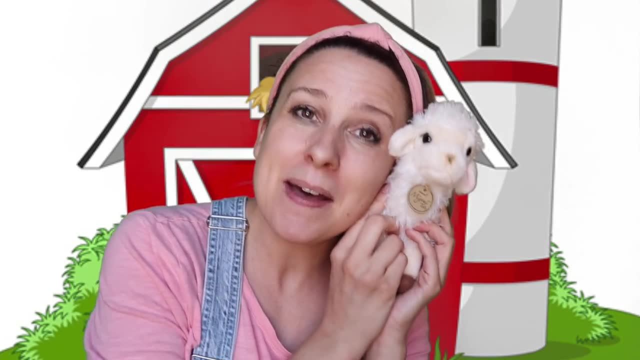 Old MacDonald had a farm E-I-E-I-O And on that farm he had a sheep E-I-E-I-O, With a bye-bye here and a bye-bye there. Here, a bye there, a bye everywhere, a bye-bye. 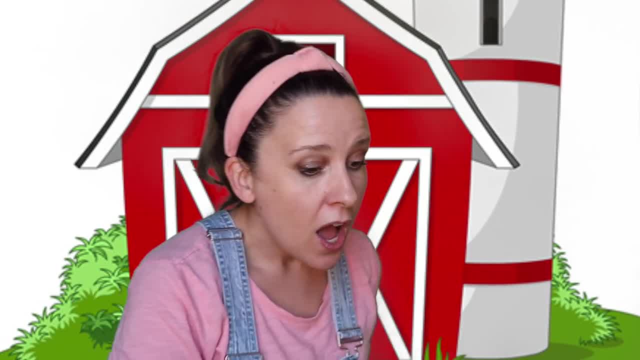 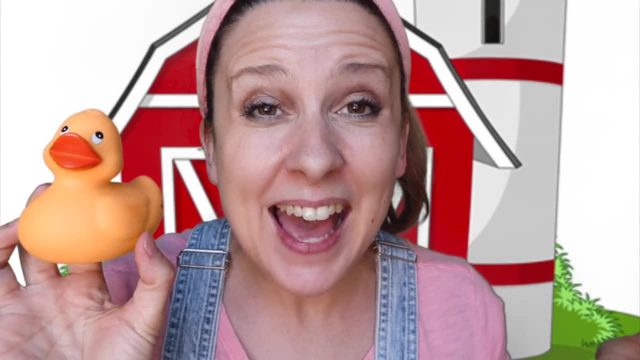 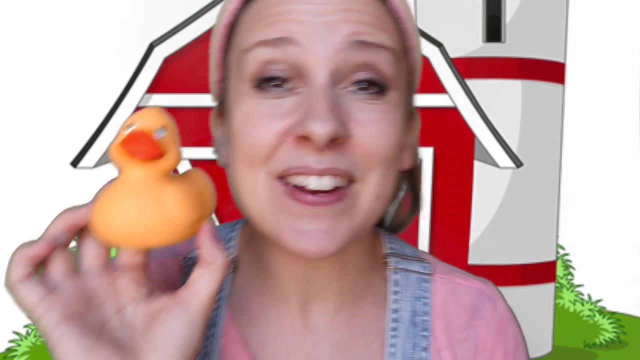 Old MacDonald had a farm E-I-E-I-O, Quack, quack. What says quack? Old MacDonald had a farm E-I-E-I-O And on that farm he had a duck E-I-E-I-O With a quack-quack here and a quack-quack there. 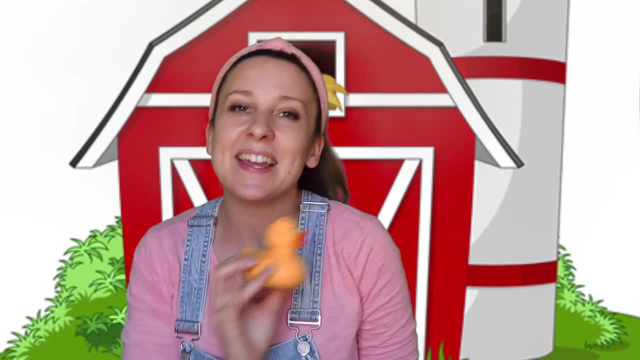 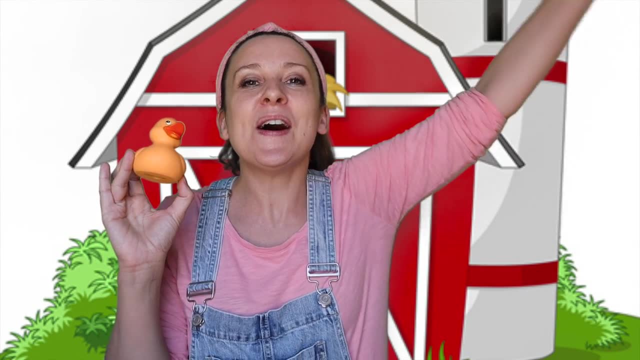 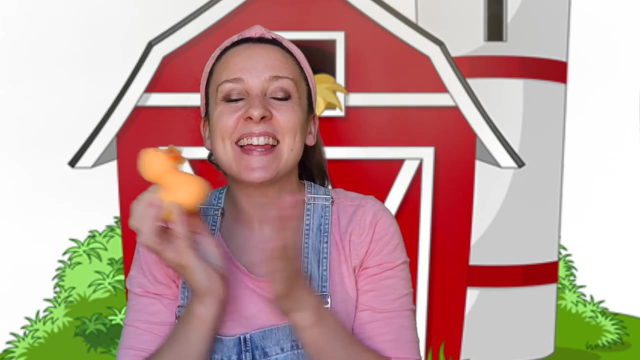 Here a quack, there a quack, everywhere a quack-quack. Old MacDonald had a farm: E-I-E-I-O, E-I-E-I-O, Yay, Great job singing, Old MacDonald. Oh no, This little duck can't find its mama. 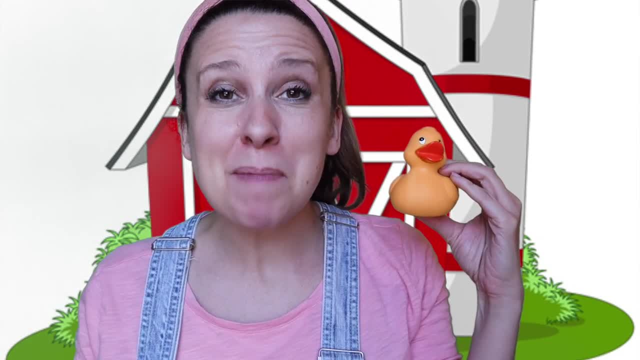 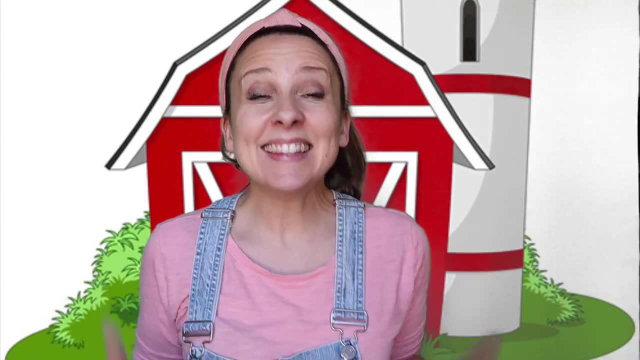 Maybe if we sing Five Little Ducks, the duck will hear its mama quack. Can you help? Can you help me find my mama? Can you help the duck? Let's sing Five Little Ducks. Get out your five little ducks, Good job. 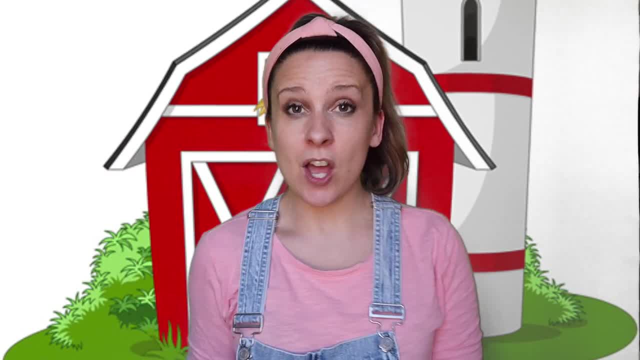 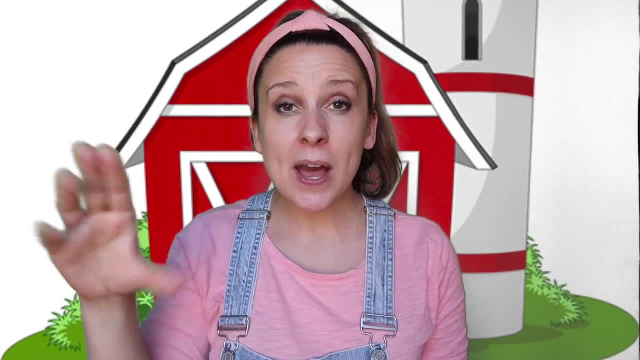 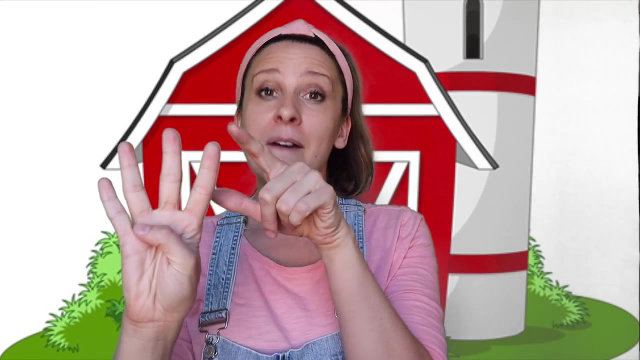 Five little ducks went out one day. Over the hill and far away, Mother duck said quack quack, quack quack. But only four little ducks came back: One, two, three, four, Four little ducks went out one day. 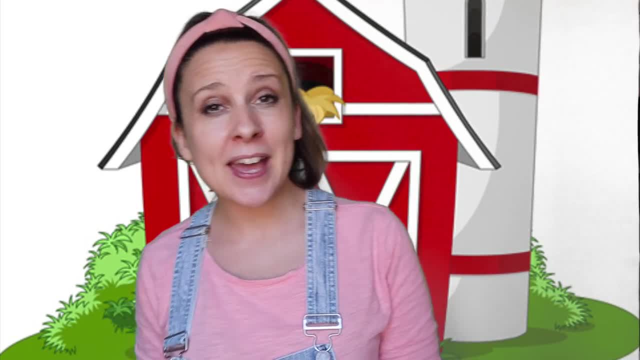 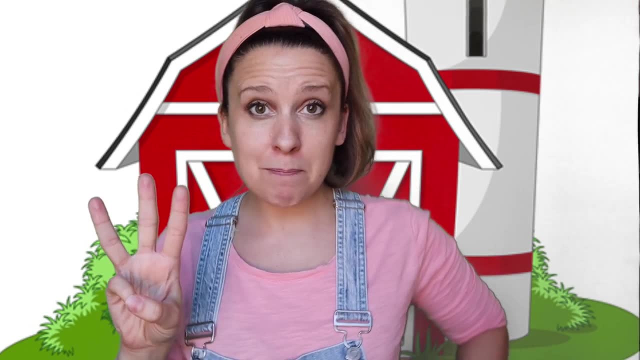 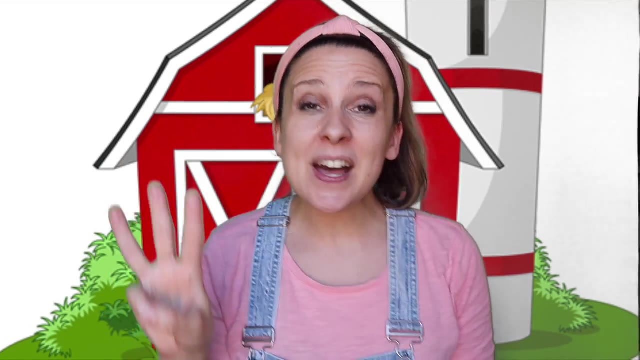 Over the hill and far away. Mother duck said quack quack, quack quack, But only three little ducks came back. One, two, three, Three little ducks went out one day Over the hill and far away. 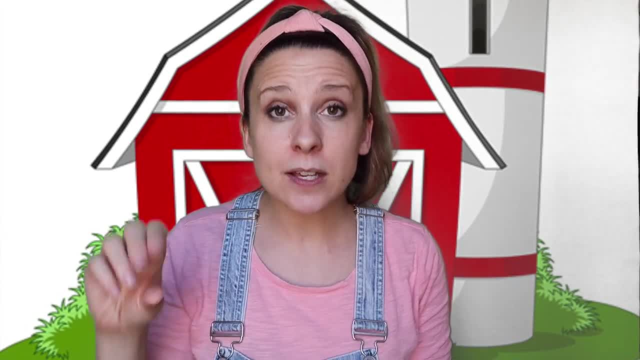 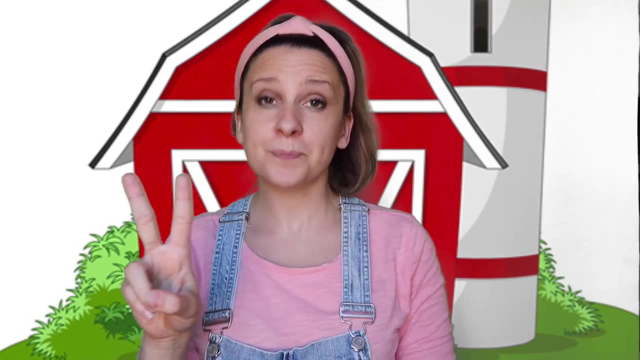 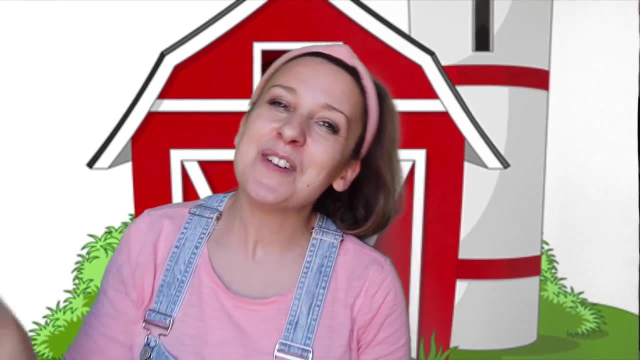 Mother duck said quack quack, quack, quack. But only two little ducks came back. One, two, Three little ducks went out one day, Over the hill and far away. Mother duck said quack quack, quack, quack. 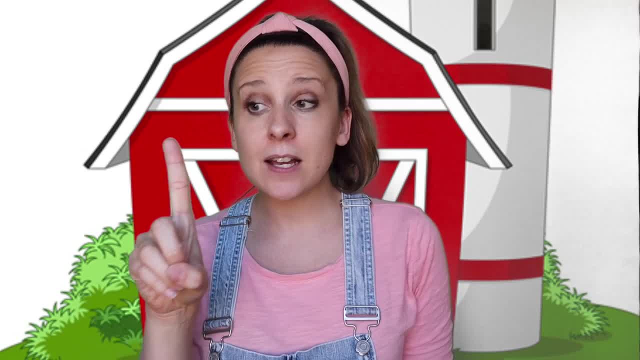 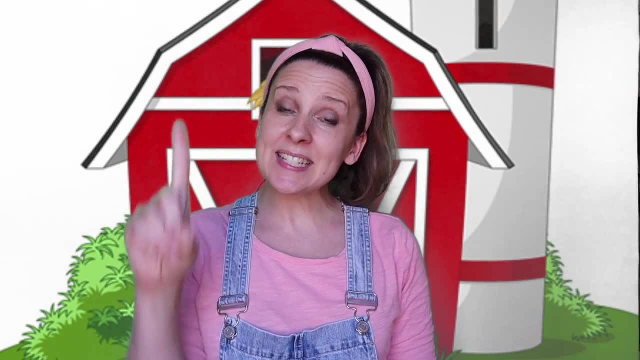 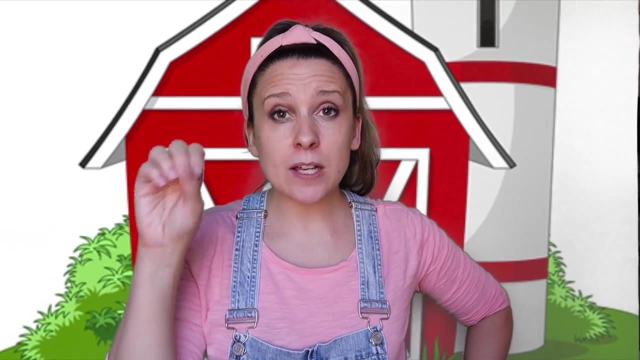 But only one little duck came back. Can you show me one, Just one, One finger. One little duck went out one day, Over the hill and far away. Mother duck said quack quack, quack, quack, But none of the five little ducks came back. 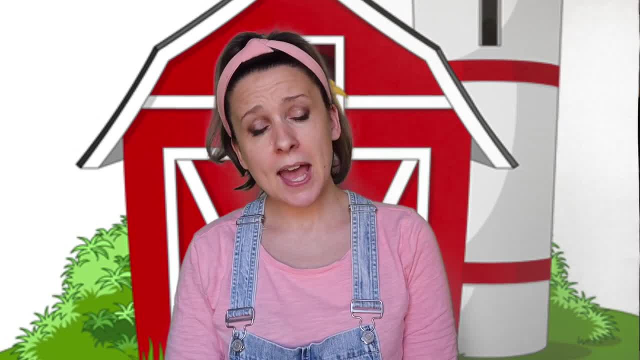 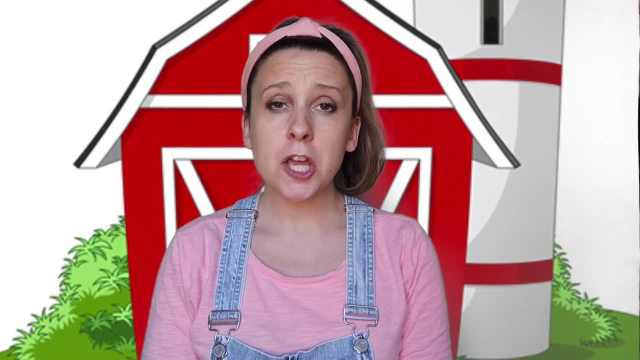 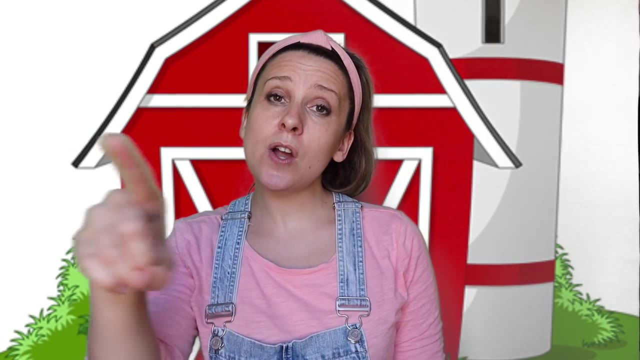 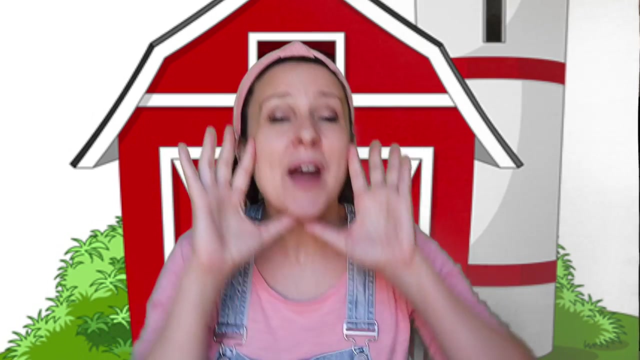 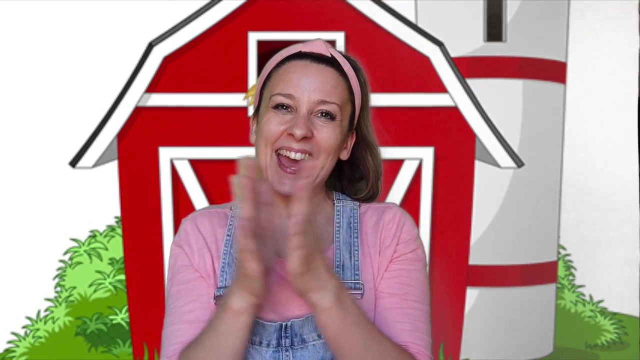 Mother duck is feeling very sad. Sad mother duck went out one day, Over the hill and far away, Mother duck said quack quack, quack, quack, And all of the five little ducks came back. Yay, The duck found its mama. 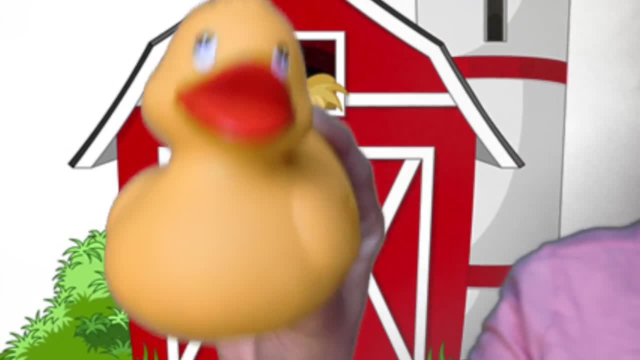 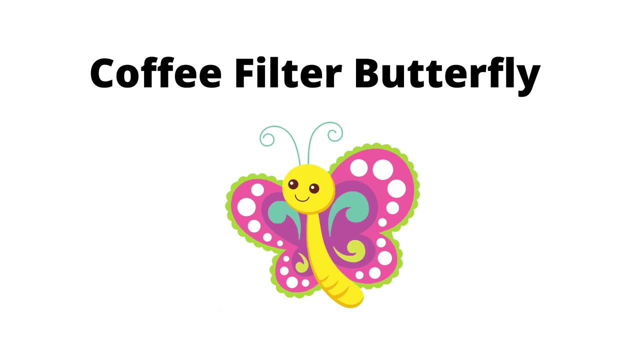 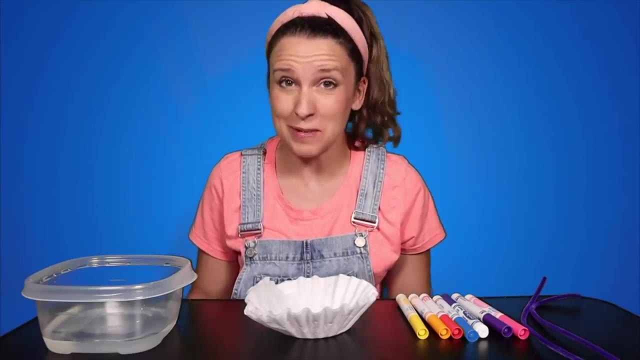 Thank you so much. I found my mama. Yay, Thank you. Give you a kiss. Hi friends, It's time for art. I can't wait to make coffee filter butterflies with you. It's going to be so much fun. 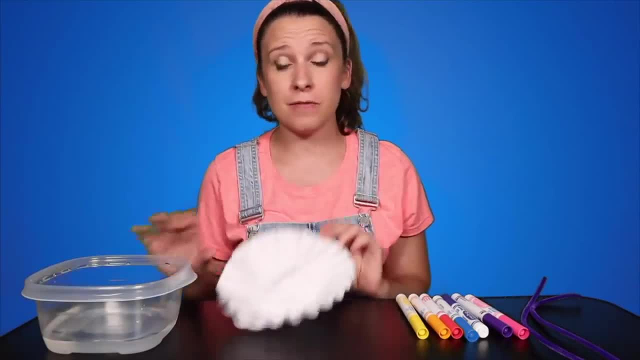 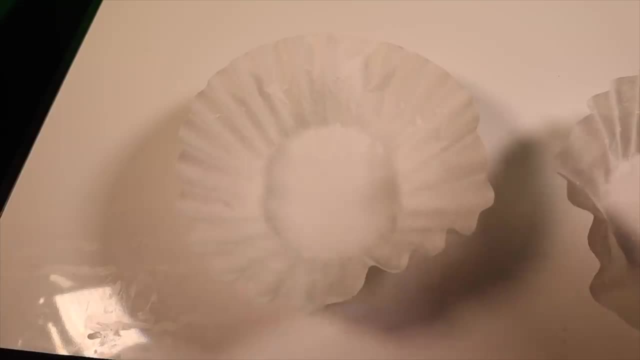 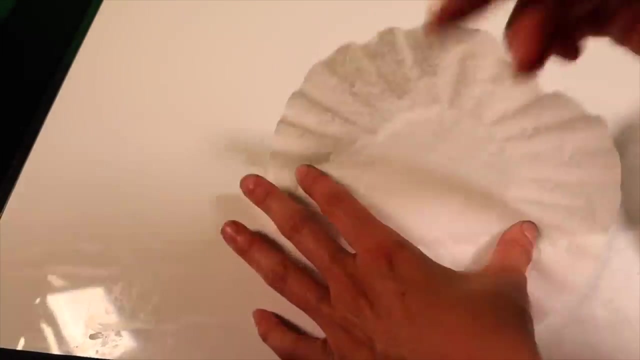 Okay, all you need for this are two coffee filters, some water markers and pipe cleaners. Let's get started. Okay, so the first thing we need to do is decorate two coffee filters. Alright, so let's start in the middle. 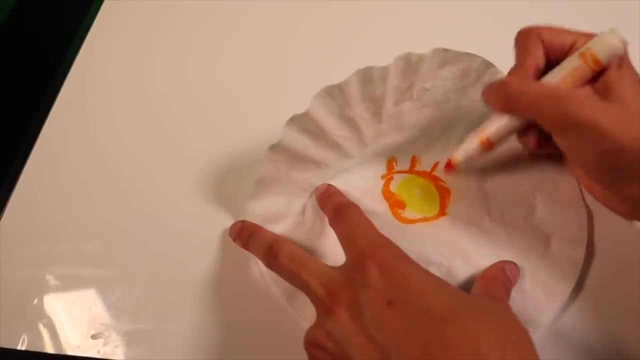 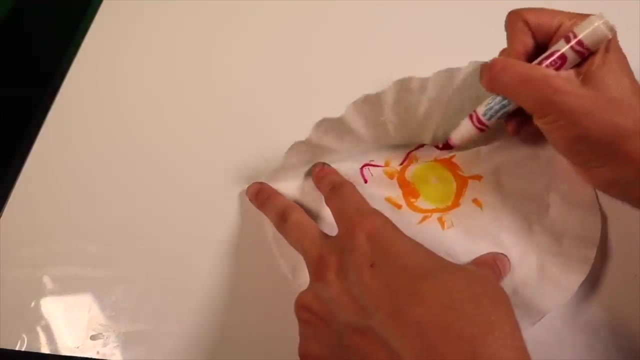 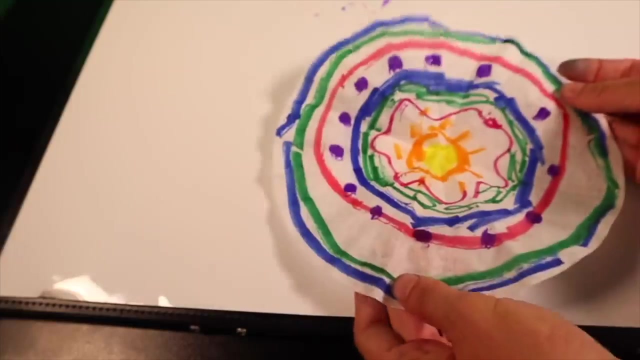 And you can do any designs you want. Work from the inside out. I think I'll do a wavy line next, Whoo Wavy line. Then you can spray it with water Or you can fold it. Fold it again. 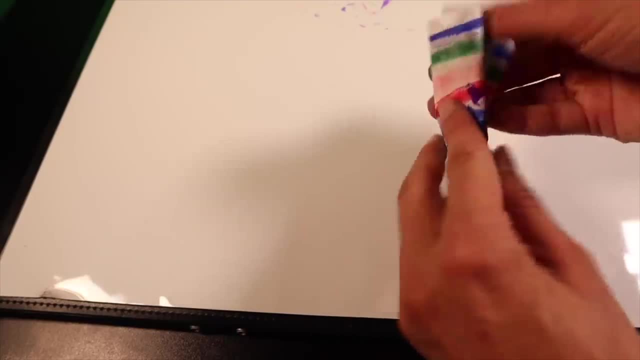 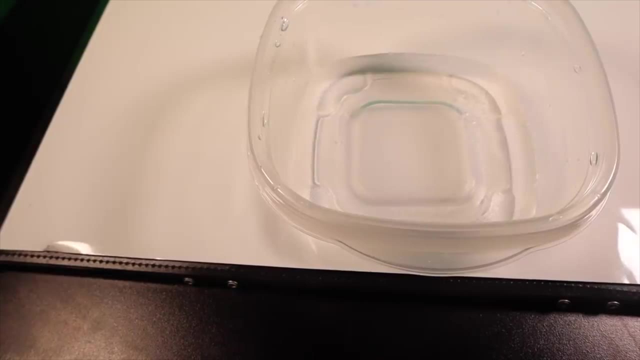 Fold it again into a triangle shape And do something kind of magic with it. I'll show you. So. you get a little thing of water, And then you put just the tip in the water And you wait for the water to climb up. 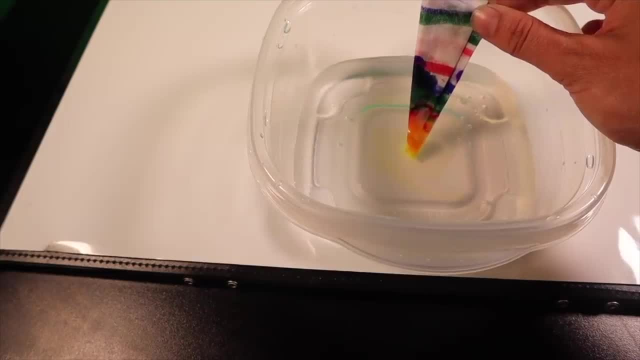 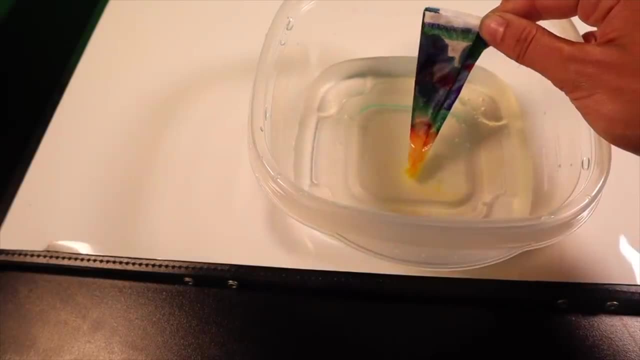 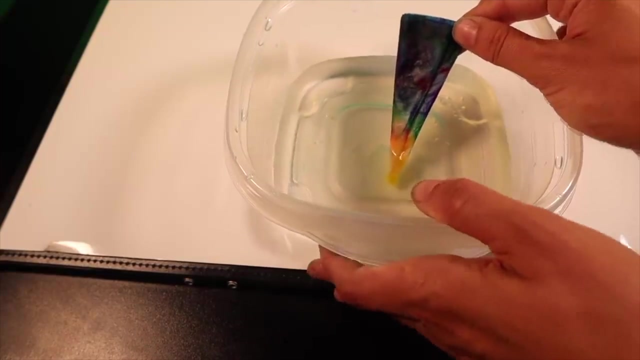 Up, Up the coffee filter to the top. It takes a lot of patience to just wait for this water to come to the top. Wow, I waited the whole time. I'm so proud of myself. Now it's time for the magic. 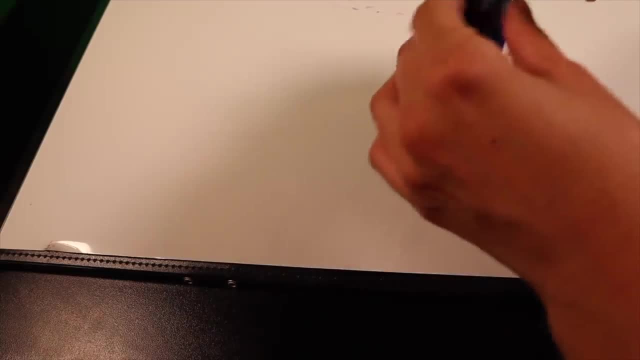 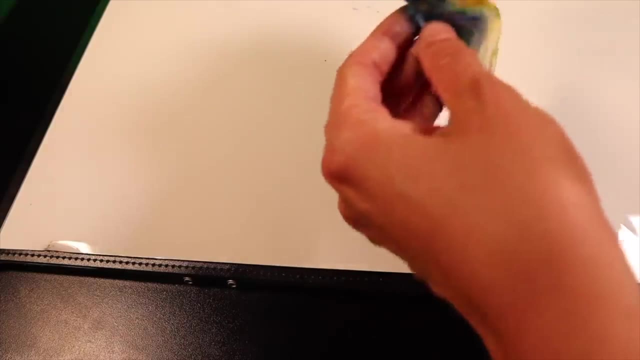 We're going to open it and see how beautiful it is. Okay, let's open the coffee filter. Ooh, it looks really, really cool. I love it. I used to do this all the time when I was a little girl. 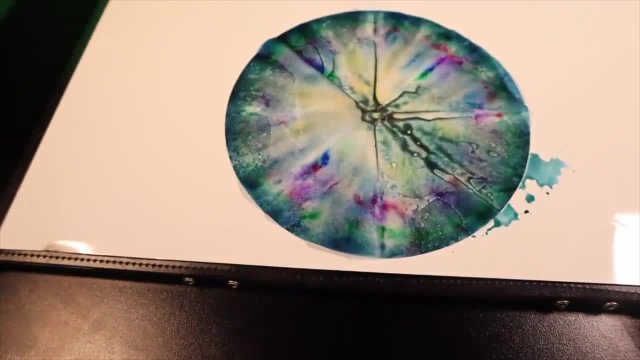 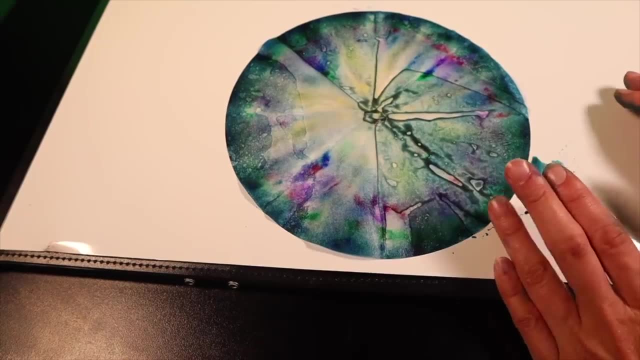 Oh wow, That looks so pretty, doesn't it? And then we let it dry. It has to dry for quite a while because we want it to be really nice and dry to make the wings. So you're going to do that two times. 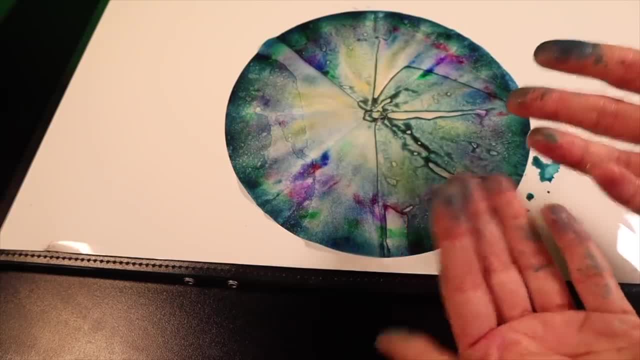 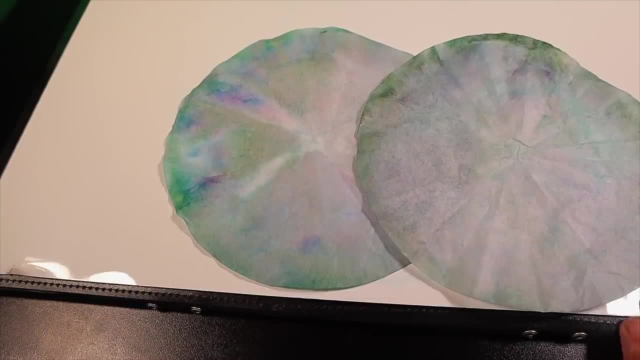 One, two. My hands are all dirty. That's okay, though I don't mind, because I can go wash them. Okay, the wings are dry and they look so nice. Now we're going to fold them like a fan, So you fold it. 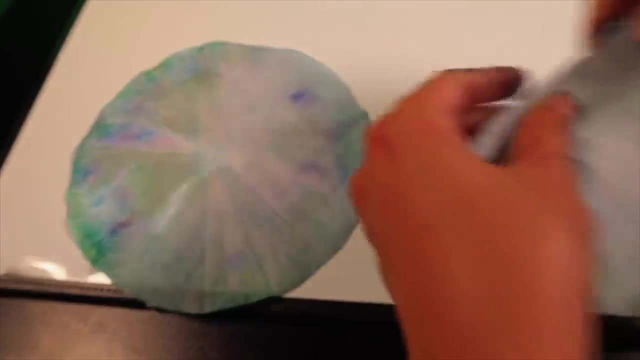 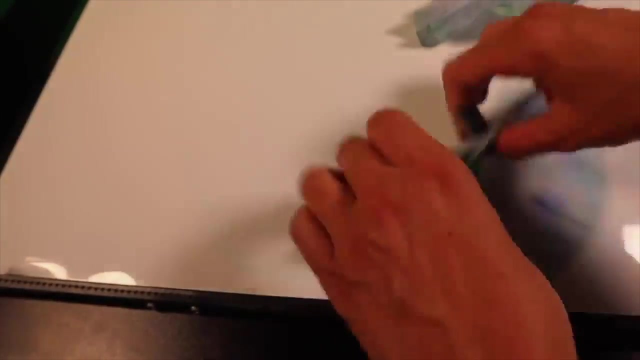 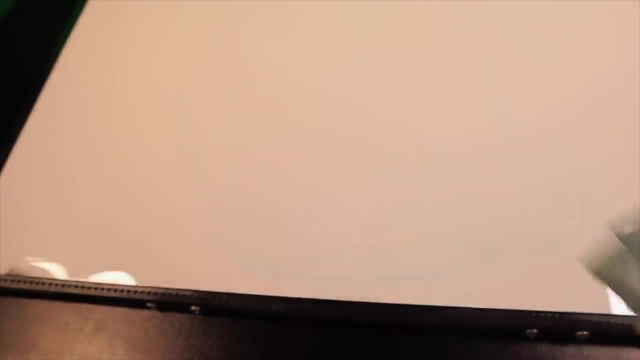 I'm going to turn it over, Fold it, Folding it like a fan. Now let's put the two wings together. I love this butterfly so much. Oh, my goodness, Spread out the wings And I'm going to add a pipe cleaner. 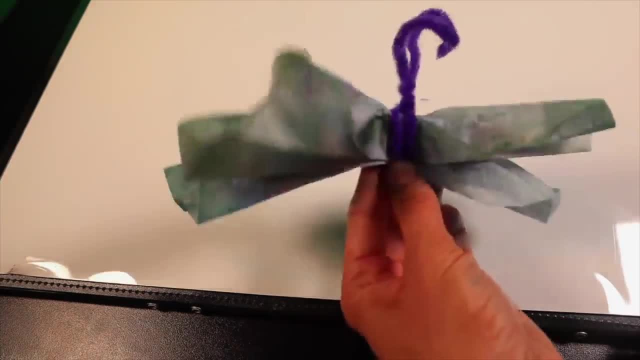 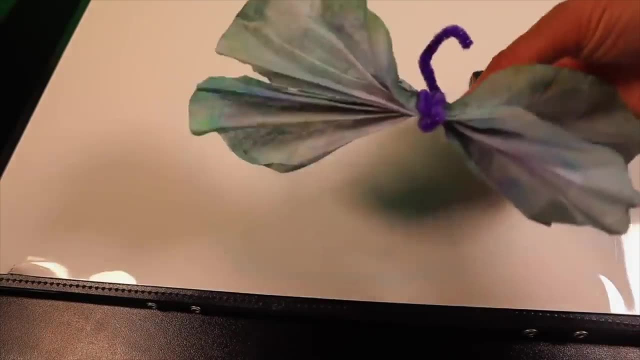 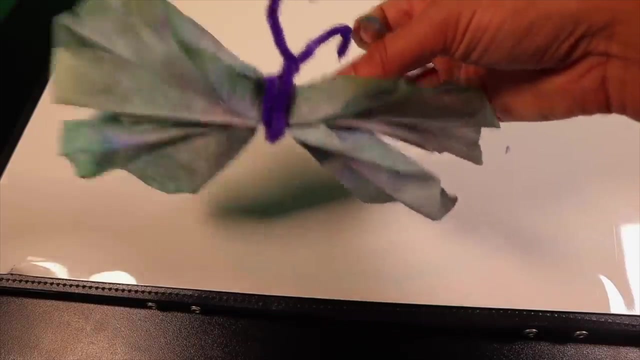 And it's a beautiful butterfly. Yay, It's flying away. I'm so proud of us for making a coffee filter butterfly with two beautiful wings. Thank you so much. Now I can go fly away. Woo, If you're happy and you know it, clap your hands. 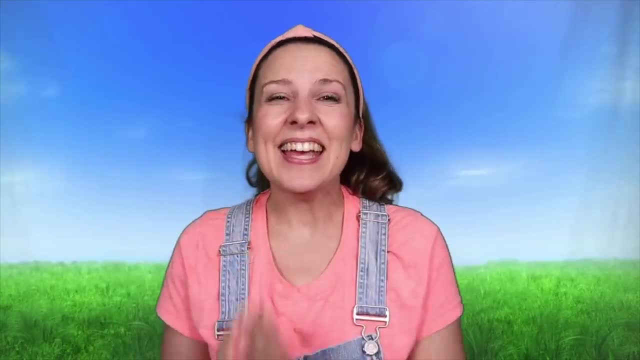 If you're happy and you know it, clap your hands. If you're happy and you know it, and you're really happy. If you're happy and you know it and you really want to show it, If you're happy and you know it, clap your hands. 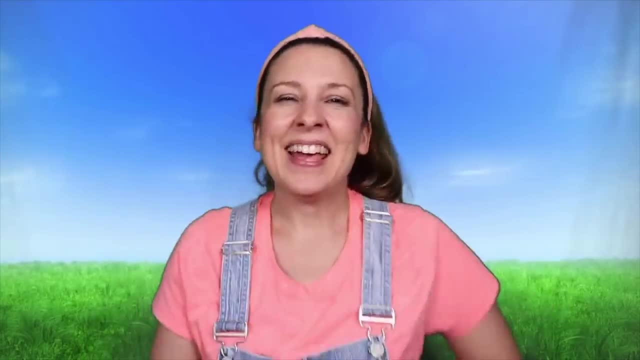 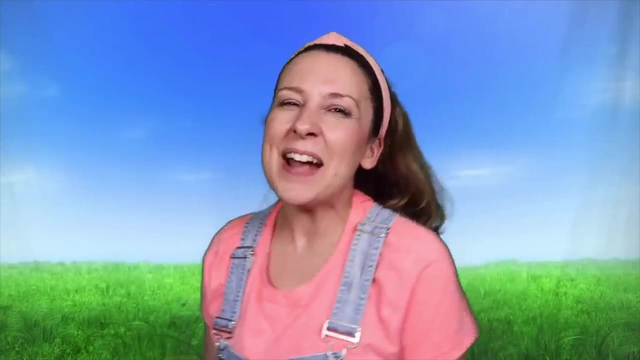 If you're happy and you know it, stomp your feet. If you're happy and you know it, stomp your feet. If you're happy and you know it and you really want to show it, If you're happy and you know it, stomp your feet. 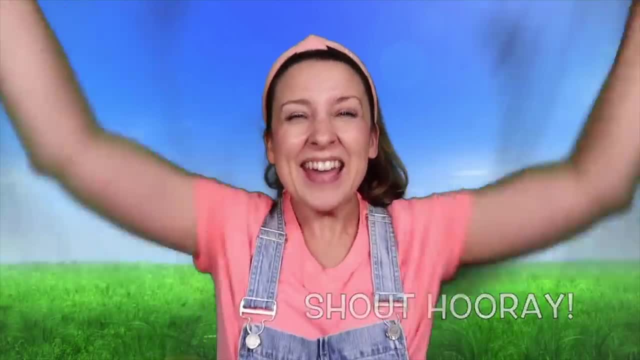 If you're happy and you know it, shout hooray hooray. If you're happy and you know it, shout hooray hooray. If you're happy and you know it and you really want to show it. 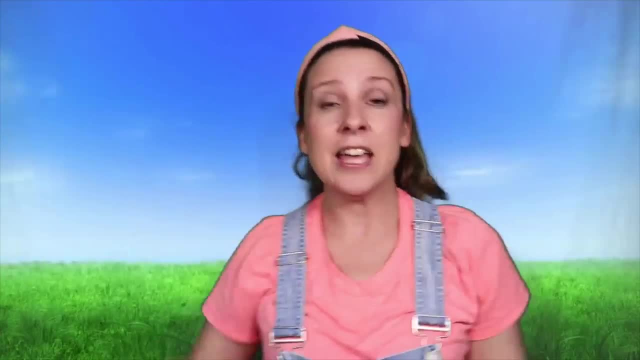 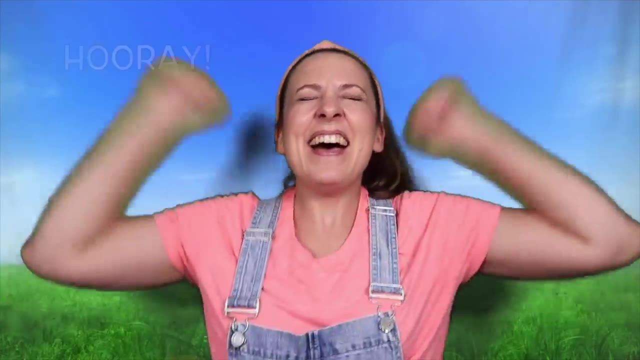 If you're happy and you know it, shout hooray, hooray. Do you think we could do all three? If you're happy and you know it, do all three, Hooray. If you're happy and you know it, do all three. 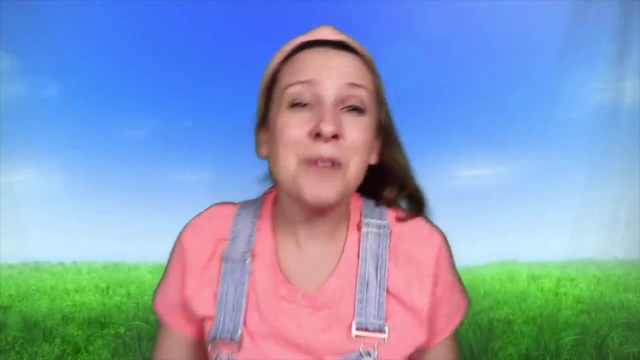 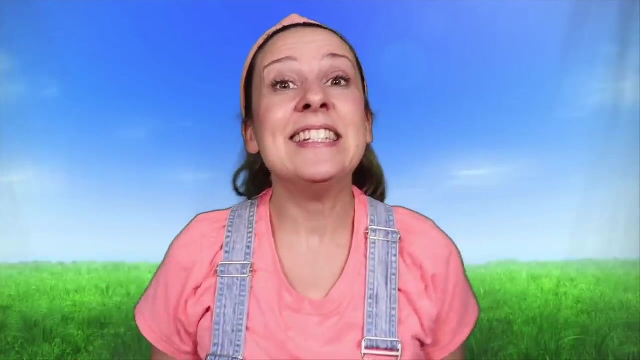 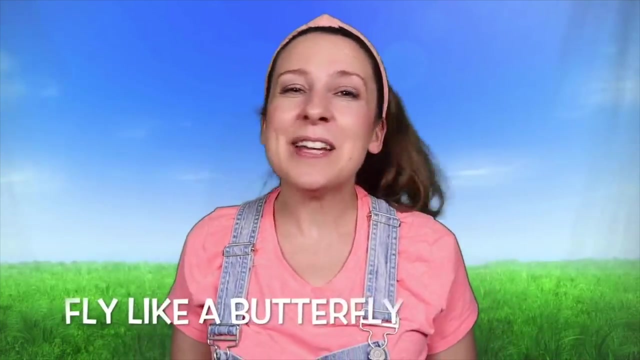 Hooray, If you're happy and you know it and you really want to show it. If you're happy and you know it, do all three Hooray. Now let's pretend to fly like a butterfly. If you're happy and you know it, fly like a butterfly. 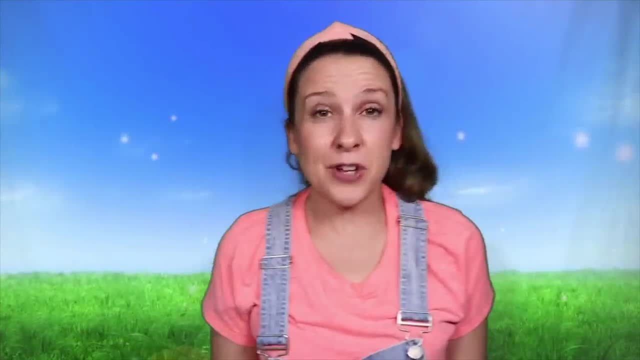 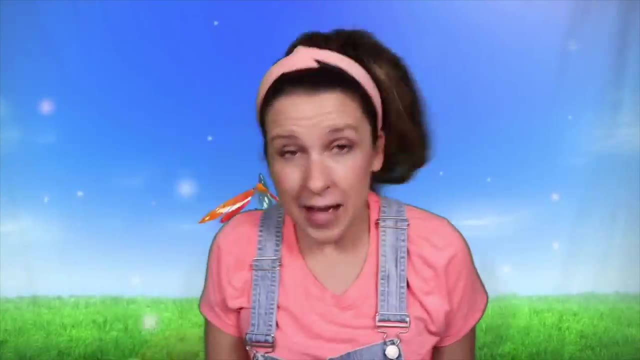 Oh good flying. If you're happy and you know it, fly like a butterfly. Oh beautiful. If you're happy and you know it and you really want to show it. If you're happy and you know it, fly like a butterfly. 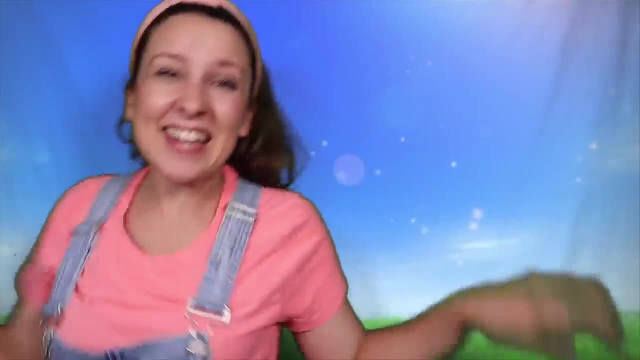 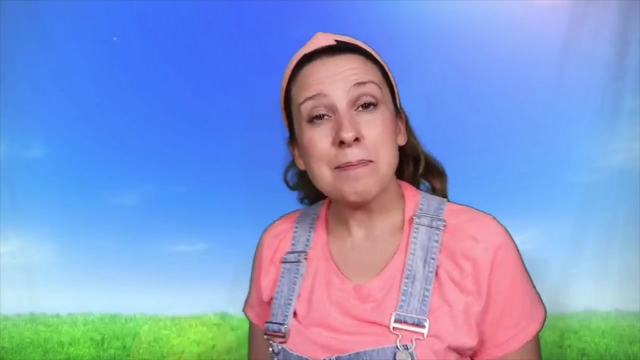 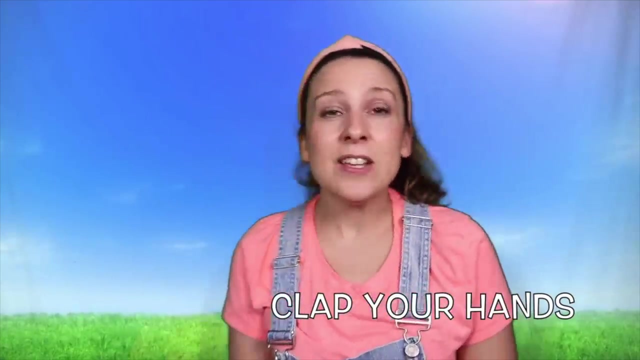 So pretty Good flying. Wow, That was so much fun, Great job. If you're happy and you know it, clap your hands. If you're happy and you know it, clap your hands. If you're happy and you know it and you really want to show it. 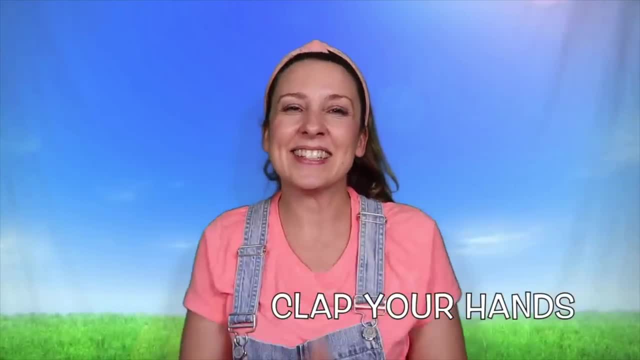 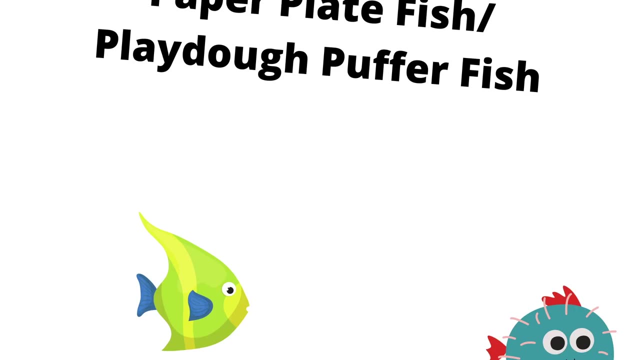 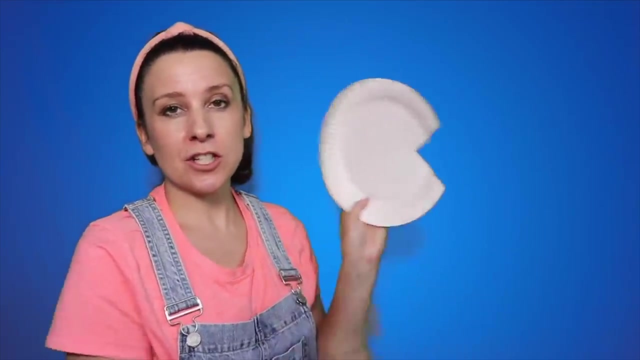 If you're happy and you know it, clap your hands. Yay, Wow, you did such a great job. Let's talk about how to do a few ocean art projects. So for this project, all you need is a paper plate. 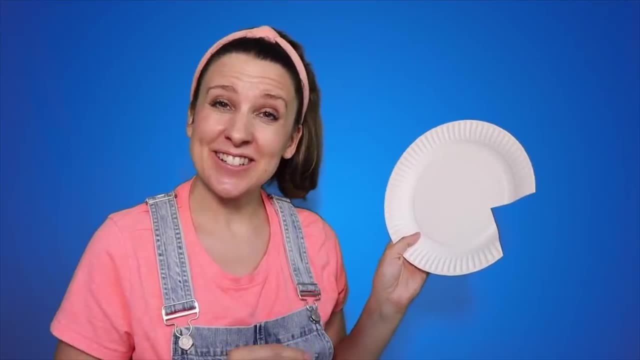 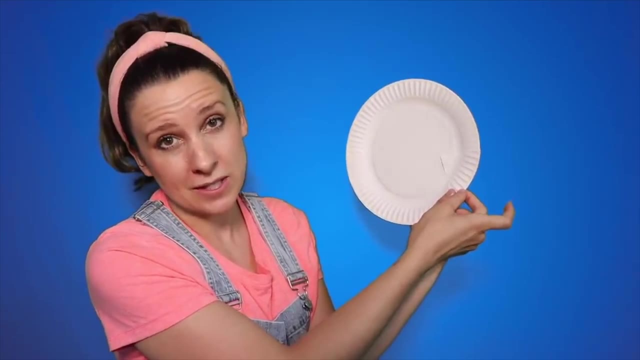 some tape and some markers or crayons. So the first thing you're going to do is cut a little slice out right there and get a parent's help with scissors, And then you take that part and you're going to put it on here. 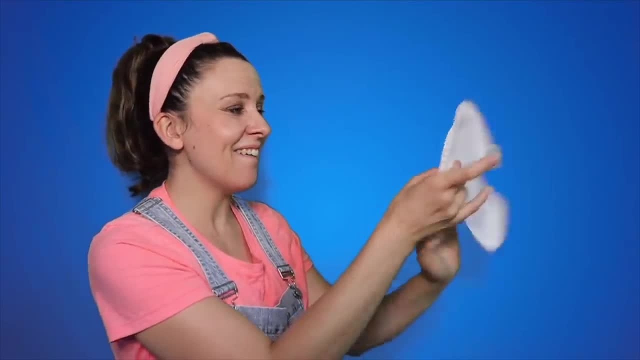 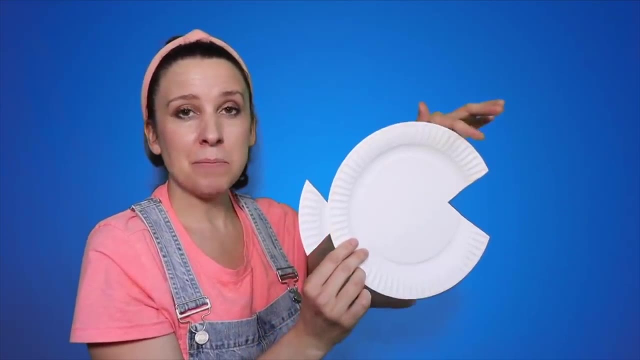 and it's going to become the tail. Wow. So you just tape the tail And now you have a paper plate fish. You can put some fins on the top with paper too, if you want. I picked a blue marker, since it's a blue fish. 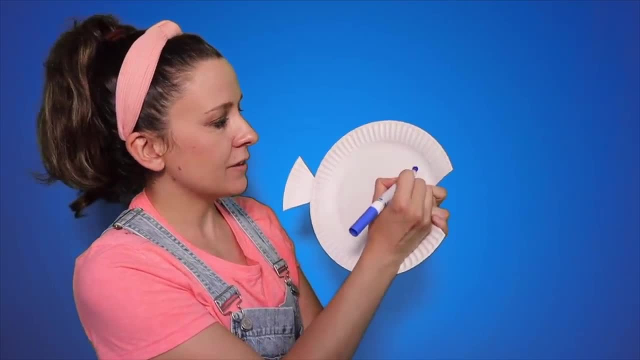 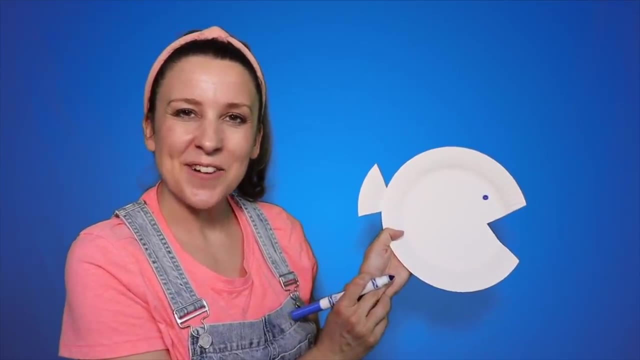 It's the color of the day And I'm going to give the fishy a little eye. Great, He has an eye now, And then you can decorate it in any way you want. For this project, you draw a puffer fish. 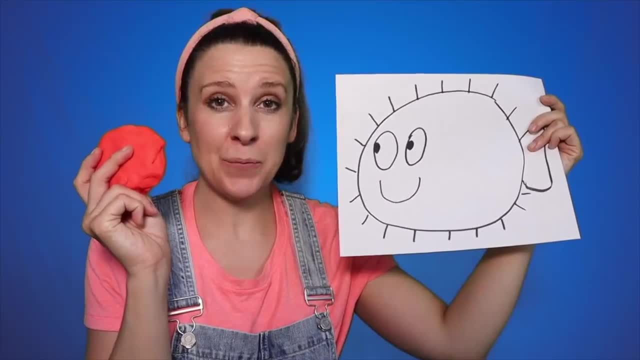 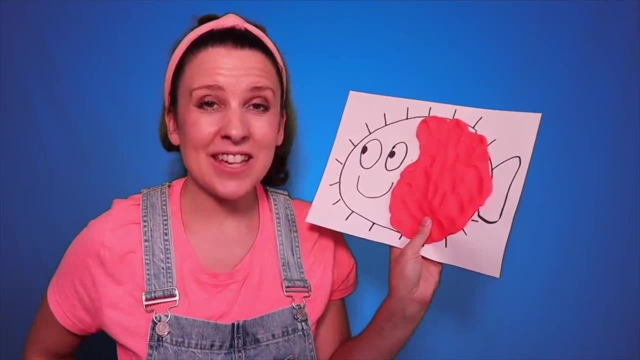 Hi, puffer fish. And then you get out some Play-Doh, okay, And then you're going to flatten the Play-Doh onto the fish. Okay, I flattened my Play-Doh onto the fish. Then you take some pipe cleaners and, with a grown-up's help, 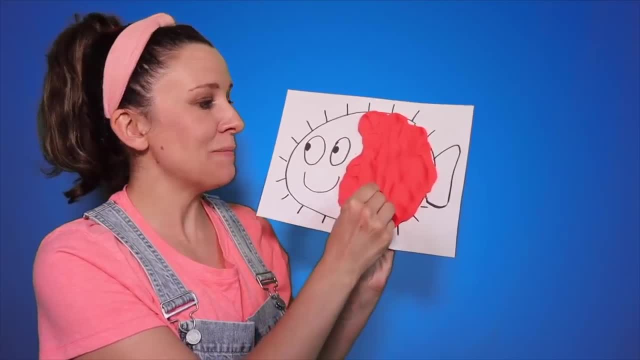 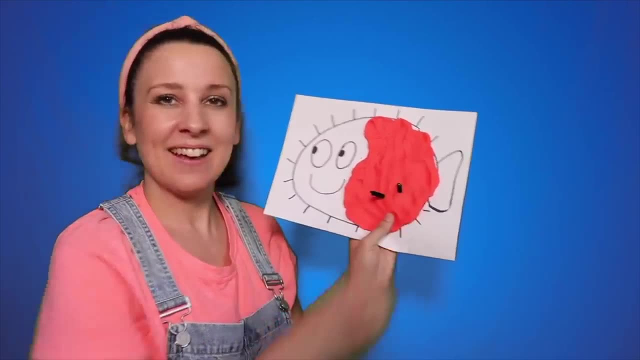 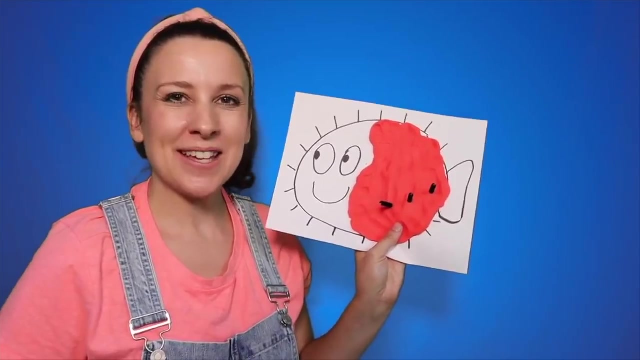 you cut them up into smaller pieces And then you stick them in the puffer fish And now he has some spikes In. Wow, Can you help Say in In: Ooh, he's getting really spiky. 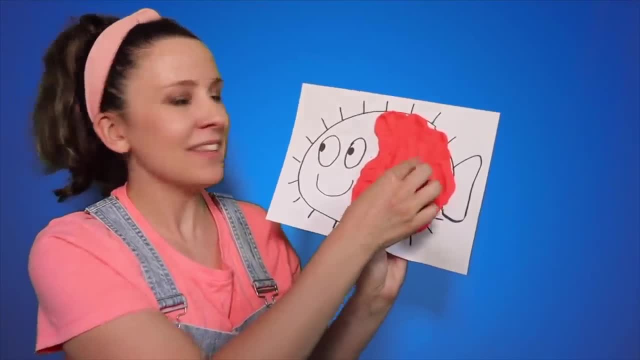 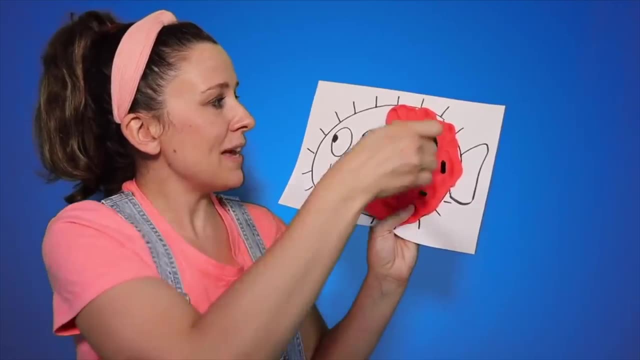 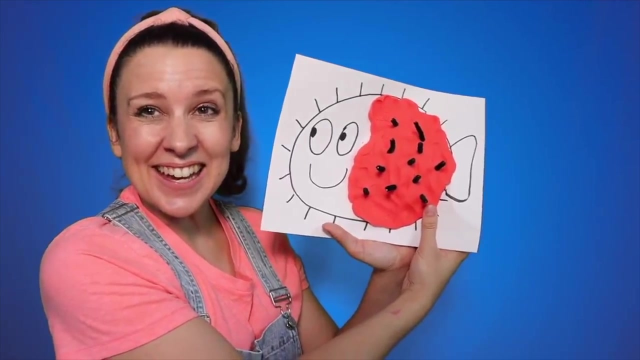 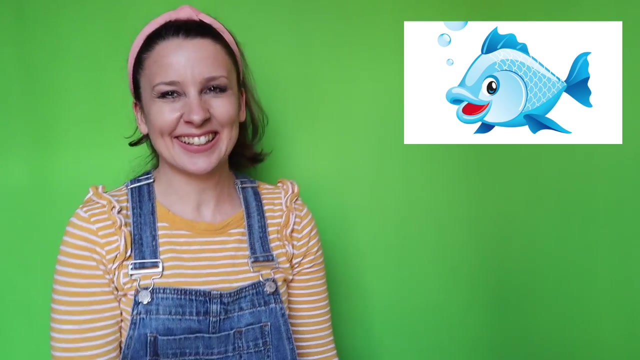 Thank you for my spikes. You're welcome In In So spiky. One more spike and we're done In. Wow, Look what we made. Great job. Let's get out one little blue fish. Are you ready? 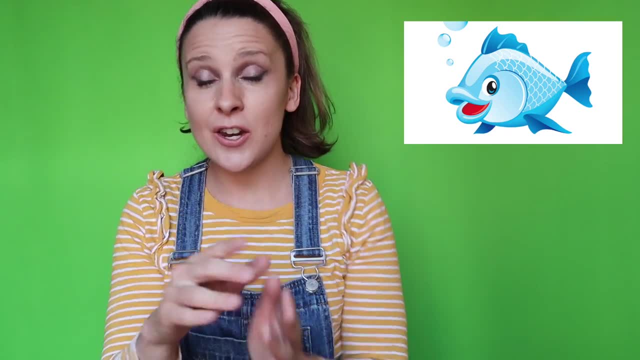 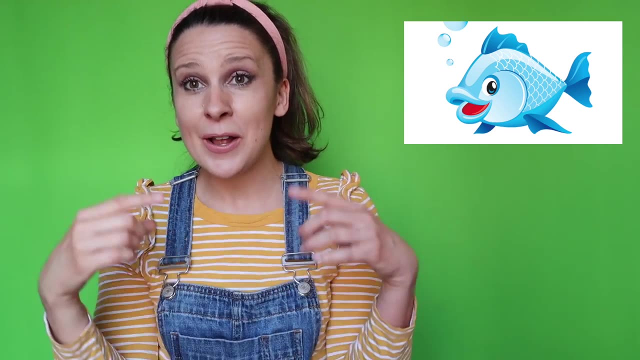 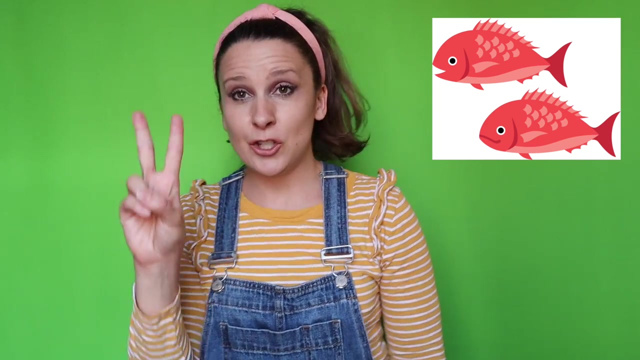 One little blue fish swimming in the water. One little blue fish swimming in the water. One little blue fish swimming in the water. Bubble bubble, bubble, bubble pop. That was fun. Let's get out two little red fish. Two little red fish swimming in the water. 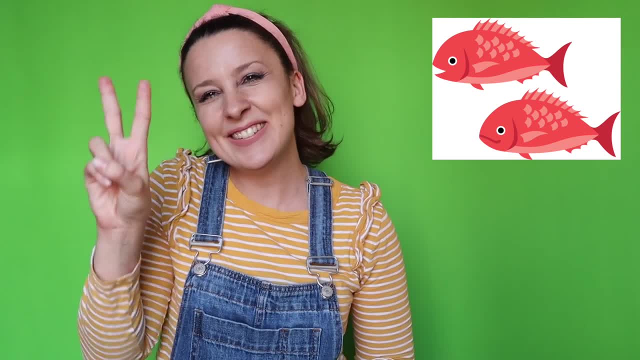 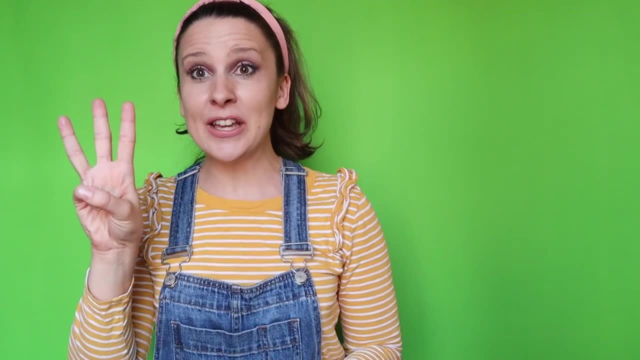 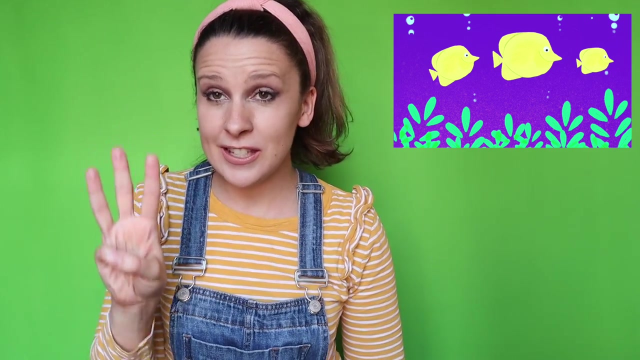 Two little red fish swimming in the water. Two little red fish swimming in the water. Bubble, bubble, bubble, bubble pop. Wow, Let's get three yellow fish. Three little yellow fish swimming in the water. Three little yellow fish swimming in the water. 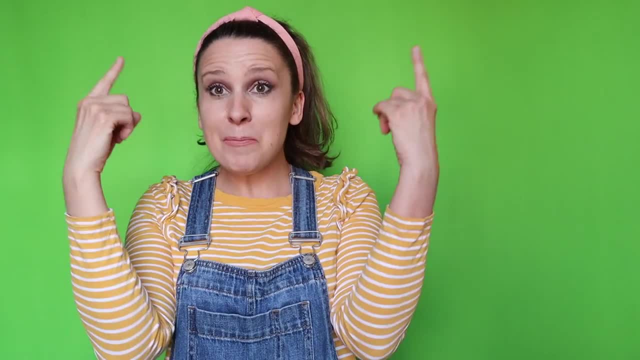 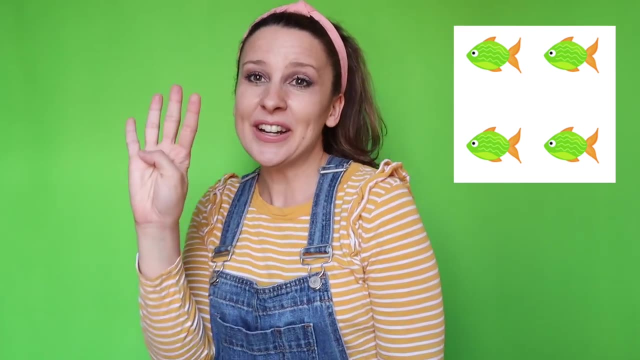 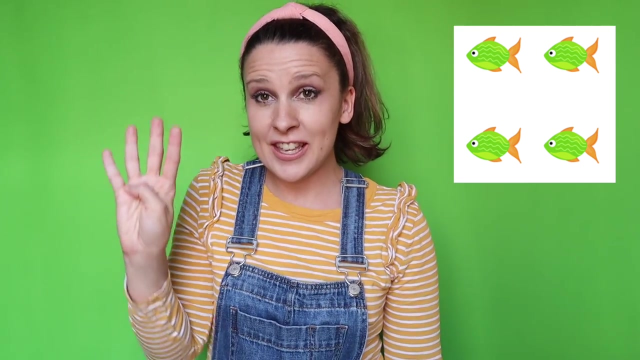 Three little yellow fish swimming in the water. Bubble bubble, bubble, bubble pop. How about four green fish? I'm excited. Four little green fish swimming in the water. Four little green fish swimming in the water. Four little green fish swimming in the water. 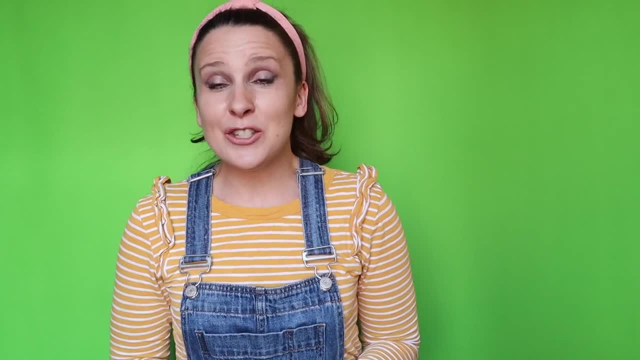 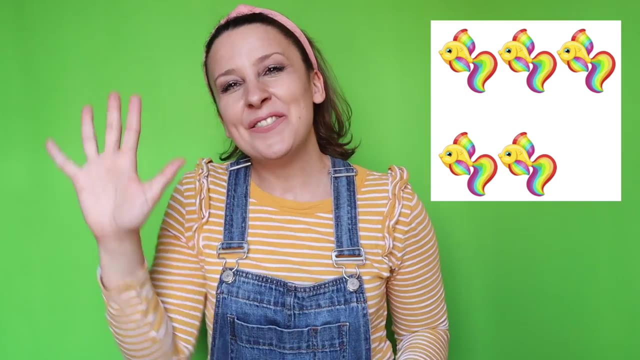 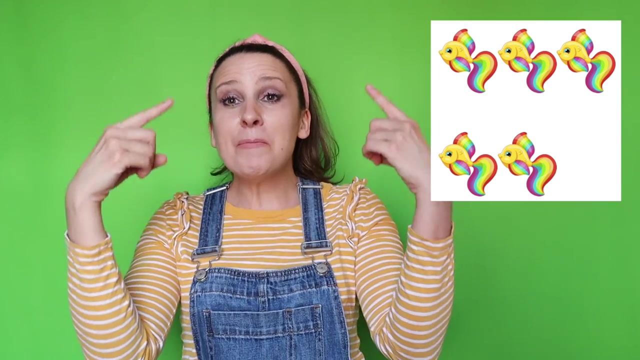 Bubble, bubble, bubble, bubble pop. Now let's do five rainbow fish. Five little rainbow fish swimming in the water. Five little rainbow fish swimming in the water. Five little rainbow fish swimming in the water. Bubble, bubble, bubble, bubble pop. 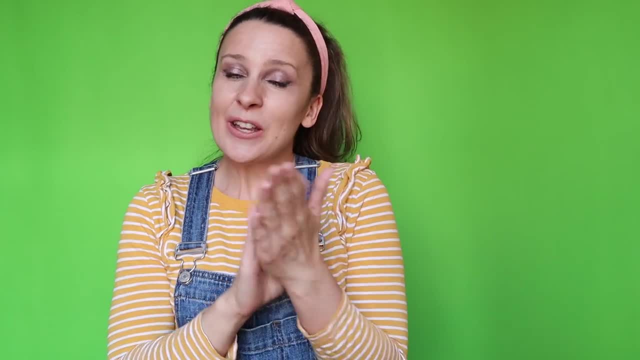 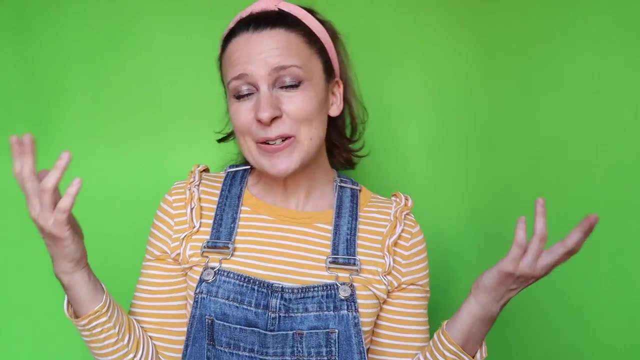 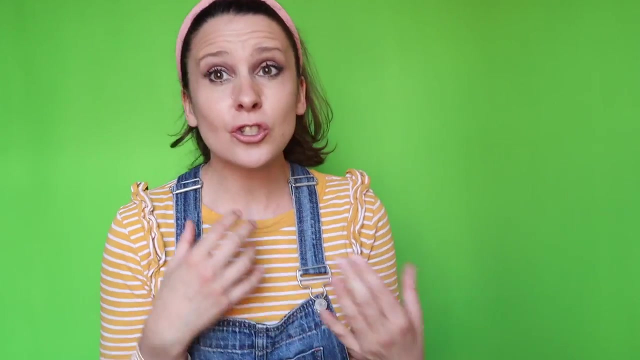 Wow, Great job. What color fish would you like to do? You could even do something like a Spiderman fish, or a Batman fish, or an Elsa fish, or an Anna fish, Or a really sparkly striped polka dot fish. I'd love to hear what you chose. 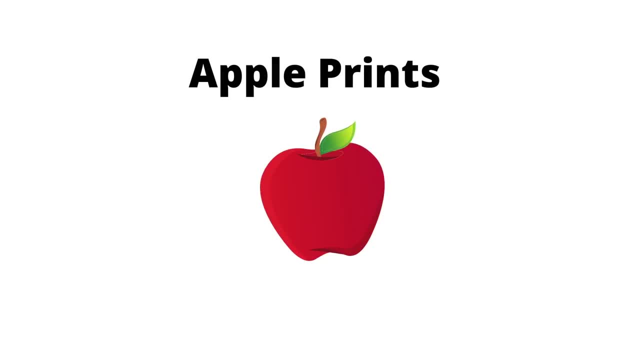 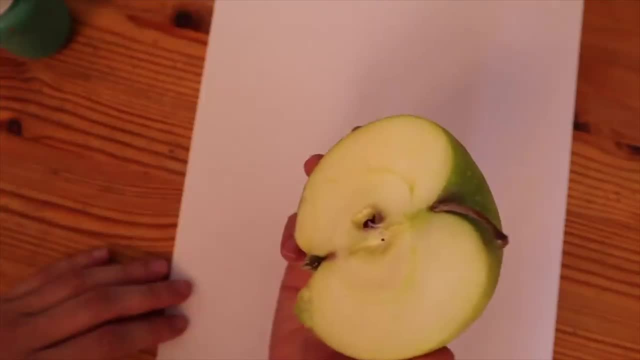 Great job. So we take an apple and you have a grown up help. you cut it in half And then we're going to make a print, So we're going to dip it in paint. Did you know? some apples are yellow, So I dip this in yellow paint. 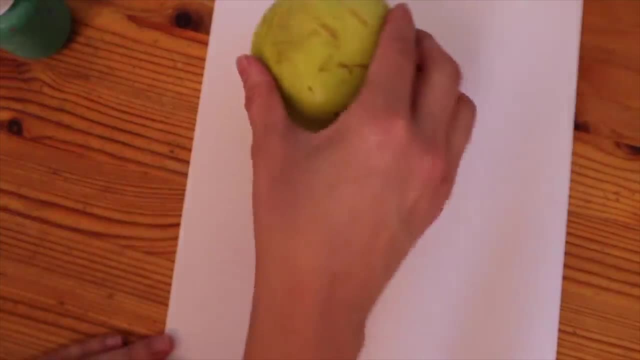 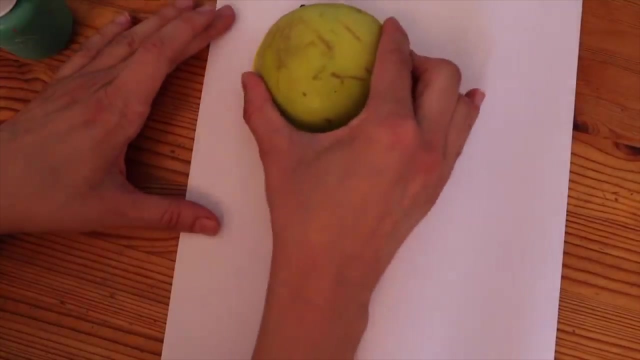 Now I'm going to stamp it on. Can you say: stamp, Stamp. Let's see how it looks. I'm so excited. Oh, it looks pretty. I like it. Maybe I should hold it down a little longer and push. Wow, that looks good. 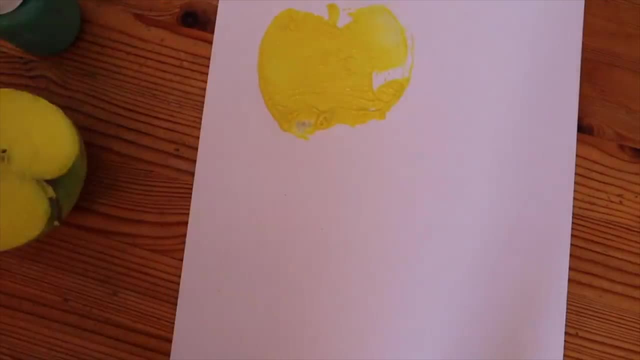 I even see the stem. I'm going to try another color paint. What's the color of the day, Do you remember? Yeah, it's red, Good job. Next, I'm going to dip it in red paint. Wow, I dipped it in red paint. 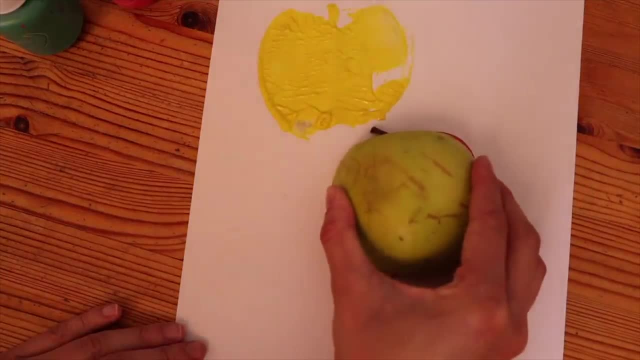 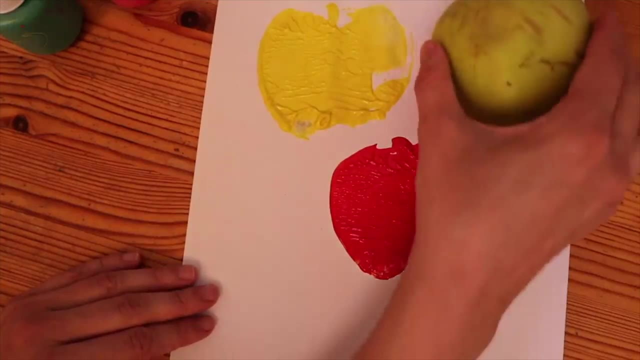 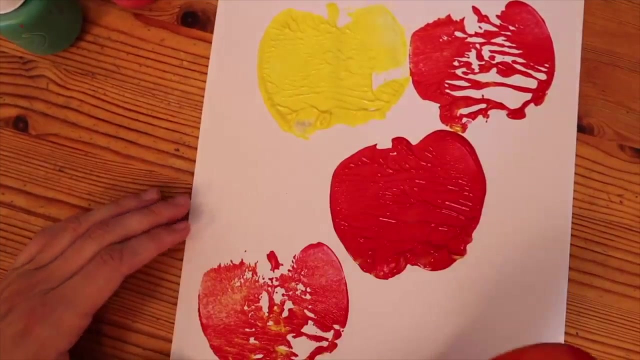 Now let's stamp it. Say stamp, Stamp, Let's see what happens. Push Pretty, Oh, my goodness, I love it. Do another one. Ooh, that one has a lot of spaces, but I like how it looks Wow. 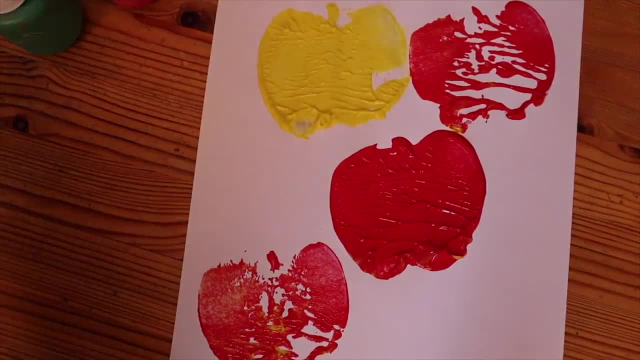 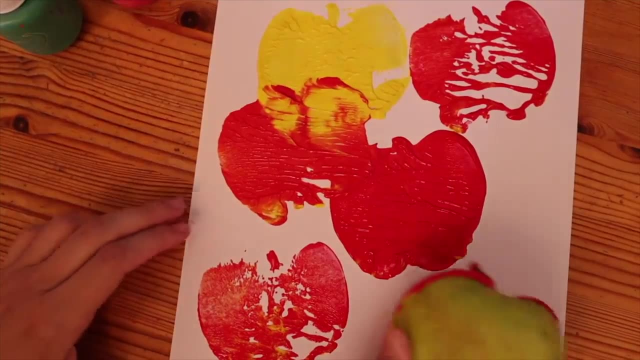 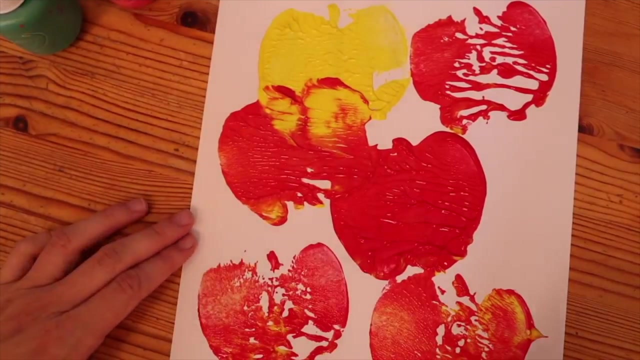 I'm going to mix the yellow and the red together a little bit. Wow, I like printing them on top of each other. It looks nice. I even see the seed prints a little bit. That's so cool. I really like my picture. 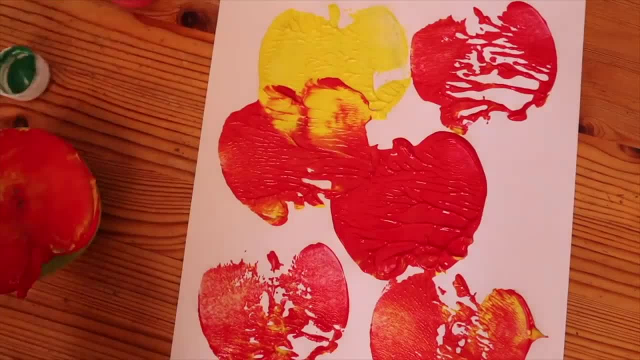 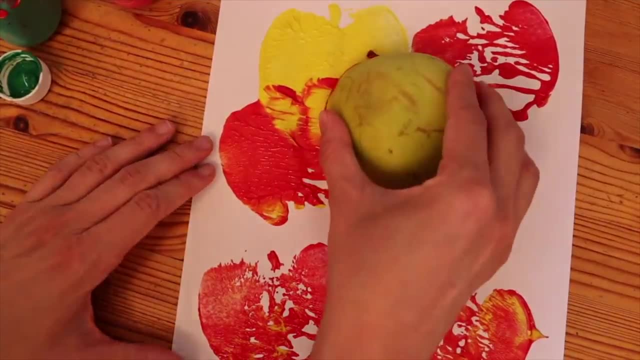 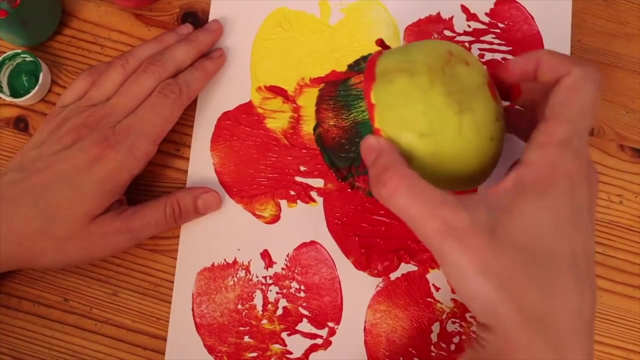 You know, we learned also that apples can be green, So I'm going to try green and see how that looks. Let's see how the green looks. I dipped it in green paint Push Printing with apples. Whoa, Whoa, it's pretty messy. 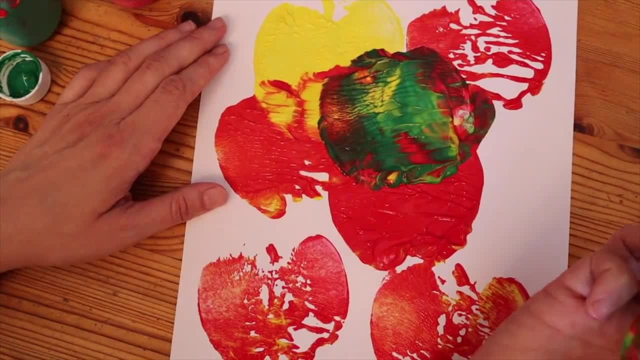 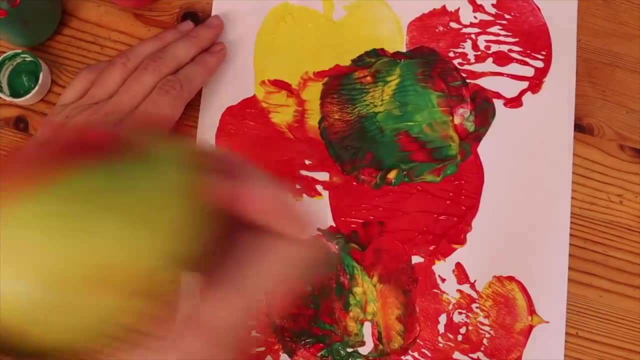 That's okay, I can wash my hands after That. one looks like a lot of colors. I like it. Push again. Oh, it's slippery. We did it. We made the apple print picture. I'm proud of myself and I'm proud of you. 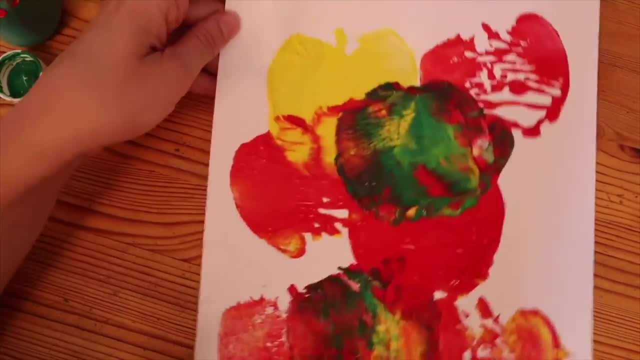 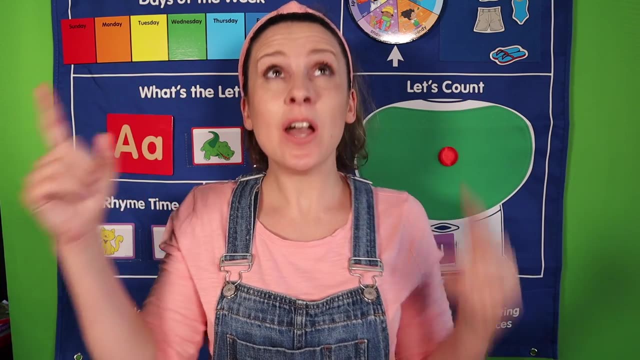 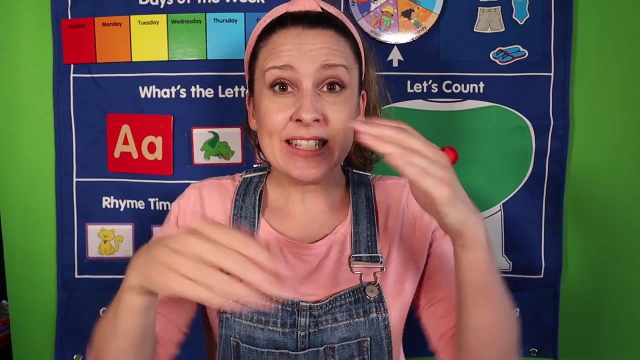 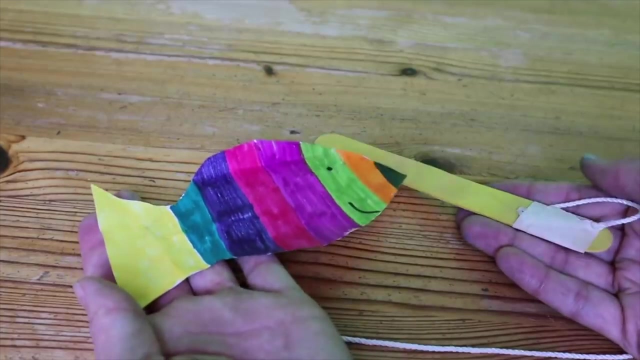 It always feels good to make something. Are you ready? Way up high in the tree, One red apple smiled down at me, So I shook that tree as hard as I could. Down came the apple: Mm-mm. good, Great job. It's time for art class. 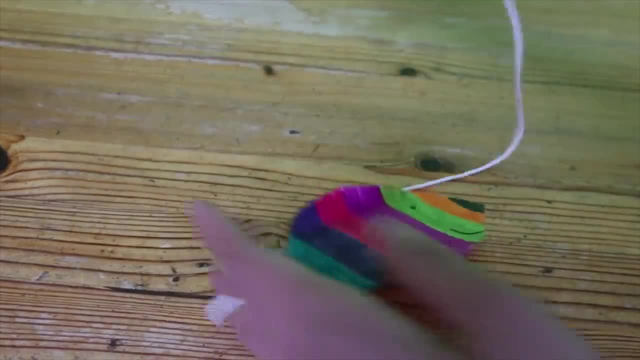 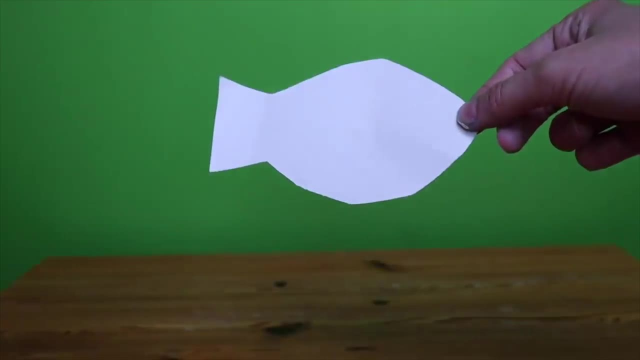 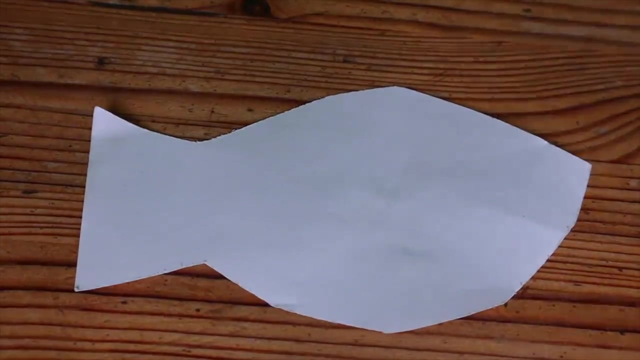 Today we're going to make a fish on a pretend fishing pole. Yeah, The first thing you do is cut a fish out of paper. Have a grown-up help you with the scissors. Now we get to decorate the fish. How would you decorate your fish? 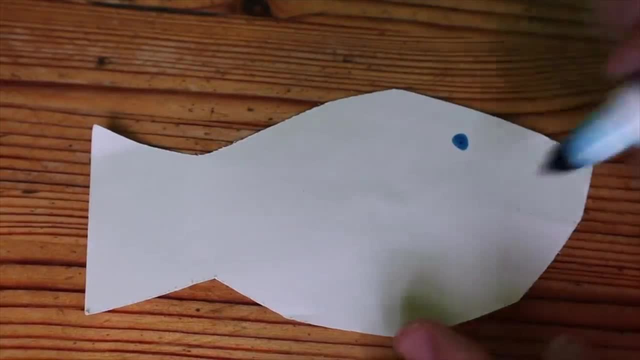 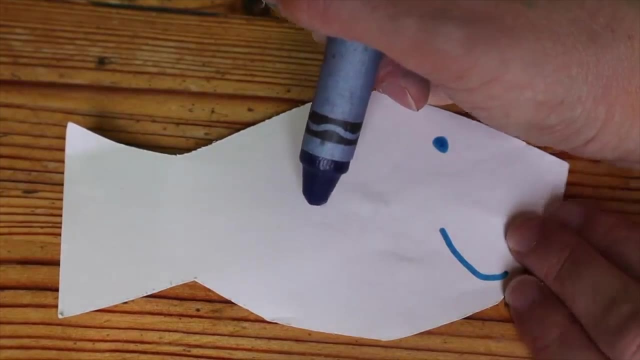 I like to put a little eye and then a smile. Happy fish. Since the color of the day is blue, I'm going to use a blue crayon. I think I'll color this fish with blue triangles, The shape of the day. 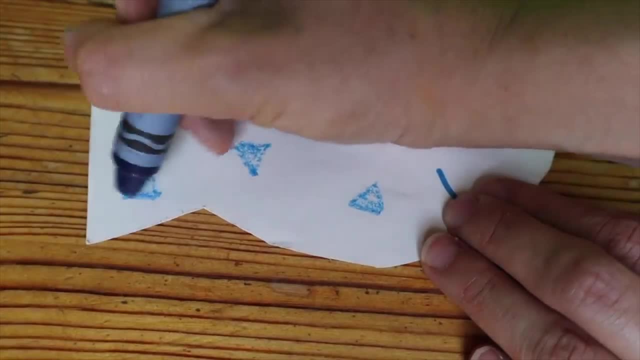 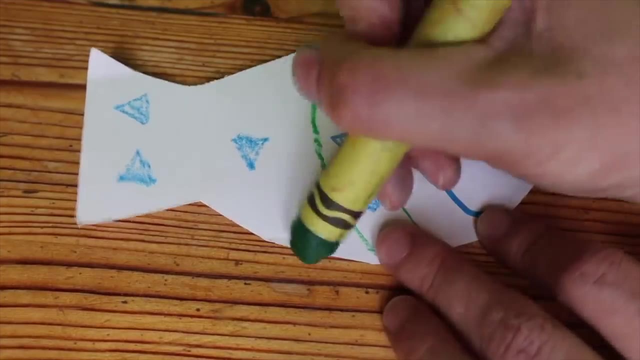 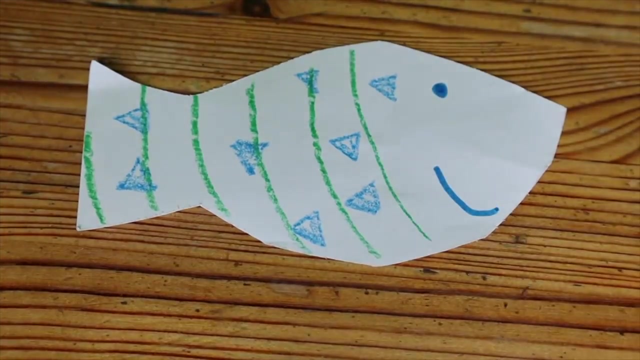 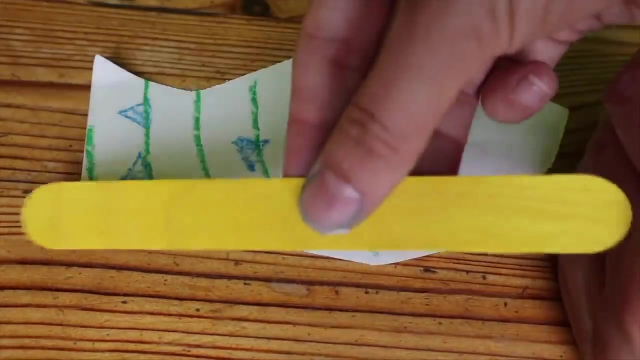 So fun I like decorating the fish. Now I'm going to add some green, Green stripes. What are you putting on your fish? Next? we take a piece of string and we're going to tape it to a popsicle stick. Get out a piece of tape. 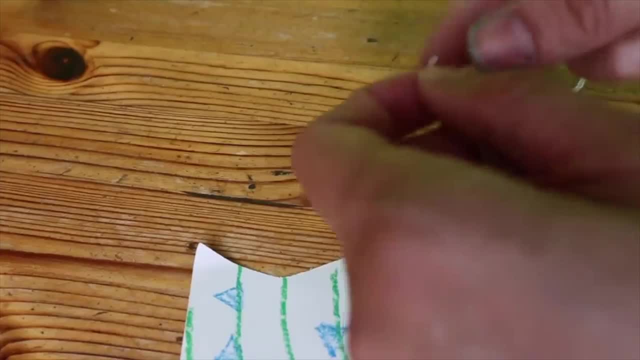 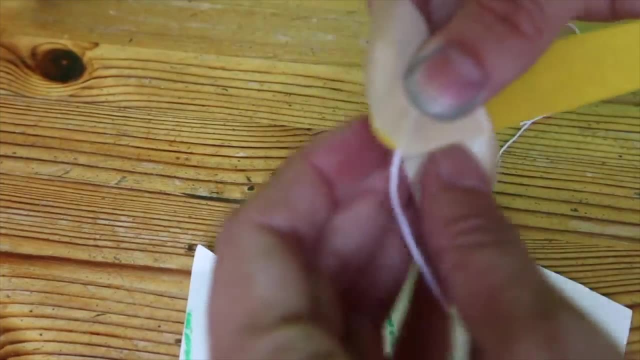 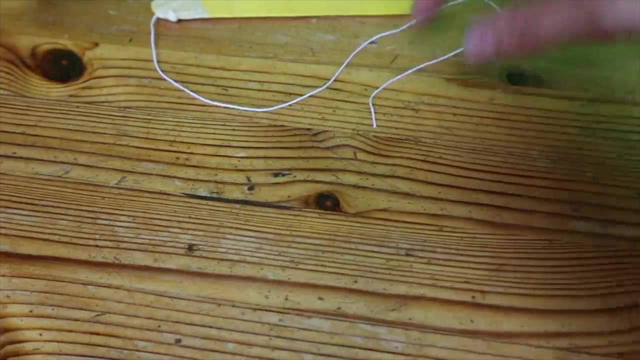 This is called masking tape, And I'm going to tape the string to the popsicle stick. Tape it, Tape it, Tape it on. Now I'm going to put some tape on this side and tape the fish. Okay, let's put some tape. 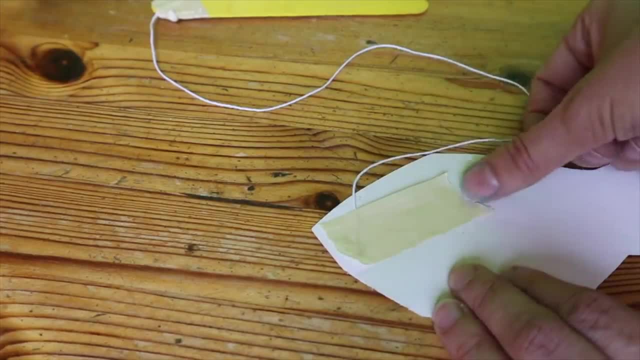 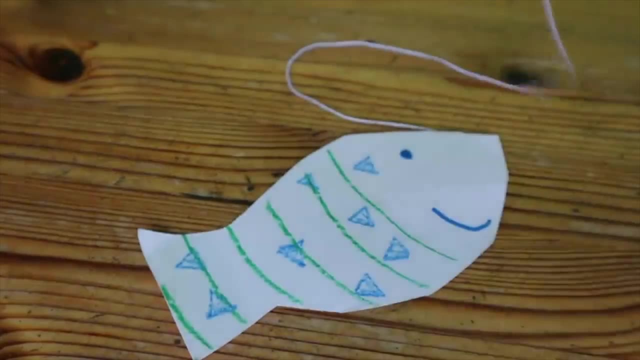 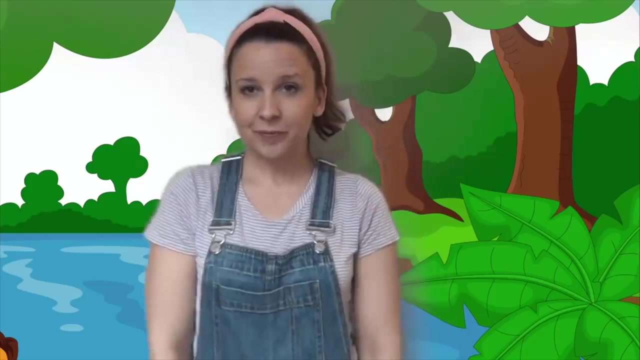 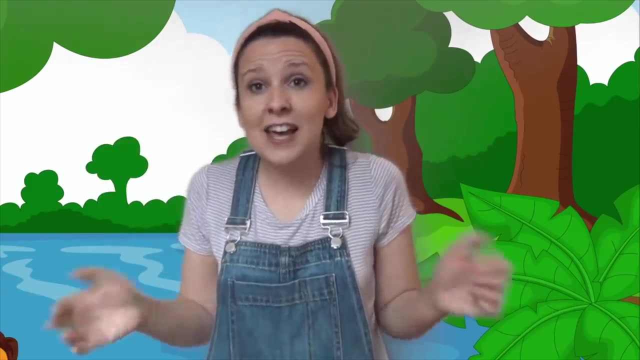 on the fish. Yay, We put it on And now the fish is on a fishing pole. We did it, We made a fishing pole and a fish. Awesome. One, two, three, four, five. Once I caught a fish alive. 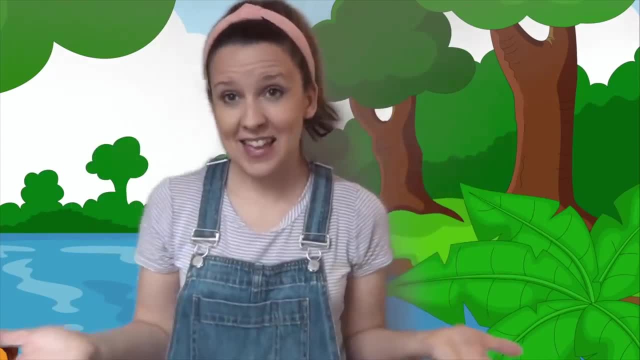 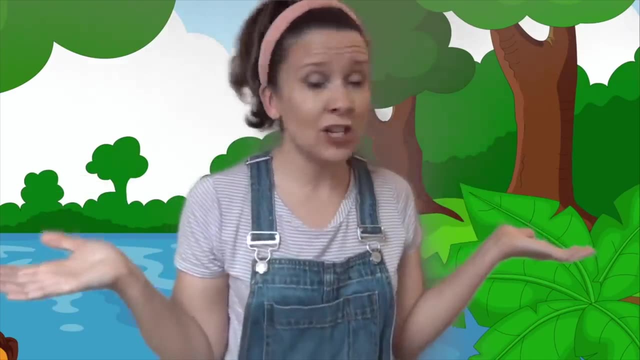 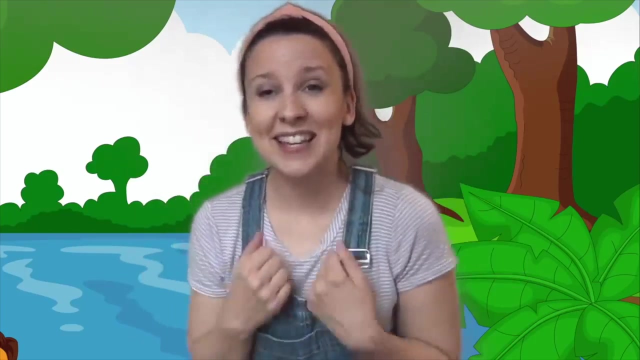 Six, seven, eight, nine, ten. Then I let it go again. Why did you let it go? Because it bit my finger. so Which finger did it bite This little finger on my right? Let's sing it again. Let me hear you sing in your nice loud voice. 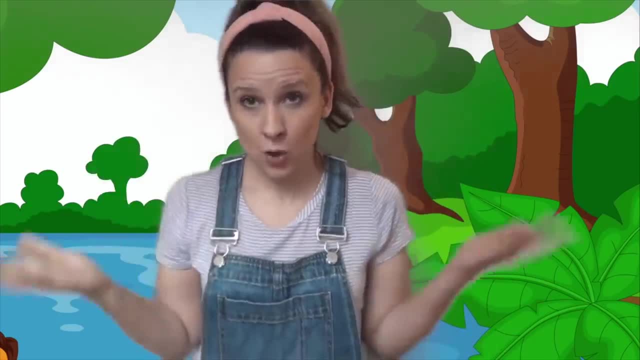 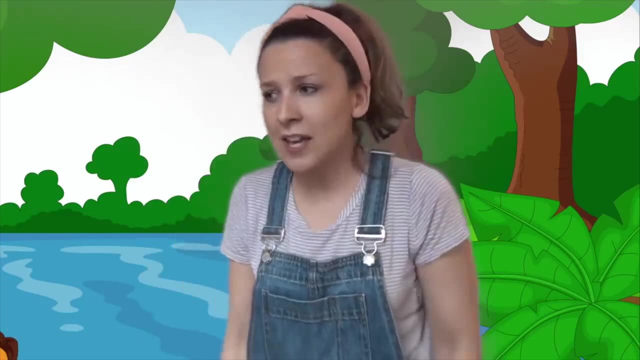 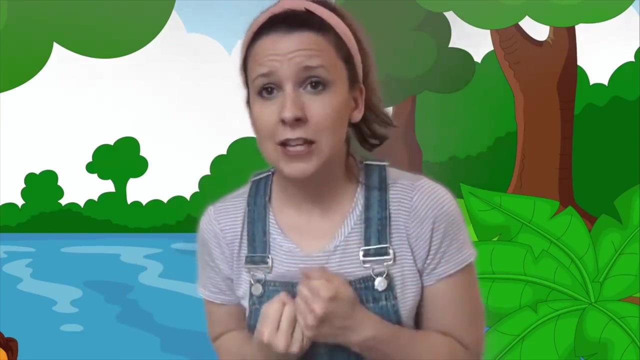 One, two, three, four, five, Once I caught a fish alive- Six, seven, eight, nine, ten. Then I let it go again. Why did you let it go? Because it bit my finger. so Which finger did it bite? 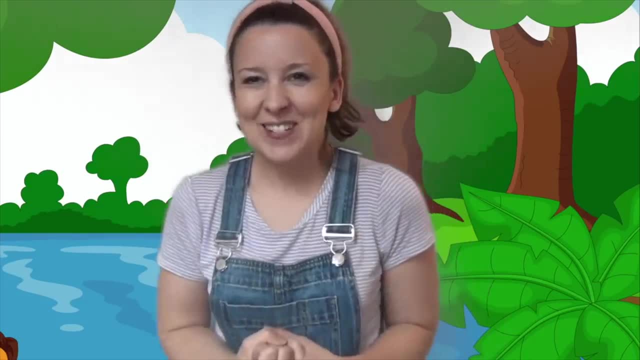 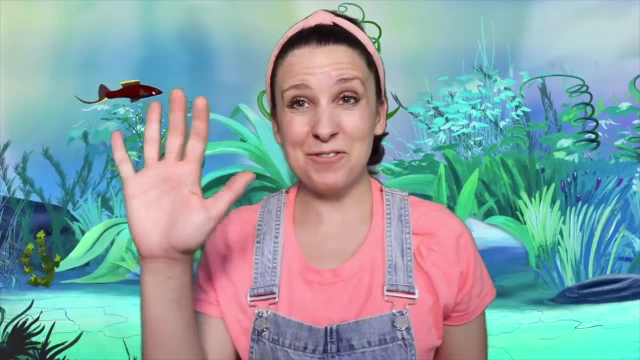 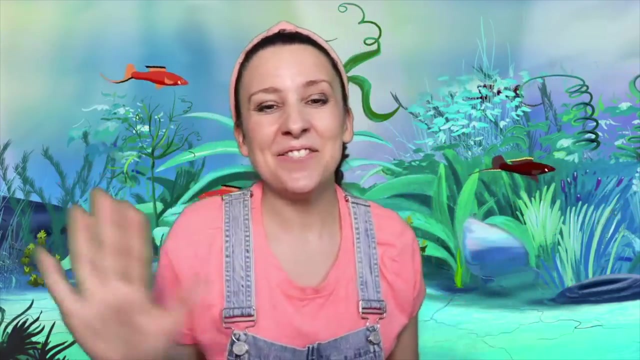 This little finger on my right. Great job. Let's put a band-aid on our finger. Let's pretend Now it feels better. Can you get out five little fishies? Good job, Five little fishies swimming in the sea. 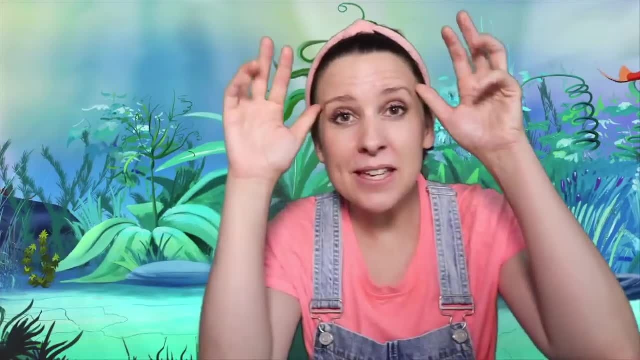 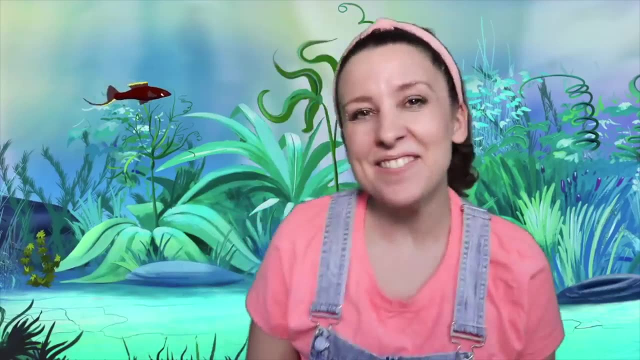 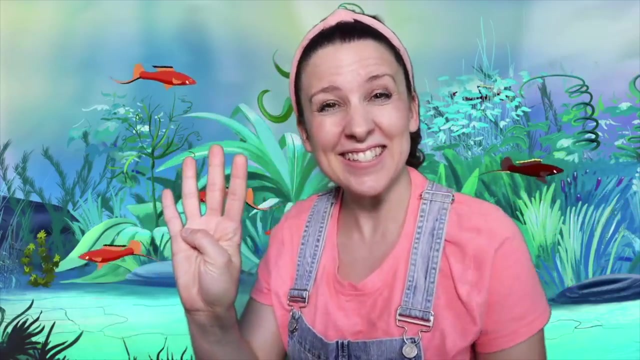 Teasing, Mr Sharky can't catch me. Along comes, Mr Sharky, quiet as can be, And snuck that fishy right out of the sea. How many are left? One, two, three, four. Good counting. 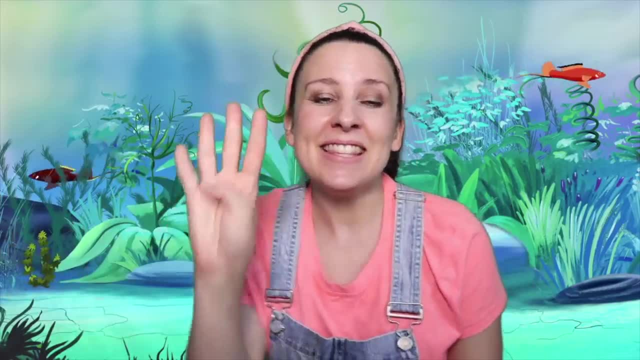 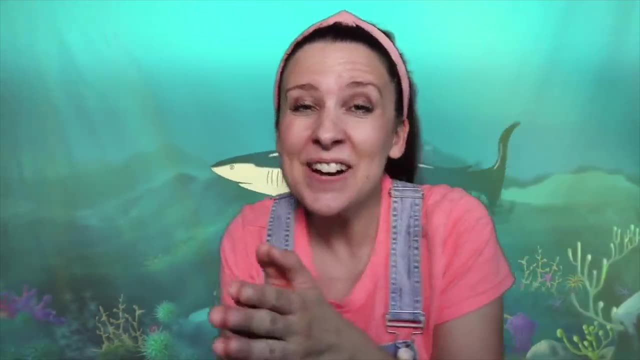 Four little fishies swimming in the sea, Teasing. Mr Sharky can't catch me Along. comes Mr Sharky, quiet as can be, And snuck that fishy right out of the sea. How many are left? Count with me. 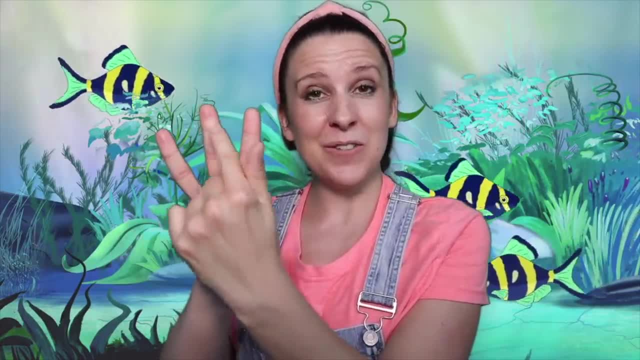 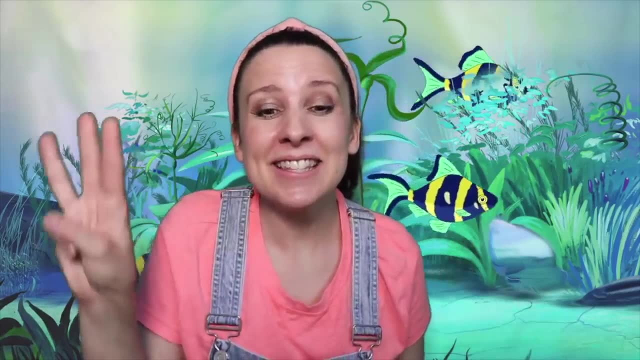 One, two, three. Good job, Three little fishies swimming in the sea Teasing- Mr Sharky can't catch me Along. comes Mr Sharky, quiet as can be, And snuck that fishy right out of the sea. 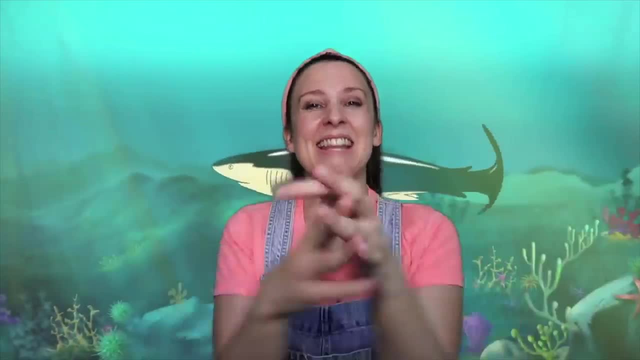 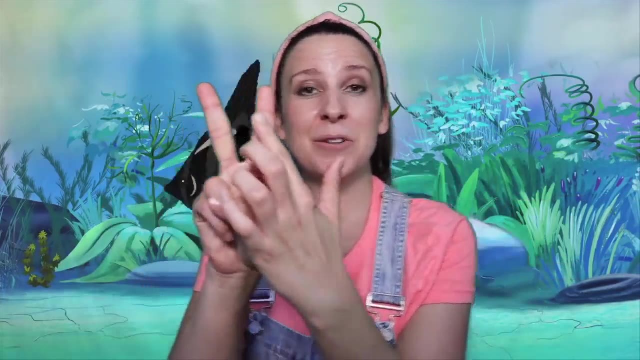 How many are left? One, two, three, four, Two little fishies swimming in the sea Teasing- Mr Sharky can't catch me Along. comes Mr Sharky, quiet as can be, And snuck that fishy right out of the sea. 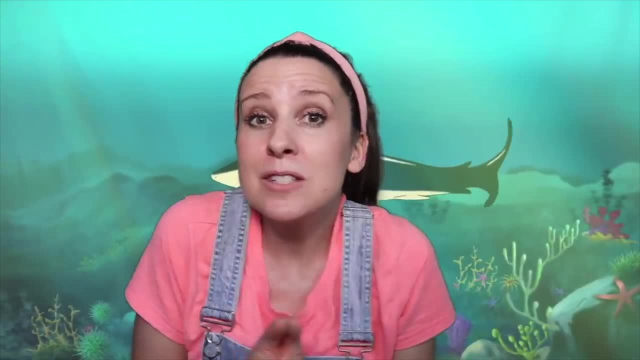 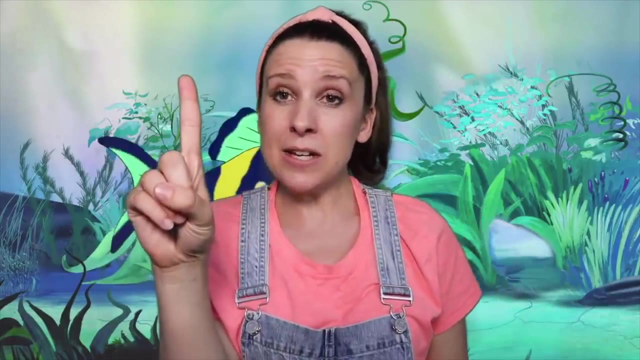 How many are left? One, two, three, four, Two little fishies swimming in the sea Teasing- Mr Sharky can't catch me Along. comes Mr Sharky, quiet as can be, And snuck that fishy right out of the sea. 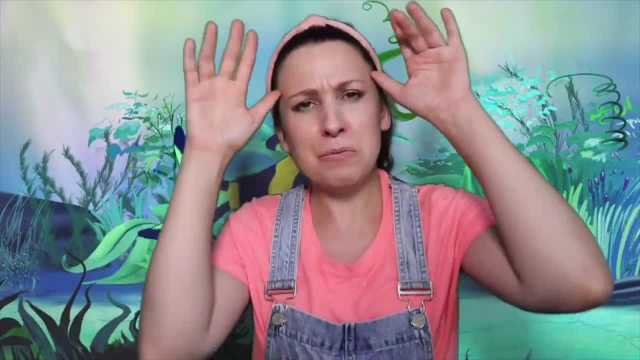 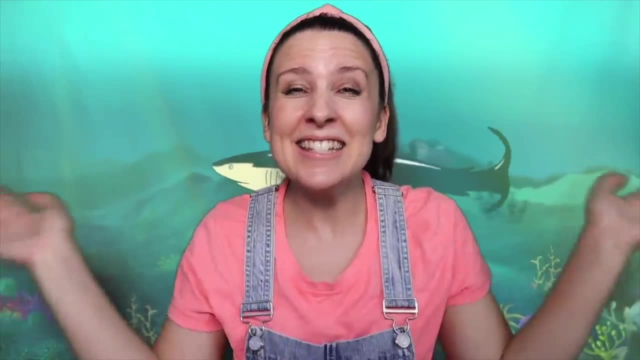 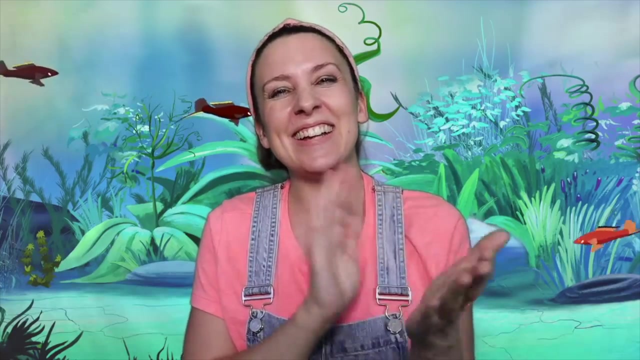 One little fishies swimming in the sea, Teasing Mr Sharky can't catch me Along. comes Mr Sharky, quiet as can be, And snuck that fishy right out of the sea. That was so good. Great job, friends. 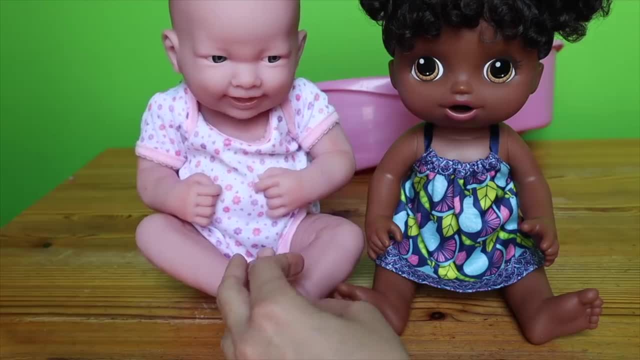 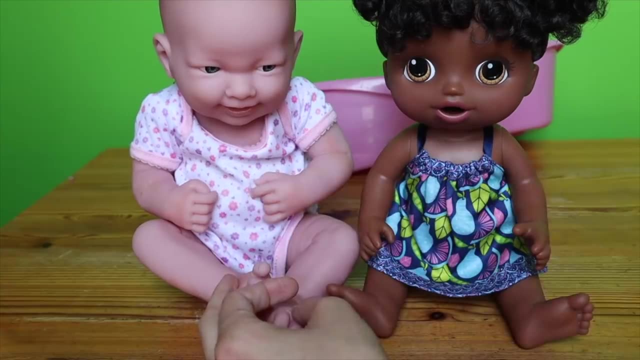 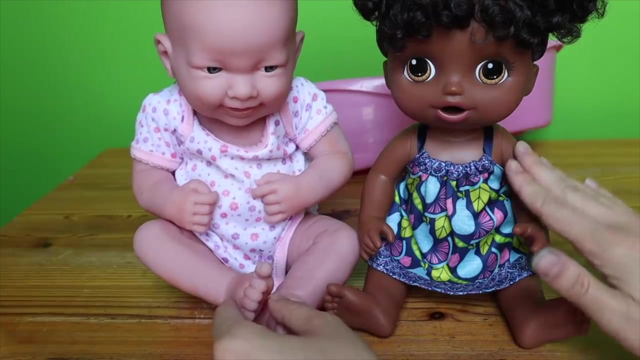 Hey friends, It's time for Show and Tell. I would like to show two babies. Let's count them. One, two, Two baby dolls. B-b-baby begins with B. This baby is hungry, So we're going to feed this baby. 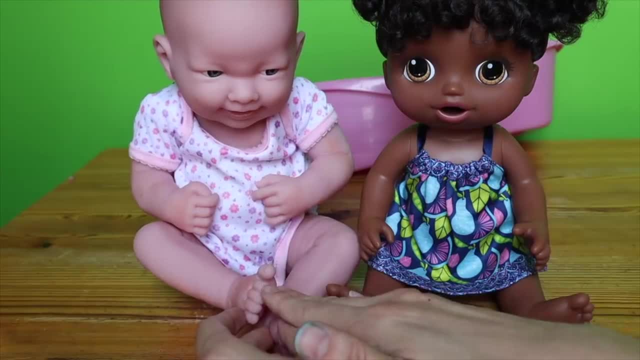 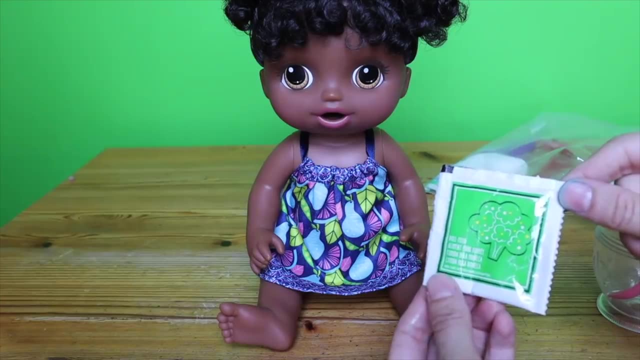 This baby needs a bath. So we're going to give this baby a bath. Are you ready? Yay, We're going to give this baby some b-b-broccoli. Broccoli starts with B, Which is our letter of the day. 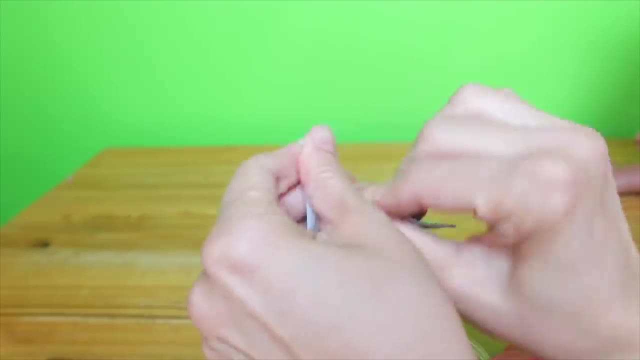 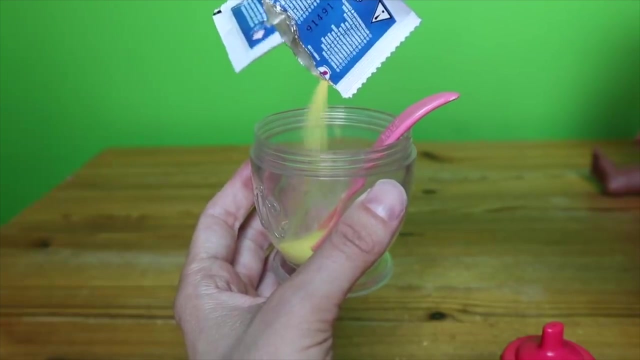 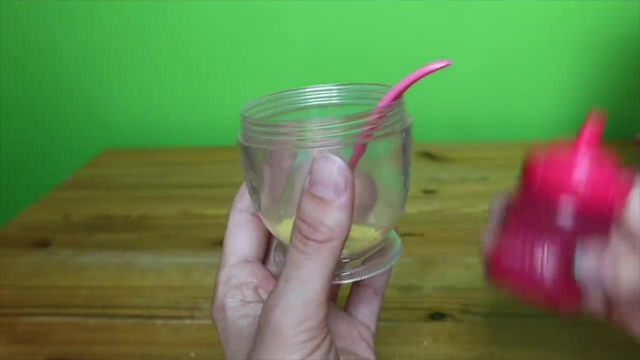 Yeah, So we open the broccoli Open And we're going to pour it into her little bowl. Pour This is pouring, Can you say? pour Help me, pour Pour Good job. Now we're going to add some water from her bottle to her bowl. 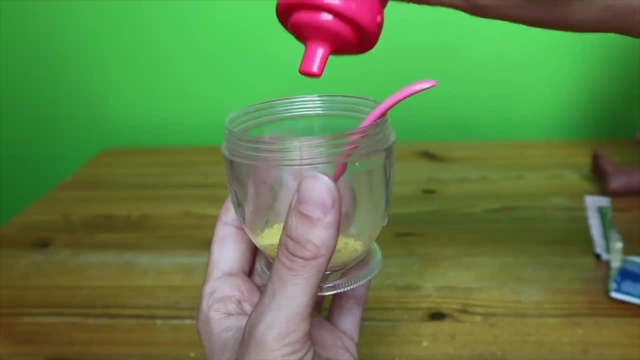 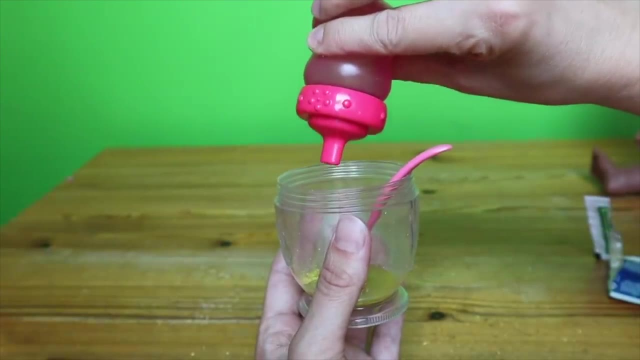 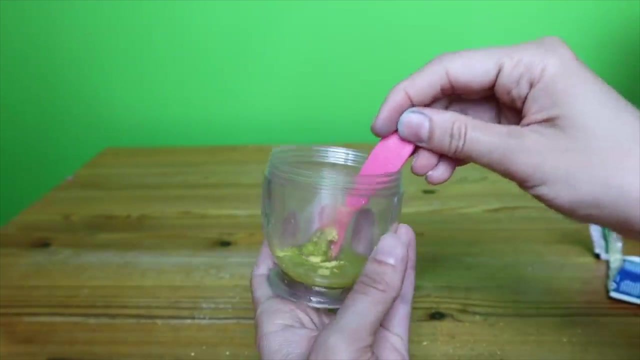 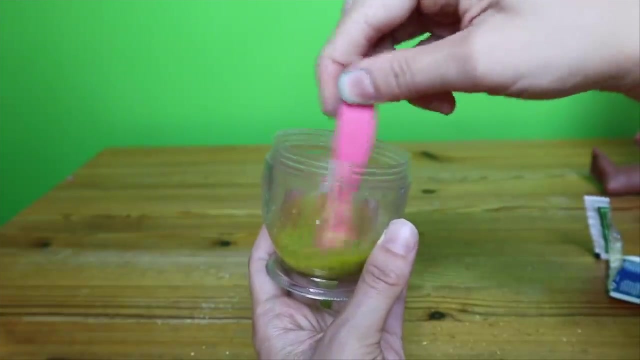 So we pour some water in, We have to squeeze this, Say squeeze, Squeeze, Squeeze the water Squeeze Squeeze. Now, what do we do with this spoon? We mix, We mix up her food, Mixing food. 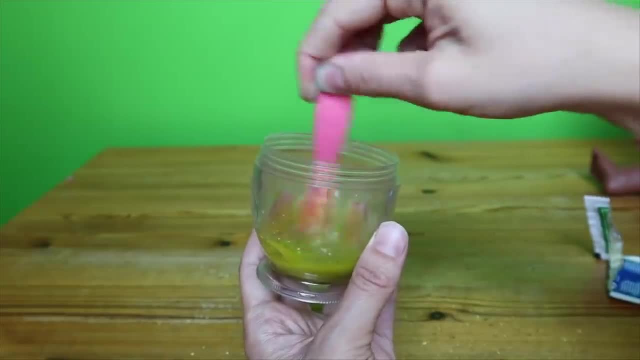 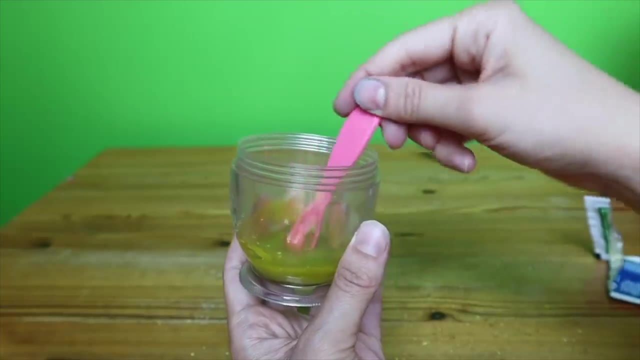 Mixing food: Mix, mix, mix. This is the way we mix the food. Mix the food, Mix the food. This is the way we mix the food for the baby. Okay, baby, we have your food. You're having bro-bro-broccoli. 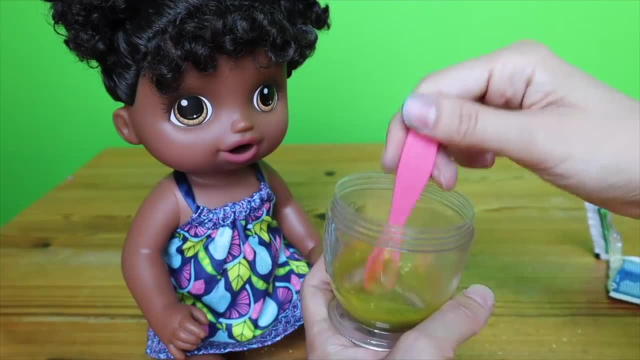 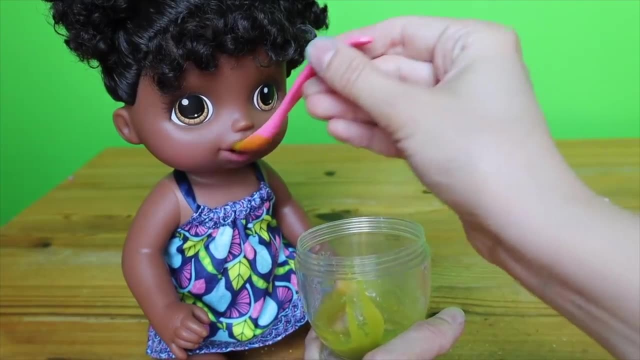 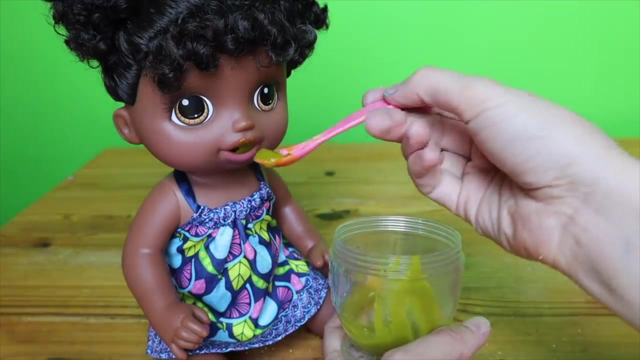 Which begins with B. Can you say eat? You say eat and I'll feed the baby Eat. Oh, she's eating. She likes the food. You say: eat and I'll feed her more Eat. She likes it. She likes it. 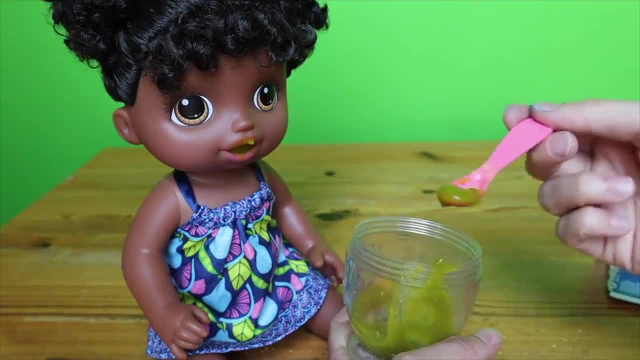 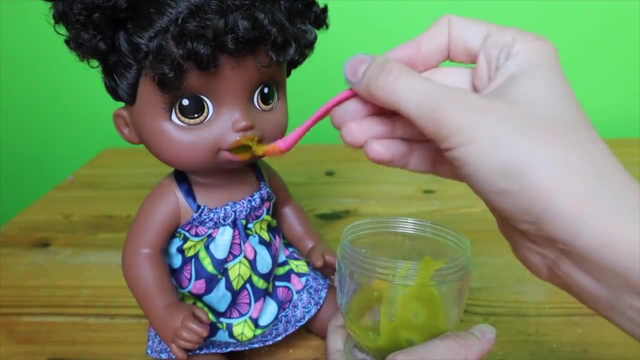 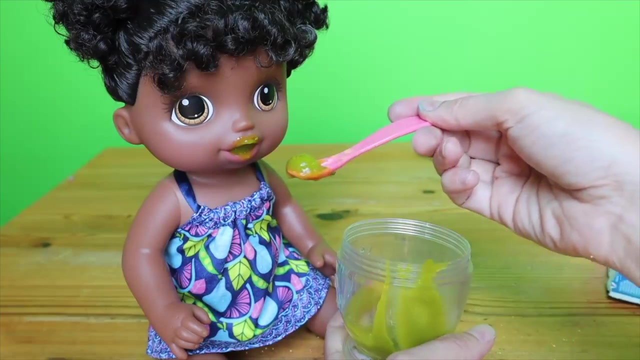 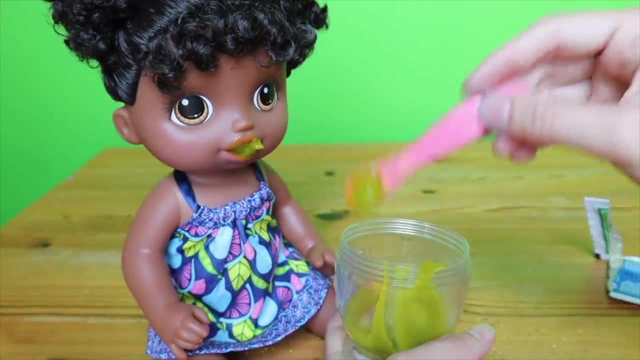 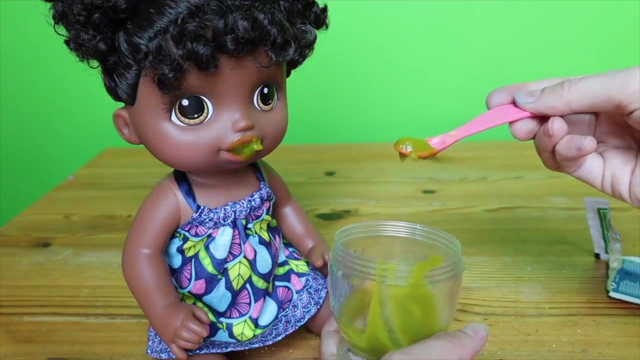 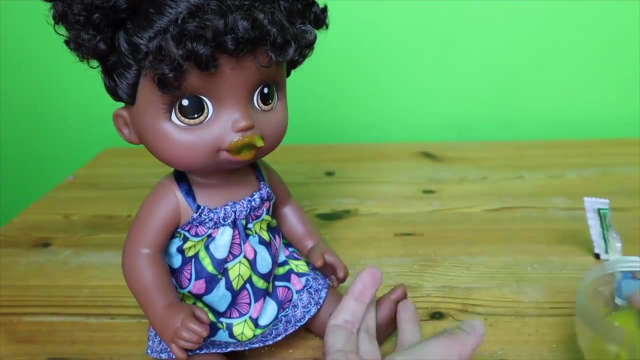 Say: eat, Eat. Good job, baby, Good job. Thank you for helping me feed the baby Eat. That's a big bite, baby. Good job. The baby is eating. Feeding baby, Feeding baby food Eat. Wow, I think the baby is all done. All done, All done, broccoli, All done. 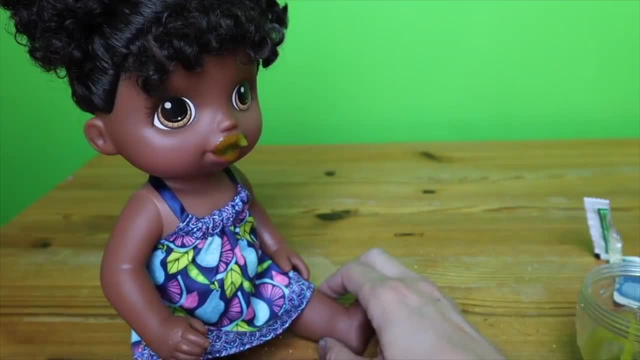 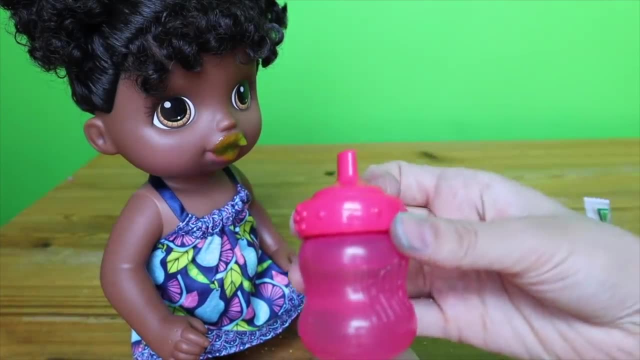 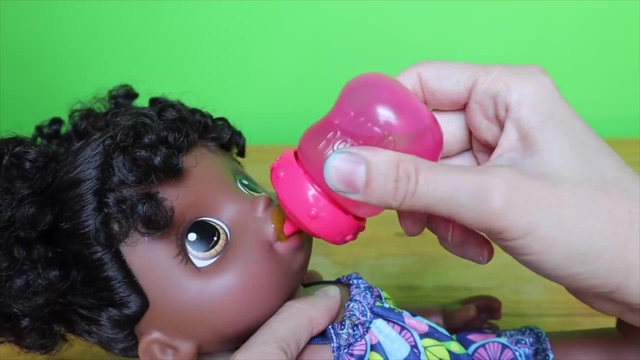 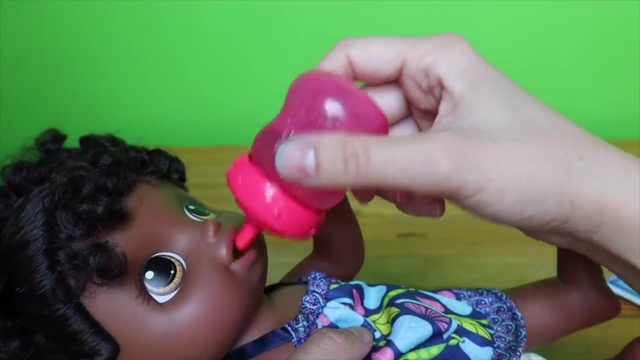 All done, All done. I hear her saying: all done, Good job, baby. Now let's give her this. What is this called Water? Let's help the baby take a drink of water. Aw, the baby is drinking her water. The baby is drinking. The baby had some broccoli and 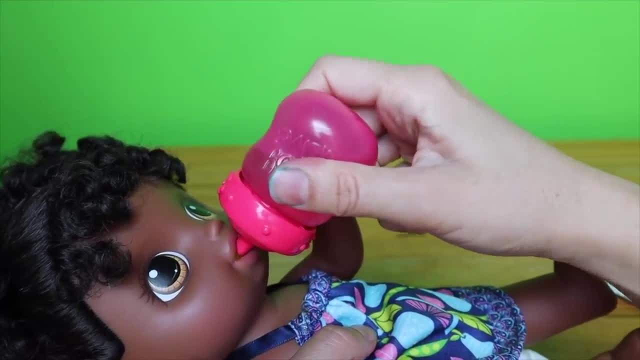 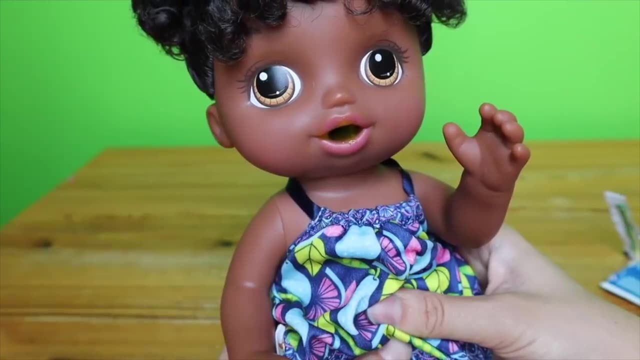 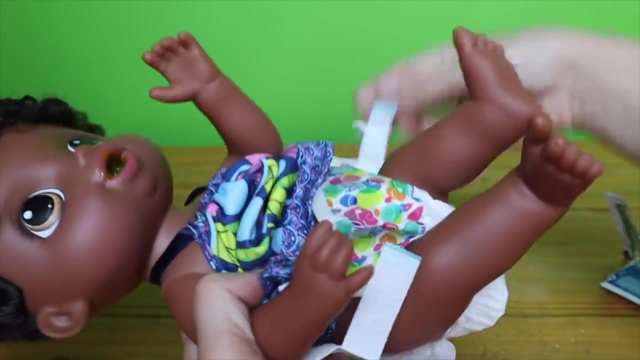 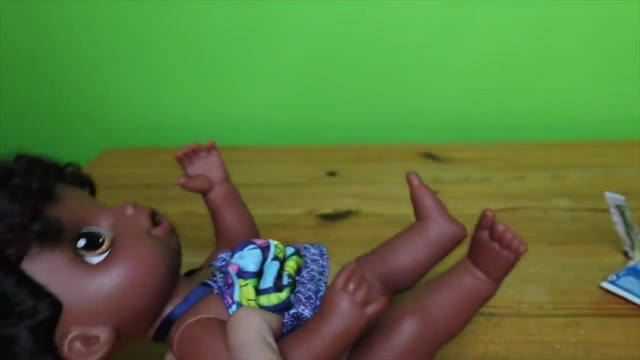 now she's having some water. I think we'll have to change her diaper soon. The baby's all done water. Uh-oh, We have to change the baby's diaper. So we pull these and we change the baby's diaper. Oh, she did a poo-poo. Gotta get a nice, clean diaper for the baby. Okay, let's put on the nice. 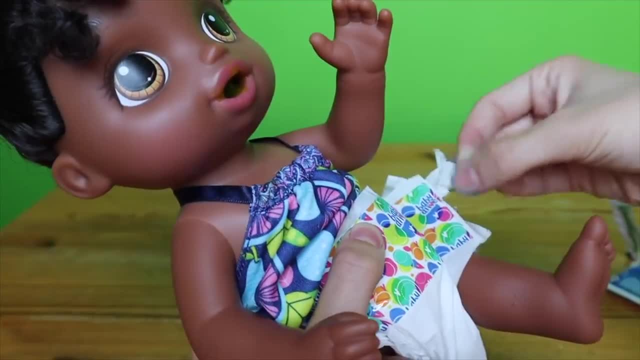 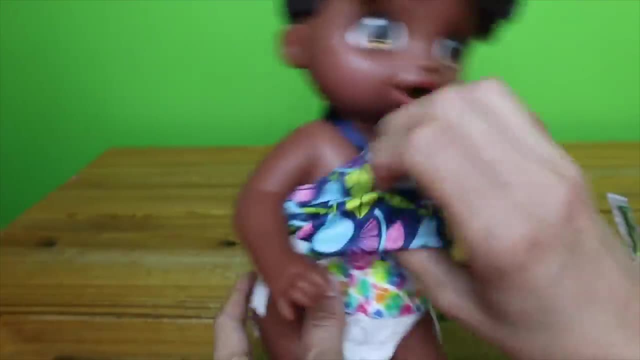 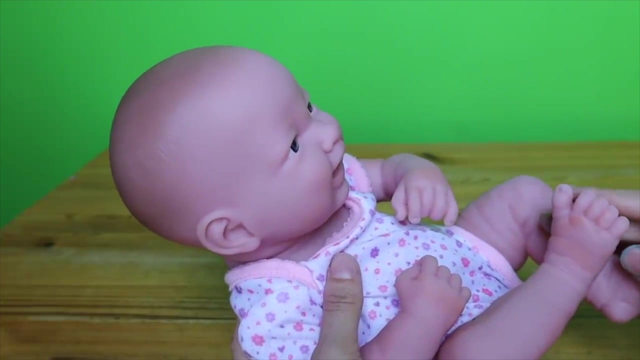 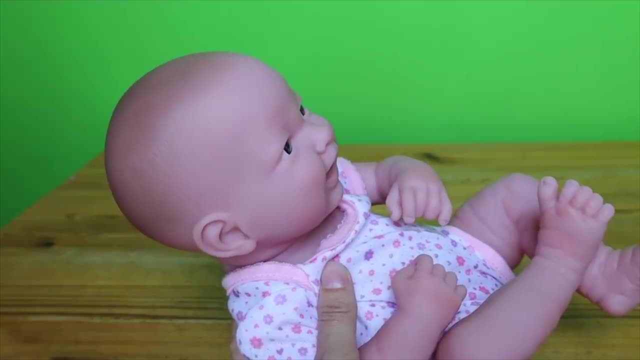 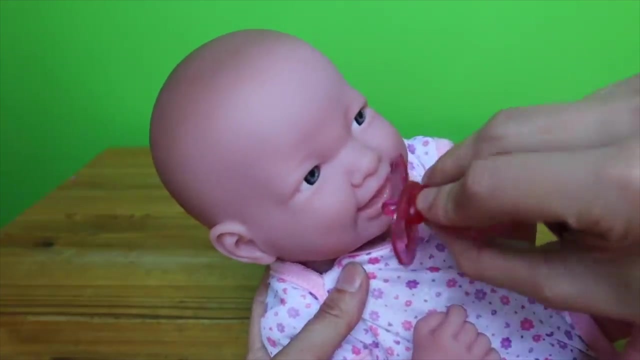 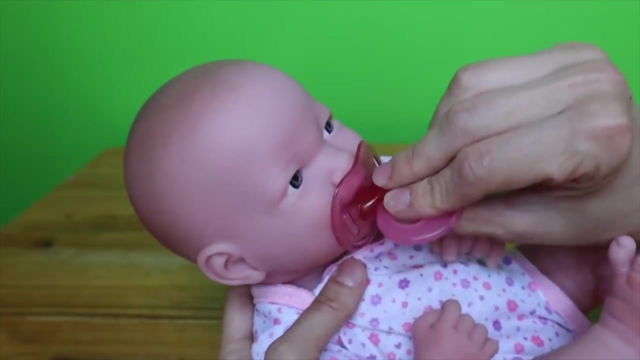 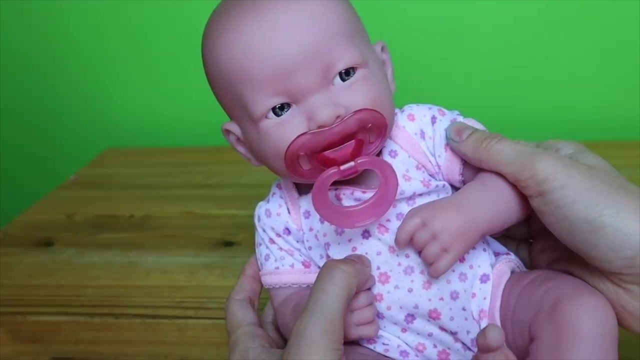 Let's give the baby a pacifier. She's a little baby, so she still uses a pacifier. Put it in, Put it in. Put it in. Wah, Wah, Wah, Wah In. She stopped crying. She is happy with her pacifier. Good job. 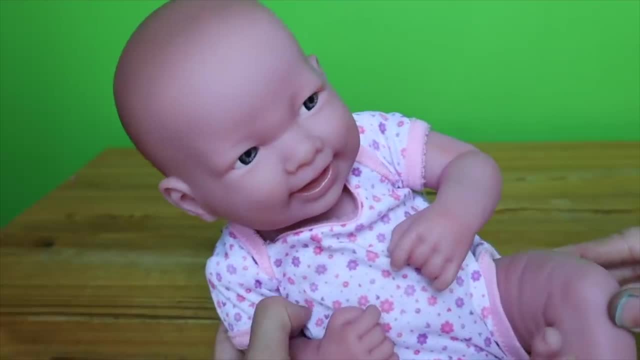 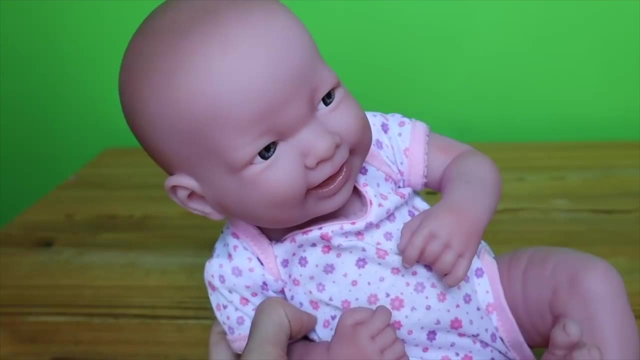 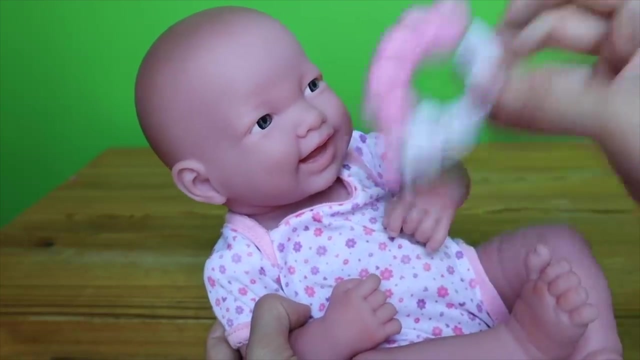 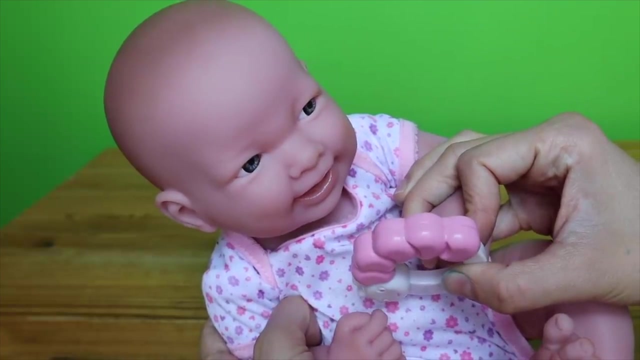 You helped the baby stop crying. Wah, Wah, Wah. She's crying again. Hmm, What should we do? Let's give her a toy. Can you say toy, Toy, Toy, Wah, Wah, Wah. Give baby toy. Oh, she has the toy and she stopped crying. Good job. 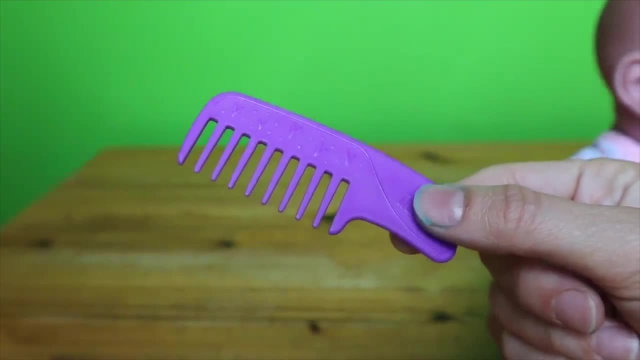 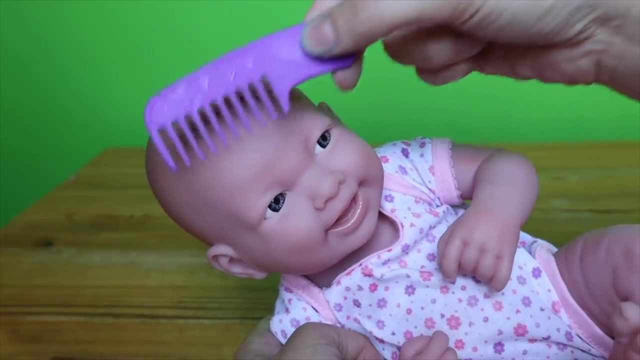 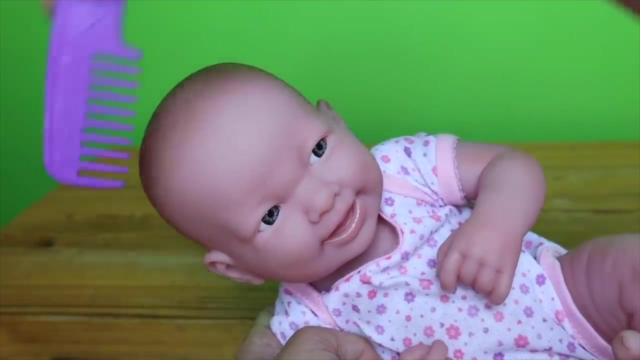 What is it? What's this? It's a comb. Can you help me comb the baby's hair? Say comb, Say comb, Comb. Good job, We're combing the baby's hair. We're combing the baby's hair. 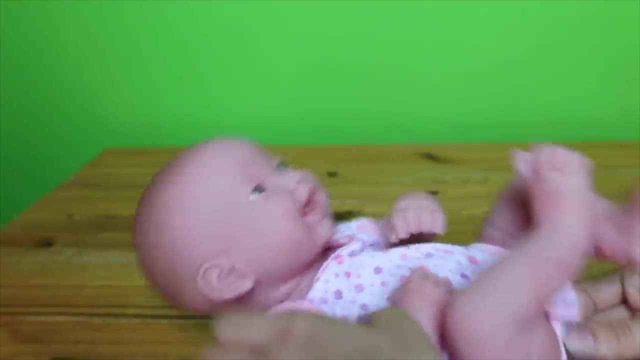 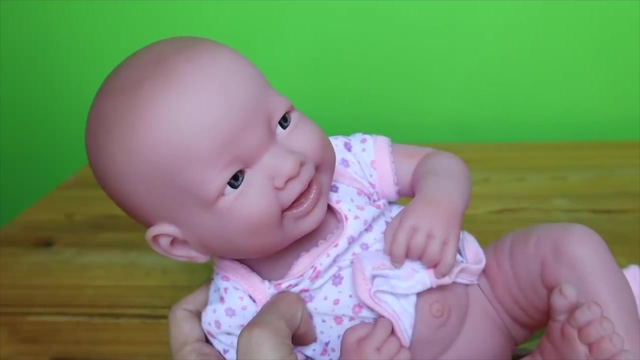 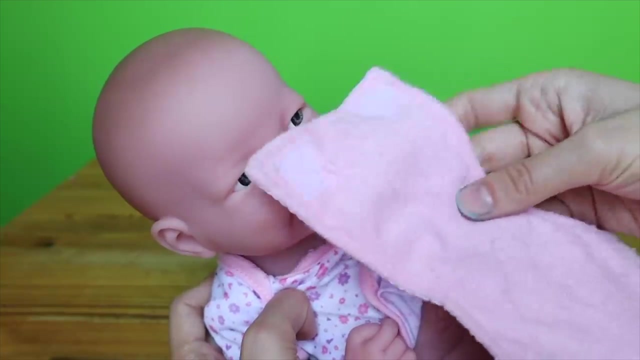 We're making the baby look so nice. We're combing the baby's hair. Good job, Wah, Wah, Oh. no, The baby is crying again Uh-oh. Can you say uh-oh, Uh-oh, Hmm, how about we try? 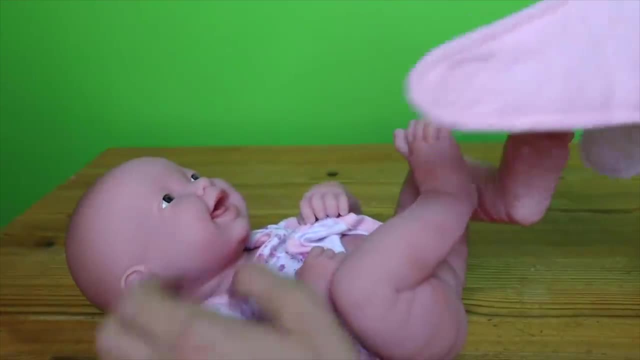 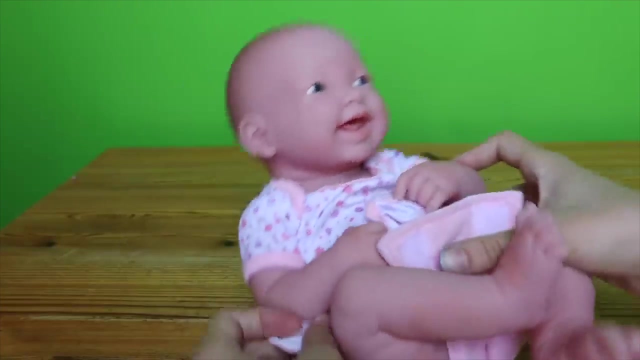 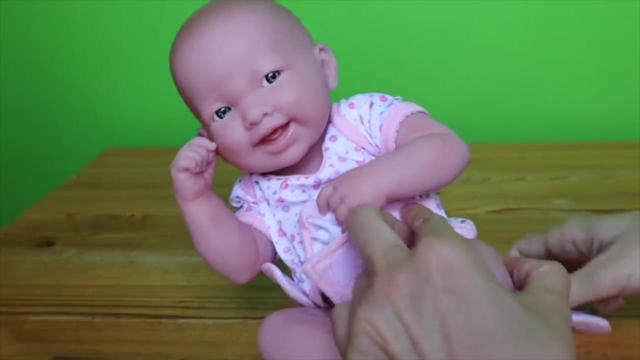 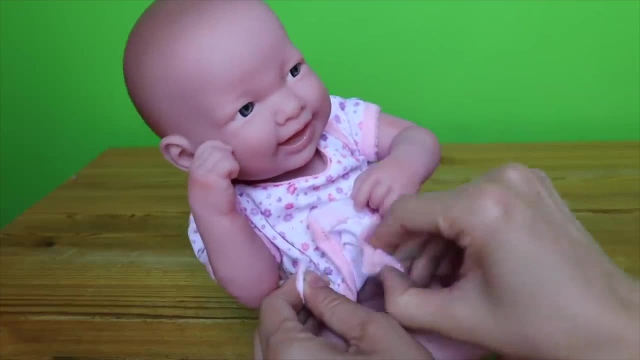 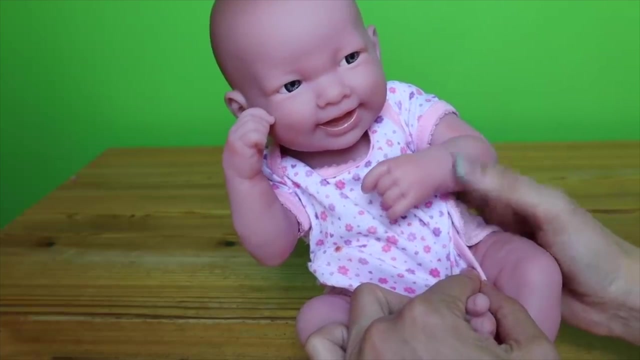 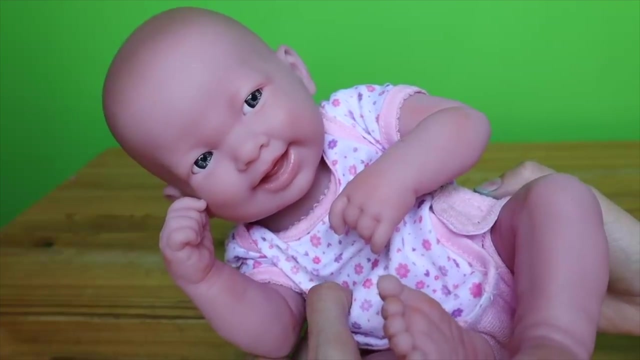 it on, Put it on, put it on, put it on. Good job, Hee, hee, hee. Now the baby's happy, She's laughing, Hee, hee, hee, Wah, Wah, Uh-oh, The baby's crying again. Uh-oh, Can you say on? 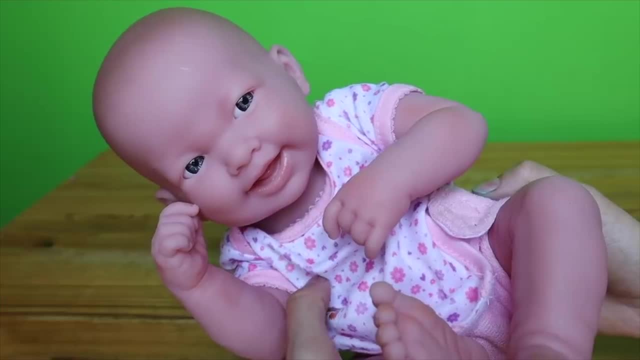 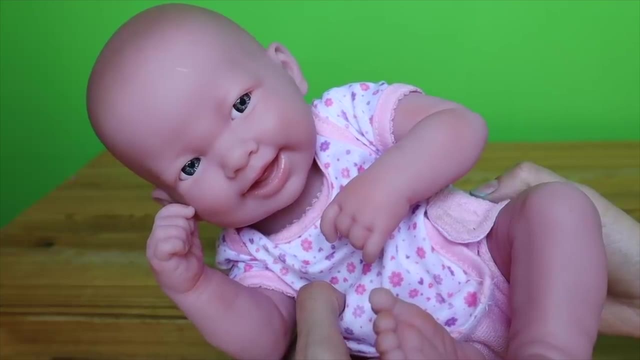 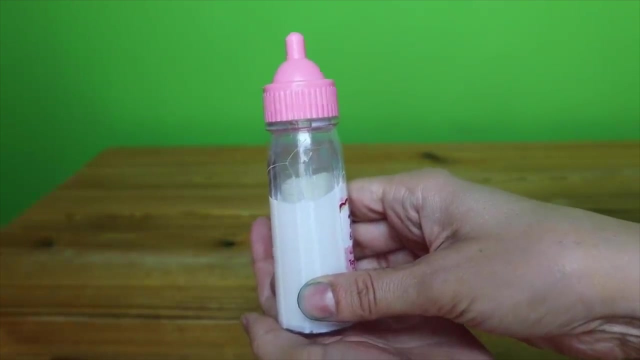 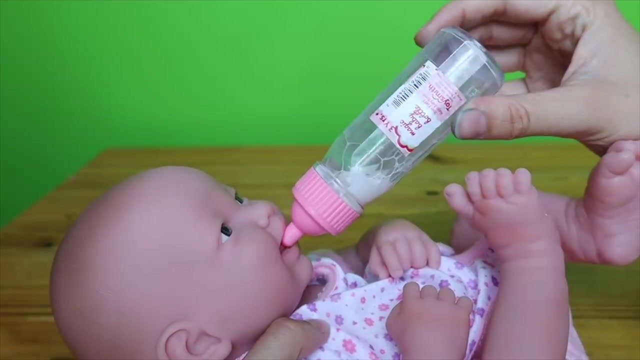 What should we do? Maybe we should give the baby some mmm milk. Can you say that Milk? Mmm Milk Say milk. You said milk and the milk came out. Good job. Give baby milk. Give baby bottle, Drinking bottle. The baby is drinking a bottle. 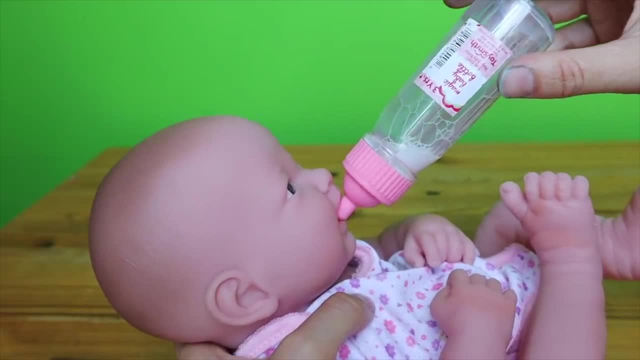 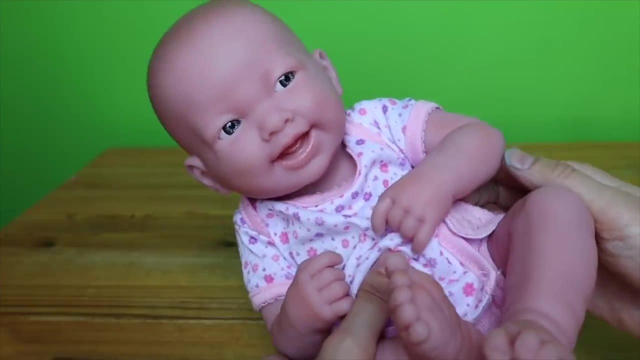 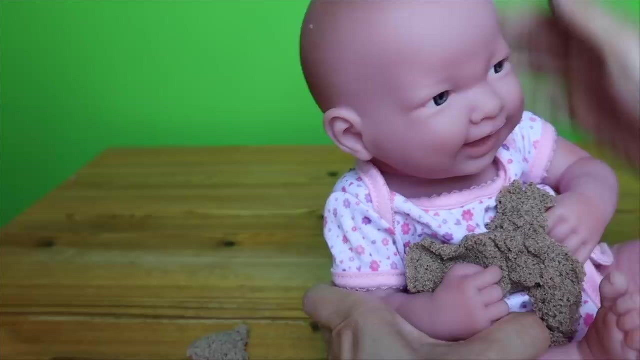 Ah, She's all done, All done. The milk is gone. All done, bottle, All done. Hee, hee, hee. She's happy now She has a full tummy. Hee, hee, hee. She's laughing. Uh-oh, Can you say uh-oh? 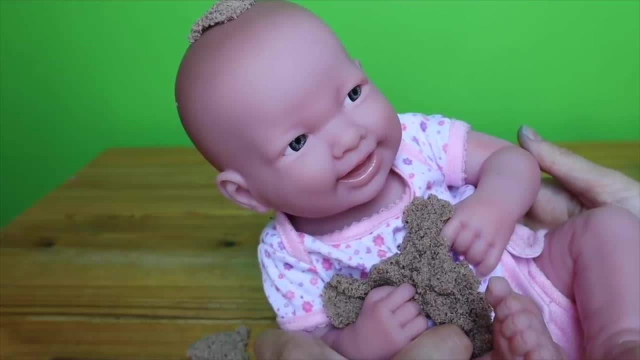 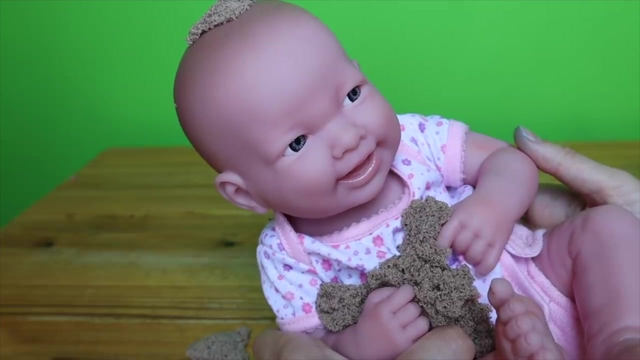 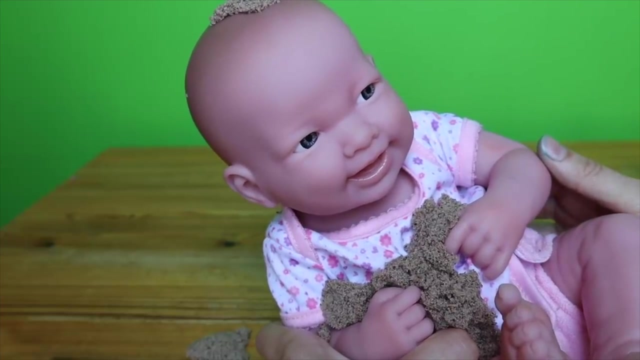 Uh-oh, The baby was playing in the sand and now she's dirty, Uh-oh. So what do we need to do to clean the baby? if she's dirty, We need to give her a bath. Yeah, The baby's covered in dirt, So we need to give her a. 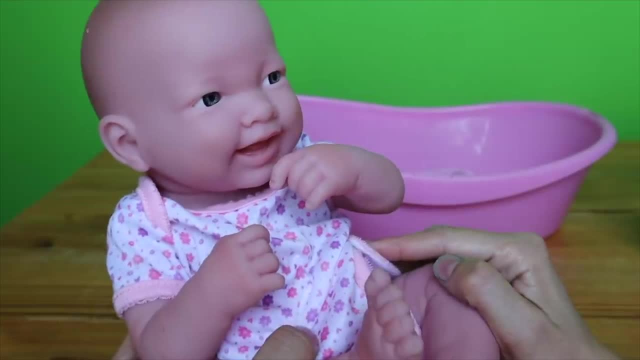 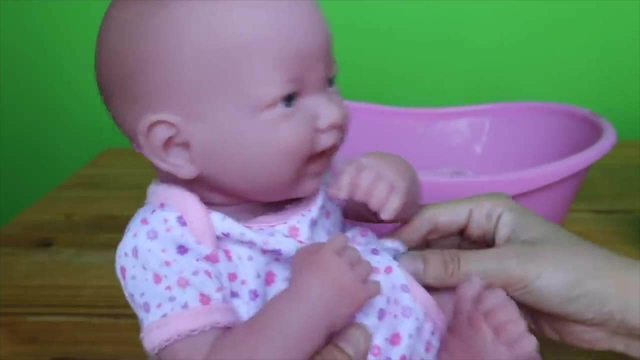 bath. Let's go get her bath. Should the baby wear her clothes in the bath? No, So silly. We don't wear clothes in the bath. No, Can you shake your head? no, They will notice, Aaaahhh. 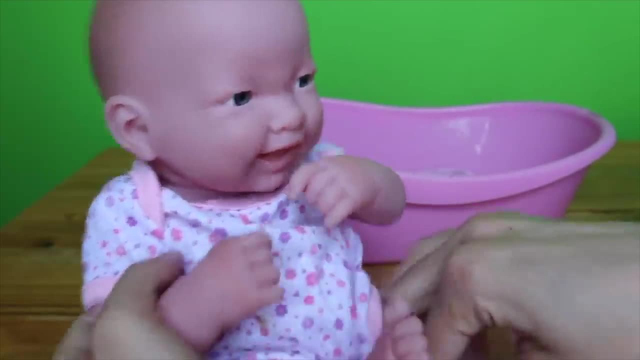 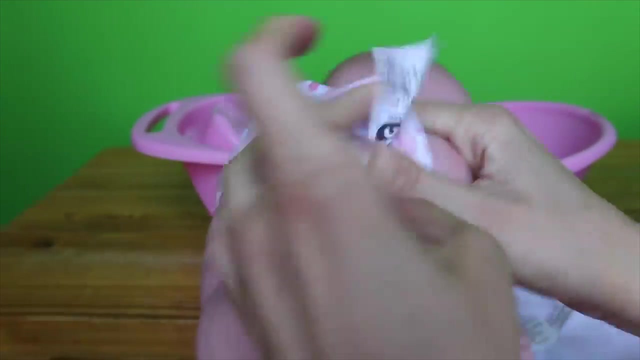 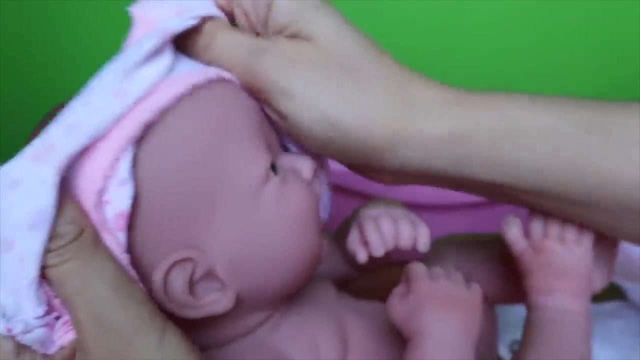 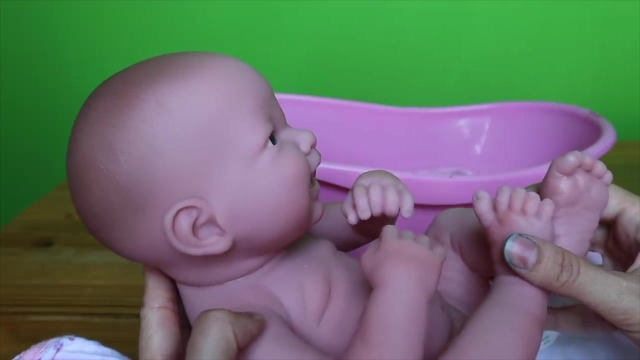 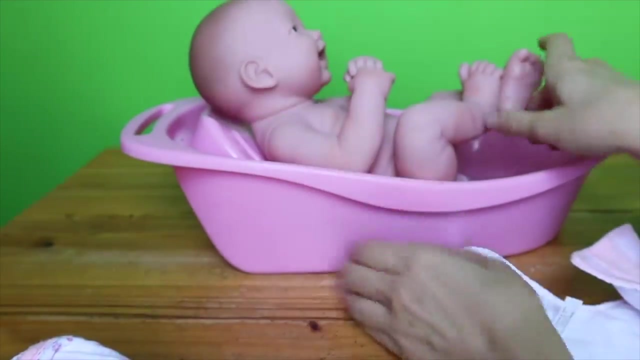 Gracias, mas head. no, That's so silly. Off, Take clothes off, Off, Off, Take off. Now we need to put the baby in the bath. Can you say in, Put her in, Put her in, Put her in. Oh she's. 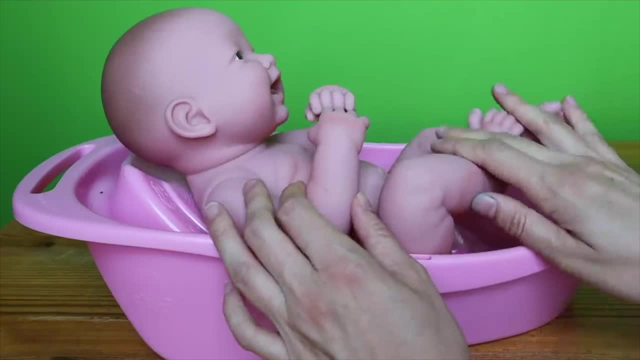 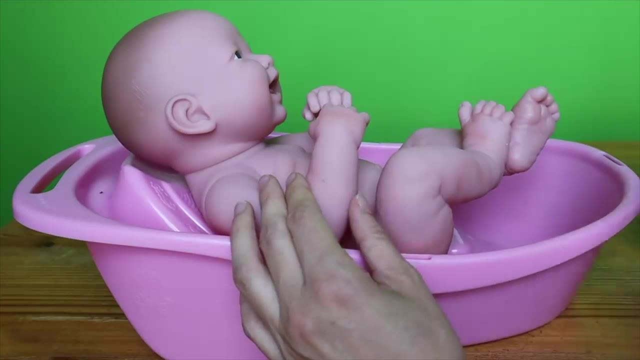 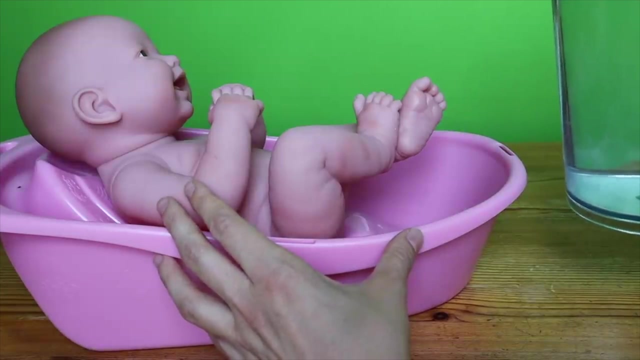 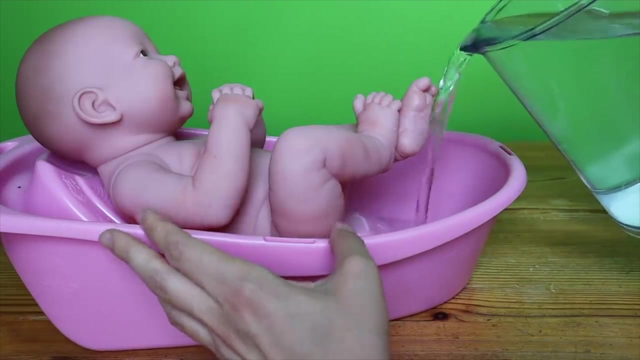 happy in her bath. Now what do we need to wash the baby? It begins with the w sound, W, w: Water. We're going to pour in some water. You say in and I'll pour the water in. Pour it in, Pour it in, Pour it in. You said in, so I'm pouring the water in She likes. 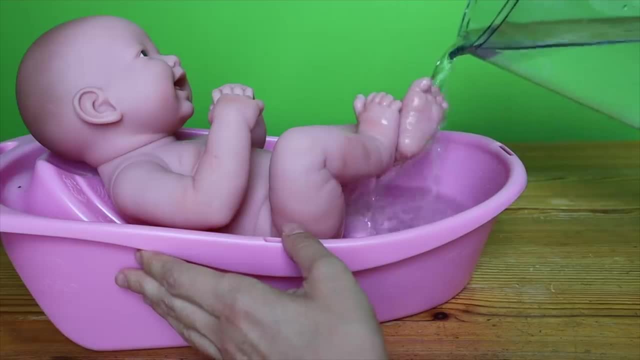 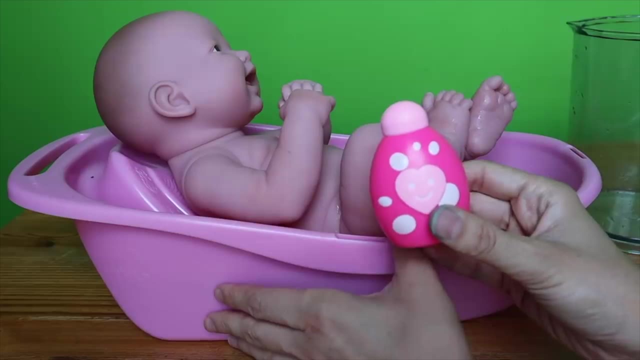 the water on her little toesies. She likes the water on her toes. She's laughing. She likes the bath. Now we have some pretend soap. Let's put it on the baby. Put it on. Put it on On the baby. 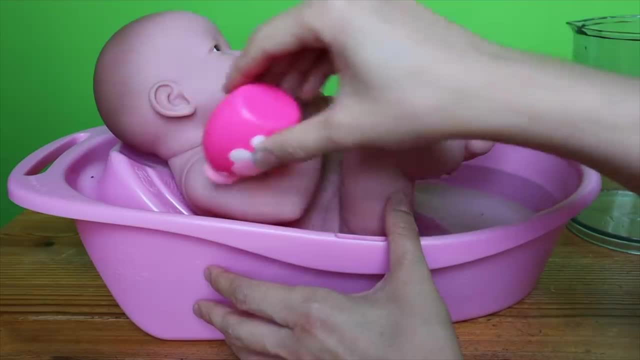 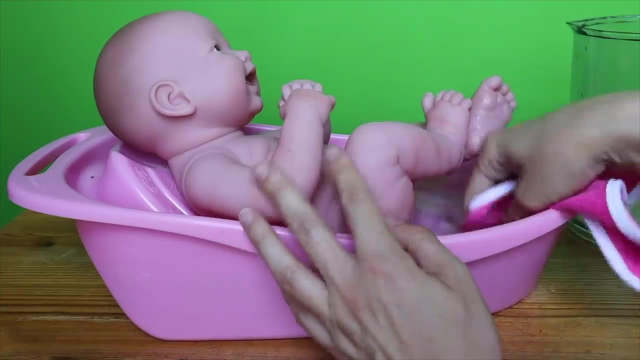 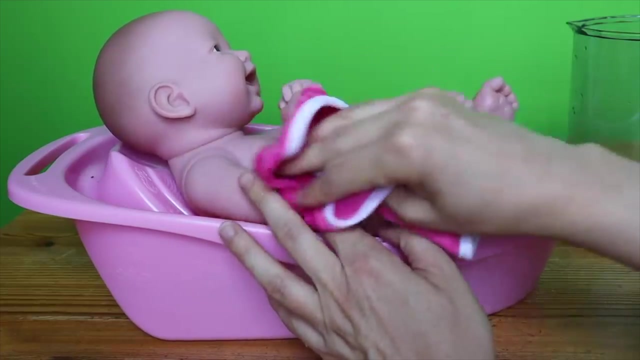 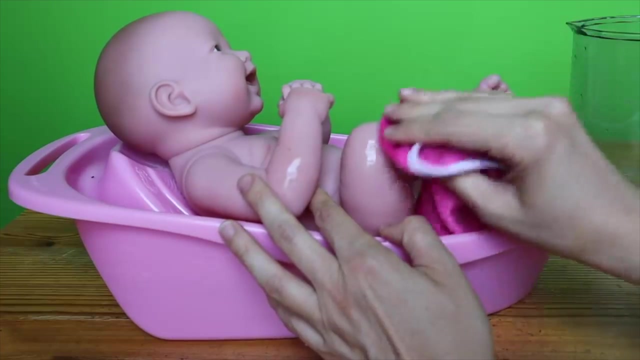 Putting the pretend soap on the baby, On the baby and in the water. Now we take a wash cloth and we wash the baby, Wash baby, Wash baby, Wash baby. Good job, washing the baby. Wash baby's feet, Wash baby's legs. 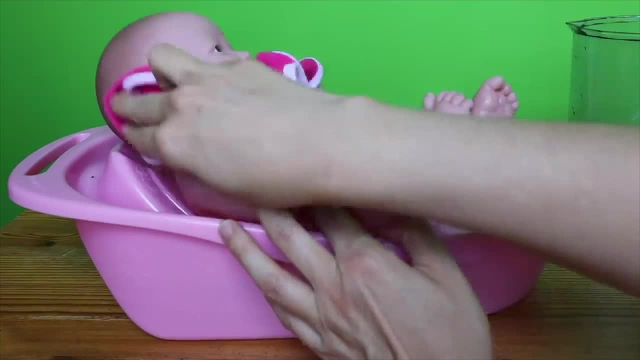 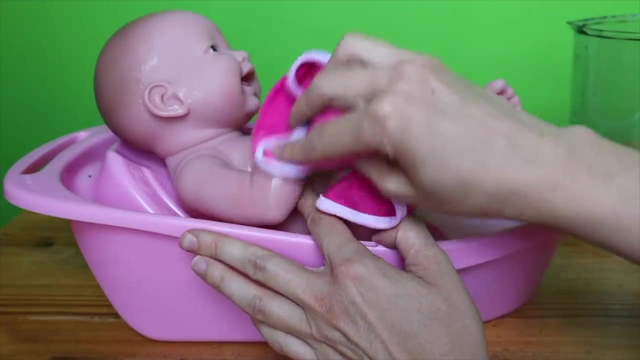 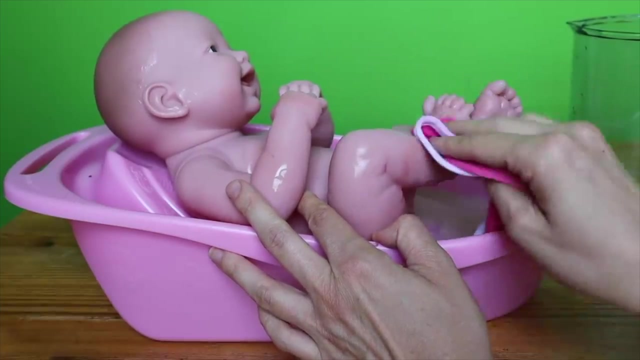 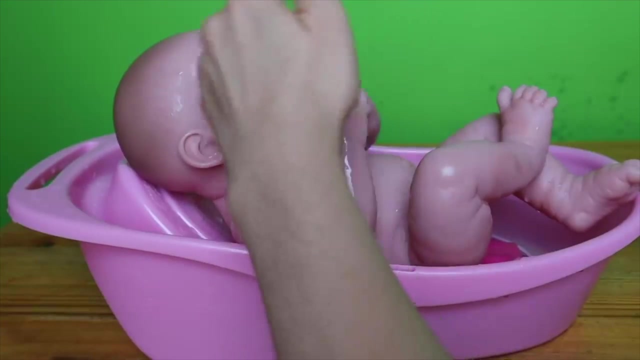 Good. Wash baby's head. Wash baby's hair. Wash baby's ears. Wash baby's arms. Wash baby's hands. She likes the water. Now I'm going to rinse off the baby. When I rinse off her hair, I'll put my hand here so we don't get any soap in her eyes. I like that. 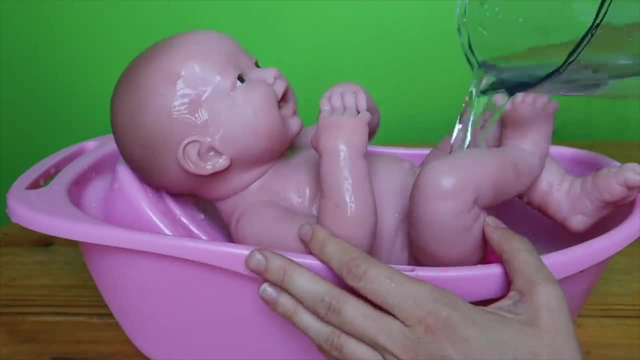 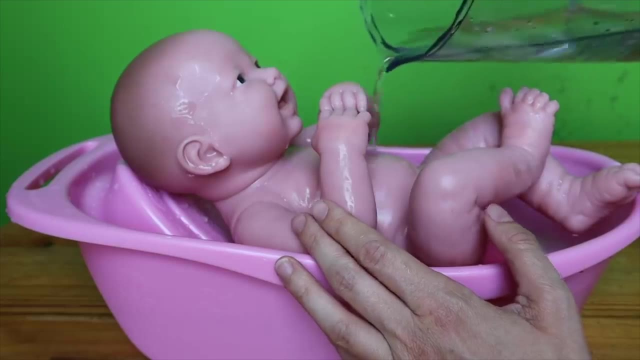 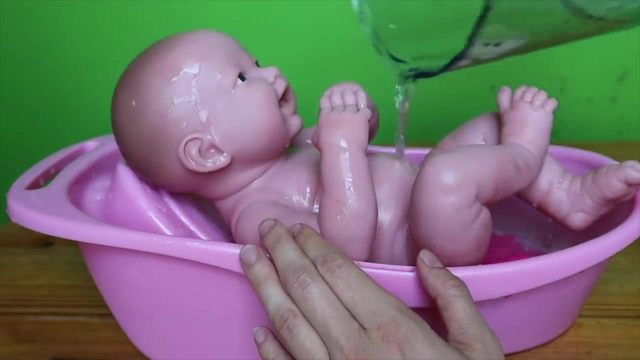 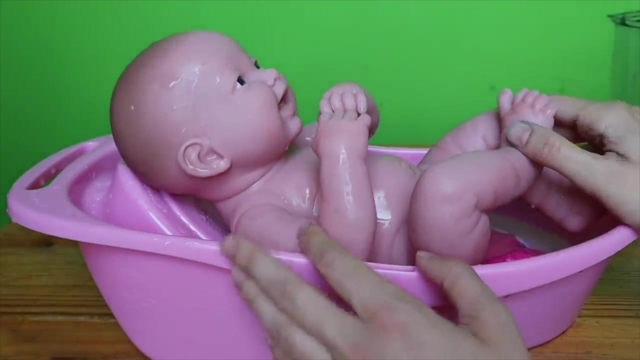 Yeah, it doesn't hurt. Water feels good. I like the bath. Oh, the baby likes the bath. Rinse off the baby, Rinse her hair. Good job, baby. Rinse off the baby. Yay, The baby is getting so clean Now. the baby's all done the bath, All done, All done bath. 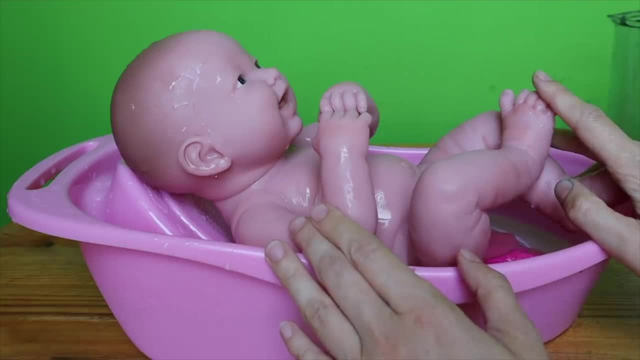 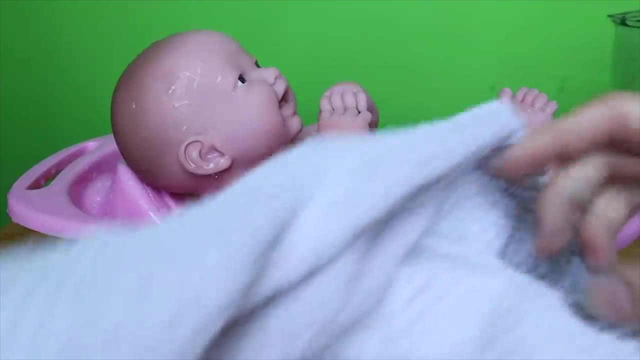 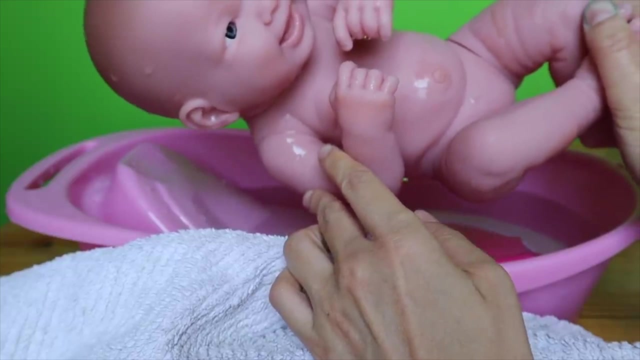 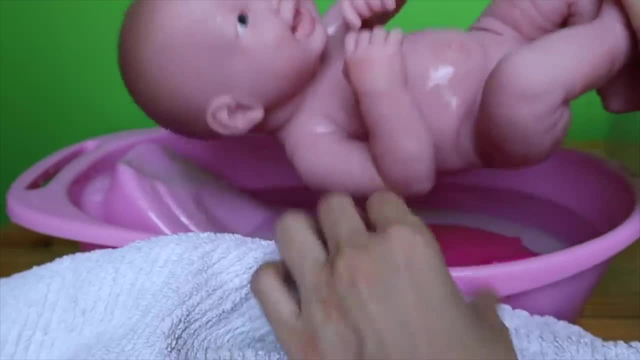 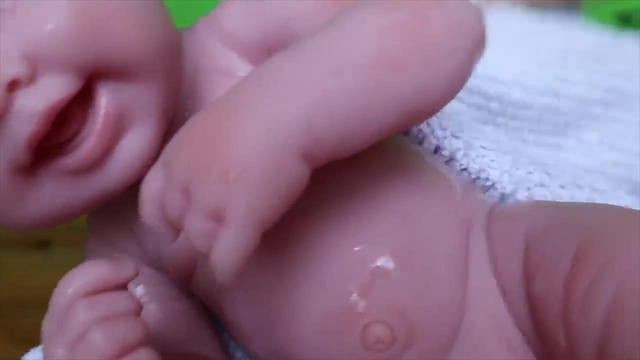 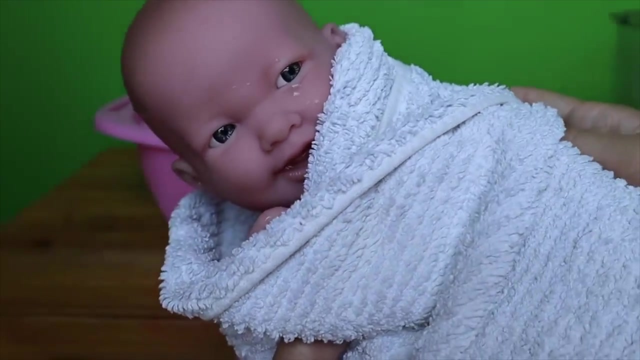 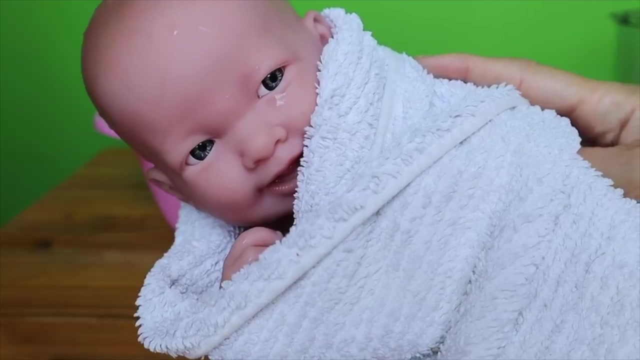 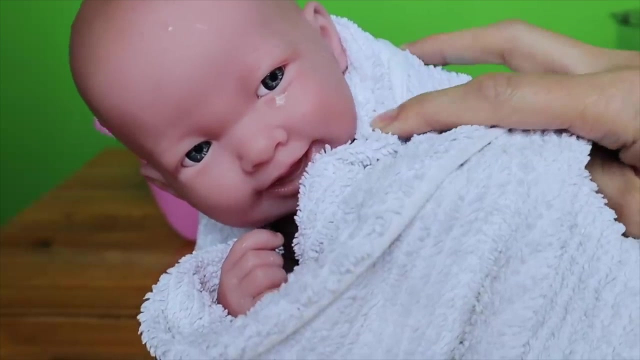 bath tomorrow. Maybe she's cold. Let's wrap her in the towel, Put her in. Put her in. Put her in. Wrap her in the towel. She feels so warm and happy now. Thank you for my bath. Oh, she's babbling. Let's listen to what she's trying to say. 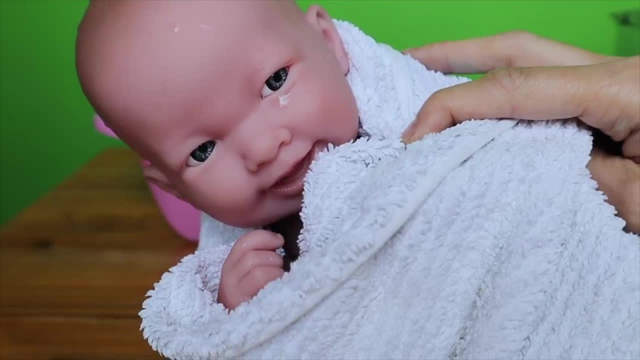 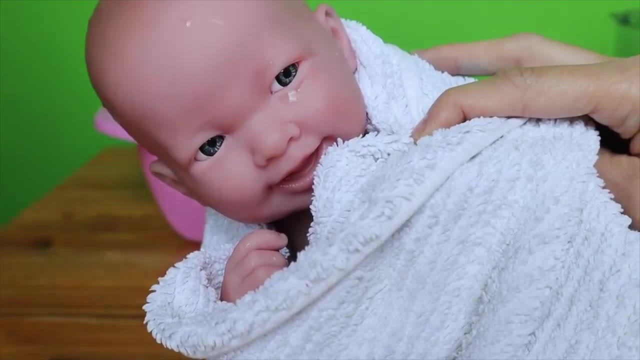 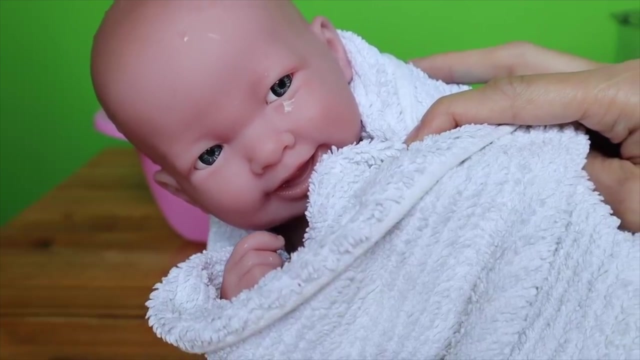 Ba-ba-ba-ba-ba-ba-bath. She said: bath, Da-da-da-da-da-da-da-da-da. She said: da-da, Mmm, Mmm, Ma-ma-ma-ma-ma-ma. She said: mama. 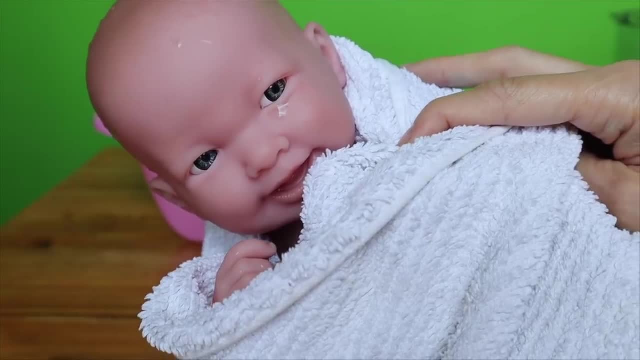 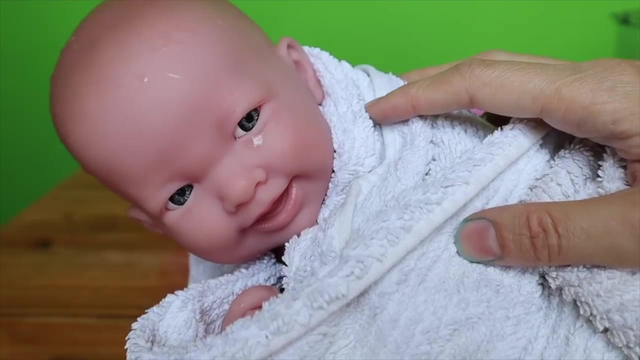 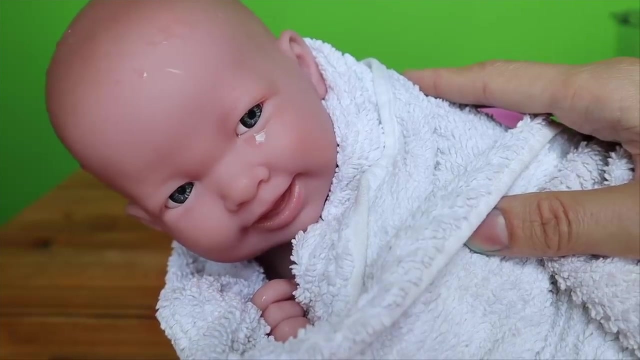 Ba-ba-ba-ba-ba-ba-baby- Yes, you're a baby. Ca-ca-coo-coo. Oh, you're so cute. I love you, baby Muah. Give the baby a hug, Give it a kiss. So much fun. Thank you for helping me give the baby a b-b-bath. Good. 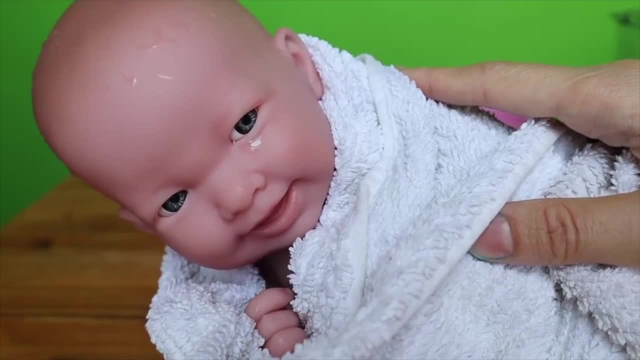 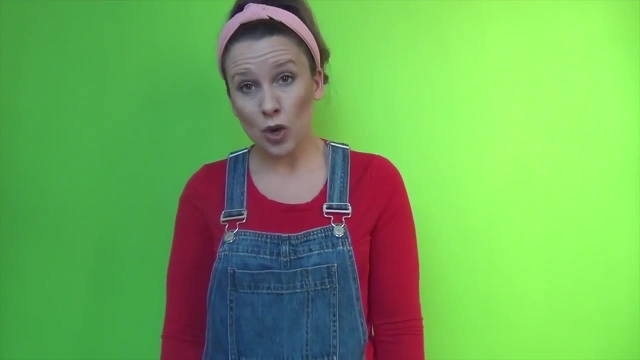 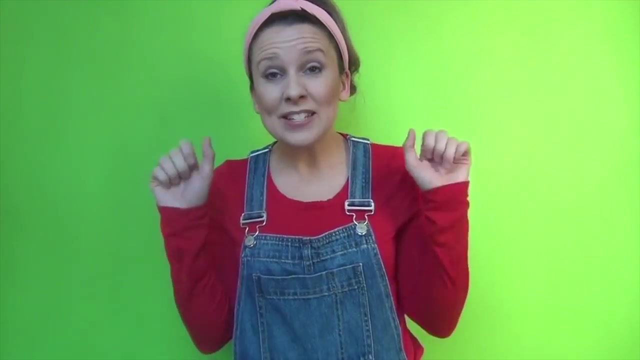 job. The baby is all clean, All clean, All done. bath. Next let's do my favorite song. It's called Open Shut Them. For that we need our two hands. One, two. Are you ready? Open, shut them. Open, shut them. 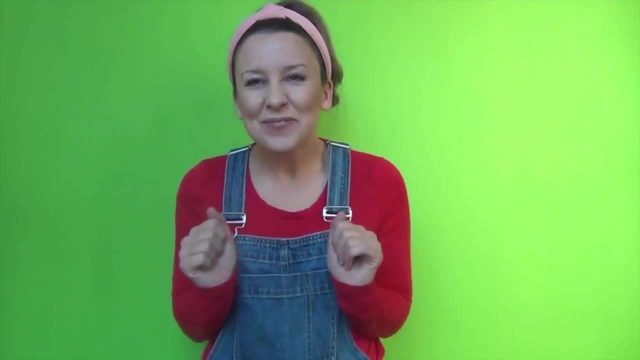 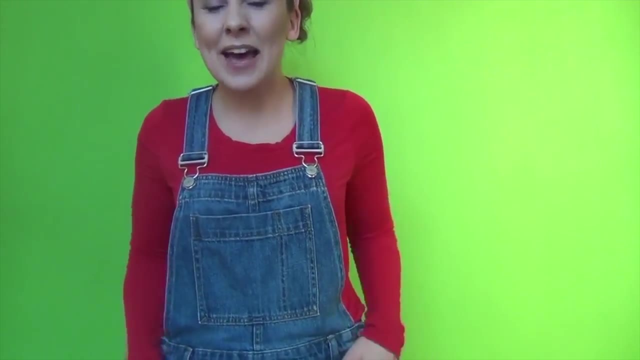 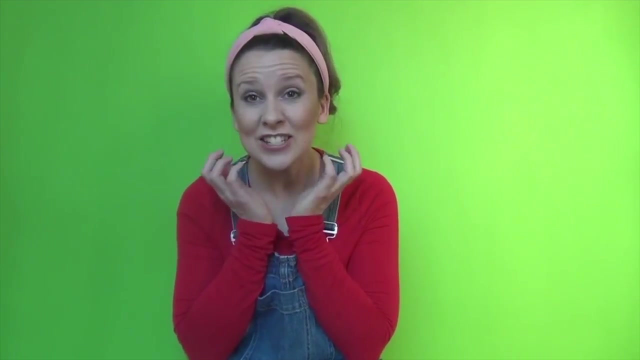 Give a little clap, clap, clap, Open, shut them, Open, shut them. Put them in your lap, lap, lap, Creep them, crawl them, Creep them, crawl them Right up to your chin, chin, chin. Open wide your little mouth. 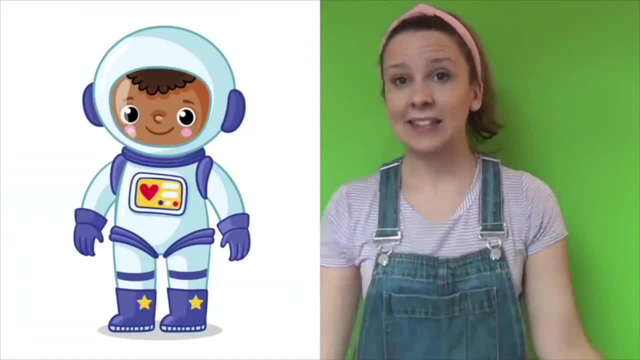 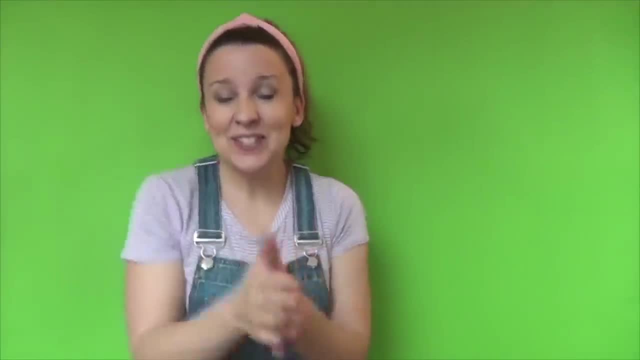 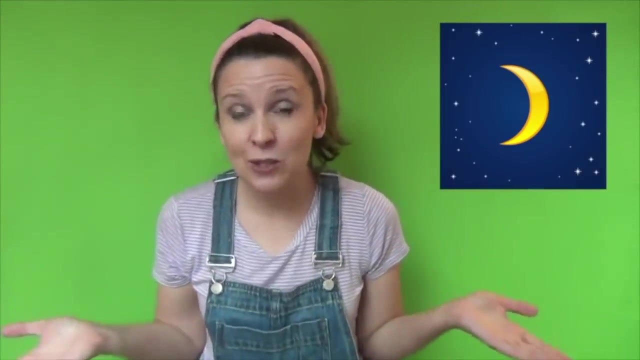 But do not let them in. That was so fun. Let's put on her space helmet And put on our space suit. Zoom, zoom, zoom. We are going to the moon. Zoom, zoom, zoom, We are going to the moon. 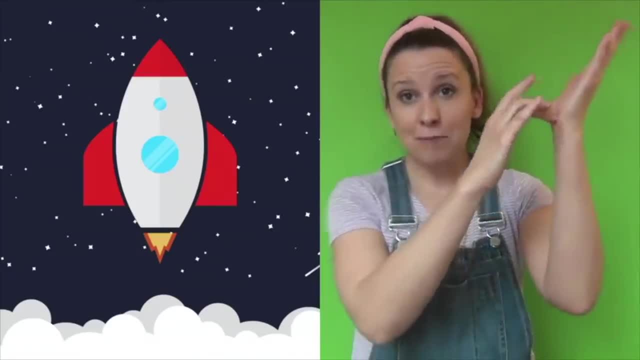 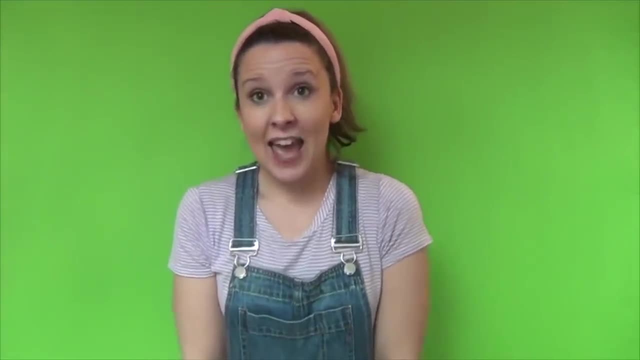 If you want to take a trip, I'm aboard my rocket ship. Zoom, zoom, zoom. We are going to the moon. Ten, nine, eight, seven, six, five, four, Five, four, three, two, one. 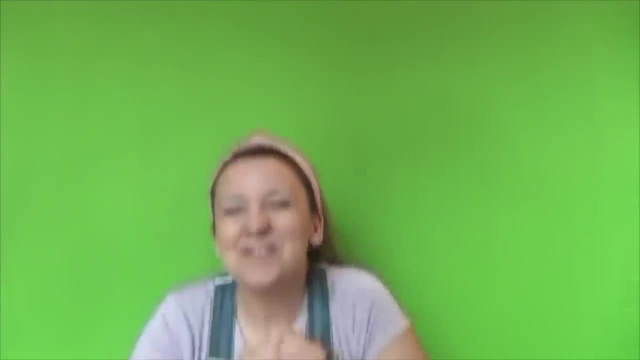 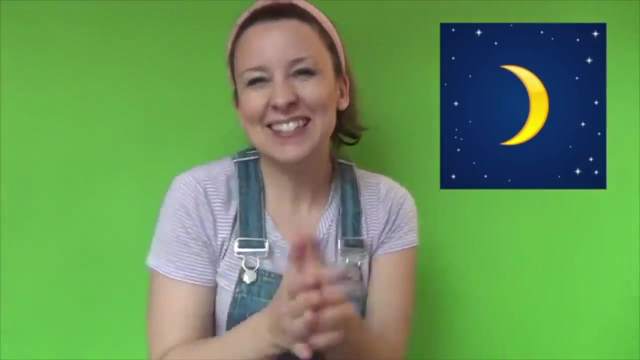 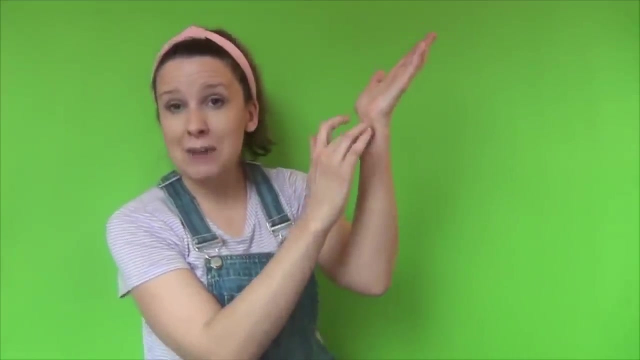 Three, two, one blast off. Zoom, zoom, zoom, we're going to the moon. Zoom, zoom, zoom, we're going to the moon. If you want to take a trip, climb aboard my rocket ship. Zoom, zoom, zoom, we're going to the moon. 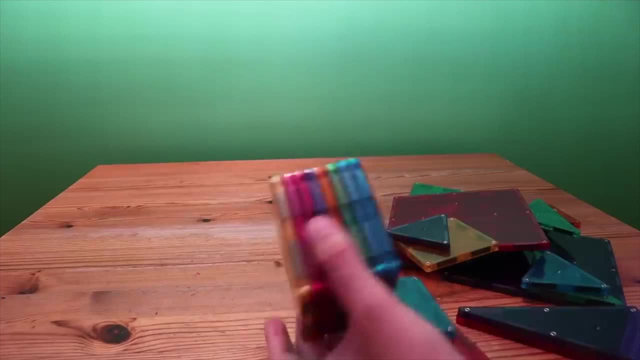 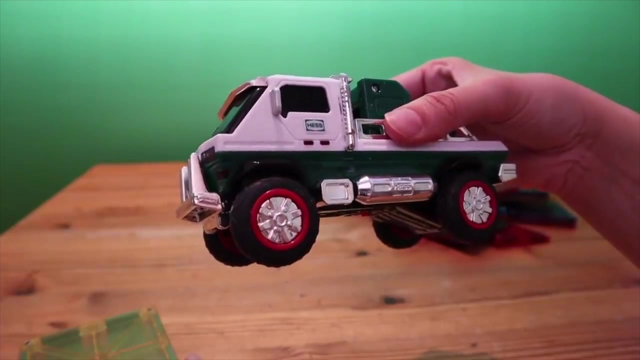 Now let's play with some toys. Have you ever played with these? They're called magnetiles. Oh no, the truck needs a garage. Can you help me build it? Great, Okay, let's use this big one as the bottom of the garage. 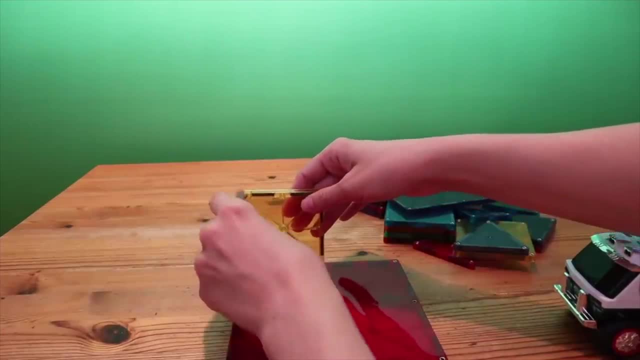 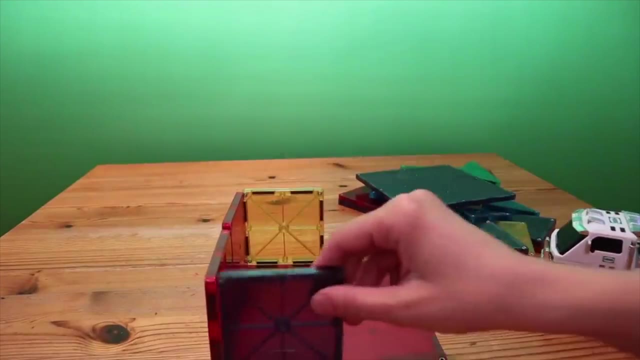 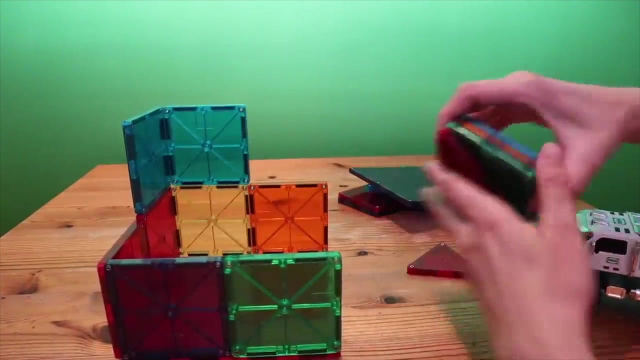 That looks great. Now let's put some smaller ones to make the sides of the garage. I like my garage already Good. we'll keep making your garage. Put on those. Yeah, they stick together. Put on the parts of the garage. 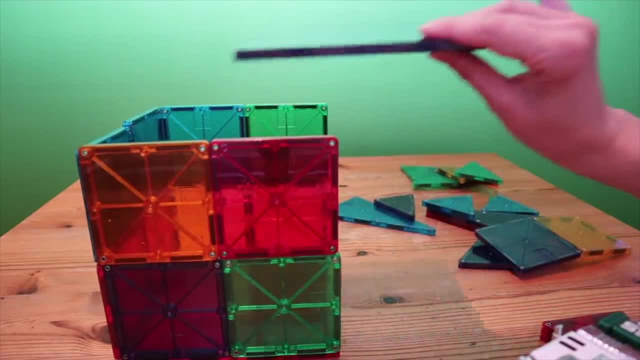 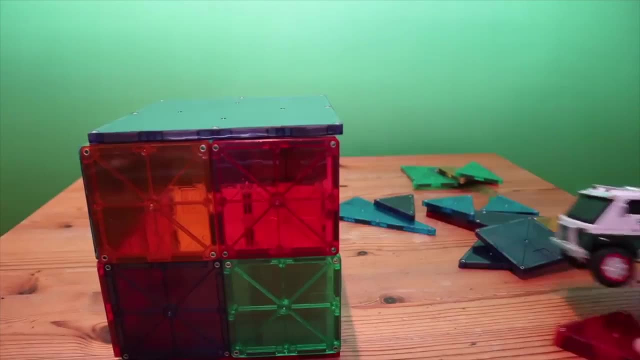 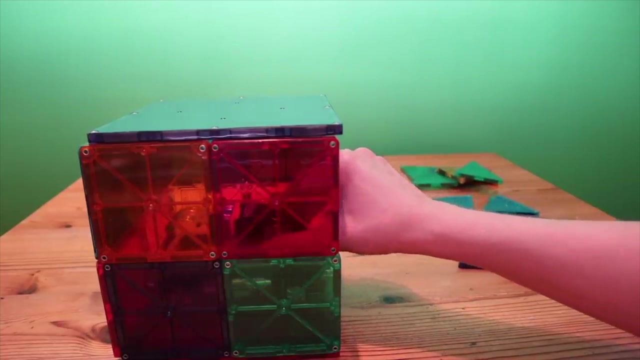 Okay, should we put the roof on? Putting on the roof of the garage. good job, My garage is awesome. I'm going to drive in Vroom, vroom, vroom, Going in the garage. I love it. We did it. 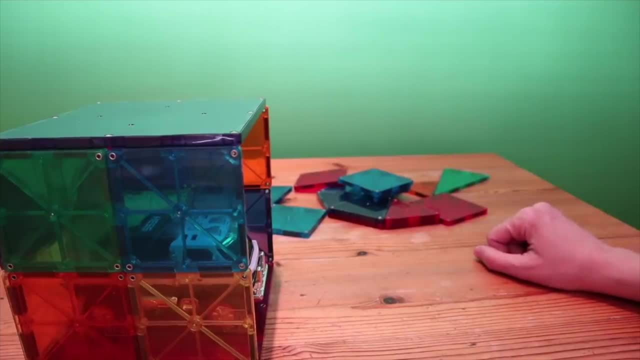 Ding, ding, ding, ding, ding. it's morning. The truck needs to go to work. That's my alarm clock. I gotta go to work. Oh, I had such a nice night in my garage, Bye-bye. The itsy bitsy spider went up the water spout. 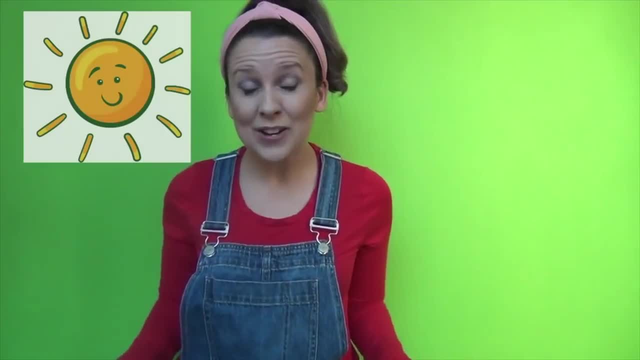 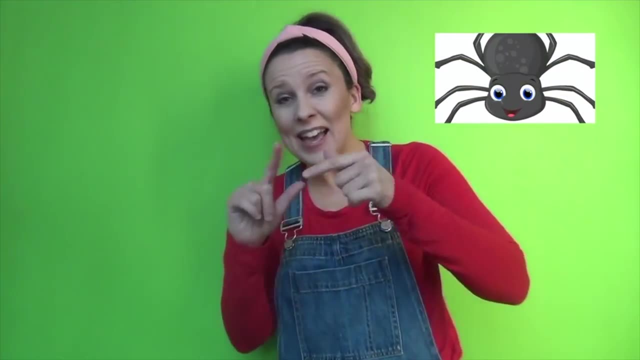 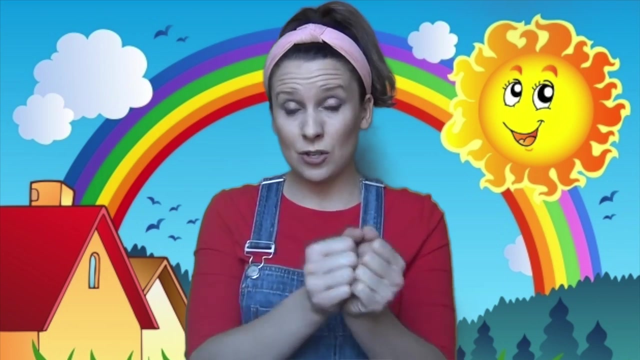 Down came the rain and washed the spider out. Out came the sun and dried up all the rain And the itsy bitsy spider went up the spout again. The more we get together, together, together, together, the more we get together. 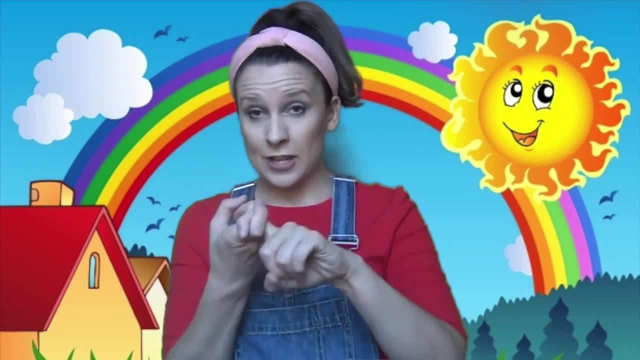 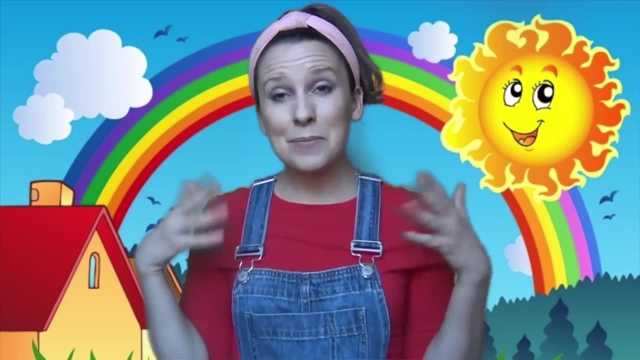 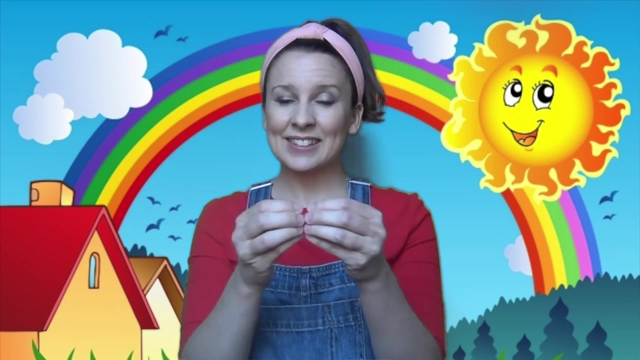 the happier we'll be, Cause your friends are my friends and my friends are your friends. The more we get together, the happier we'll be. Can you try this? sign for more More Good job. Wow, this bin is full of treasure. 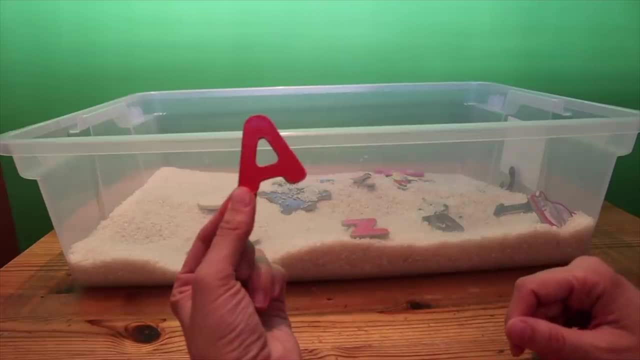 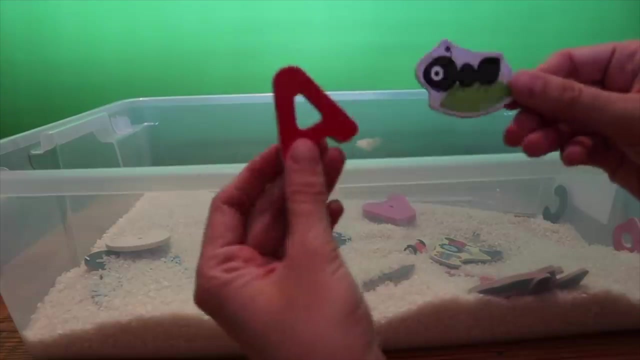 To find the treasure, we have to find another capital A that matches this A, A red capital A. Do you think we can do it? Great, Thank you so much. That's a cat, That's not an A. Hmm, is this the same? 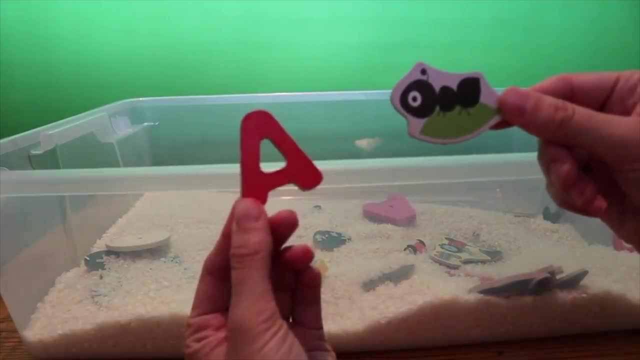 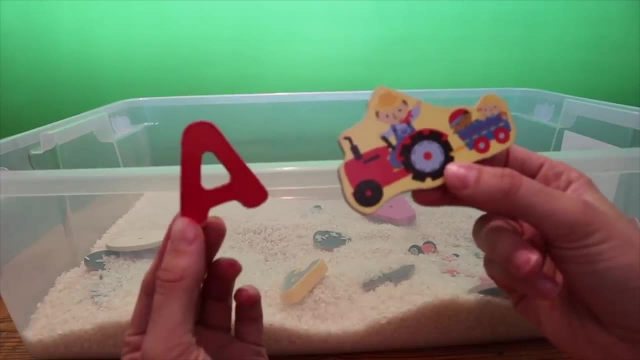 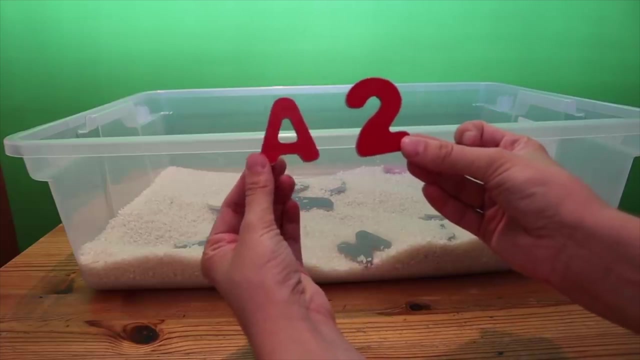 No, Ant does start with A, but it's not a capital A. Wow, a tractor. A tractor's red, but it's not an A. This is red. Is this the same? No, It's the number two. Oh, this is a red circle. 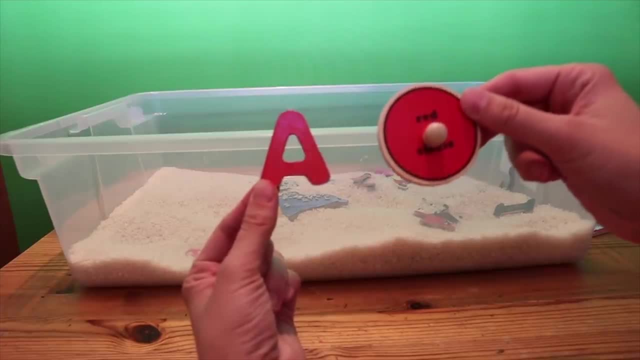 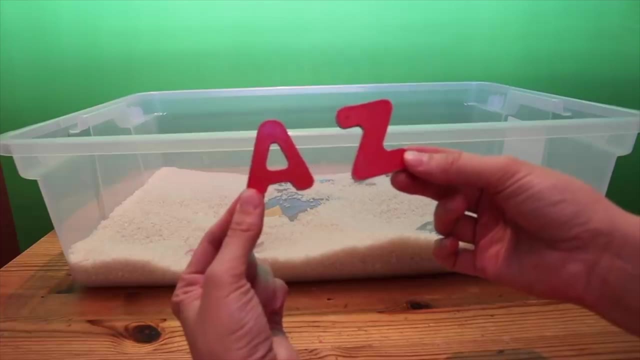 A circle is the shape of the day and red is the color of the day, but that doesn't match. Oh wow, It's a capital letter and it's the color red. But it doesn't match, does it, Cause it's a C. 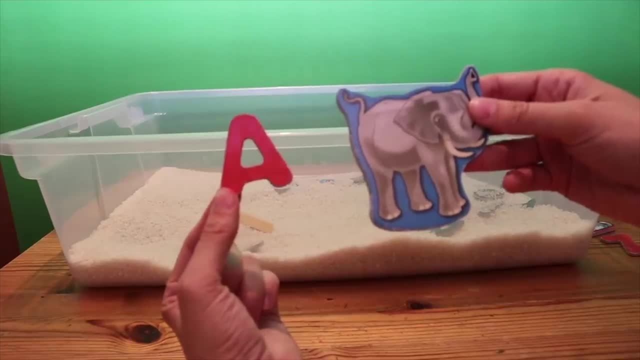 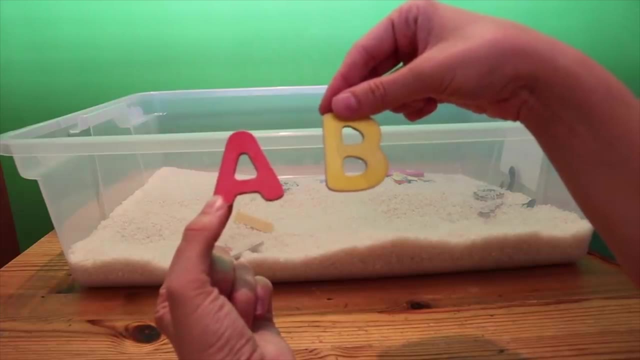 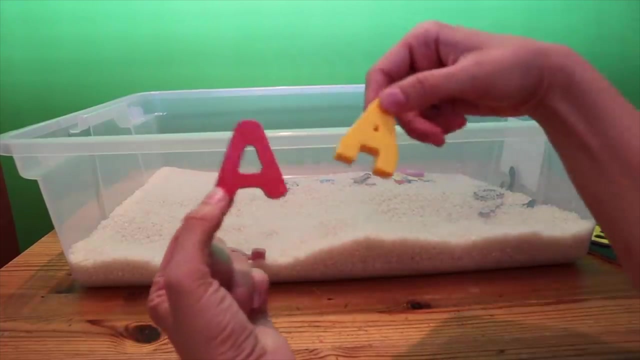 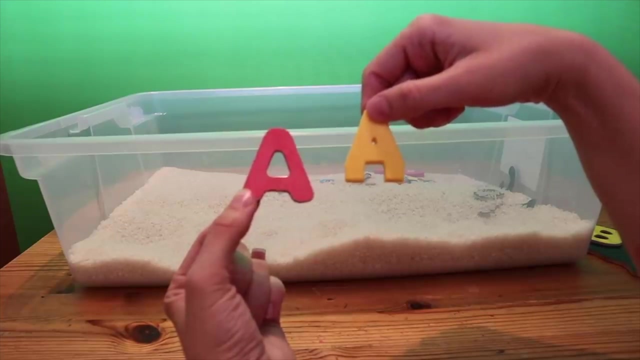 No, That's an elephant. Here's a capital letter, but it's a B and it's yellow. Nope, I found another capital A. Does it match? No, it doesn't match completely, because this A is yellow. We're looking for another capital letter. 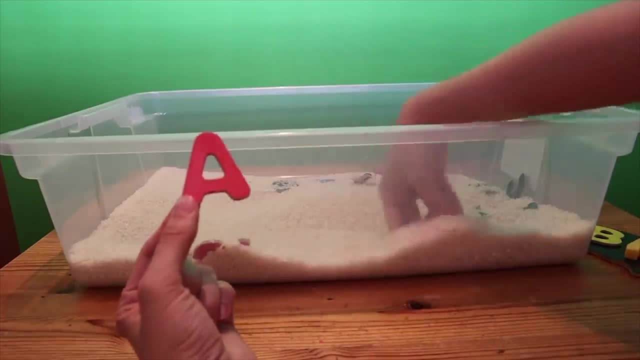 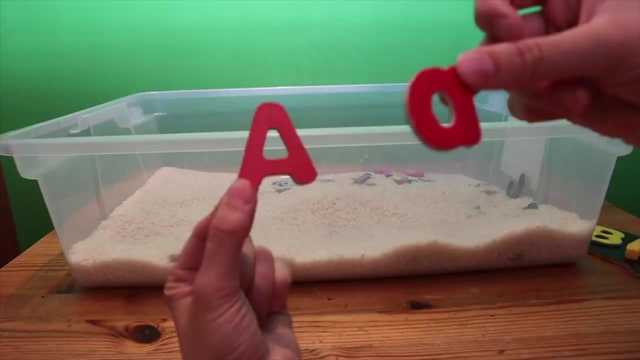 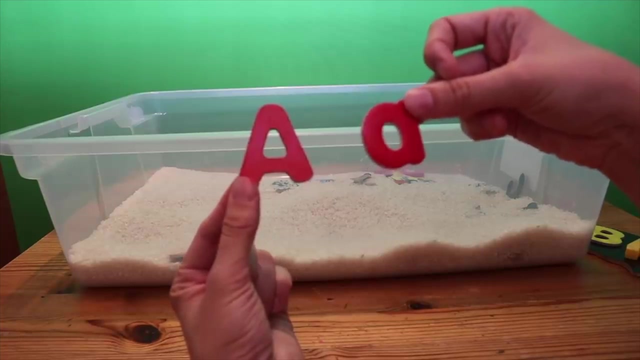 and we're looking for another red A Digging around. Help me dig. Can you help me dig? You helped me find another red A. Did these match? Well, this is a capital A and this is a lowercase a. It looks different. 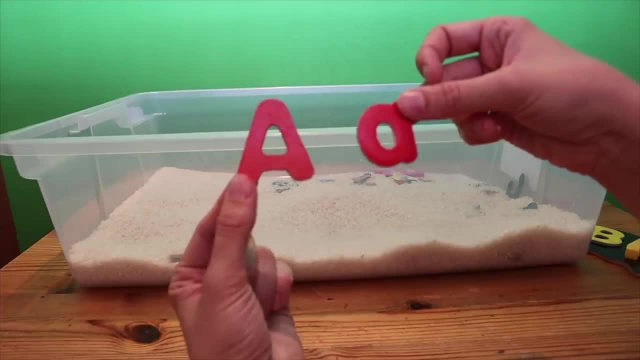 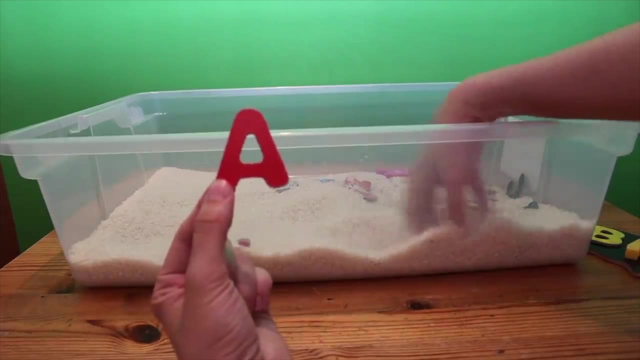 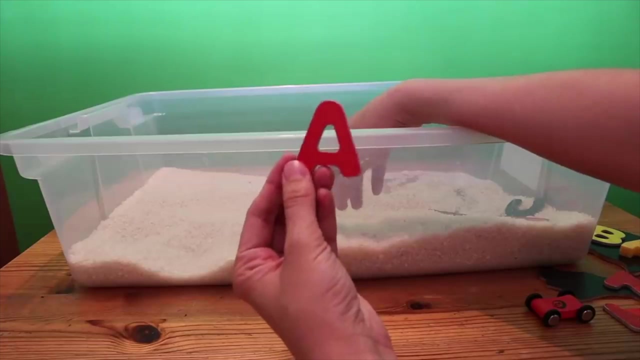 but it has the same sound, A, But it's not exactly the same, and we're looking for a match. Help me dig Dig. Ooh, A red car, No, that doesn't match. Help me dig really deep. 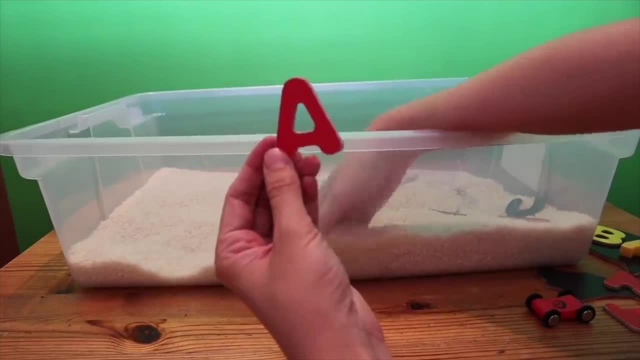 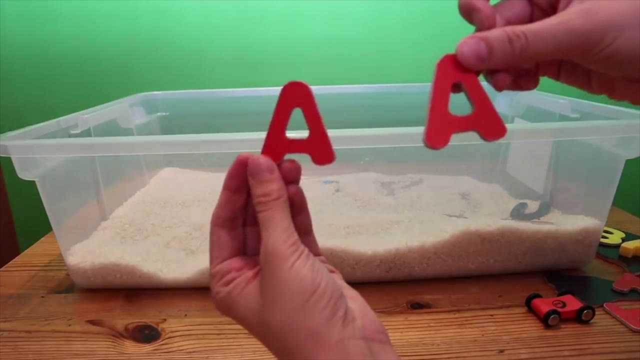 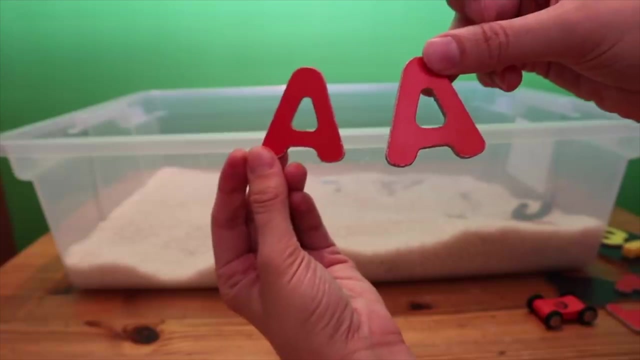 and maybe I can find it Dig really deep, Digging deeply. Whoa Does this match? Yay, Hooray, It's a match: Two capital A's that are the same size and they're both red. Yay. 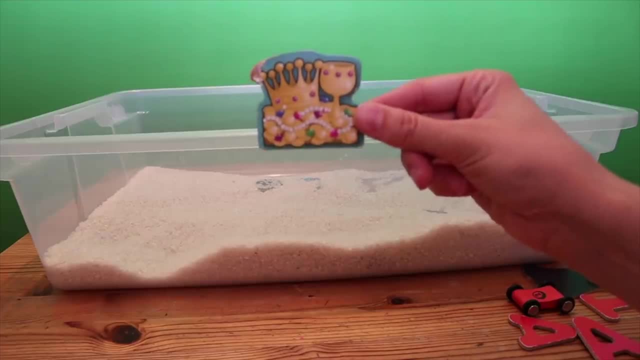 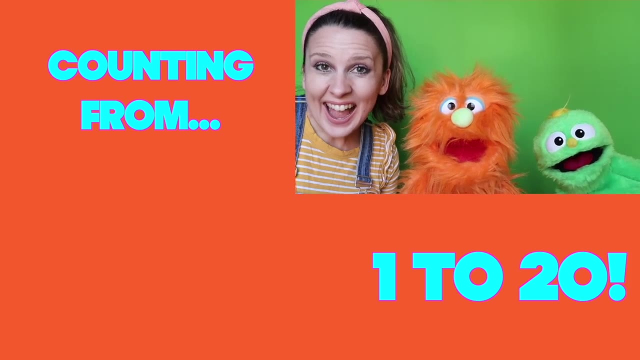 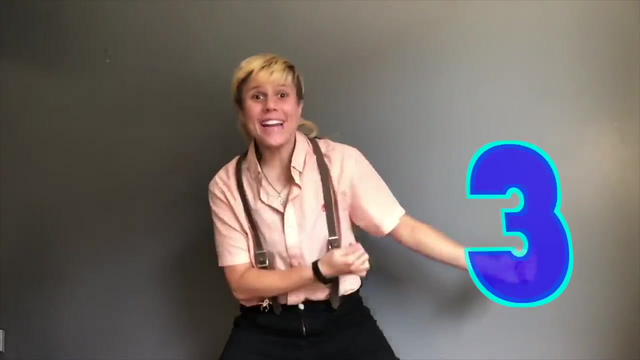 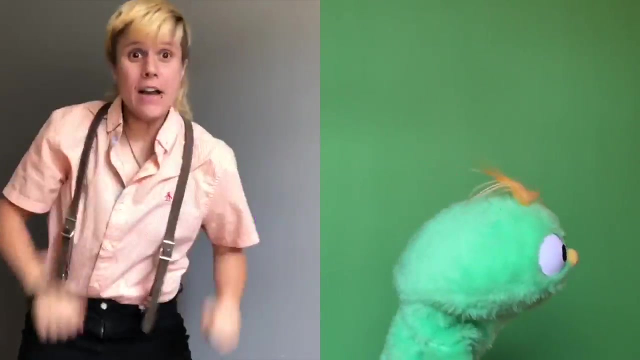 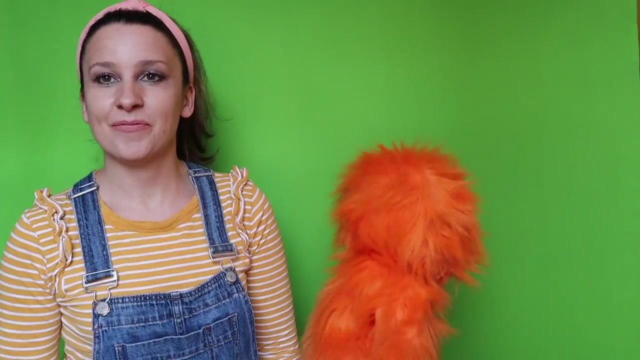 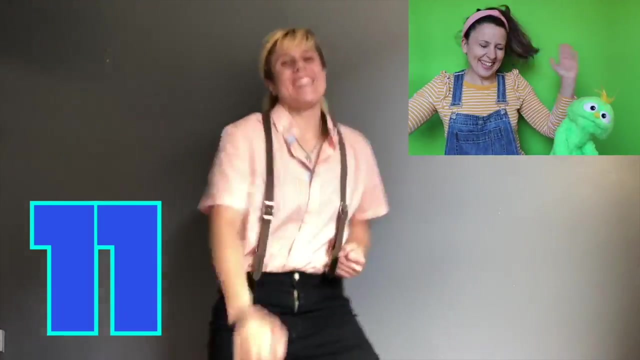 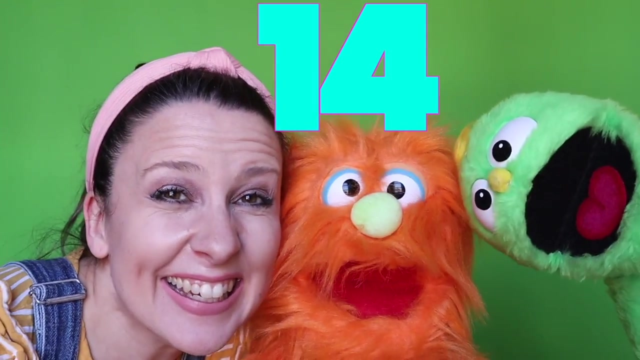 We found the matching capital A and the treasure came out. You helped us find the treasure. Great job One, Two, Three, Four, Five, Six, Seven, Eight, Nine, Ten, Eleven, Twelve, Thirteen, Fourteen. 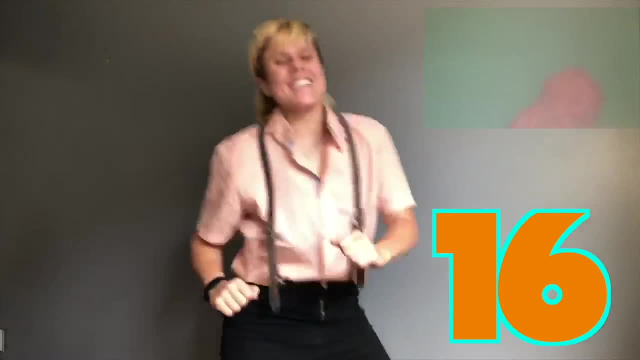 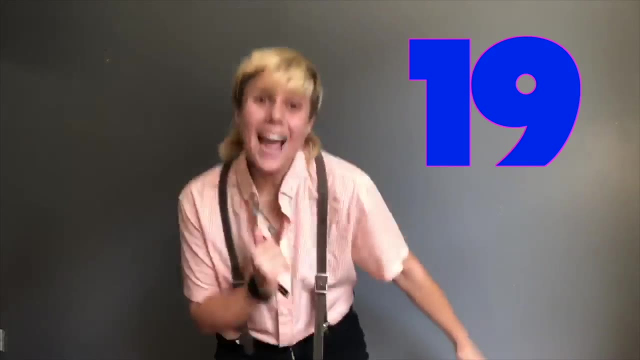 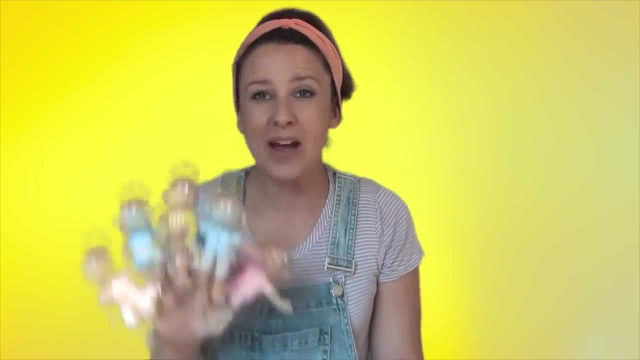 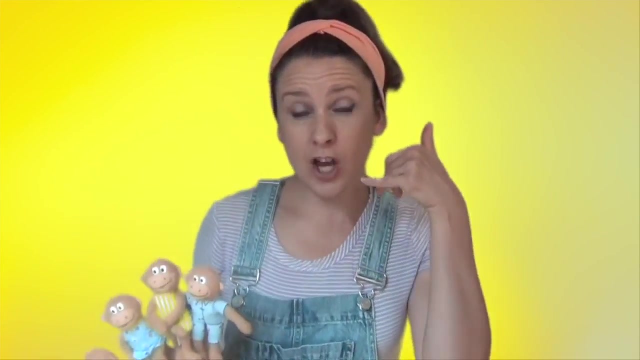 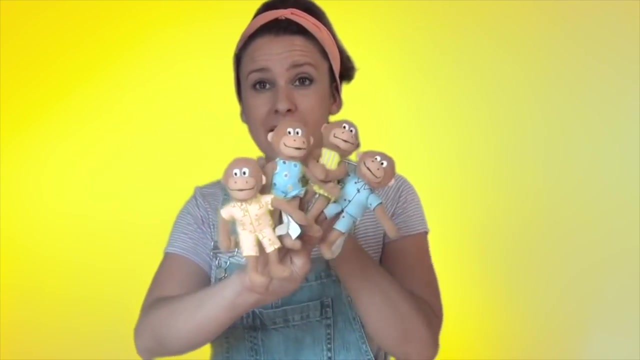 Fifteen, Sixteen, Seventeen, Eighteen, Nineteen, Twenty, Thirteen, Thirteen, Fourteen, Twenty, Twenty, Fifteen, Esther teaspoon, Twenty, Twenty Mine One Alright einf Emp Strategy Wednesday. 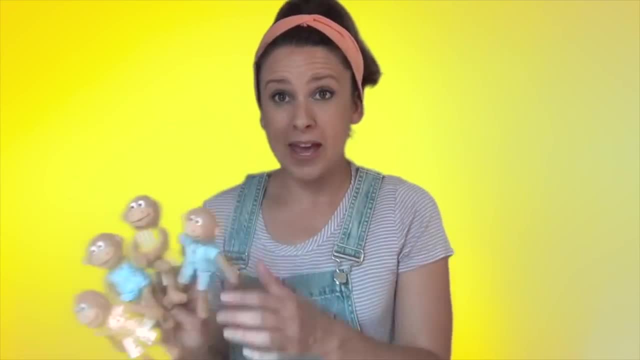 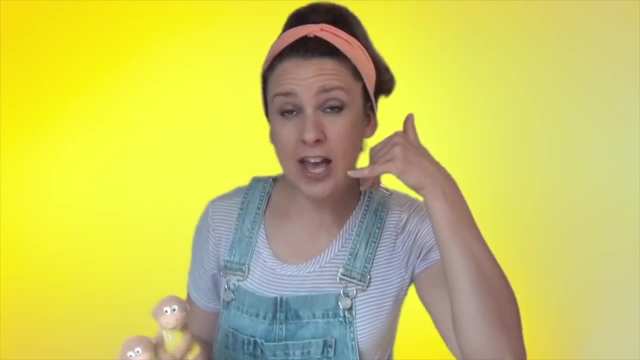 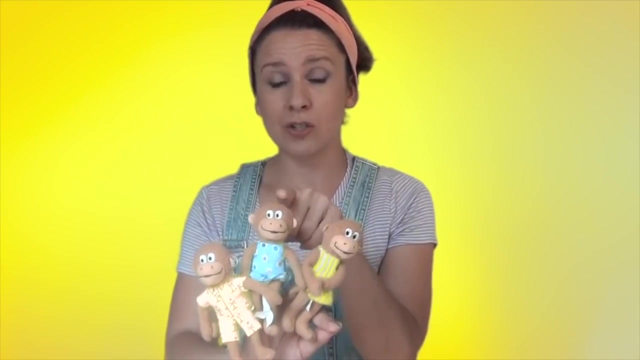 See you in the next video. Bye, Bye. You're studying Tomorrow. Huh, You're sending it to that friend. Her called the doctor and the doctor said: no more monkeys jumping on the bed. how many are left? count with me one, two, three, three little monkeys jumping on. 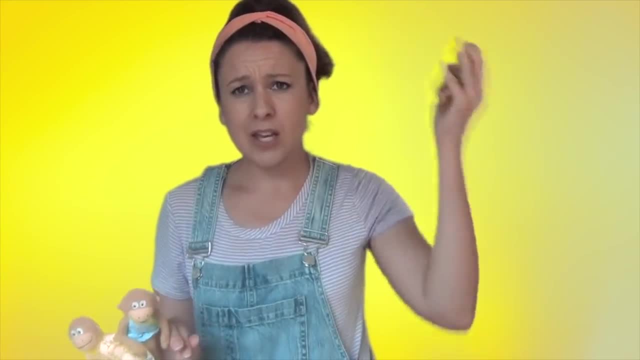 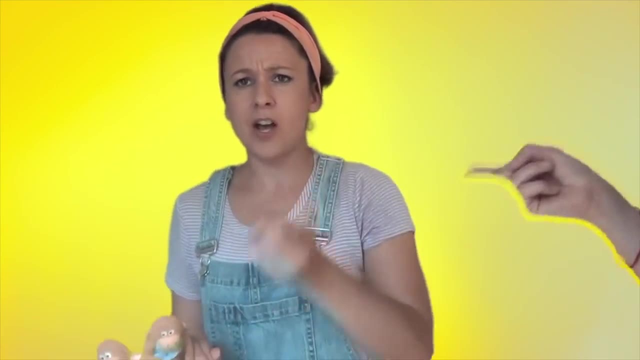 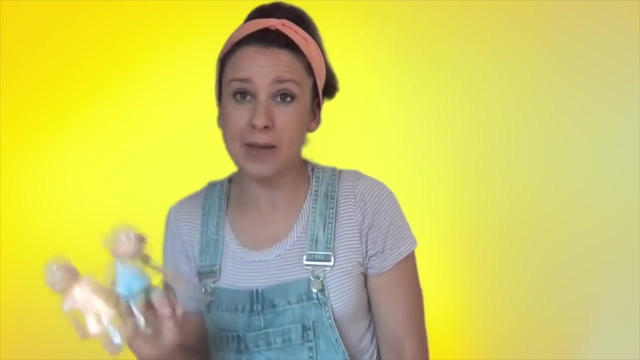 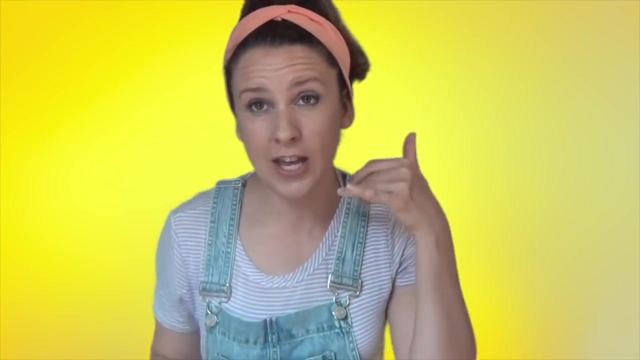 the bed. one fell off and bumped his head. mama called the doctor and the doctor said: no more monkeys jumping on the bed. how many are left? one, two, two little monkeys jumping on the bed. one fell off and bumped his head. mama called the doctor and the doctor said: no more monkeys jumping on the bed. how many are? 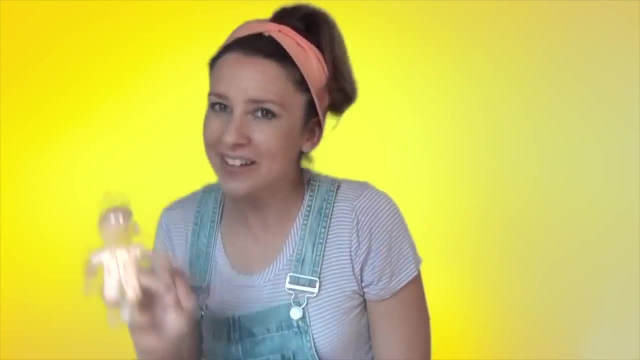 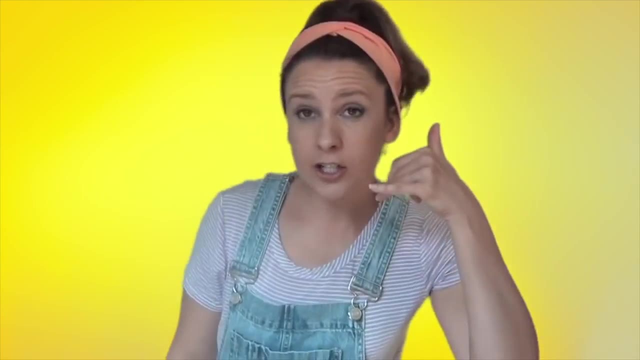 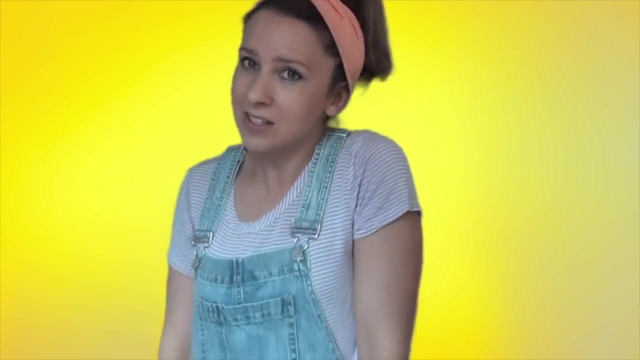 left just one little monkey. one little monkey jumping on the bed. he fell off and bumped his head. mama called the doctor and the doctor said: no more monkeys jumping on the bed. great job, monkeys jumping on the bed. great job telling me to get those monkeys to stop. 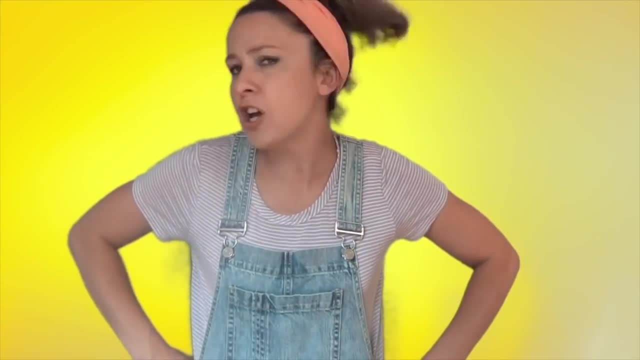 telling me to get those monkeys to stop. telling me to get those monkeys to stop jumping on the bed. say no, monkeys, no, jumping on the bed. say no, monkeys, no, jumping on the bed. say no, monkeys, no, don't jump on the bed. shake your head, no, don't jump on the bed, shake your head, no. 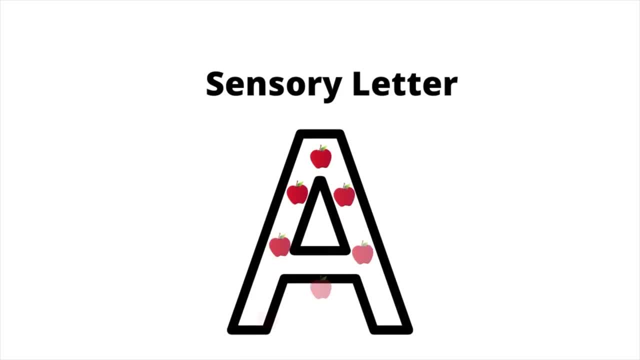 don't jump on the bed, shake your head. no, no, no, no, no. I have a big letter a now. no, no, no, no. I have a big letter a now. no, no, no, no. I have a big letter a now. can you help me glue some little apples? 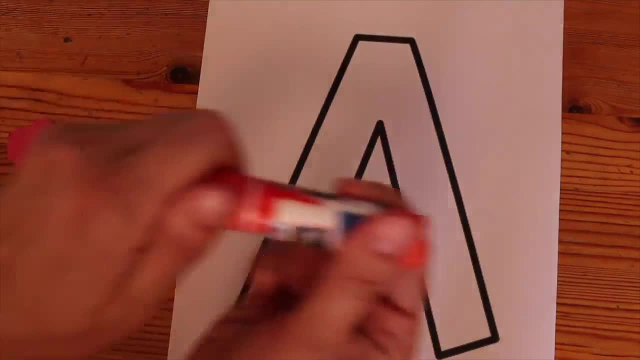 can you help me glue some little apples? can you help me glue some little apples onto it? be so much fun. okay, let's get onto it, be so much fun. okay, let's get onto it, be so much fun. okay, let's get out our glue stick. we put glue on the. 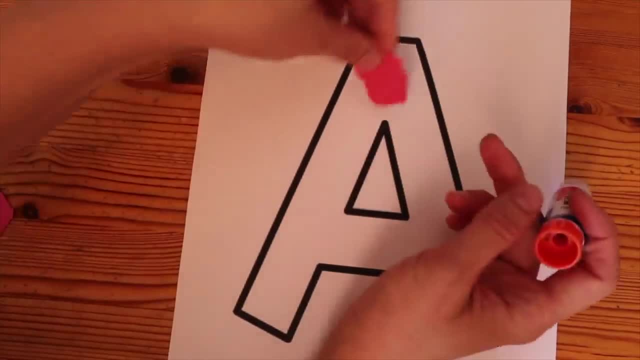 out our glue stick. we put glue on the out our glue stick. we put glue on the apple see. and then we put it on a Wow, apple see. and then we put it on a Wow, apple see. and then we put it on a Wow, that was fun, take a little apple, put on. 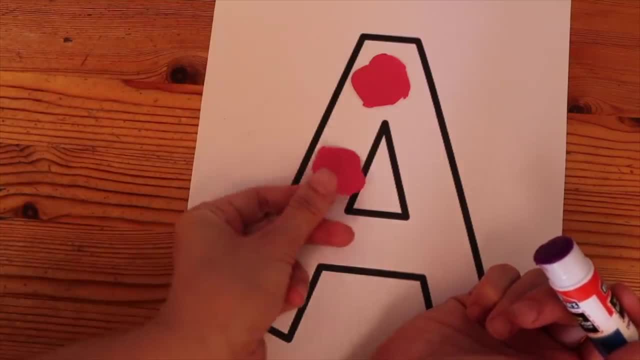 that was fun. take a little apple put on, that was fun. take a little apple put on the glue, say on and I'll stick it on. on the glue, say on and I'll stick it on. on the glue, say on and I'll stick it on on. Wow, this a is getting covered in apples. 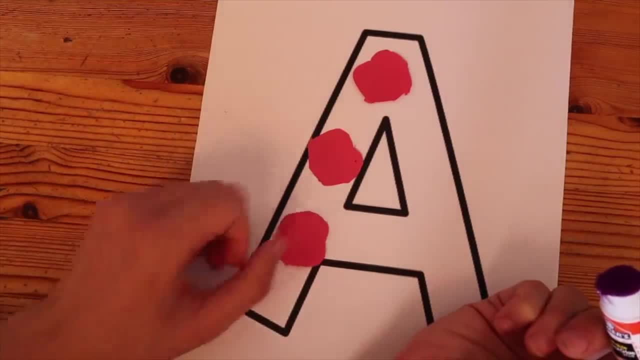 Wow, this a is getting covered in apples. Wow, this a is getting covered in apples. the glue is purple, Wow, and then I stick. the glue is purple, Wow, and then I stick. the glue is purple, Wow, and then I stick it on. can you help me with this one put? 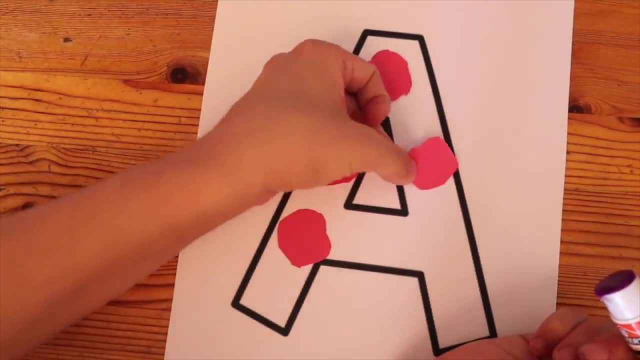 it on. can you help me with this one? put it on. can you help me with this one? put on the glue and then say on on the glue and then say on on the glue and then say on on: good job. Wow, I think the a is so happy to have. 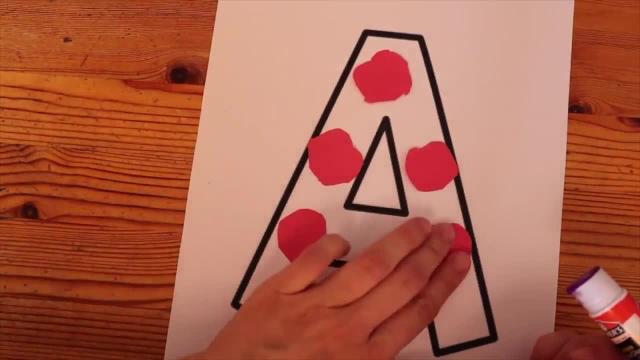 on the glue and then say on on good job, Wow, I think the a is so happy to have on the glue and then say on on good job, Wow, I think the a is so happy to have all these awesome apples on it on. let's put all these awesome apples on it on. let's put. 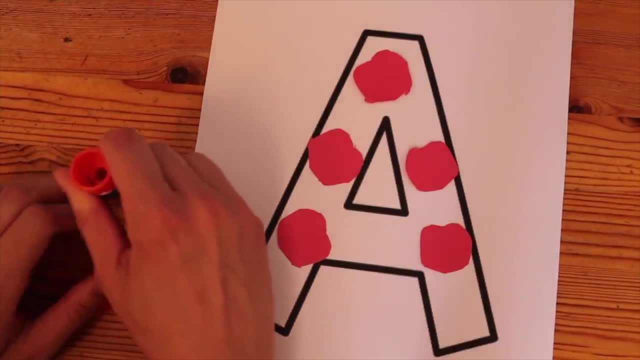 all these awesome apples on it. on, let's put one in the middle. can you help? you're one in the middle, can you help? you're one in the middle, can you help? you're such a good helper. I'm so happy to be such a good helper. I'm so happy to be. 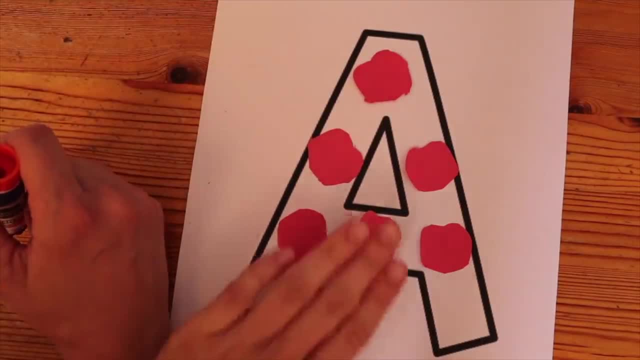 such a good helper. I'm so happy to be spending time with you on good job. you spending time with you on good job. you spending time with you on good job. you helped me say on and I'll put one right. helped me say on and I'll put one right. 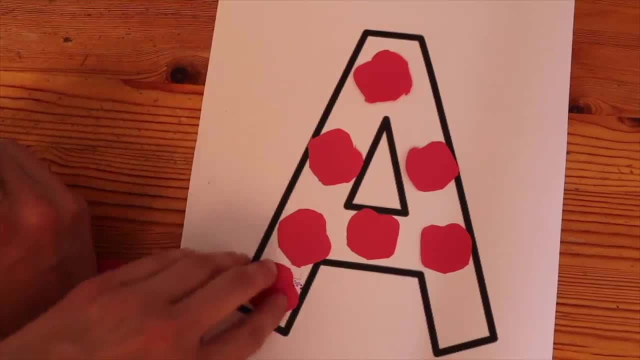 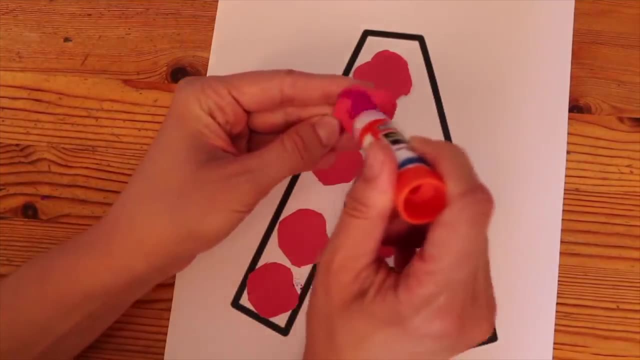 helped me say on and I'll put one right here on good job. see how I put the glue here on good job. see how I put the glue here on good job. see how I put the glue on. yeah, fill it with glue so it sticks on. yeah, fill it with glue so it sticks. 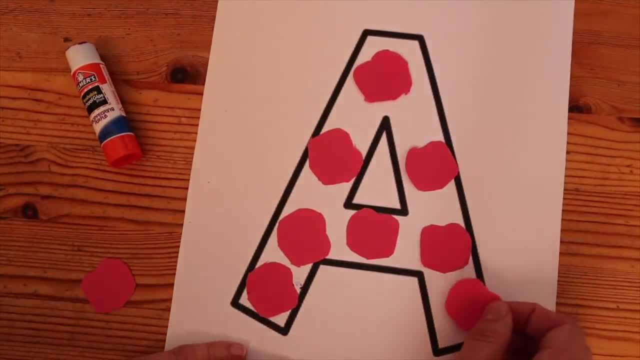 on. yeah, fill it with glue so it sticks, put it on, put it on. put it on, Wow, put it on. put it on. put it on, Wow, put it on, put it on, put it on, Wow. friends, look what you helped me make I'm friends. look what you helped me make I'm. 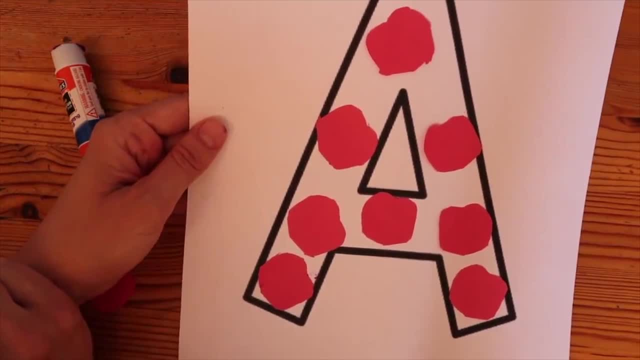 friends, look what you helped me make. I'm so proud of you. we made it a with apples. so proud of you. we made it a with apples. so proud of you. we made it a with apples stuck all over it so awesome. stuck all over it, so awesome. 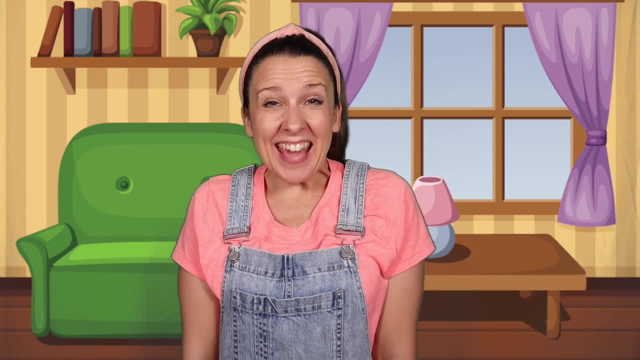 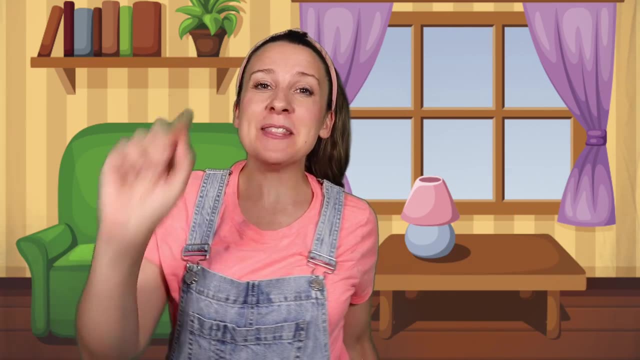 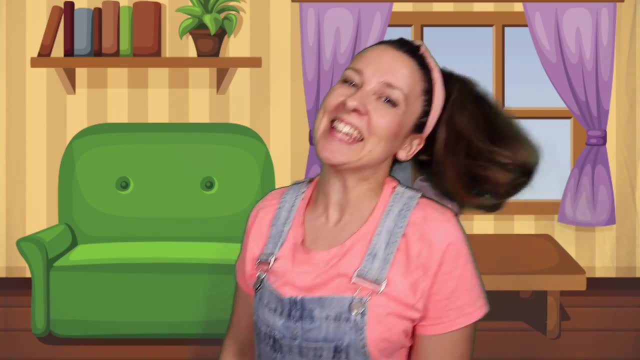 struck one, the mouse went down. hickory struck one, the mouse went down. hickory, dickory duck, let's do it again. that was dickory duck, let's do it again. that was dickory duck, let's do it again. that was so much fun. let me hear you sing hickory. 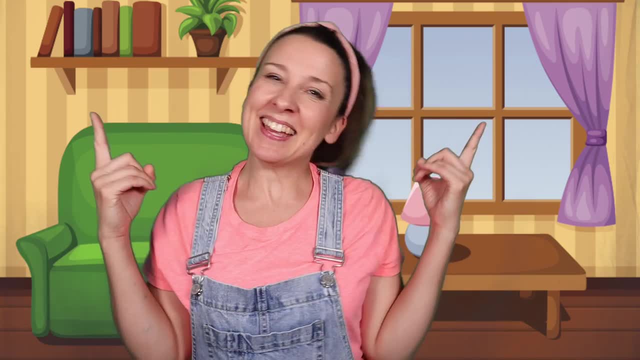 so much fun. let me hear you sing hickory. so much fun, let me hear you sing hickory. dickory dock. the mouse went up the dickory dock. the mouse went up the dickory dock. the mouse went up the clock. the clock struck one, the mouse went. 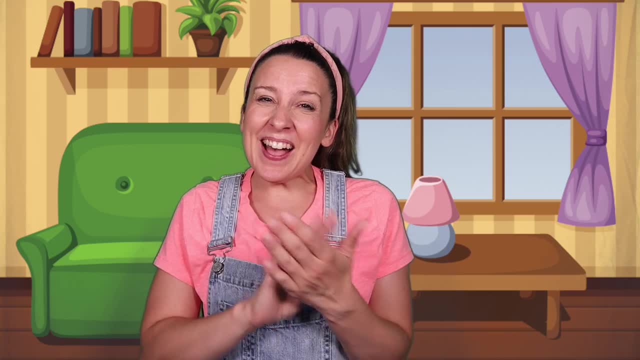 clock. the clock struck one. the mouse went. clock the clock struck one, the mouse went down. hickory dickory dock, great job down. hickory dickory dock, great job down. hickory dickory dock, great job. now you fill in the words hickory. 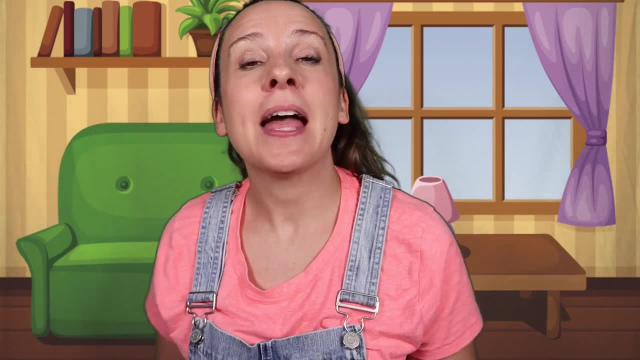 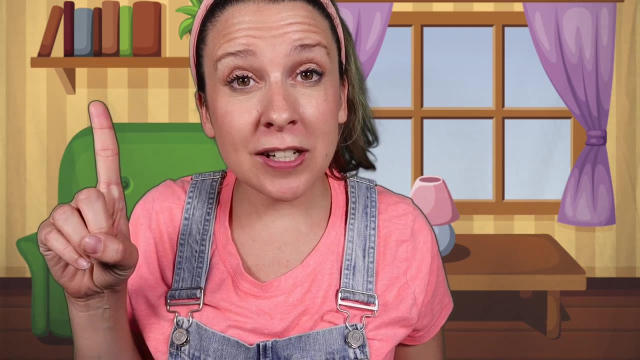 now you fill in the words hickory. now you fill in the words hickory, dickory, dock, dickory, dock, dickory, dock. the mouse went up the clock. the mouse went up the clock. the mouse went up the clock. the clock struck, the clock struck. 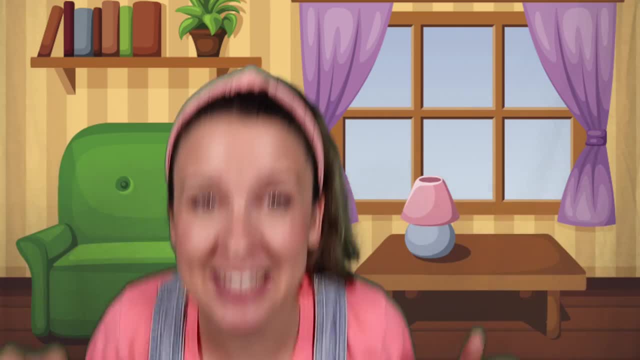 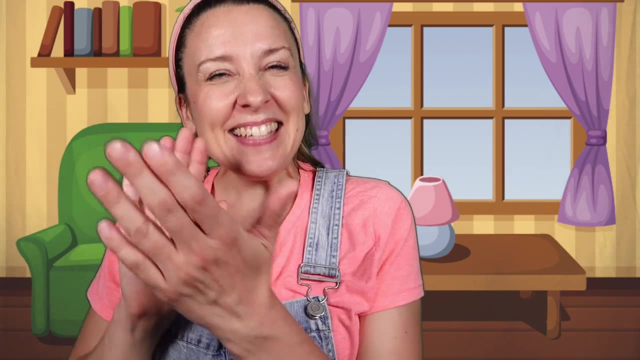 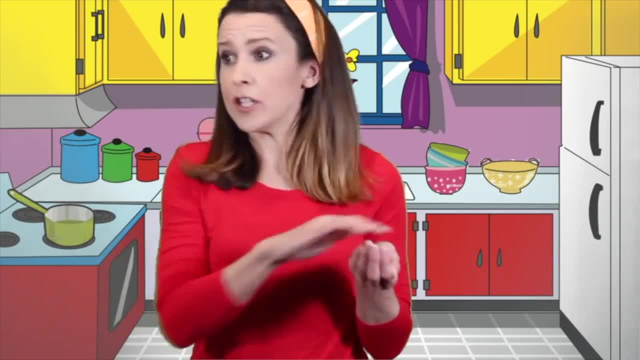 dock, yay, wow, dock, yay, wow. five little hot dogs frying in a pan. five little hot dogs frying in a pan. five little hot dogs frying in a pan. the grease got hot and one went. the grease got hot and one went. the grease got hot and one went. damn, how many are left? one, two. 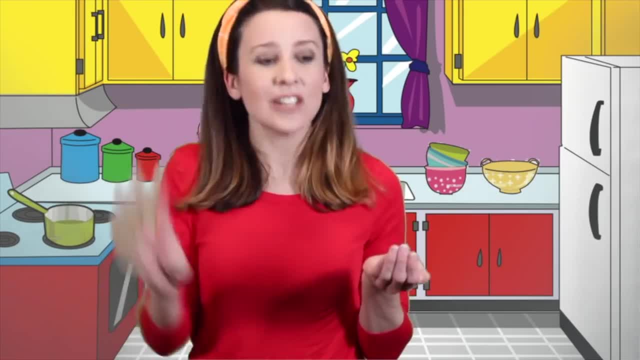 damn how many are left: one, two. damn how many are left: one, two, three, four, four little hot dogs: three, four, four little hot dogs. three, four, four little hot dogs frying in a pan. the grease got hot. frying in a pan, the grease got hot. frying in a pan. the grease got hot and one went damn. 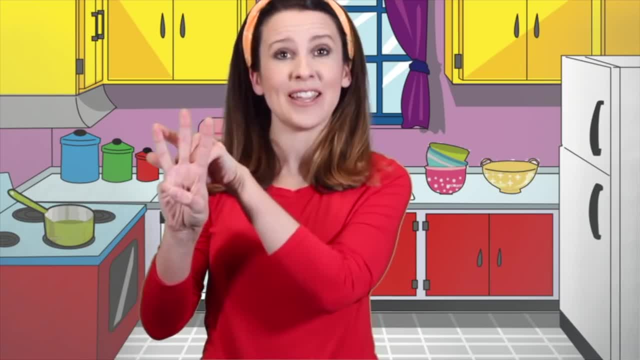 and one went damn, and one went damn. how many are left one, two, three? how many are left one, two, three? how many are left one, two, three, three little hot, three little hot dogs, three little hot dogs. frying in a pan, the grease got hot. frying in a pan, the grease got hot. 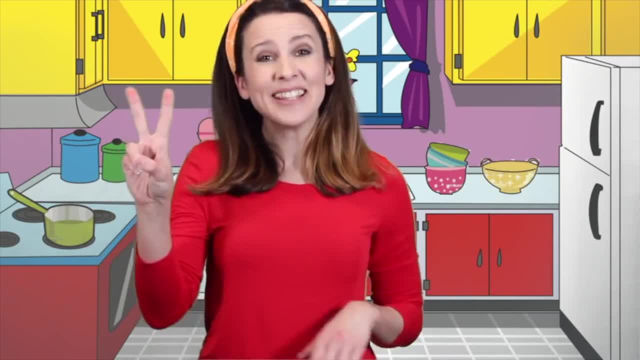 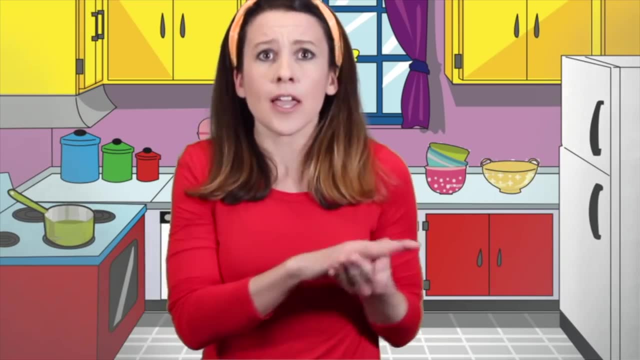 frying in a pan. the grease got hot, and one went damn, and one went damn and one went damn. how many left one, two, two little hot? how many left one, two, two little hot? how many left one, two, two little hot dogs frying in a pan? the grease got hot. 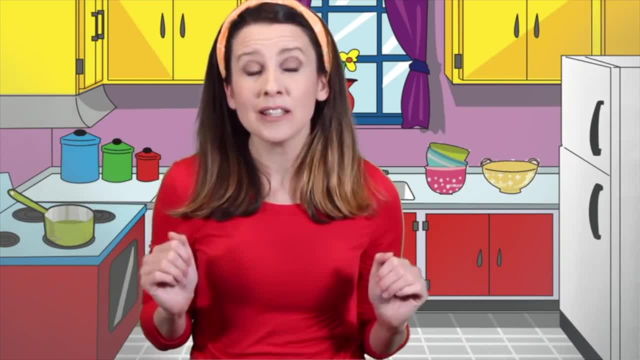 dogs frying in a pan. the grease got hot dogs frying in a pan. the grease got hot and one went and one went and one went. how many left just one little hot dog? how many left just one little hot dog? how many left just one little hot dog? one little hot dog frying in a pan? the 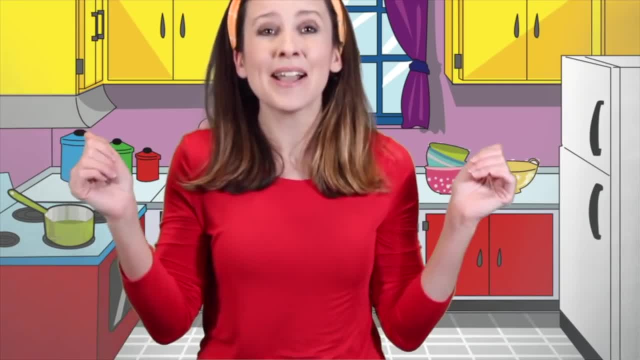 one little hot dog frying in a pan. the one little hot dog frying in a pan. the grease got hot and one went. grease got hot and one went. grease got hot and one went. how many are left? there's no. how many are left? there's no. how many are left? there's no hot dogs left and i'm so hungry, okay. 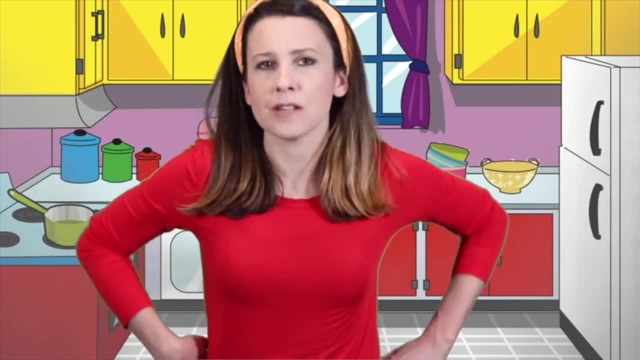 hot dogs left and i'm so hungry. okay, hot dogs left and i'm so hungry, okay. so this time we're gonna do it with the. so this time we're gonna do it with the. so this time we're gonna do it with the pan going bam and it's gonna be the. 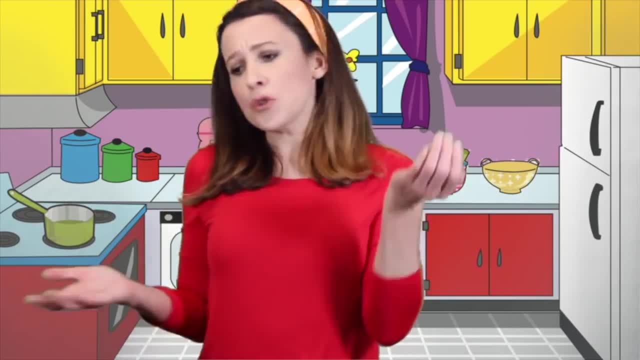 pan going bam, and it's gonna be the pan going bam, and it's gonna be the biggest bam yet. biggest bam, yet, biggest bam yet. no little hot dogs frying in a pan, no little hot dogs frying in a pan. no little hot dogs frying in a pan. the pan got hot and it went. 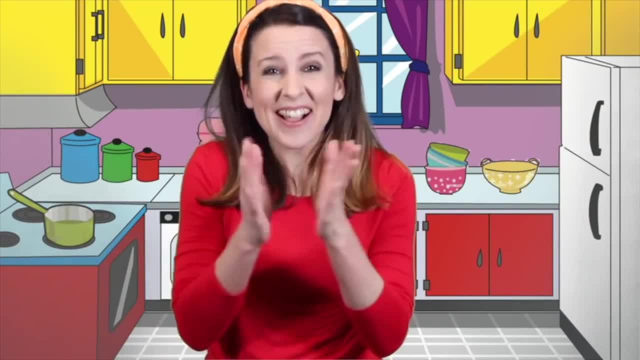 the pan got hot and it went. the pan got hot and it went: bam bam bam. great job, great job, great job. can you pretend your little thumb is a? can you pretend your little thumb is a? can you pretend your little thumb is a mouse, mouse, mouse, and then your other hand is going to be. 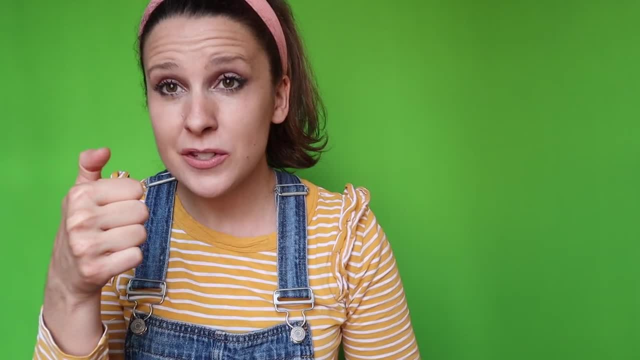 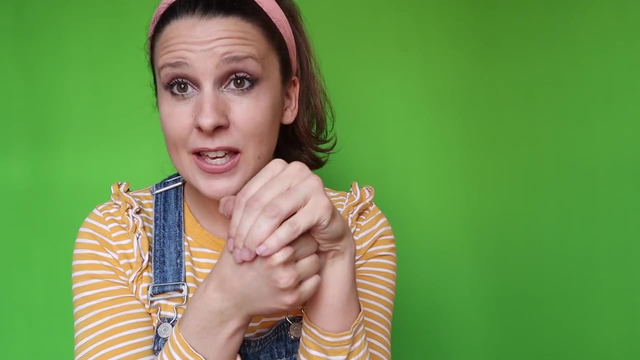 and then your other hand is going to be, and then your other hand is going to be: the house, the house, the house, a quiet little mouse, a quiet little mouse, a quiet little mouse in a quiet little house, in a quiet little house, in a quiet little house, when all was quiet as quiet can be. 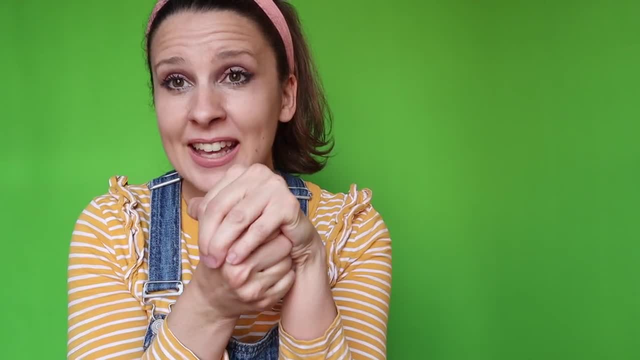 when all was quiet as quiet can be. when all was quiet as quiet can be, shh, shh, shh. alphatea, alphatea, alphatea. what a silly mouse. let's try that again. what a silly mouse. let's try that again. what a silly mouse. let's try that again. that was so silly. 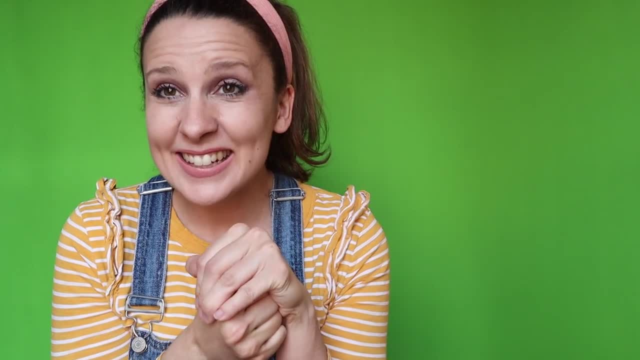 that was so silly. that was so silly, a quiet little mouse. a quiet little mouse. a quiet little mouse in a quiet little house, in a quiet little house, in a quiet little house, when woe was quiet, in a quiet little house, when woe was quiet in a quiet little house, when woe was quiet as quiet can be. 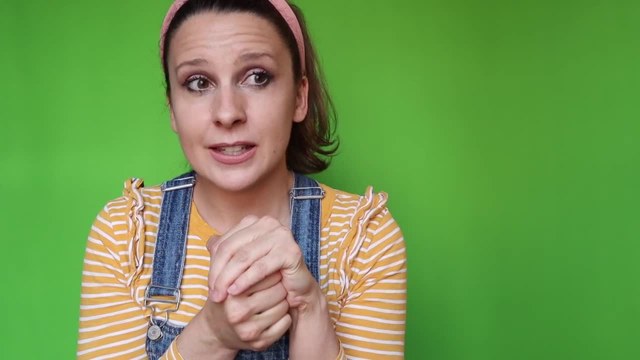 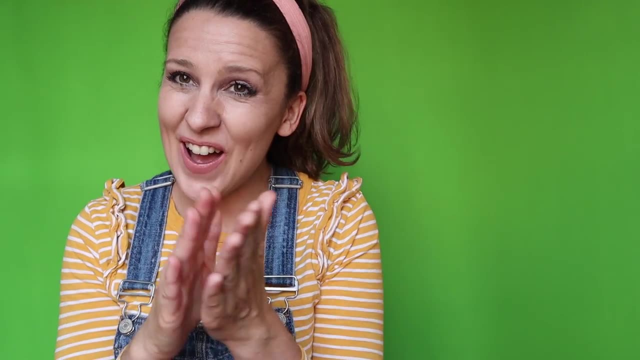 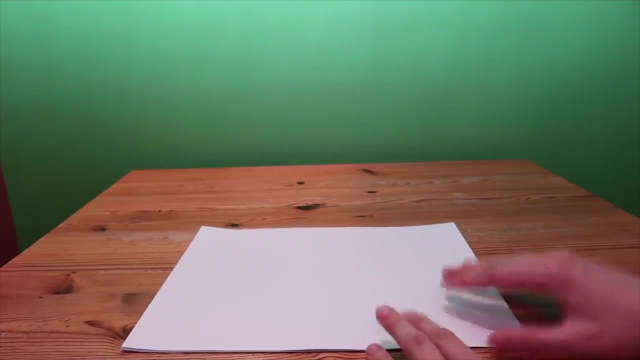 as quiet can be, as quiet can be, shh, shh, alpati, alpati, alpati. that was so silly, that was so silly, that was so silly. the little mouse surprised us. good job for circles around the house, for circles around the house, for circles around the house. and i noticed that 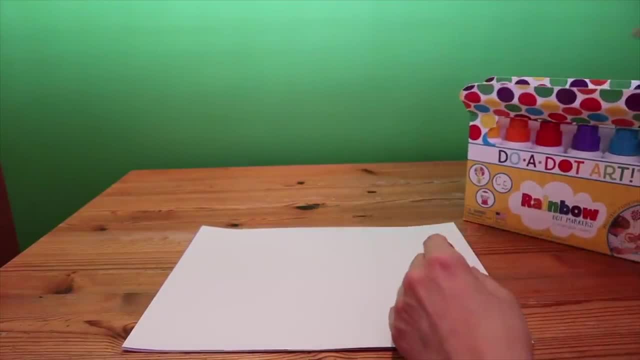 and i noticed that, and i noticed that these dot markers make circles. these dot markers make circles. these dot markers make circles. these are so fun. these are so fun. these are so fun. have you ever tried these? have you ever tried these? have you ever tried these? here's a. 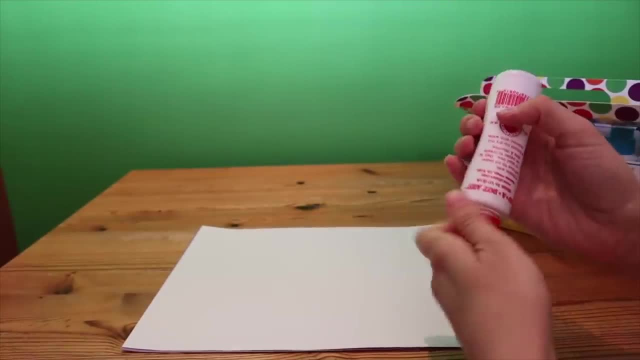 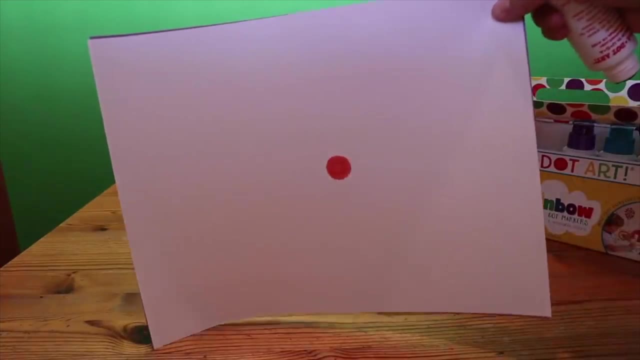 here's a. here's a. red color of the day. red color of the day, red color of the day. let's see if we can make a circle. let's see if we can make a circle. let's see if we can make a circle. yep, it made a circle. it's so cool. yep, it made a circle, it's so cool. yep, it made a circle, it's so cool. we could even make the letter of the day. we could even make the letter of the day. we could even make the letter of the day with our dots, with our dots. 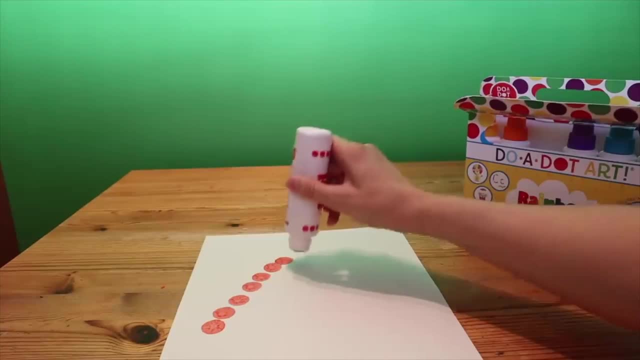 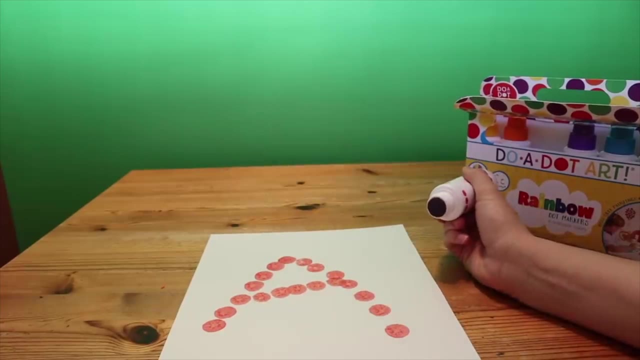 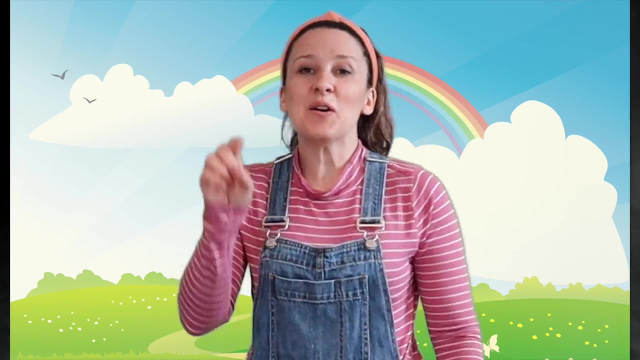 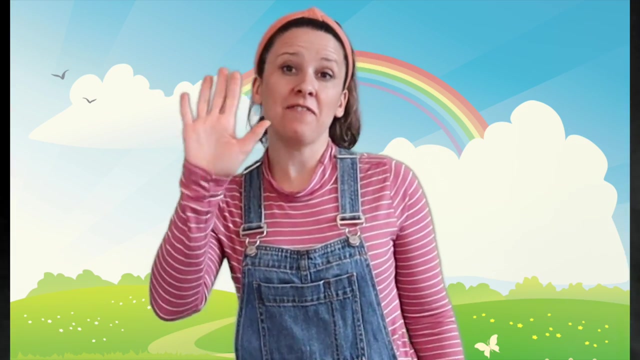 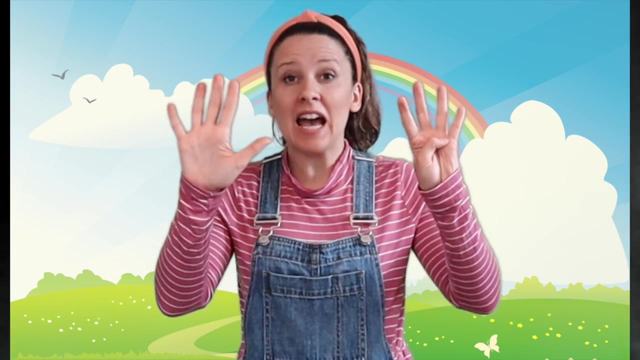 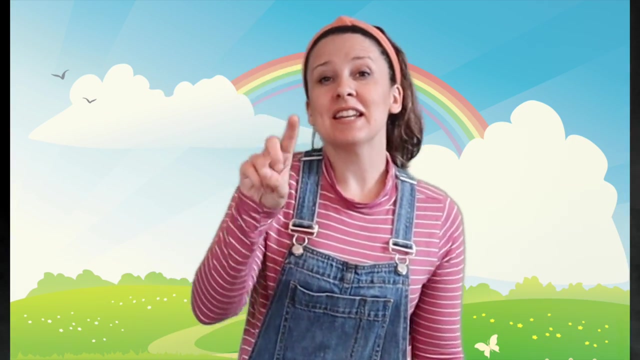 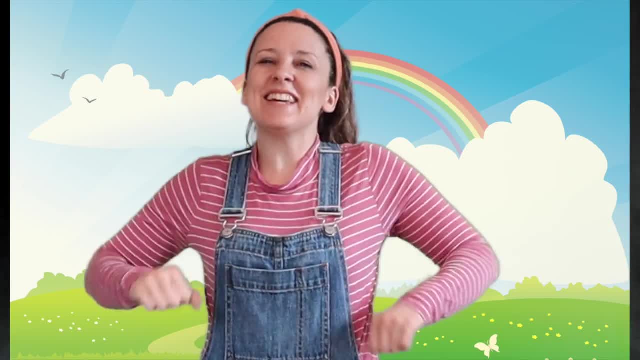 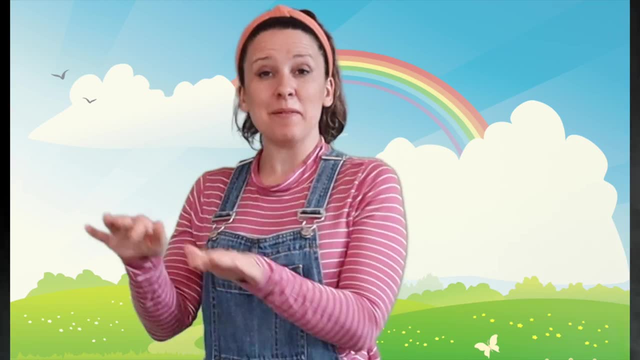 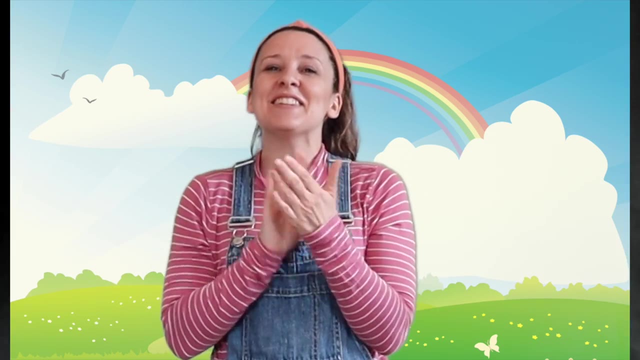 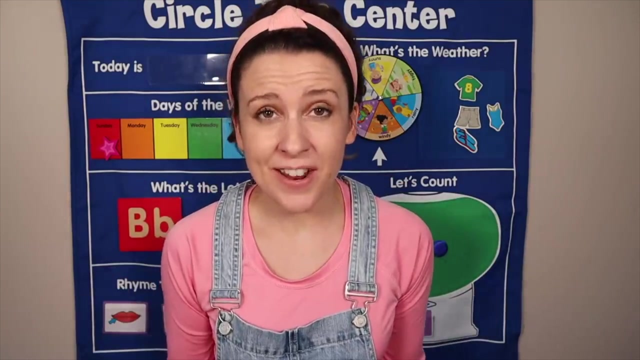 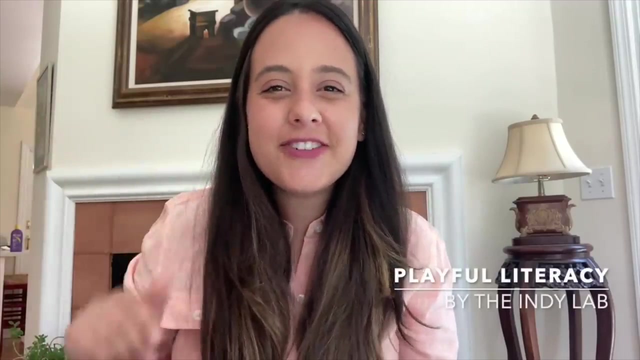 my shoe. Three, four, shut the door. Five, six, pick up sticks. Seven, eight, lay them straight. Nine, ten, a big red hand, Great job. Let's go see my friend Frida at Playful Literacy to learn more about the letter B. Hi everybody, Welcome to Playful Literacy. 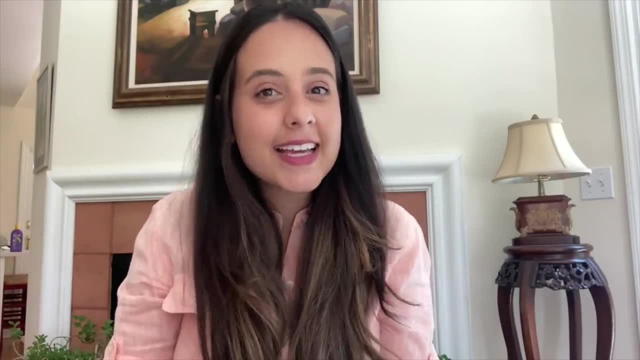 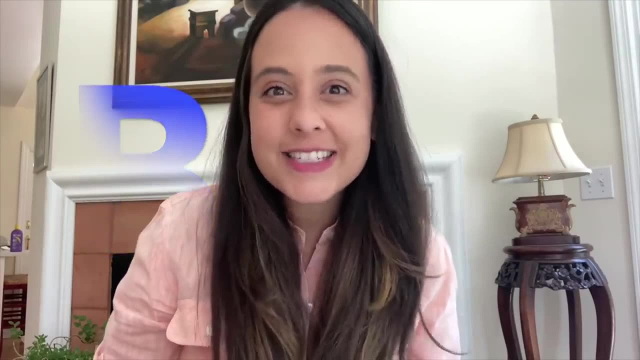 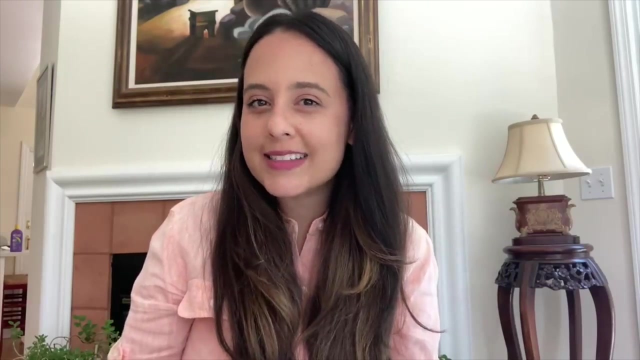 My name is Frida and I'm going to teach you the letter of the day. Today's letter is B. Do you know what sound B makes? That's right, the B sound. And in my class I like to act out my sounds. Do you want to act it out with me? Okay, ready, Here we go, Grab your two. 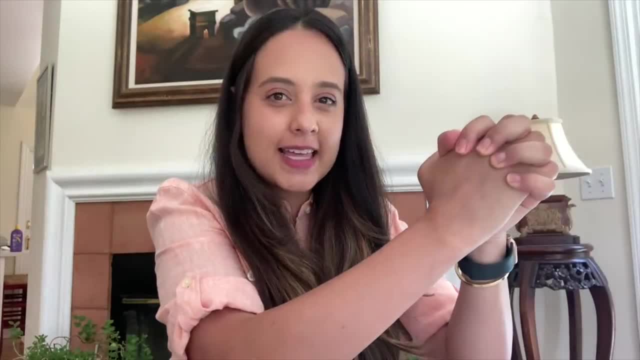 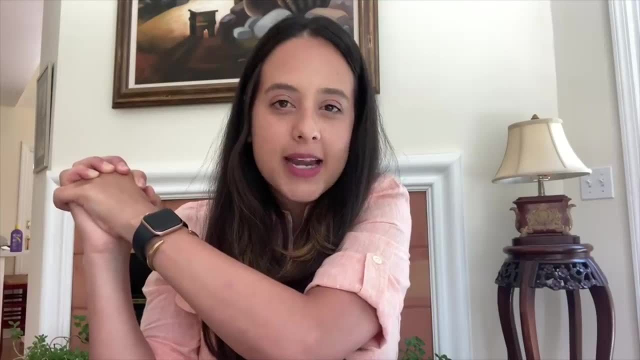 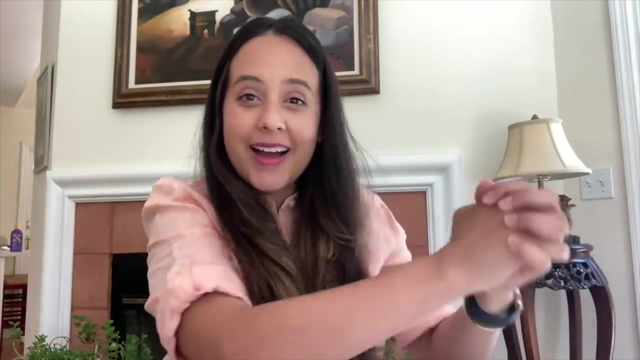 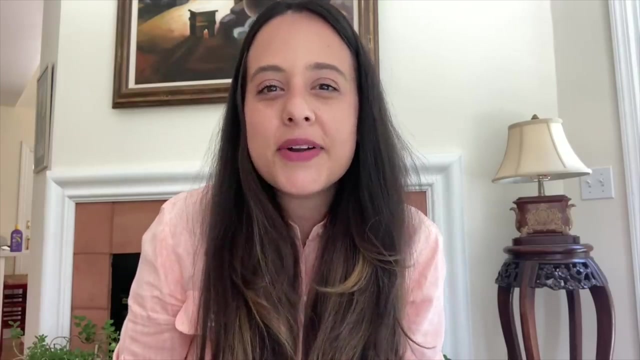 hands, Clasp them together just like this, And now, while they're holding hands, we're going to swing our arms around our body and make a B sound too. Here we go: B, B, B. Nice job, That's how I like to act out my B sound, so that I learn it a little bit easier Now. I 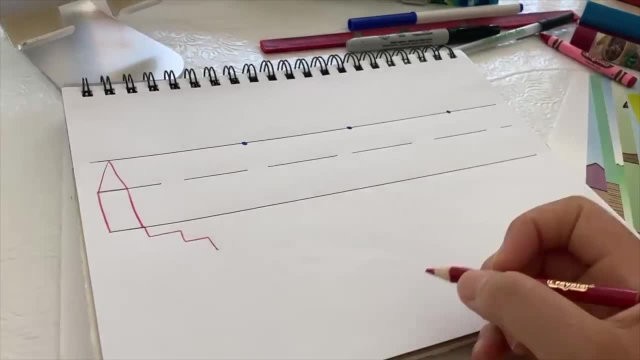 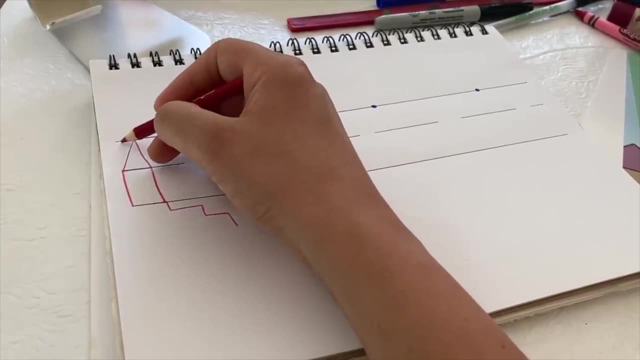 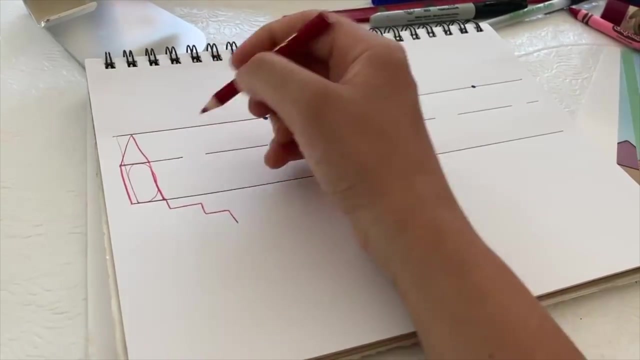 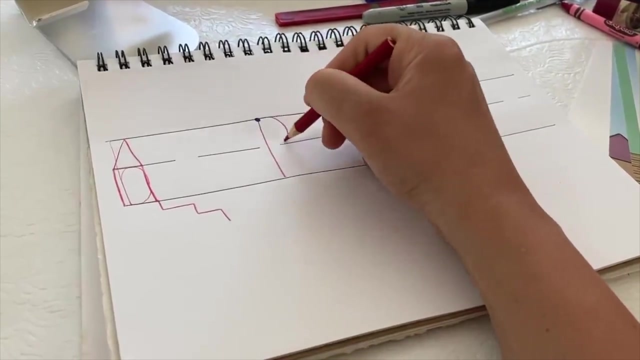 want to show you how you make the letter B. This is how I make my letter B. This is my house, And my lowercase letters go inside my house, just like this, And my uppercase letters, they can go to the top of my house, just like this. I make a line and then a. 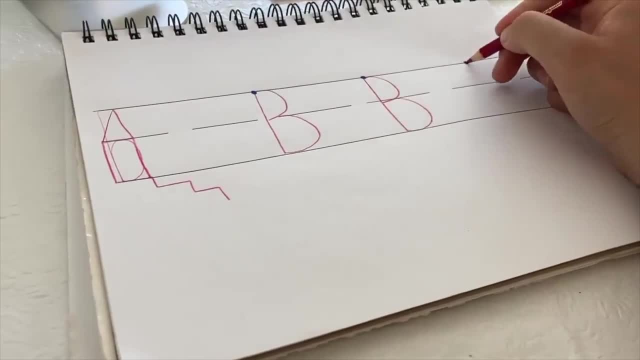 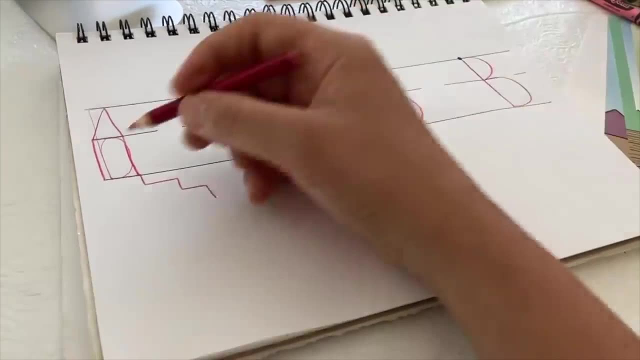 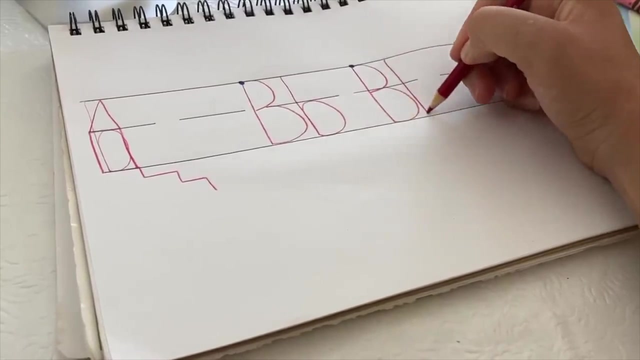 bubble and then a belly. I make a line and then a belly. I make a line and then a belly. And if I want to add my lowercase b, I make a line and a belly. I make a line and a. 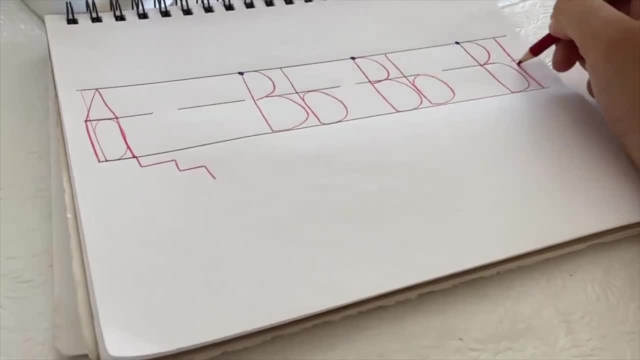 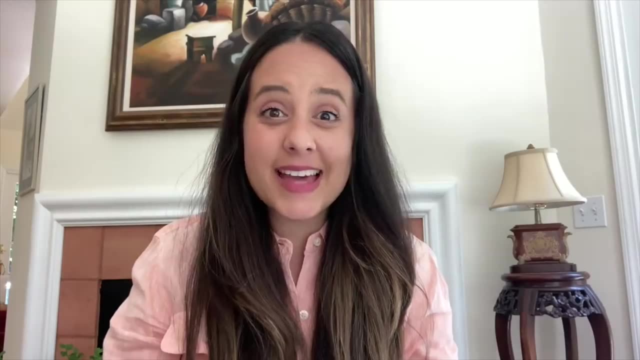 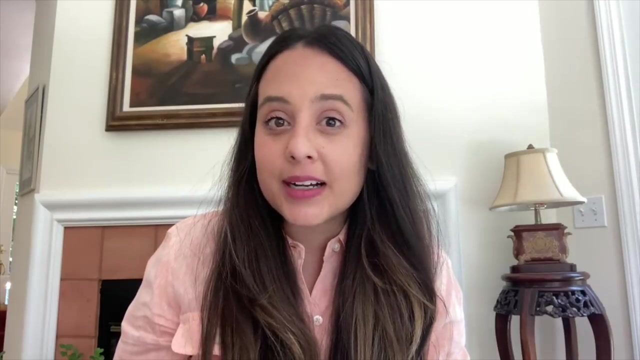 belly. I make a line and a belly. One of my favorite things to do when I have my sound of the day is to see how many words I can come up with with that sound. Today's sound is B, So let's see if my pictures have the sound we're looking for. Let's start with. 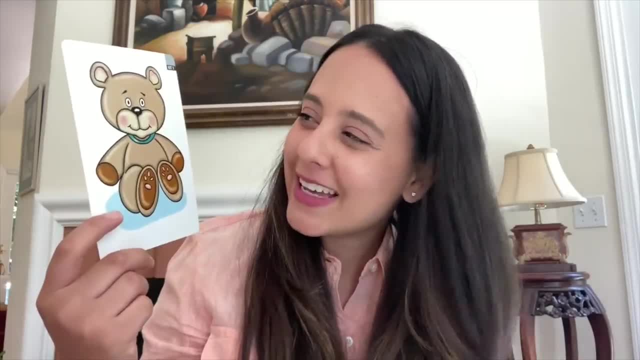 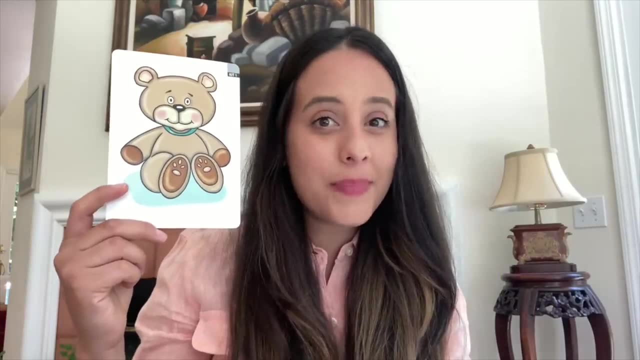 this one. Oh my gosh, he's so cute. What is it? That's right, guys, It's a bear, B bear. Do you hear the B sound that? we're looking for Me too? Good work, Let's look at my next. 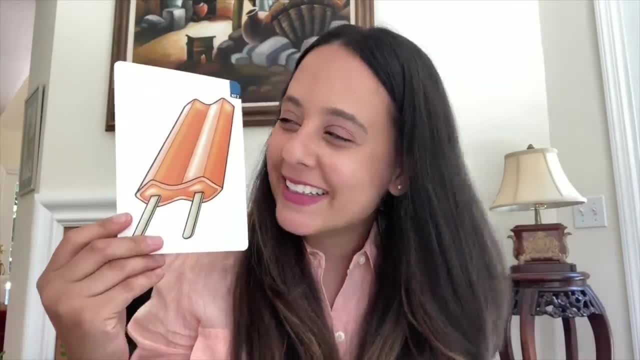 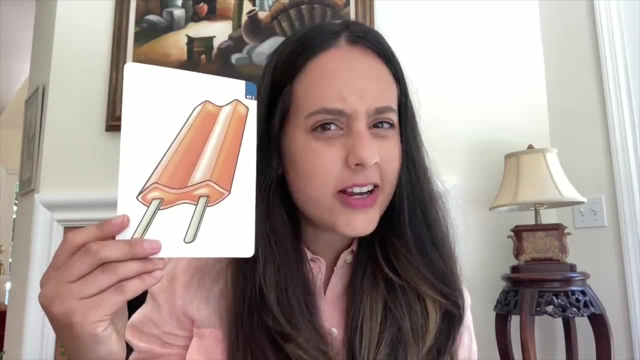 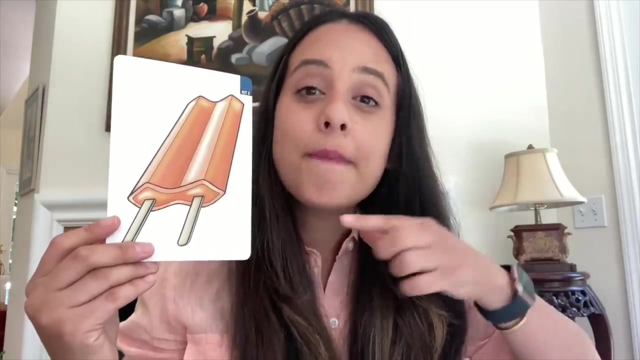 picture: Yummy, It's a popsicle. Do you hear the B Sound in popsicle? It's very close but it's actually kind of soft at the beginning. My lips come together but my voice is not on, so it's a different sound: Popsicle, There's. 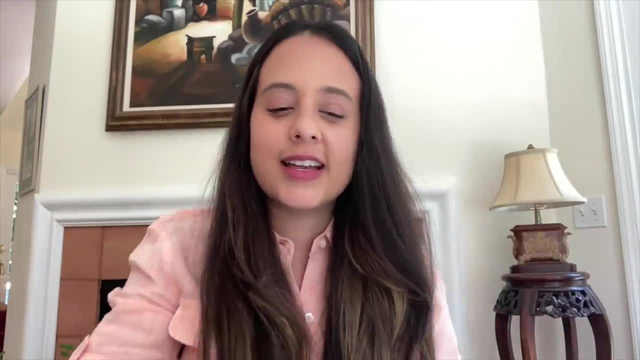 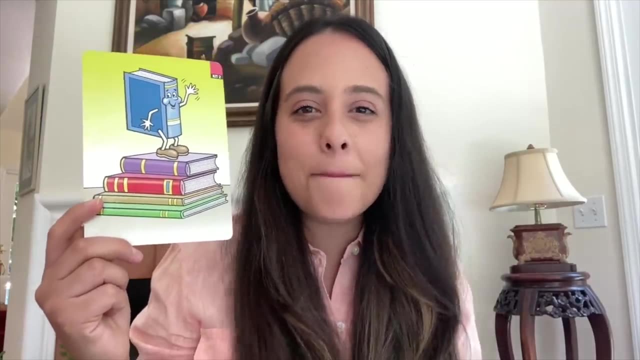 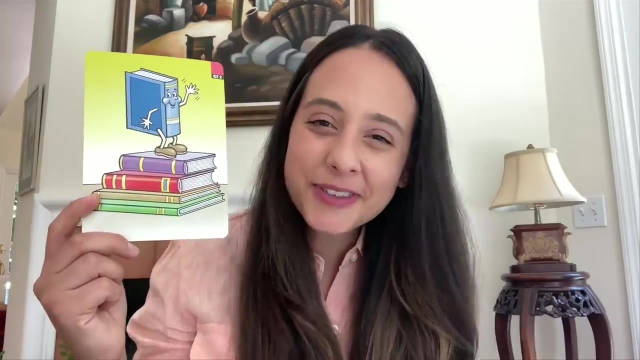 no B in that word. Let's put it over here Now. let's look at this one. What is this, everyone? It's a book, B for book. Do you hear the B sound? Me too. Nice work, Let's put it over here Now. we have two pictures with our P sound. 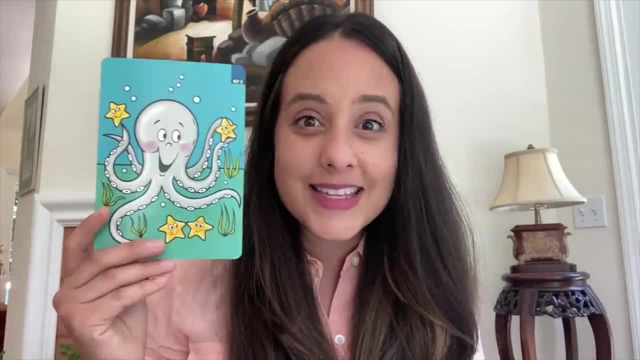 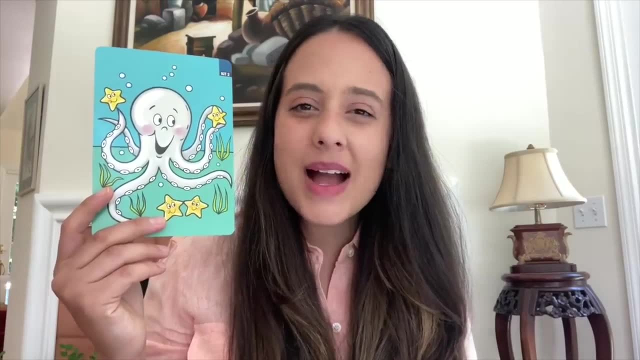 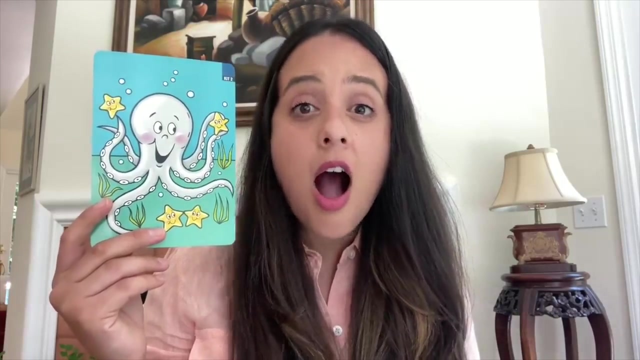 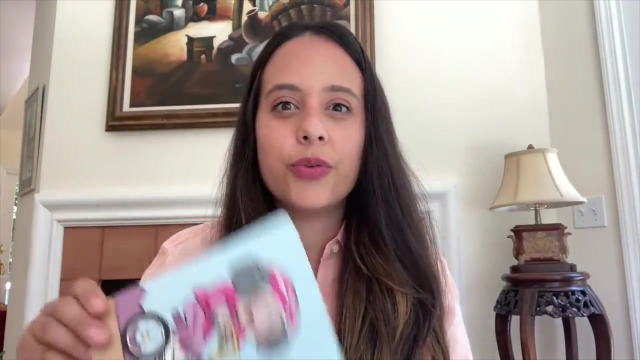 Let's do another one. What's this ocean animal? An octopus? Wait a second. My lips didn't come together for octopus. Actually my mouth got really big and open. Octopus, That's not a, B, That's a different letter. Let's put him over here. Ooh, but this one, guys, what is the girl? 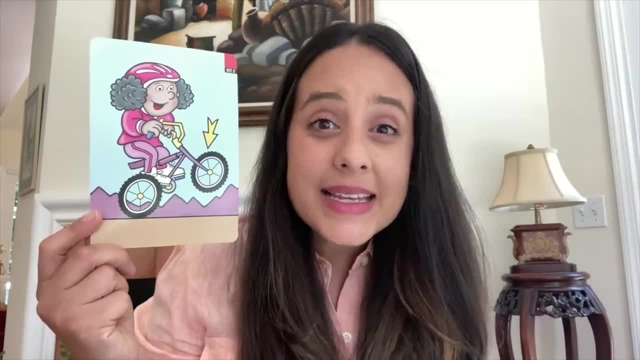 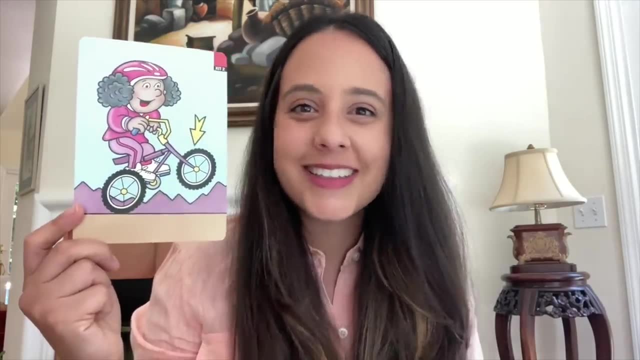 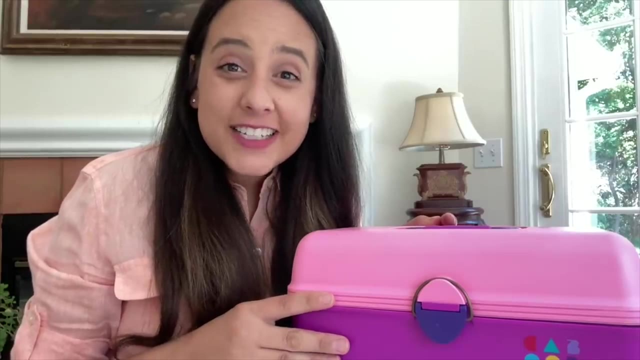 doing. She's riding her bicycle, Bike, B bike. I hear the B do you? That's right, guys, It's at the beginning of the word: Nicely done. One of my favorite activities to do is our sensory. 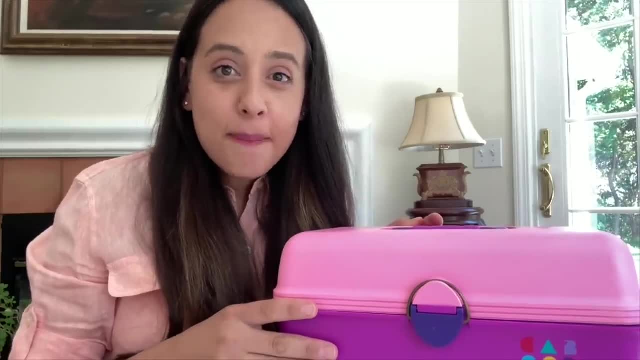 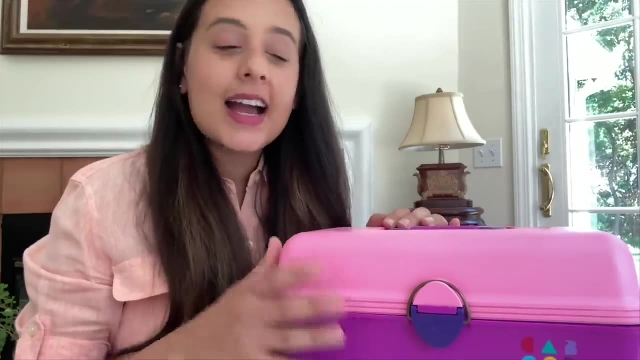 letters. Today we're going to make a B out of buttons. Now everybody has a bunch of buttons at their house somewhere. Go and find your buttons. I found mine in my kit and I want to open this up and show you all. 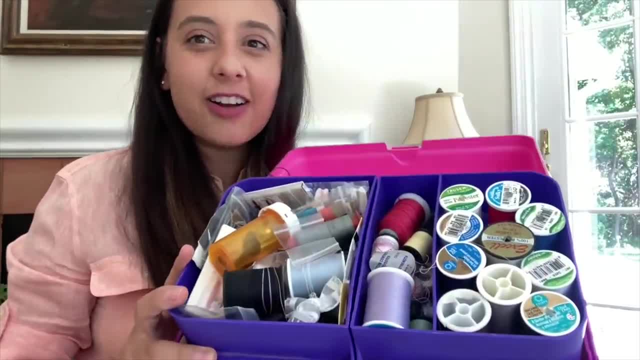 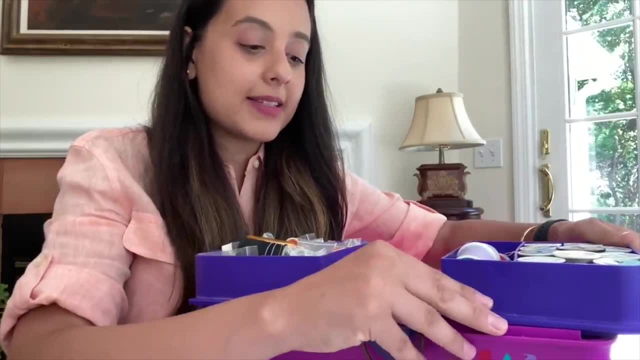 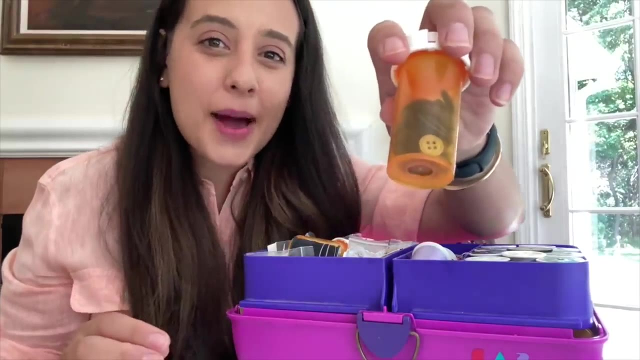 the things I have inside. Oh my gosh, look at all of this. A lot of things for sewing. Sewing is when we put clothes back together that have holes or where their zippers and snaps have broken, And here I found some buttons. Let's use these for our sensory letter. 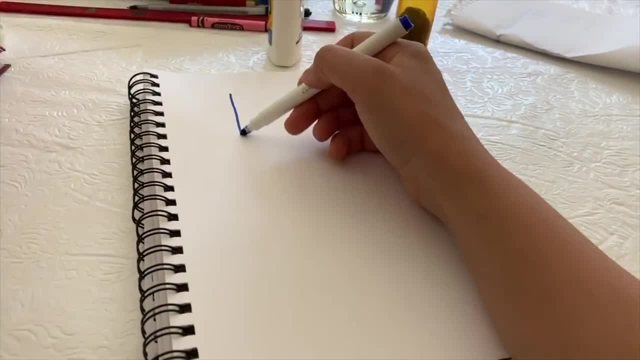 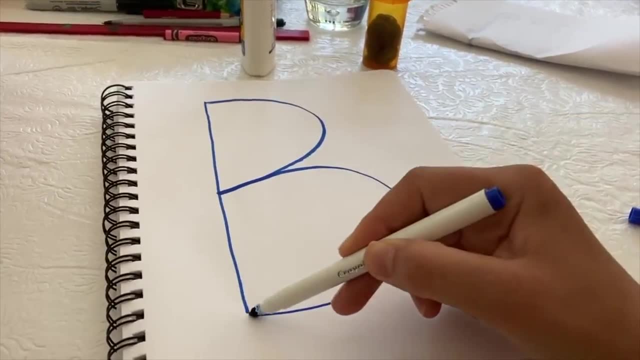 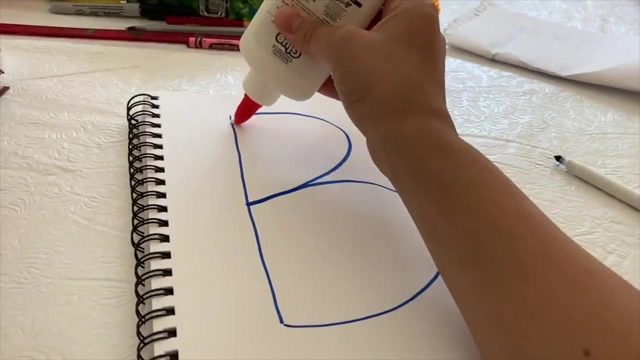 I'm going to make my letter B. Here's my big bubble and my belly. Now I'm going to take my glue and make my line and trace the bottom of my letter. I'll go ahead and do this. I'm going to make this: 1,2,3,4,5,6,7,8,9,10, 3,5,5,6,6,7,9,10. I'm going to make my letter B. Here is my big bubble and my belly. Now I'm going to take my glue and make my line and trace myソウ osu bb. Here's my big bubble and my belly. Now I'm going to take my glue and make my line and trace my belly. 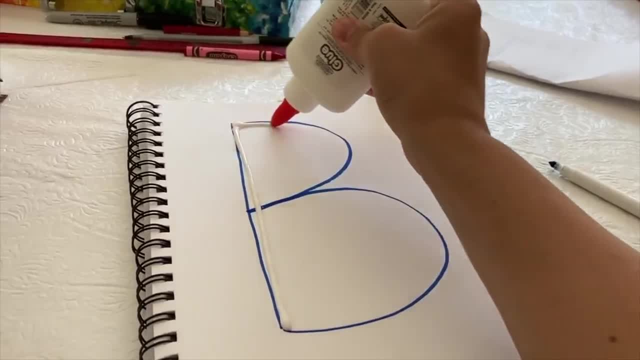 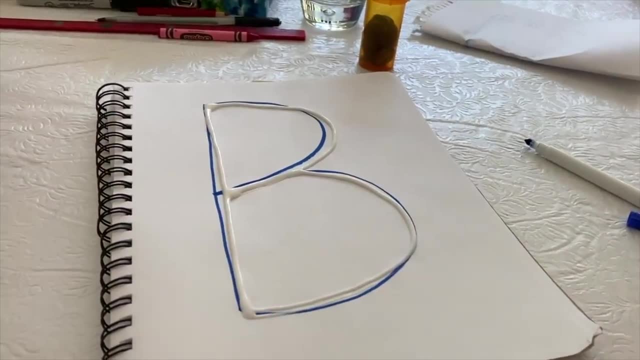 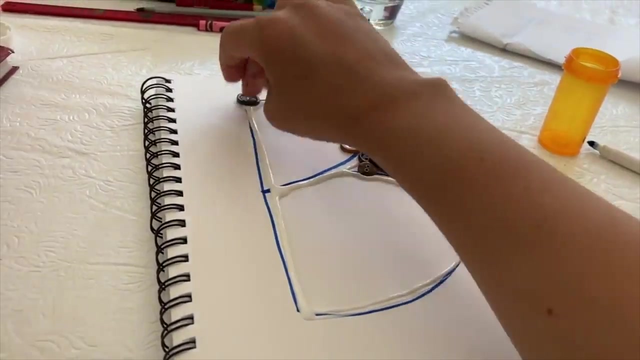 my letter. You can get your grown-up to make you a bee and you can use your glue to help trace the bubble and the belly. Now I'm going to take all of my buttons and I'm going to put them, starting from the top, all the way down my bee. I'm. 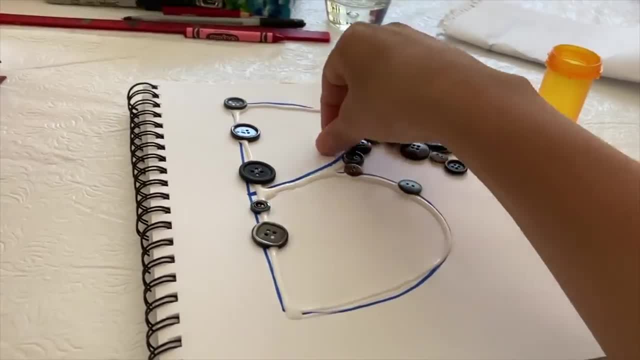 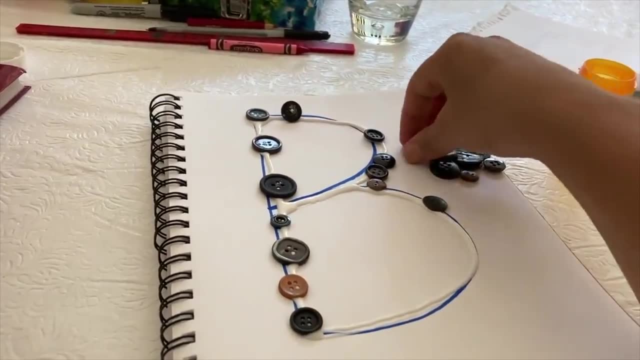 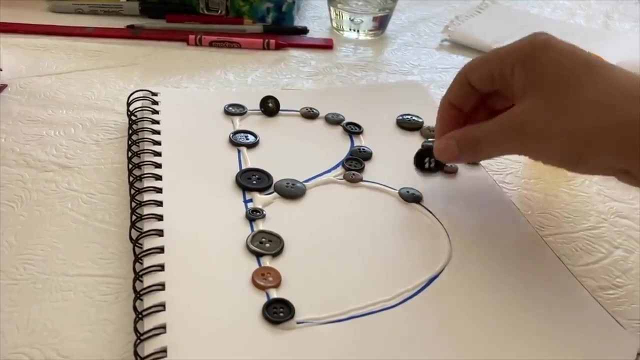 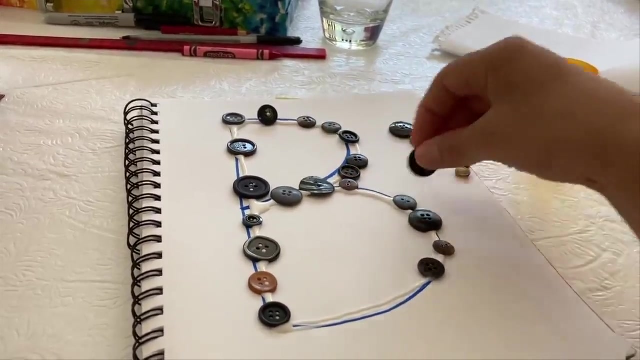 going to make a button bee. This is so much fun. Look at all of my buttons. There are so many kinds and I can put them all around my letter. Wow, I have big buttons and I have small buttons. Look at these tiny little ones. 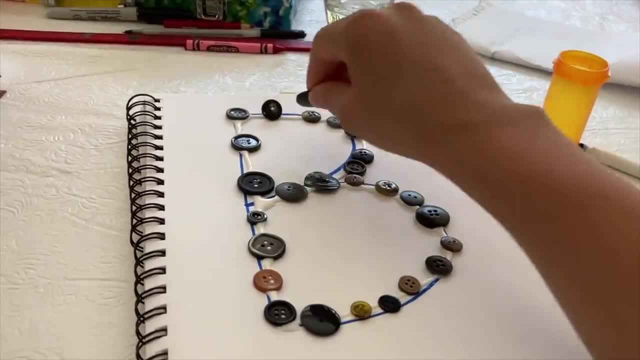 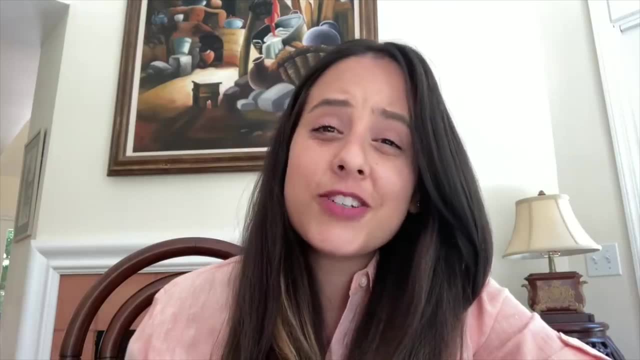 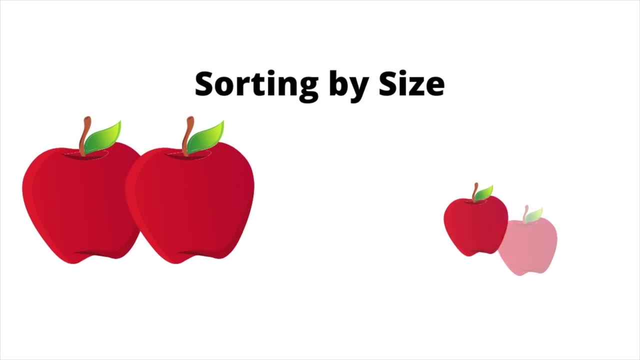 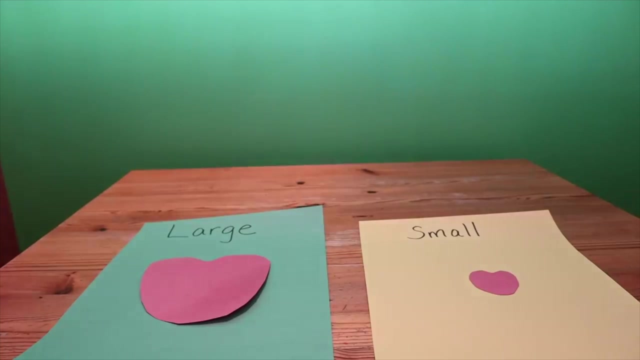 Wow, we made a button bee. I had so much fun learning all about the letter B with you today. Thanks for coming to Playful Literacy. Bye, It's time for a super fun game. Let's sort these apples by size. Okay, does this apple go with large or? 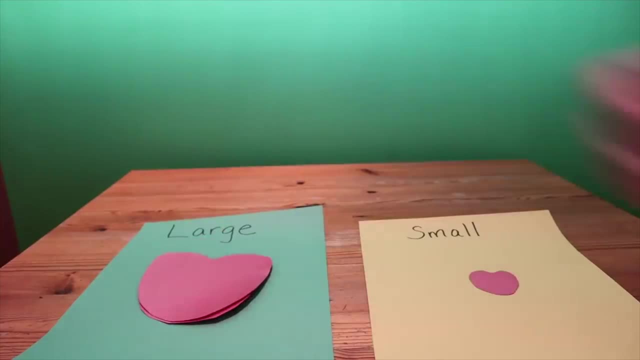 small, Large, Good job. How about this one? Large or small, Small, Good job. Large or small, Large, Good. Large or small, Small? Uh-oh, I'm not sure where this goes. Large or small, Small, Good job. 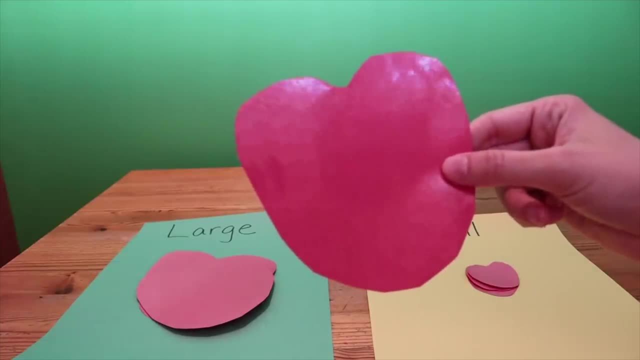 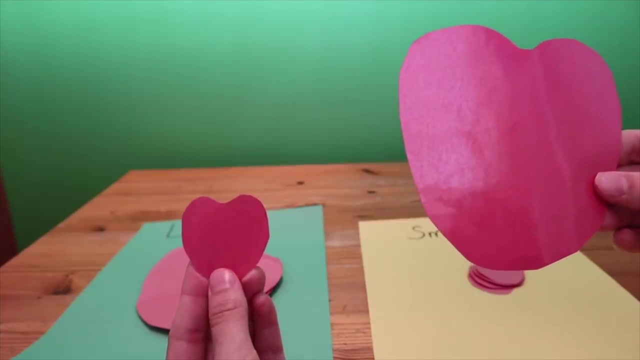 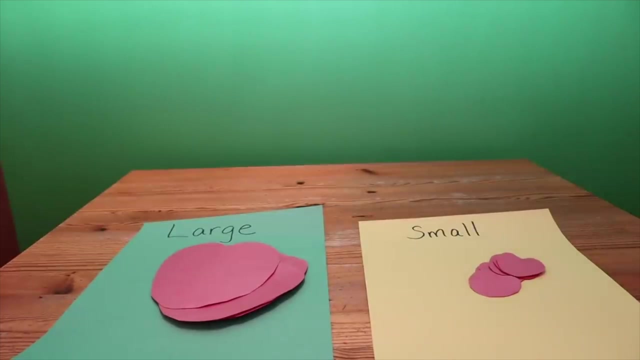 Large or small, Small, Large, Great work. What about the last two? Yeah, this is large and this is small. Yay, we did it. I'm so proud of you. Next, we're gonna get into our boat, So we're gonna get out our paddles. 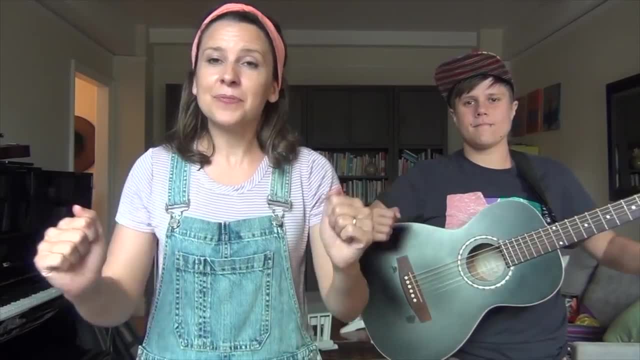 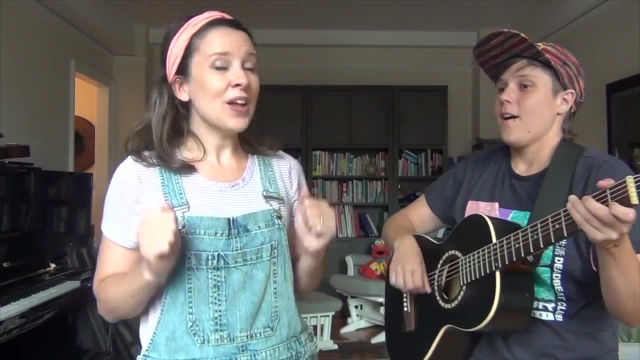 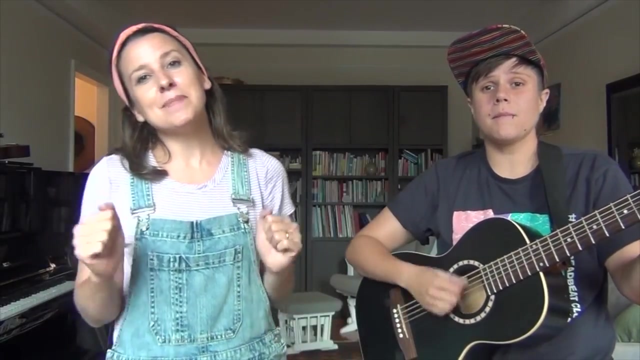 Let's pretend we're in a boat. Did you get out your paddles? And we're gonna row so nicely? and we're in a nice calm stream. What a beautiful day. Row, row, row your boat gently down the stream, merrily, merrily, merrily, merrily life. 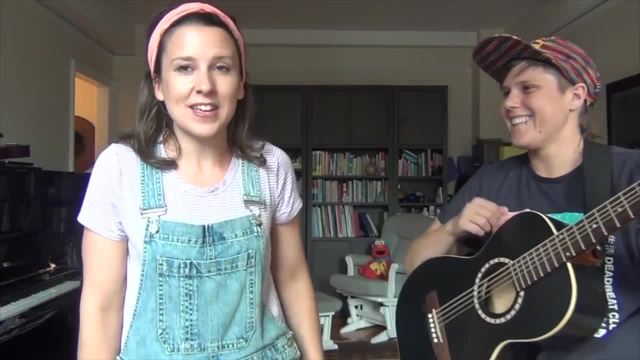 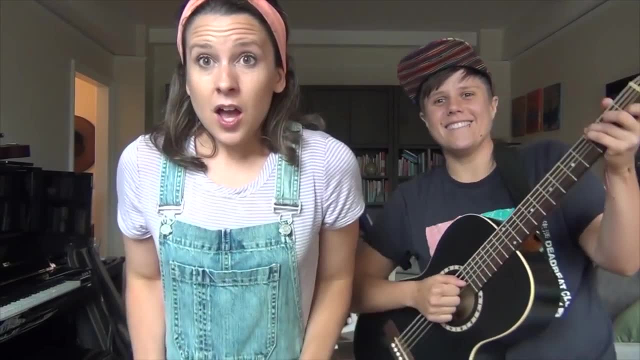 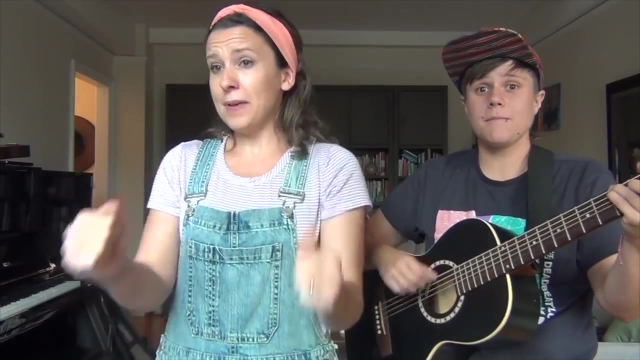 is but a dream. That was so nice and fun. This time we're gonna get in our boats again, but we're gonna pretend that we see a crocodile. Are you ready? Row, row, row your boat gently down the stream. If you see a crocodile, don't forget to scream. 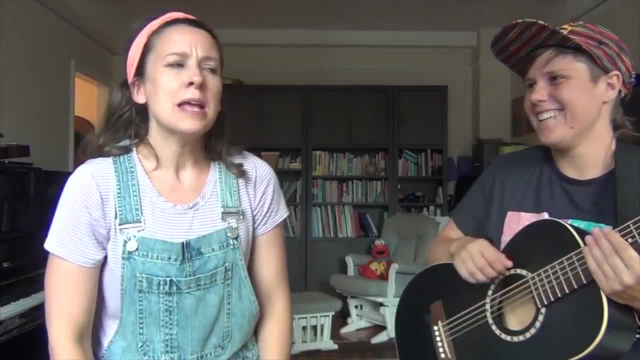 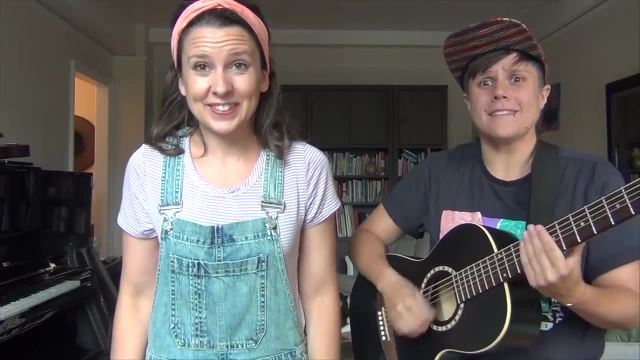 That was so fun. Maybe we should do a faster tempo because we want to get away from that crocodile. You ready? One, two, three, four Row row. row your boat Gently down the stream. If you see a crocodile, don't forget to scream. 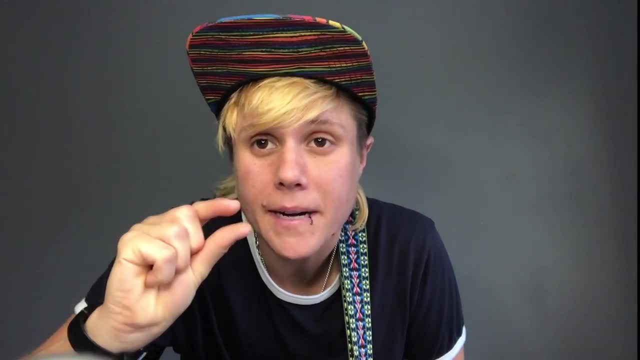 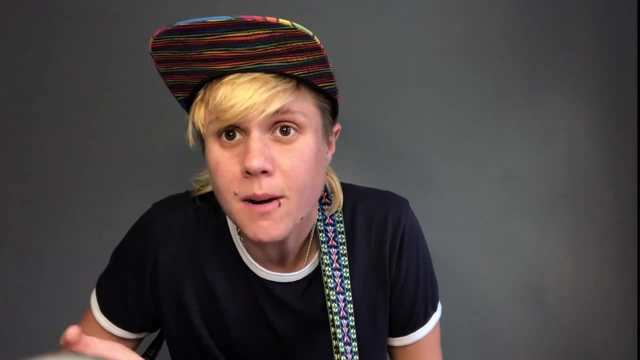 The next song we're going to sing is about a tiny little bug called an ant. We're going to sing a song about them marching and we're going to count them as they march. Can you march with me? Let's go, Here we go. 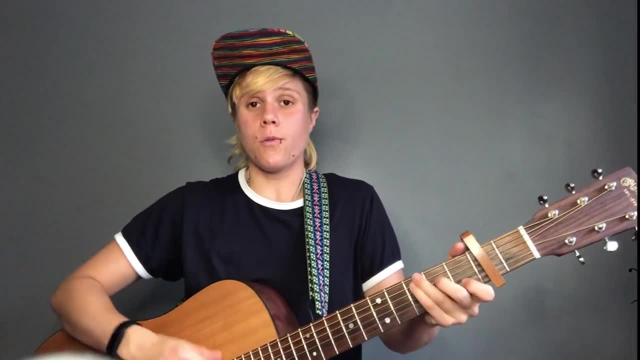 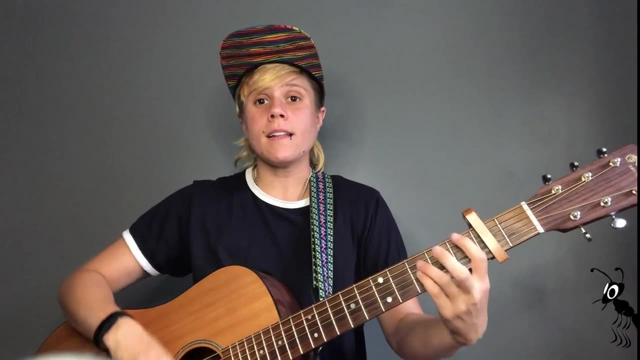 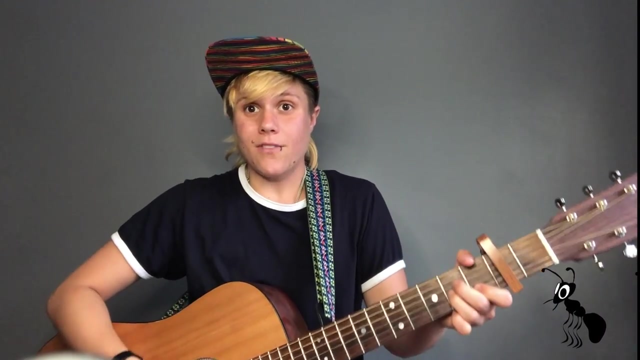 The ants go marching one by one. Hurrah, hurrah. The ants go marching one by one. Hurrah, hurrah. The ants go marching one by one. The little one stopped to suck his thumb and they all go marching Down to the ground to get out of the rain. Boom, boom, boom, boom, boom, boom, boom. 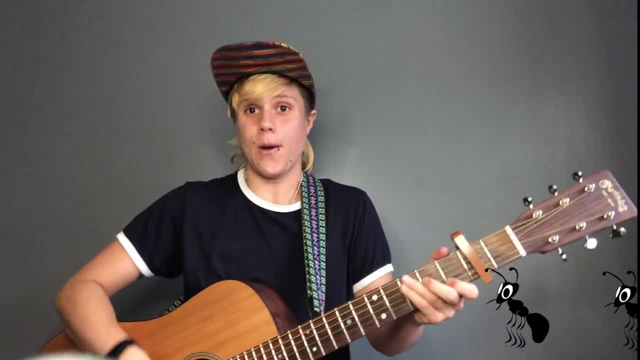 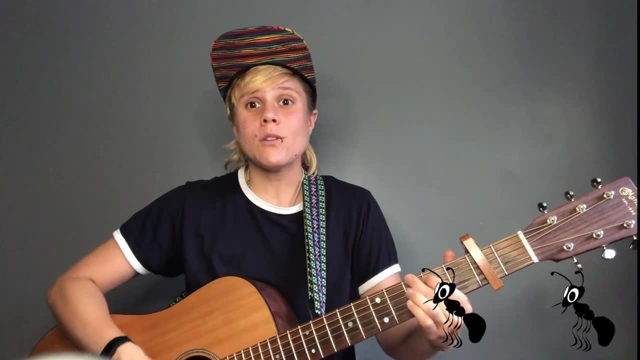 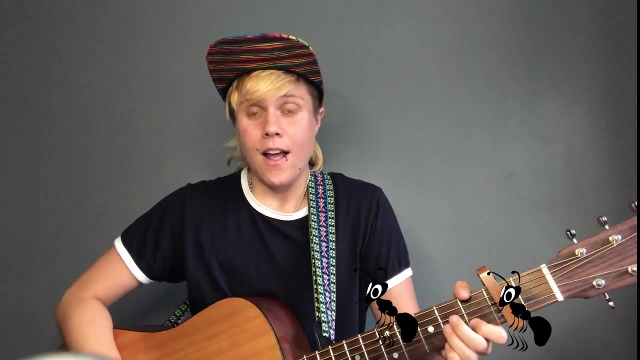 The ants go marching two by two. Hurrah, Hurrah. The ants go marching two by two. Hurrah, Hurrah. The ants go marching two by two. The little one stopped to tie his shoe and they all go marching down to the ground to get out of the rain. 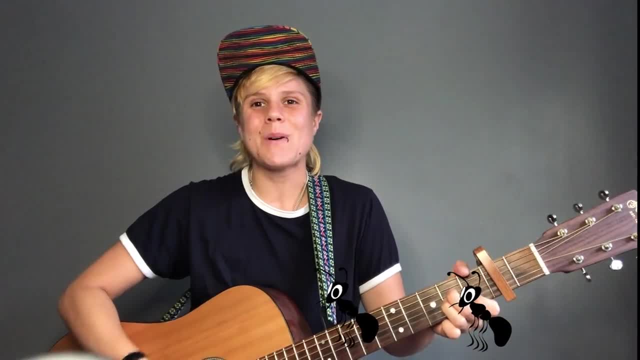 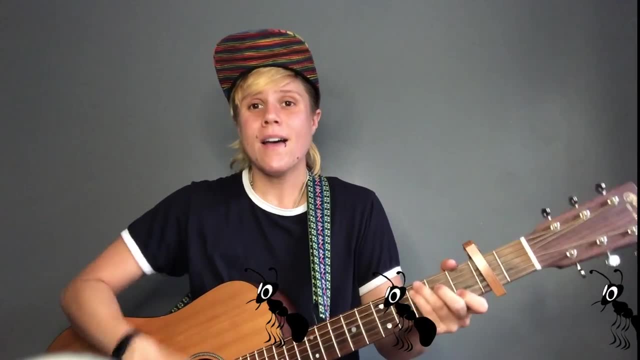 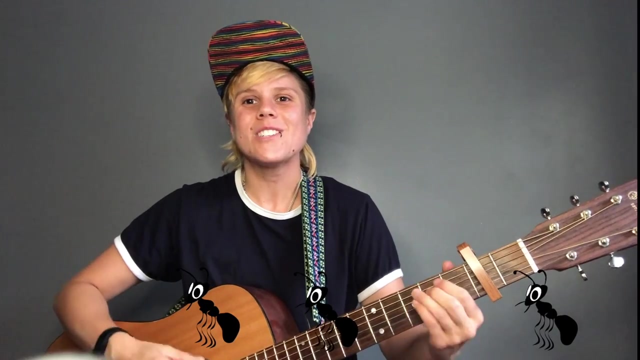 Boom, boom, boom, boom, boom, boom, boom. The ants go marching three by three. Hurrah, Hurrah. The ants go marching three by three. Hurrah, Hurrah. The ants go marching three by three. The little one stopped to climb a tree and they all go marching down to the ground to get out of the rain. 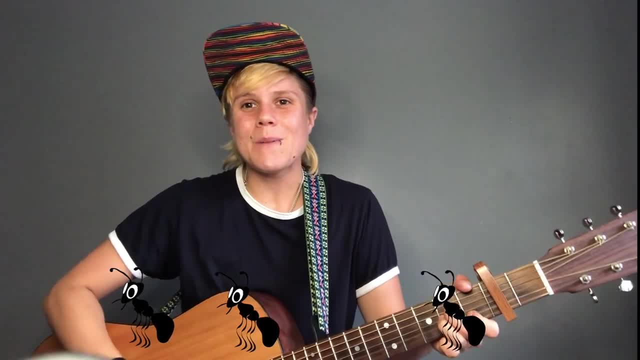 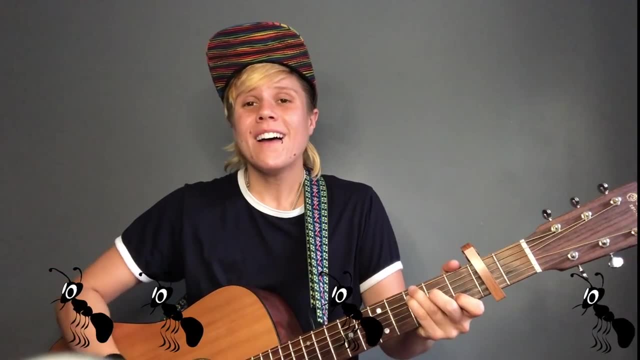 Boom, boom, boom, boom, boom, boom, boom. The ants go marching four by four. Hurrah, Hurrah. The ants go marching four by four. Hurrah, Hurrah. The ants go marching four by four. The little one stopped to shut the door and they all go marching three by three, Hurrah, Hurrah. 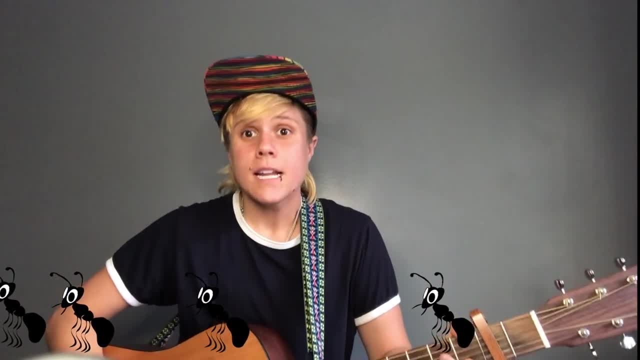 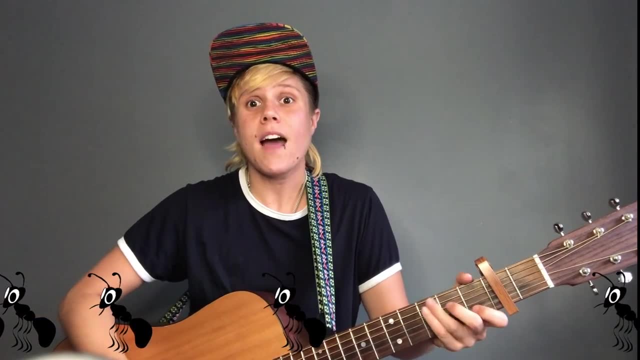 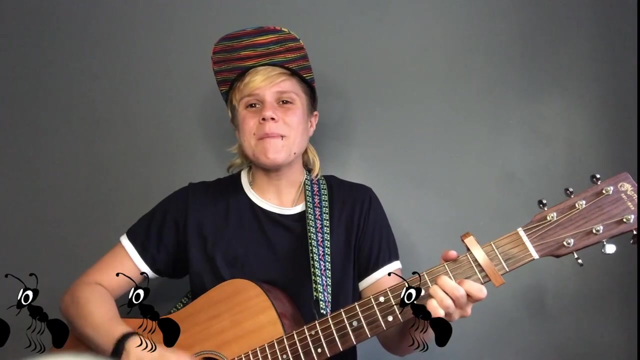 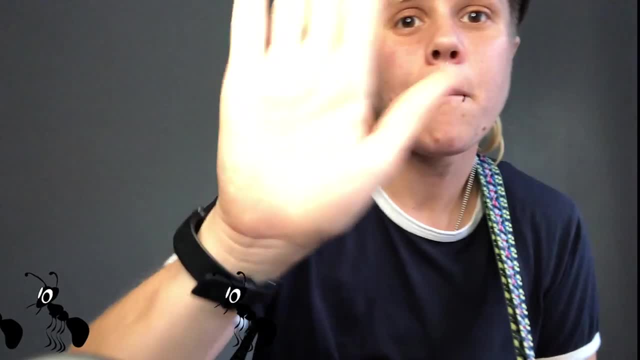 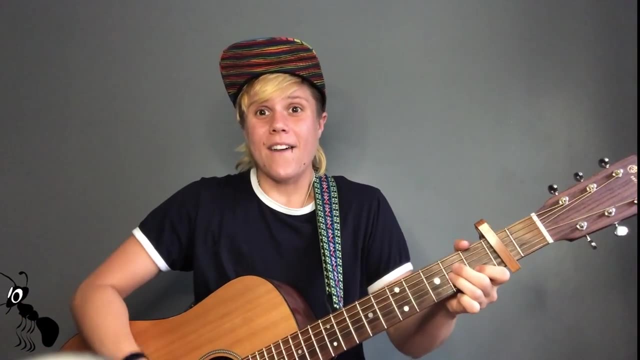 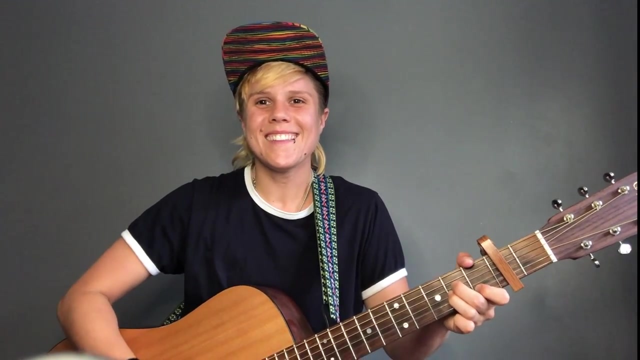 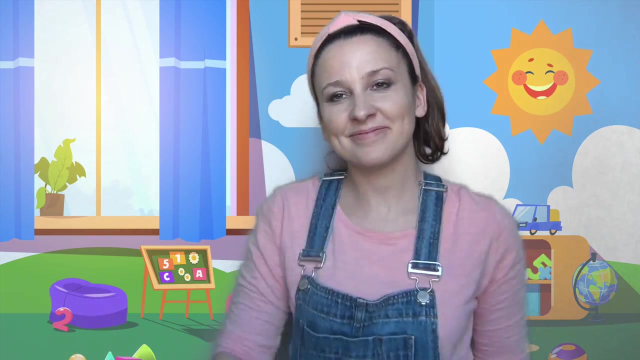 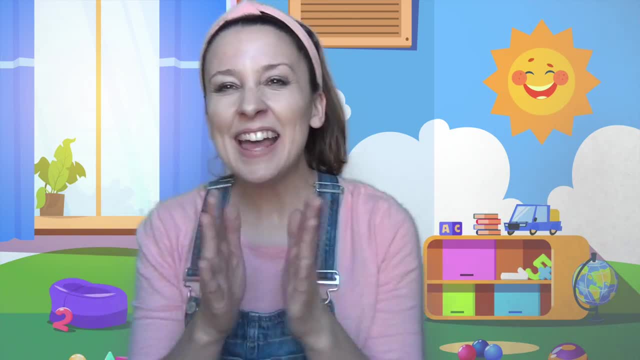 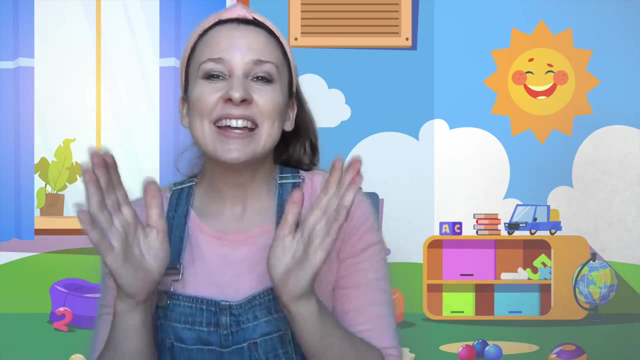 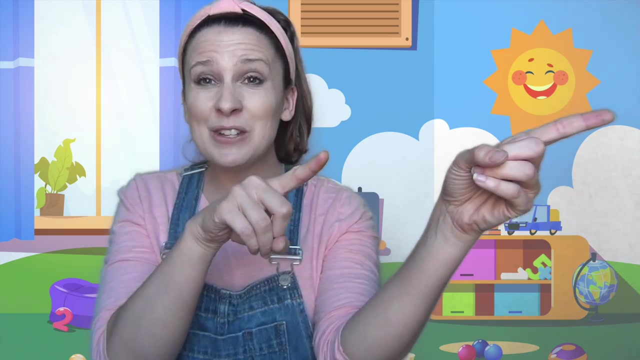 Pull, pull, clap, clap, clap. Wind it back again, Wind it back again, Pull, pull, clap, clap, clap. Point to the ceiling, Point to the floor, Point to the window, Point to the door. Put your hands together, One, two, three. 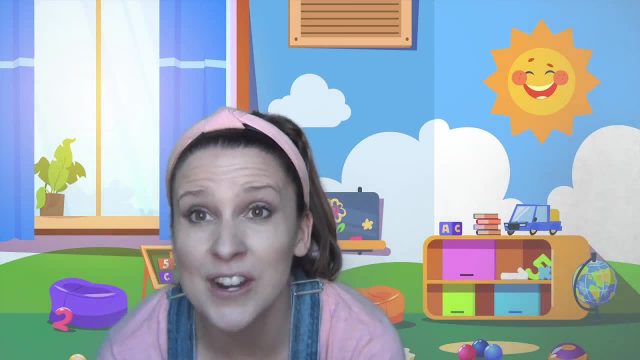 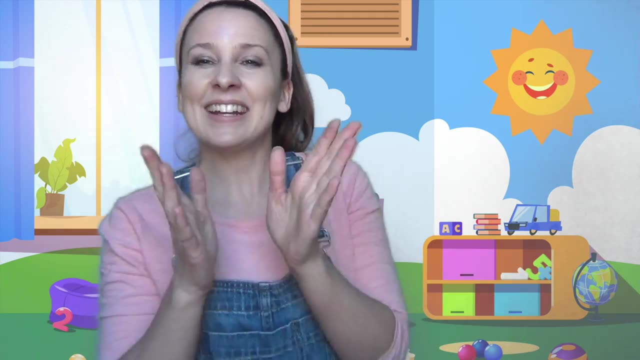 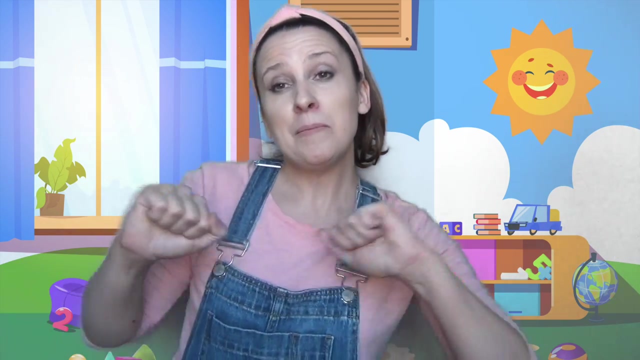 Put your hands up on your knees, Wind the bobbin up, Wind the bobbin up, Pull, pull, clap, clap, clap. Wind it back again. Wind it back again. Pull, pull, clap, clap, clap. Point to the ceiling, Point to the floor. 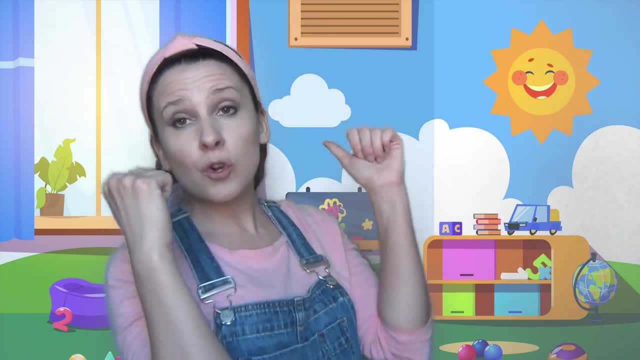 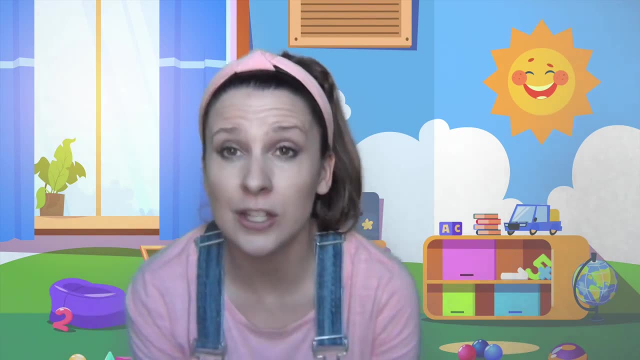 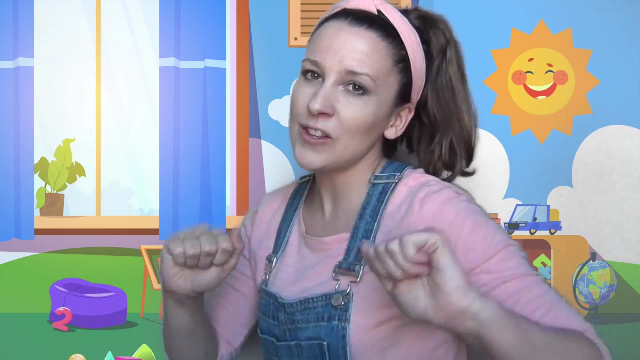 Point to the window, Point to the door. Put your hands together. One, two, three. Put your hands up on your knees. Wind the bobbin up. Wind the bobbin up, Pull, pull, clap, clap, clap. 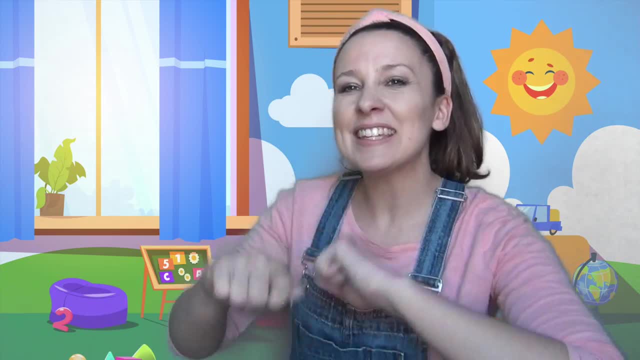 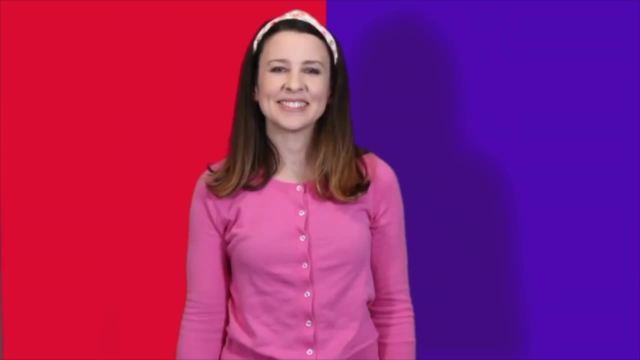 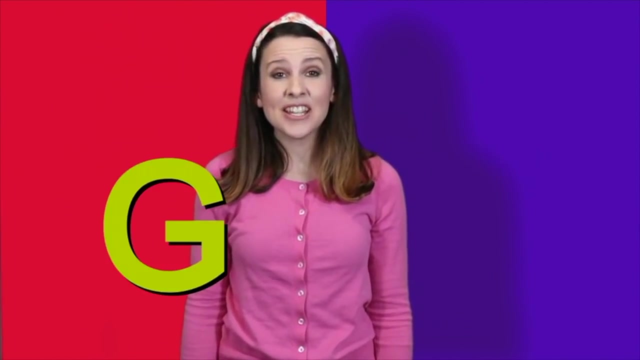 Wind it back again. Wind it back again. Pull, pull, clap, clap clap. Great job. A, B, C, D, E, F, G, H, I, J, K, L, M, N, O, P. 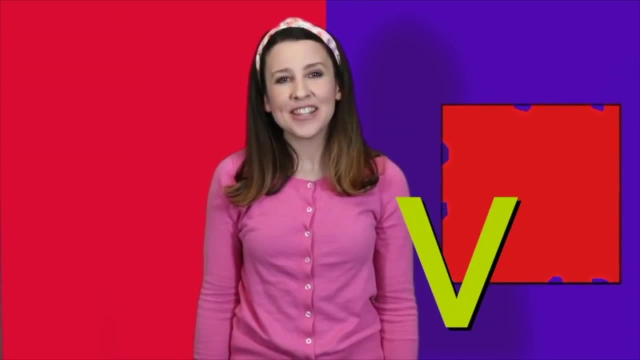 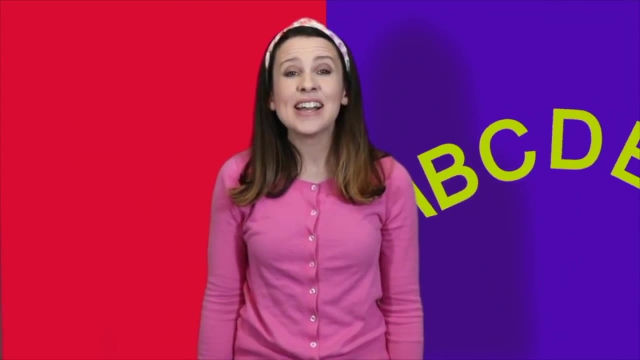 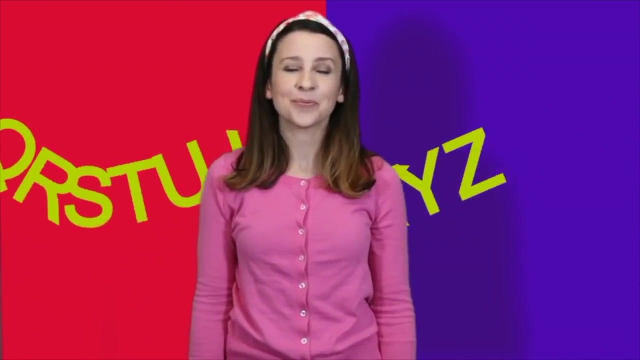 Q, R, S, T, U, V, W, X, Y and Z. Now I know my ABCs. Next time won't you sing with me: A, B, C, D, E, F, G. 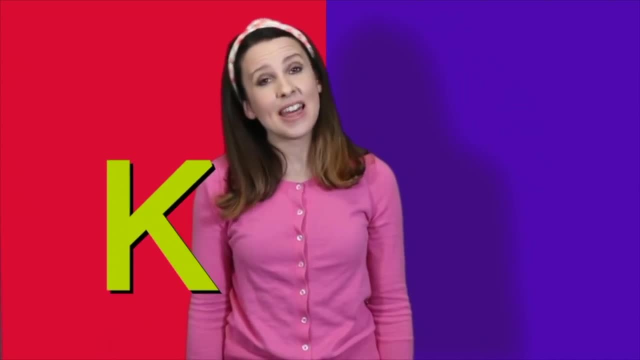 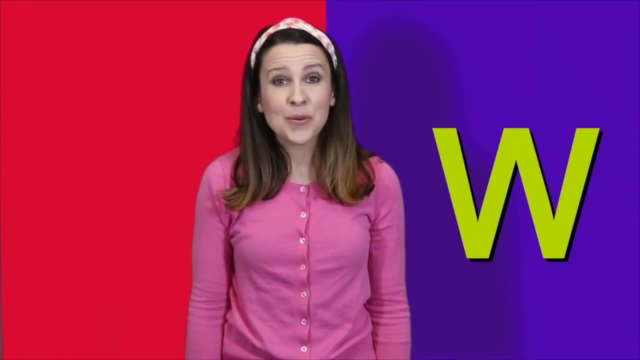 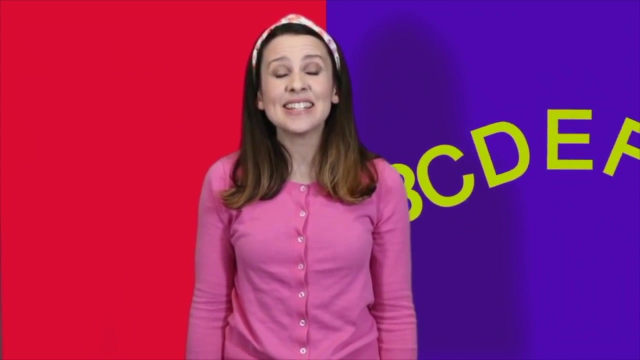 H, I, J, K, L, M, N, O, P, Q, R, S, T, U, V, W, X, Y and Z, W, X, Y and Z. Now I know my ABCs. 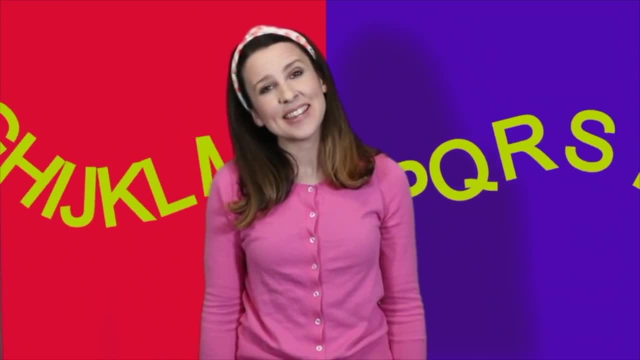 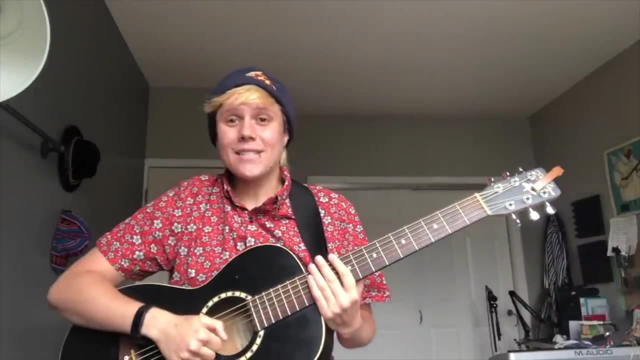 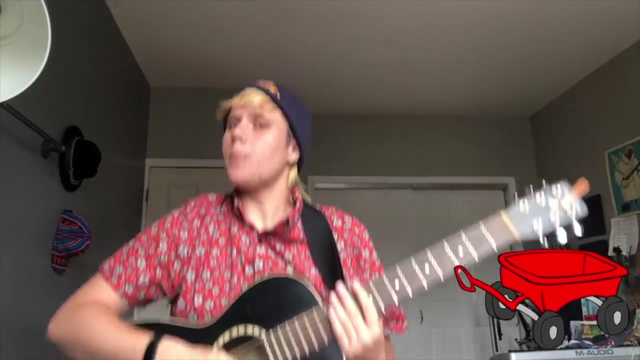 Next time won't you sing with me? Now let's try bumping up and down in my little red wagon. Let's start with a nice bumpy tempo. Bumping up and down in my little red wagon. Bumping up and down in my little red wagon. 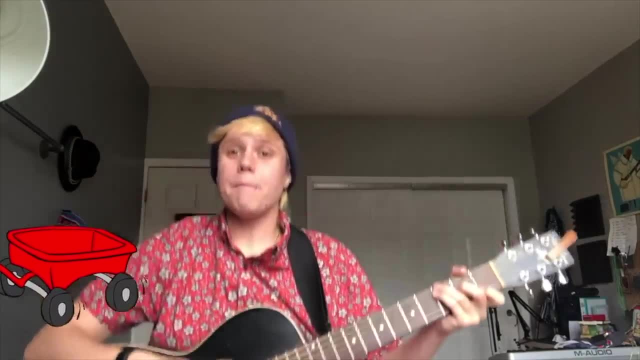 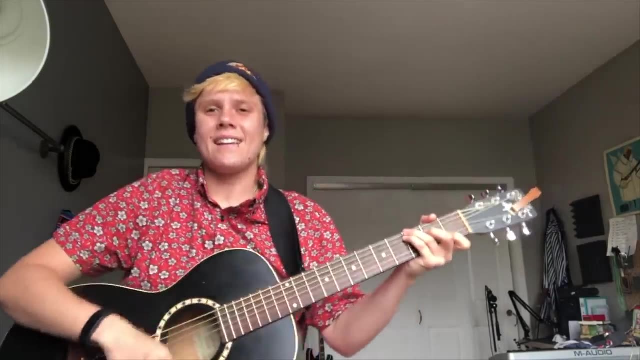 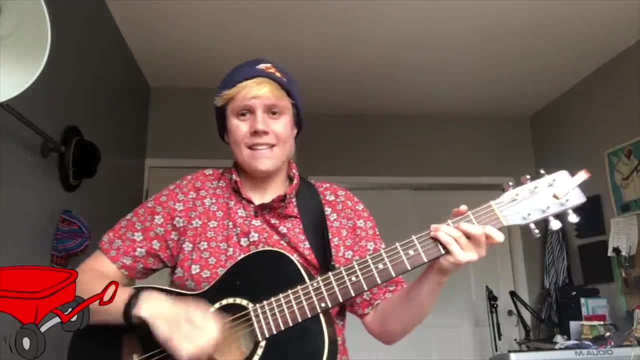 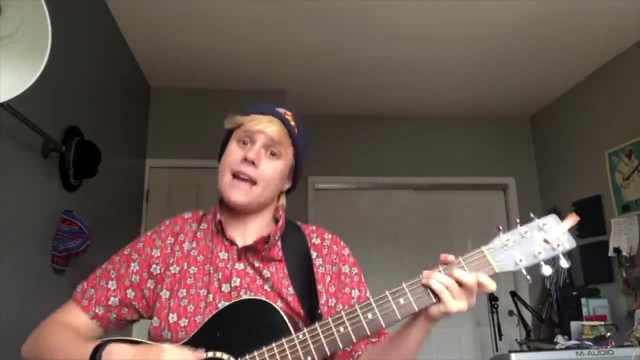 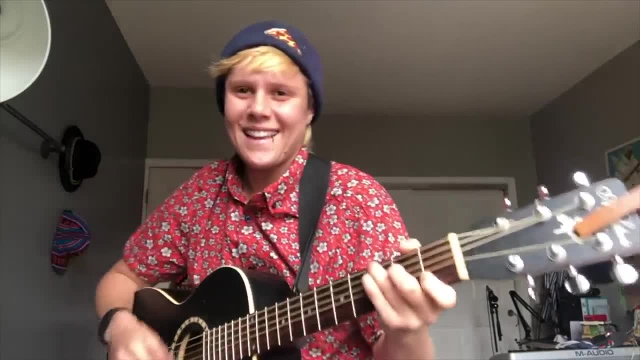 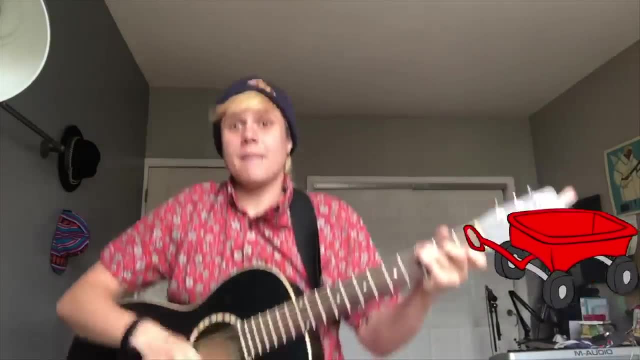 Won't you be my darling? Won't you be my darling? Okay, let's try it really fast. It's going to be a bumpy ride. Here we go, Bumping up and down in my little red wagon. Bumping up and down in my little red wagon. 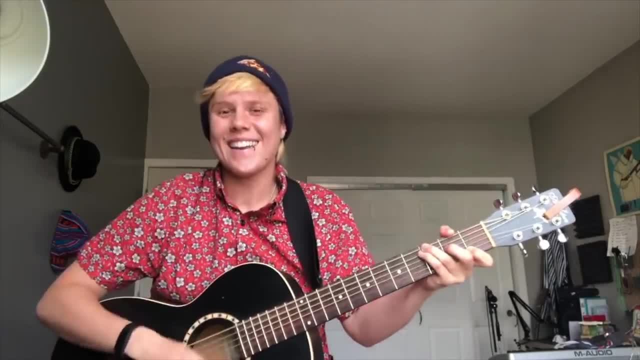 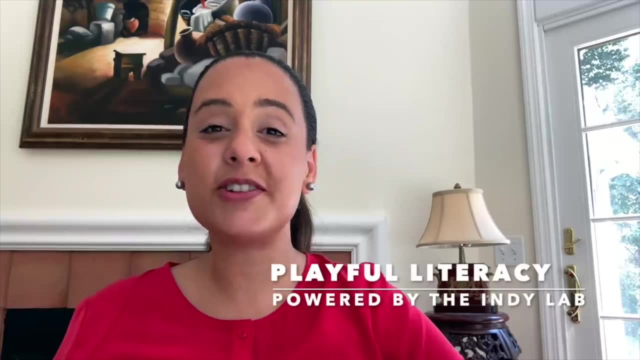 Bumping up and down in my little red wagon. Won't you be my darling? Nice job guys. Hi everybody, Welcome back to Playful Literacy. I'm so glad you could make it again. Today we're doing the letter sound C. 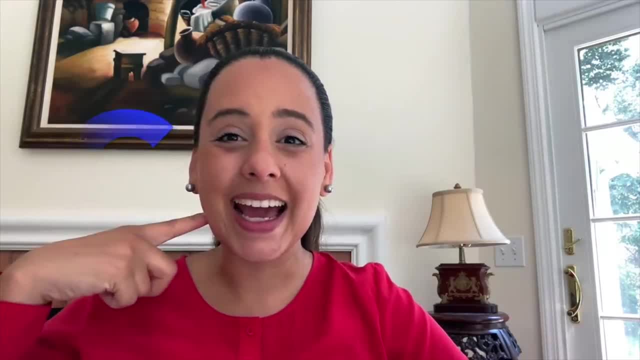 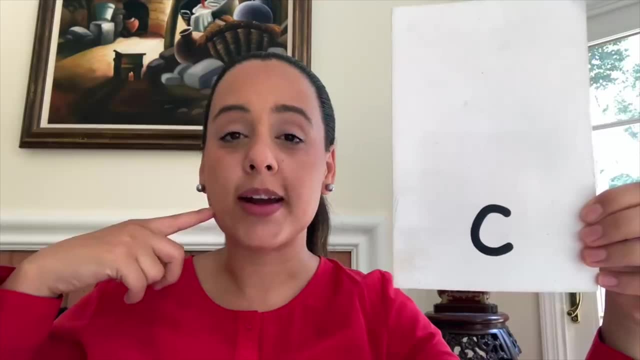 C says C. Let me show you what it looks like. This is my letter C and it makes this sound. This is my letter C and it makes this sound. When I open my mouth really big, my tongue hits the roof of my mouth. 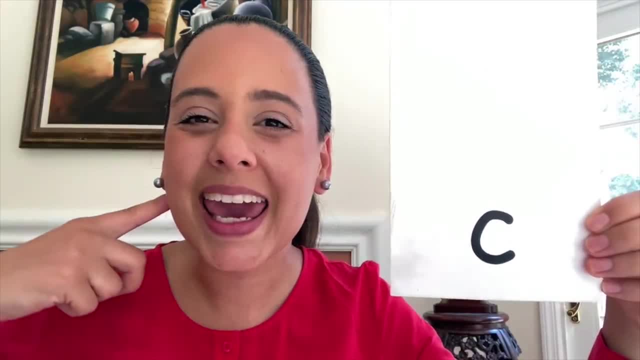 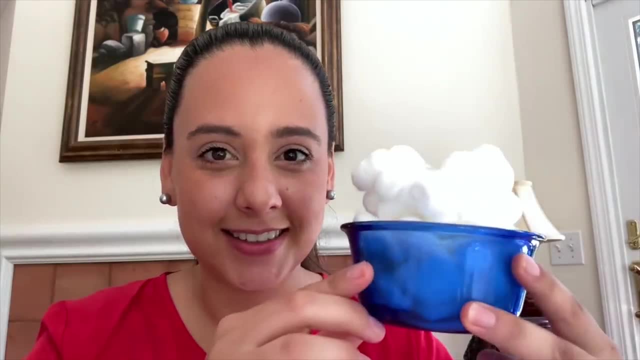 My tongue hits the roof of my mouth. Can you try? Can you guys guess what we're going to make? Can you guys guess what we're going to make for our letter C today? Look at this. Do you know what this is? This is cotton. 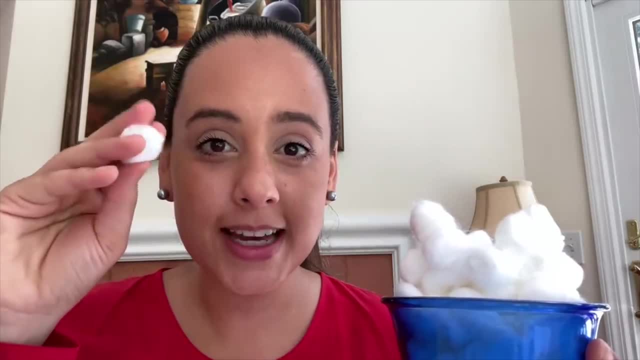 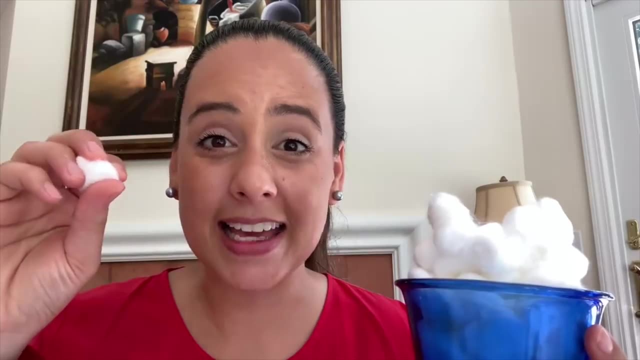 And it becomes a little ball. And it becomes a little ball. It feels super soft on your skin. It feels super soft on your skin. We're going to make cotton ball C's today. We're going to make cotton ball C's today for our letter sound K. 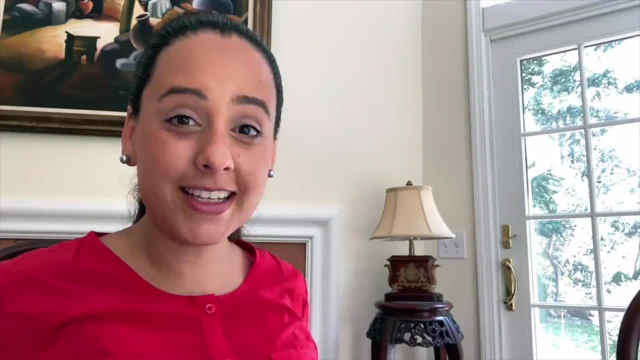 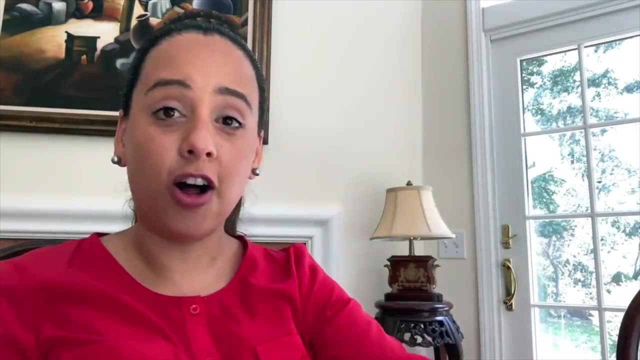 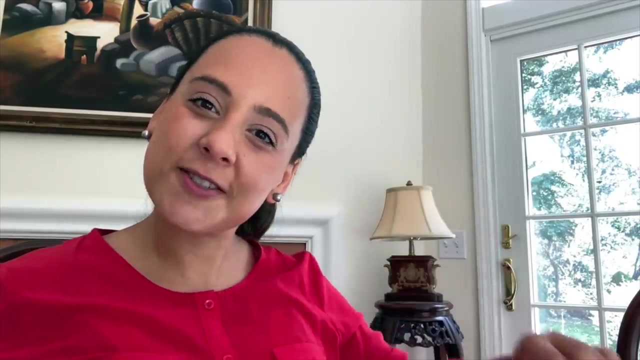 And we're going to dye them and count them. Everybody ready. I have my glue, my colorful paper, my colorful paper, all of my dyes for the food coloring and my cotton balls. We have so many things that start with our letter. sound of the day. 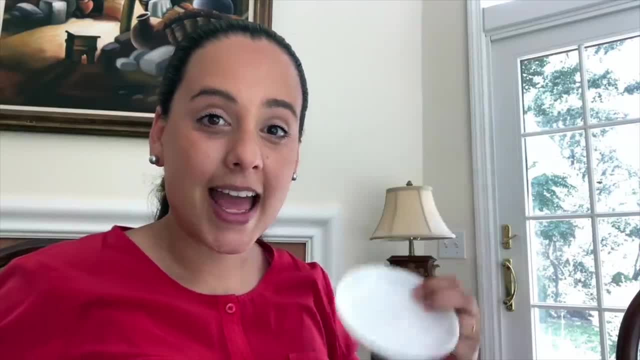 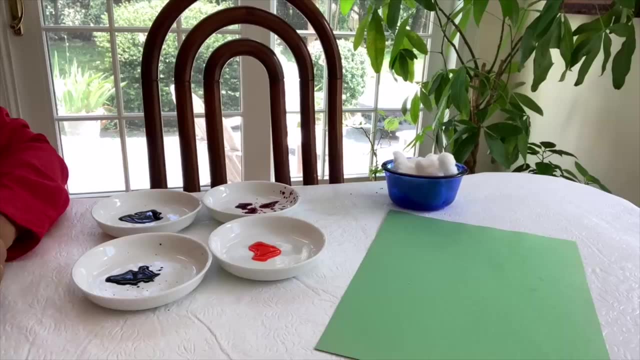 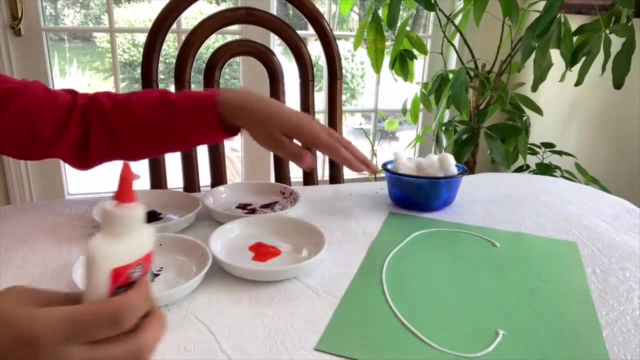 I'm going to put my dye in these plates And then I'm going to dip my cotton balls in them to make my C. Here we go. Alright, everybody, I'm going to make my C first, All the way around with my glue. 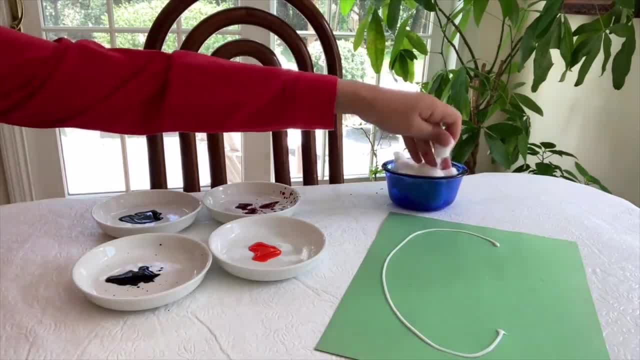 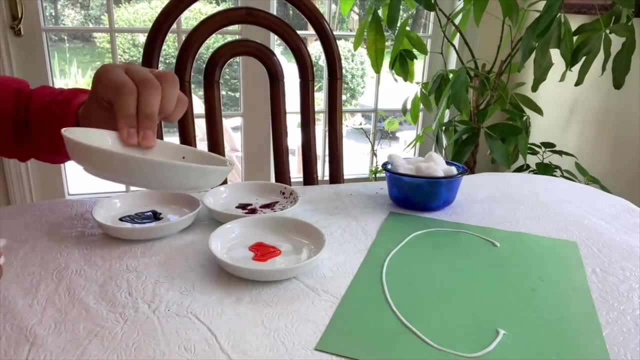 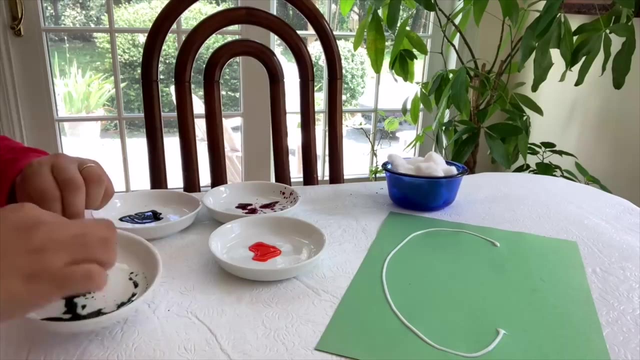 And now I'm going to take a cotton ball and dip it in one of my colors, and dip it in one of my colors. I wonder what this color is going to be. Can you tell me? Let's see Whoa. It's green. 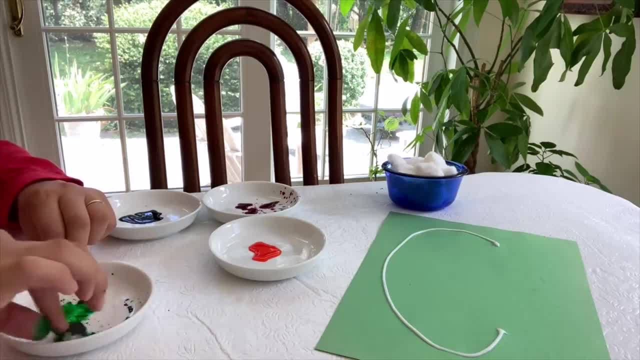 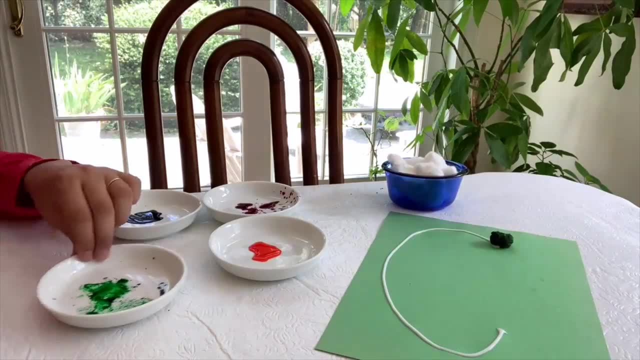 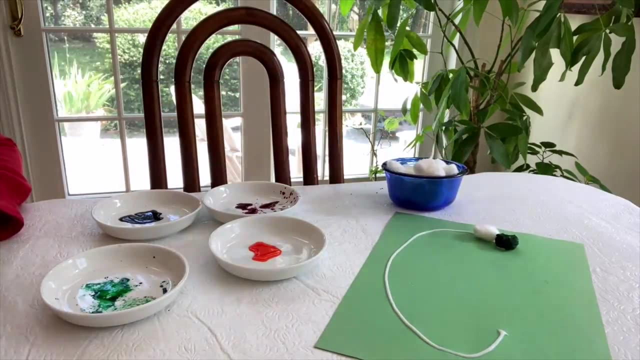 Oh my gosh, my fingers are going to get so colorful. I'm going to put my green cotton ball on my letter. Alright, now I want to do a different color. I'm going to do just white and put it on my C. 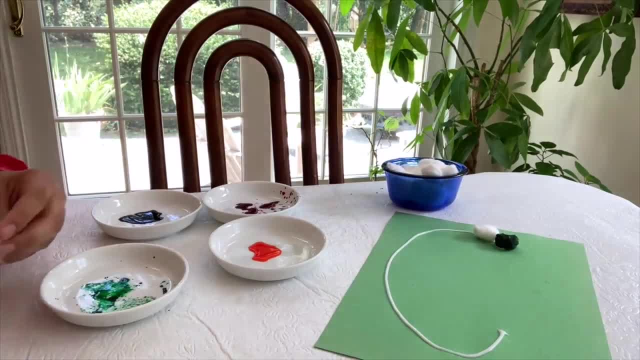 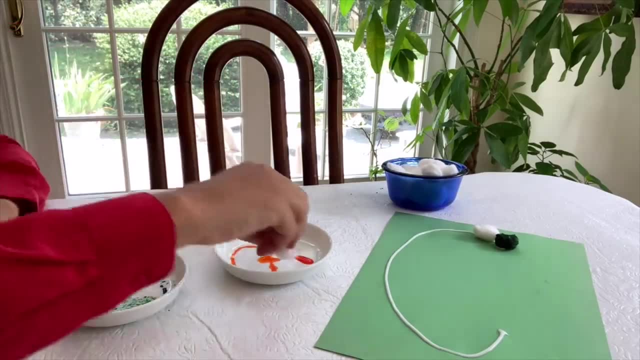 My K sound. Now I want to do a color. I'm going to do this color. Can you guess what that's going to be? It looks a little orange right now, but I think it's supposed to be yellow. Let's see what happens to it. 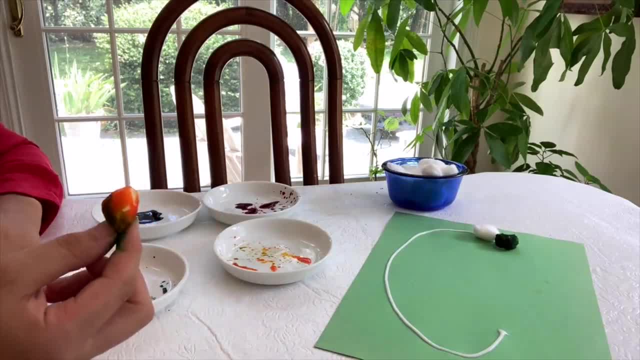 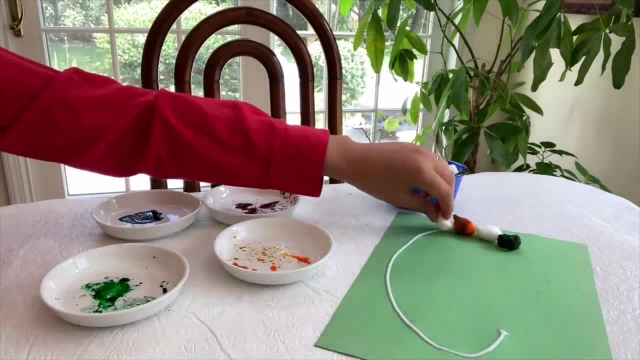 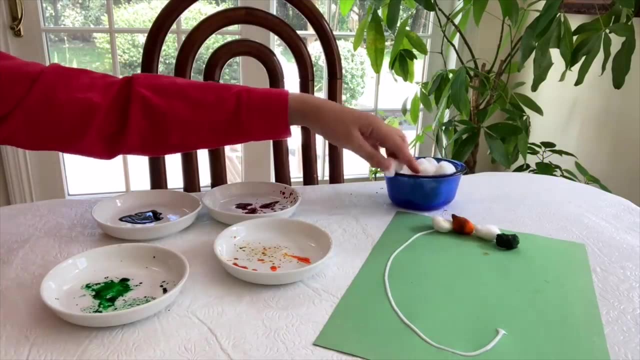 Oh, my goodness, It got mixed up with my green. That's silly. Let's put it here. Now I'm going to do another white one, So I have a green, white, orange, white. I'm going to pick a different color now. 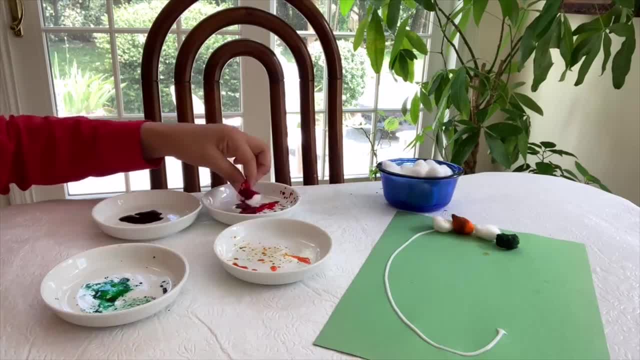 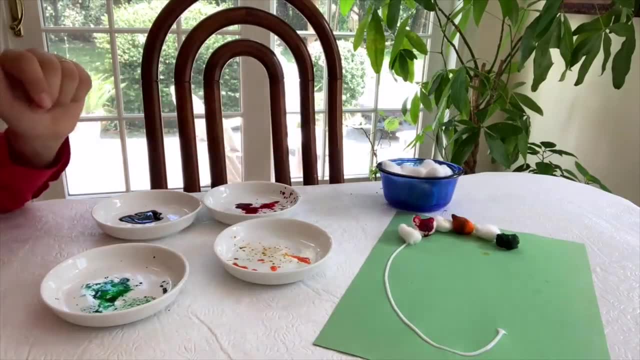 Let's make this one. It's red, everyone A dark red. Now I'm going to put white, So I do color white, color white, color white. Let's keep going. Let's do this one, Wow. 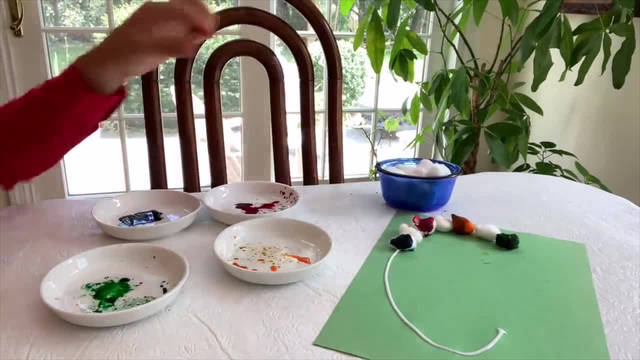 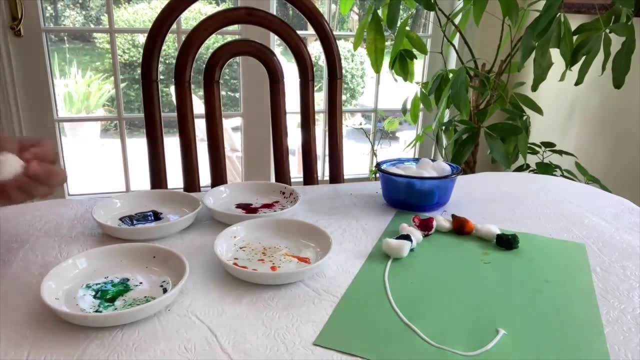 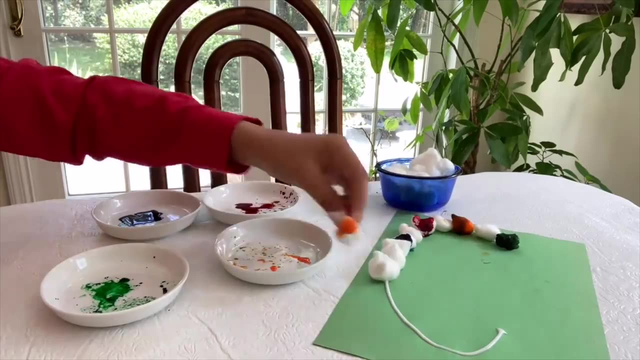 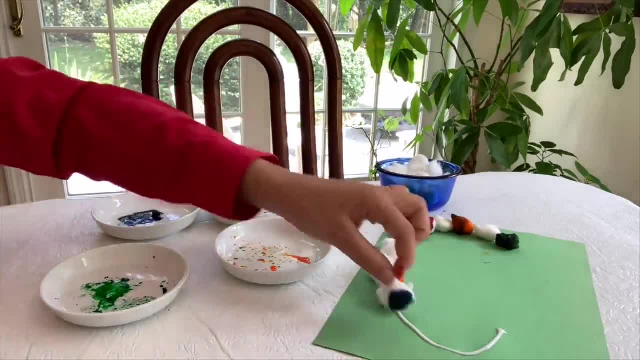 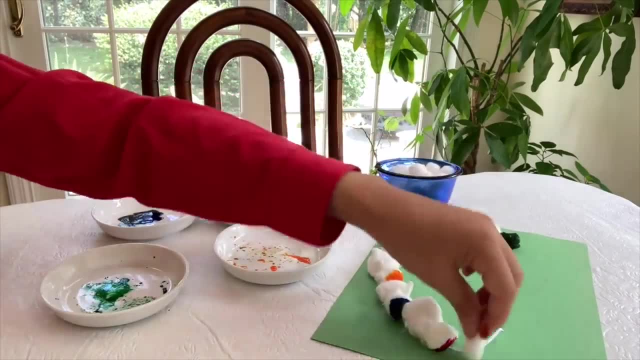 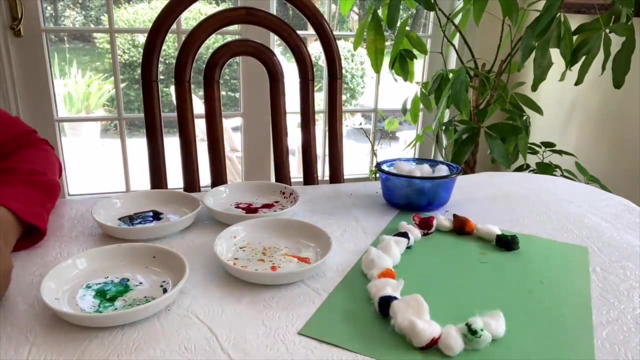 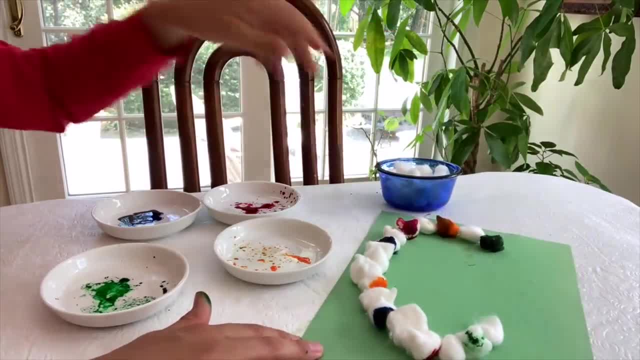 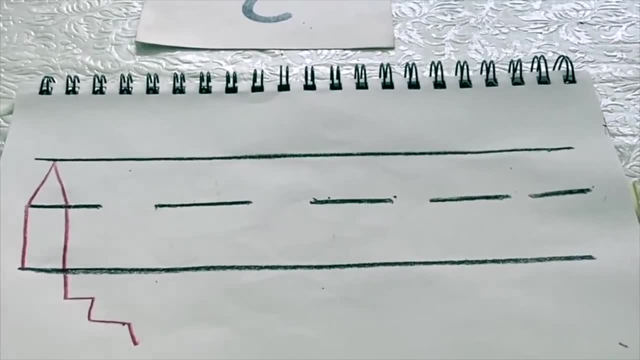 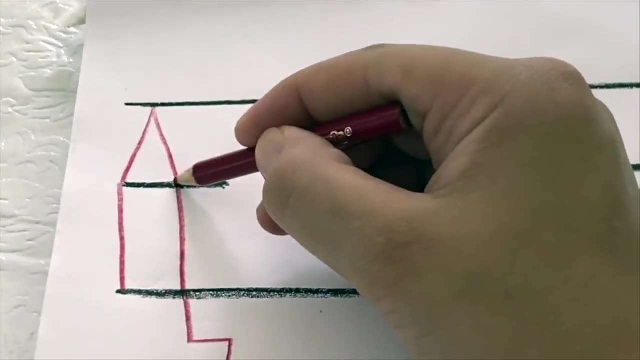 That is so much fun. Can you show me what colors you made? Do you all remember my notebook? This is my house letter paper and where I learned how to write my letters. My letter C is going to go inside my living room. I start at: 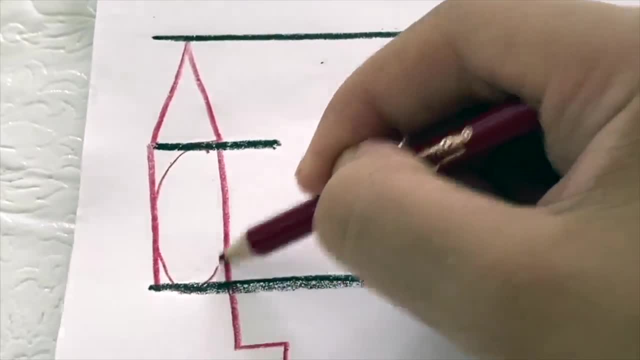 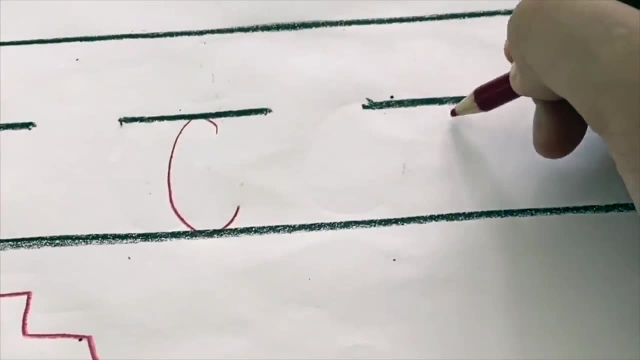 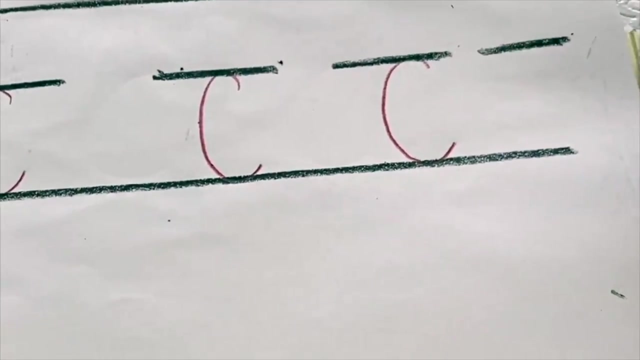 the top of my living room and I go around. Just like that. Let's make another one. I start at the top and I go around. I start at the top and I go around. I start at the top and I go around. 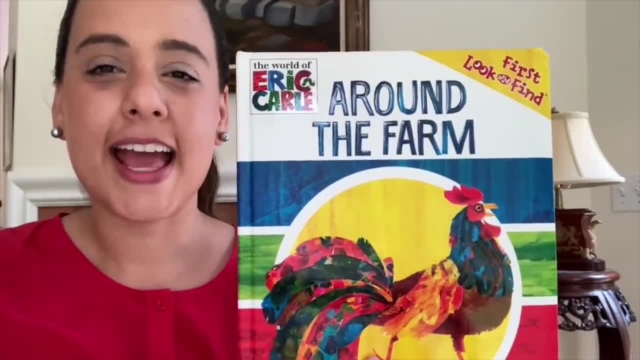 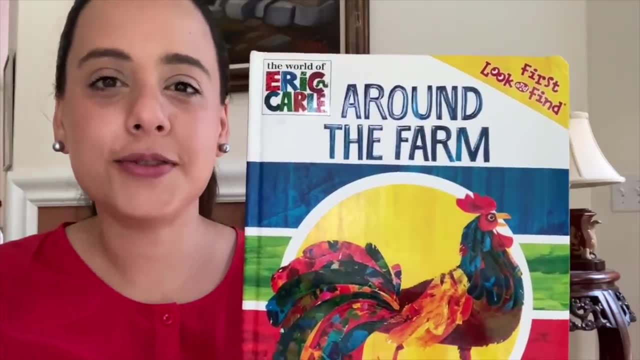 Alright, guys, we're going to do a rebus story and that's when you hear our letter sound of the day K and then you do something. I want you to clap, because that also has our K sound in it. You could do other things. 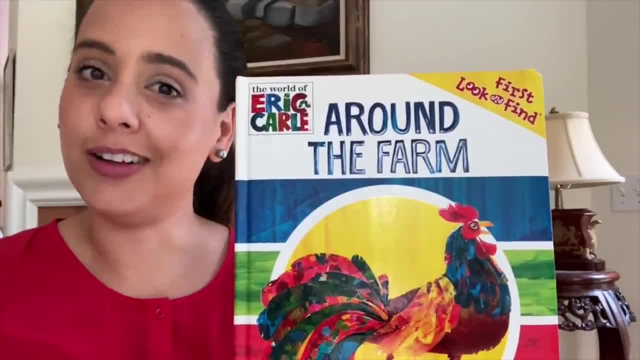 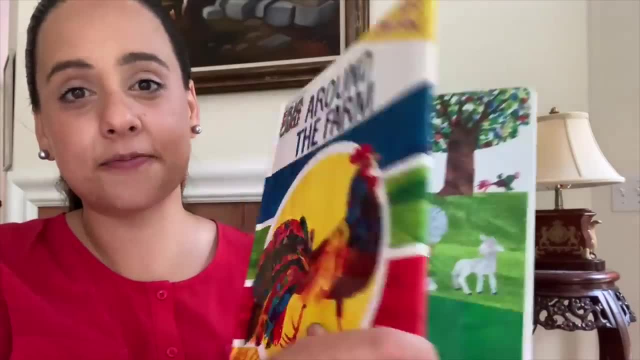 like you could kick, you could kiss, you could crawl. try to think of something else you could do with the sound K. Let's find words that start with our sound of the day: Whoa. look at all of my animals, I see one. 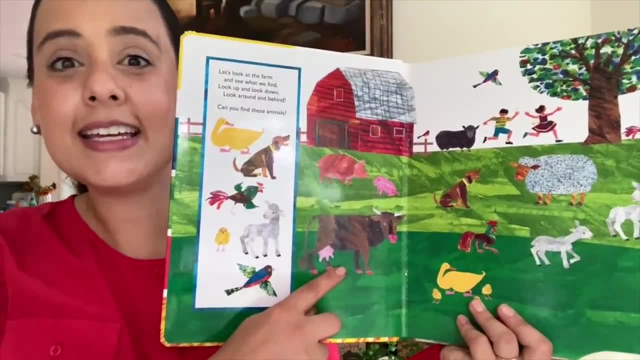 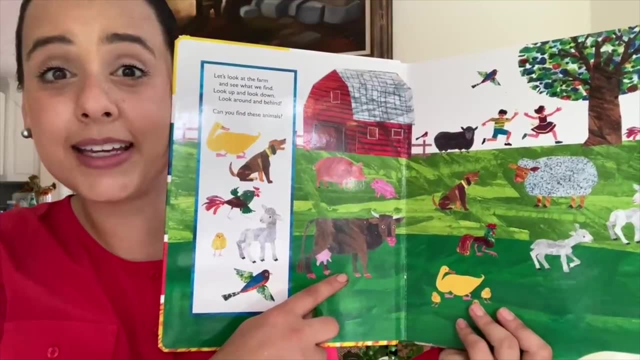 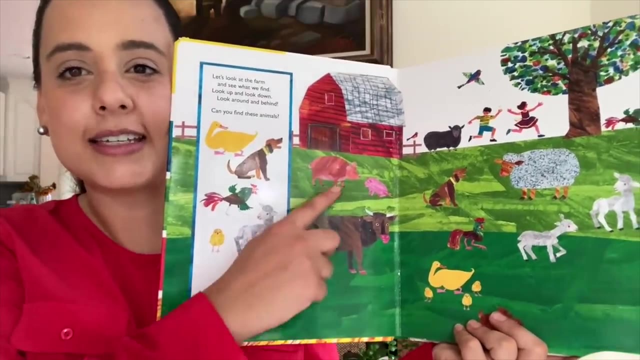 right away. Do you know what this is? That's a cow. Does that have our K sound at the beginning? Yes, you're right. So let's clap. Let's look for other animals. I see a pig. Does that have my K? 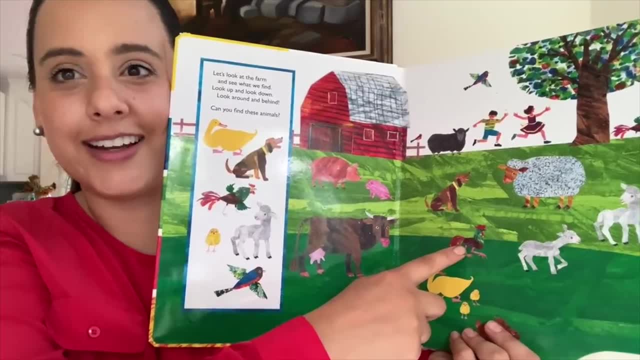 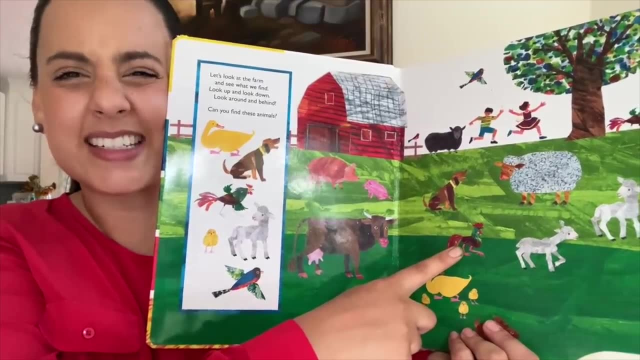 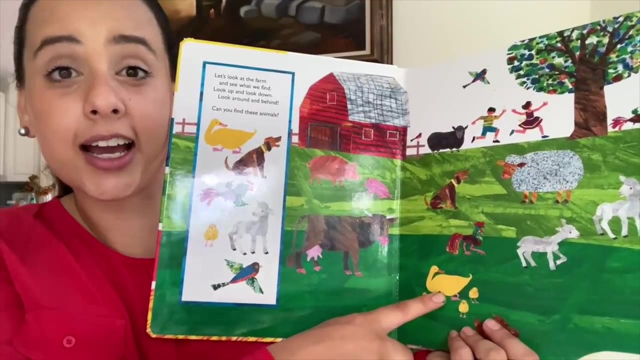 I see a chicken. Wait a second, That's a sneaky K Chicken. It's in the middle of my word, Sneaky K. What about this one? A duck? Do you hear K? It's at the end of my word. 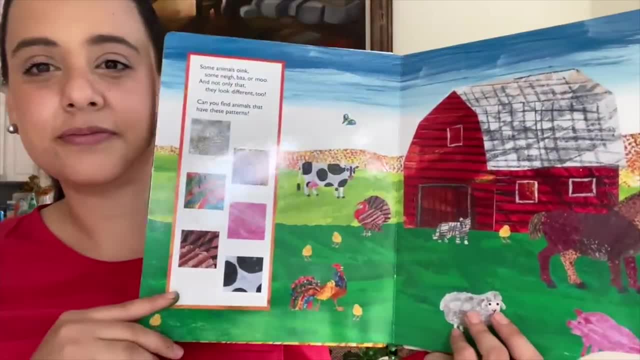 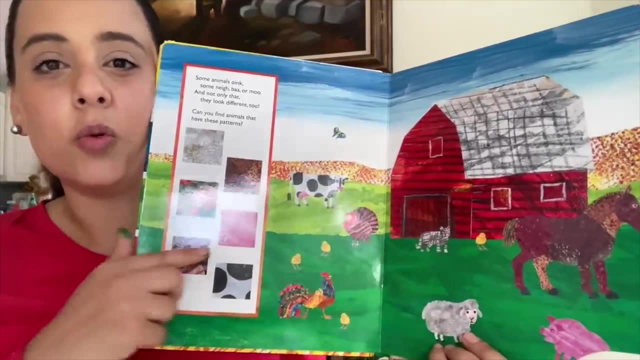 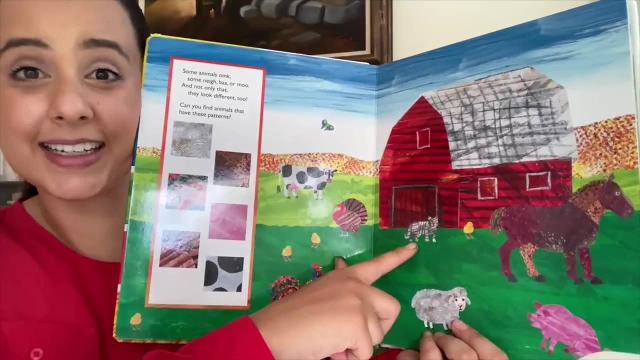 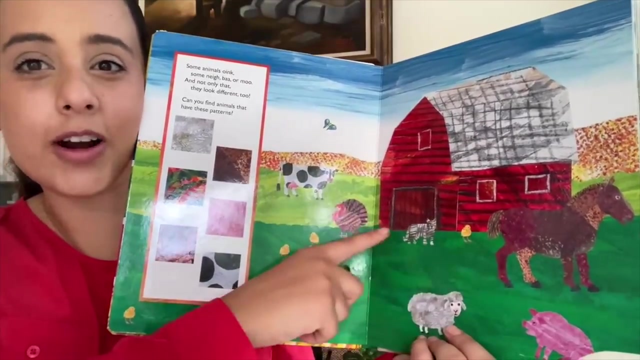 Let's keep going. Look at this. I see a new animal here and here. Which one has my K sound? Is it horse or is it cat? Hmm, Which one starts with K? Horse or cat? K, It's cat. Everybody give me a big clap. 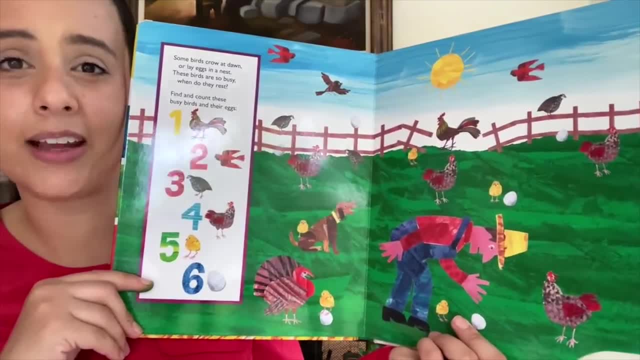 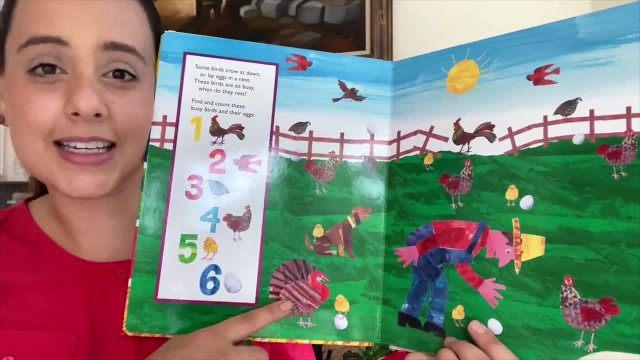 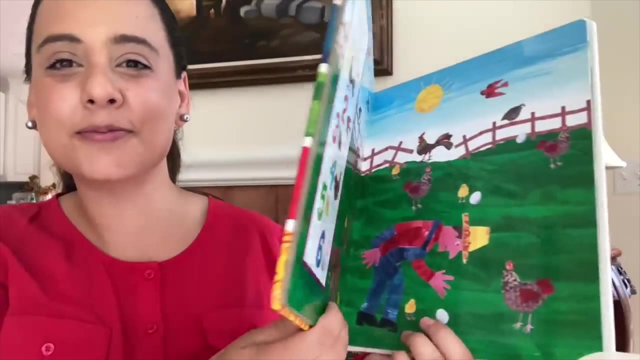 Let's try this page and see if we find any new animals. I see a turkey. Wait a second, Is my K sneaking in again. Turkey, It's in the middle of my word. Give me a big clap. You guys found so many. 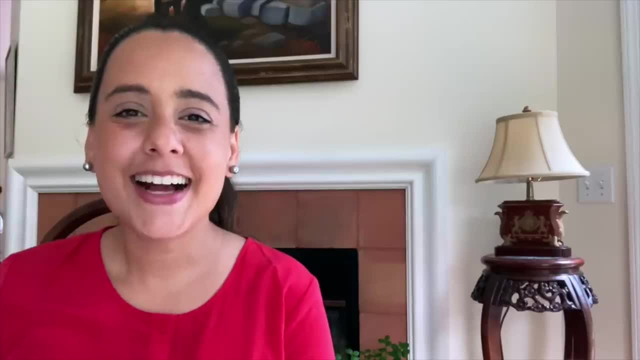 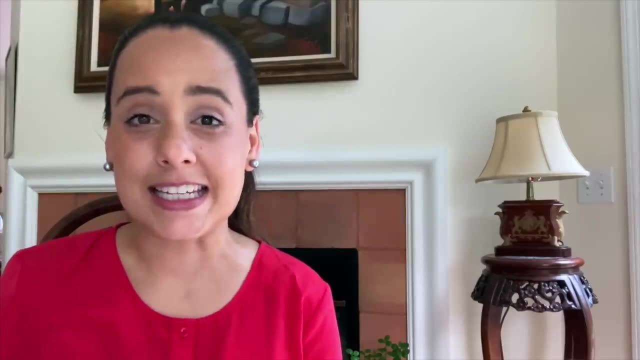 words in my Around the Farm book. Nice job, Guys. I had so much fun making cotton balls with you and learning all about the sound K today. Remember C is for K, And now you can clap every time you hear it. See you guys next time. 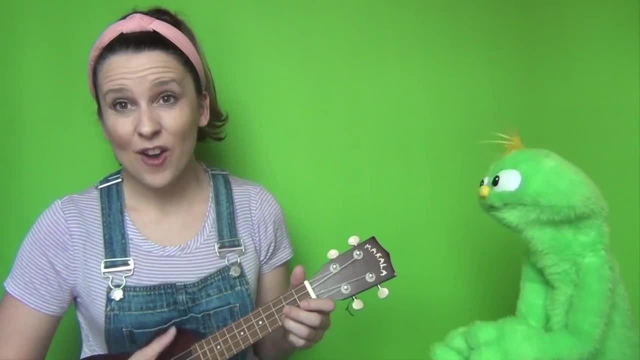 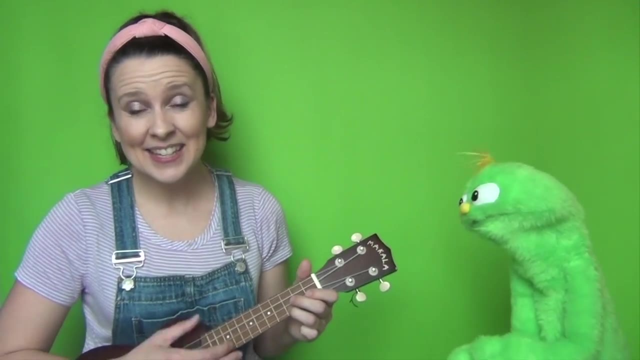 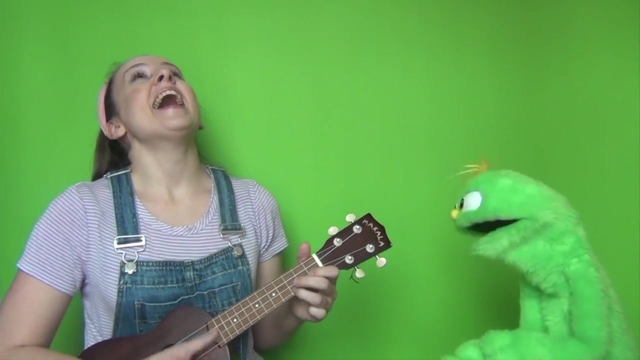 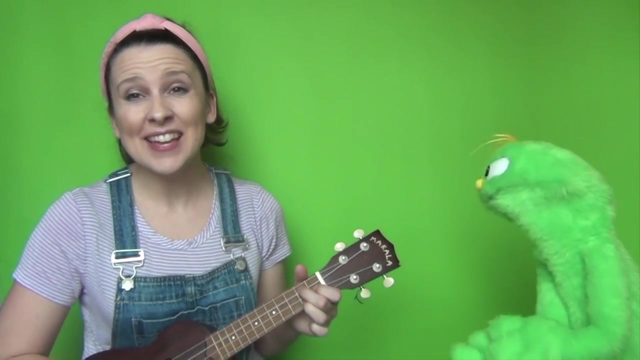 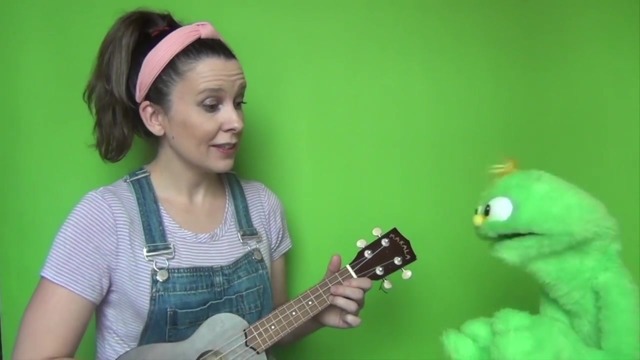 Thanks for coming to Playful Literacy. Bye, Rachel. I got an idea. What's your idea? What if it was raining candy bars and milkshakes? Such a great idea. We'll do snowflakes with that. Are you ready? 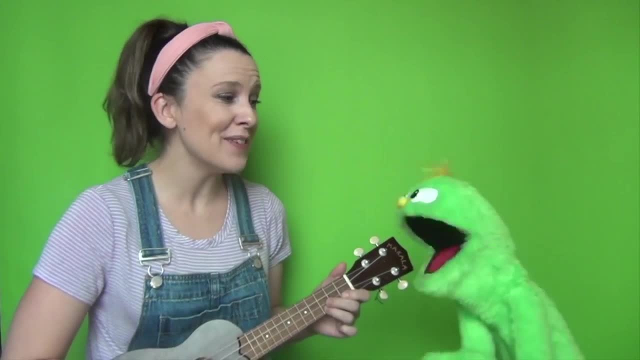 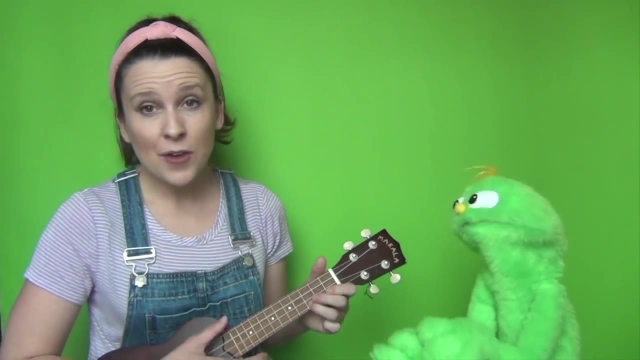 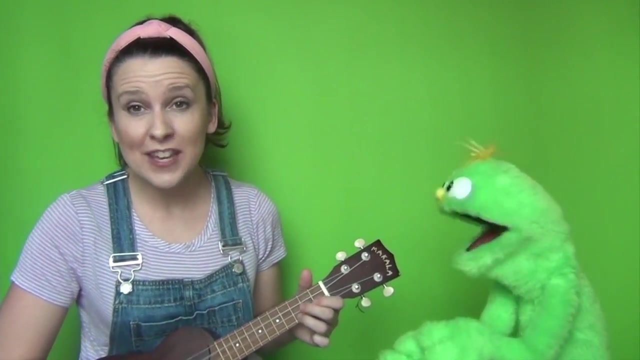 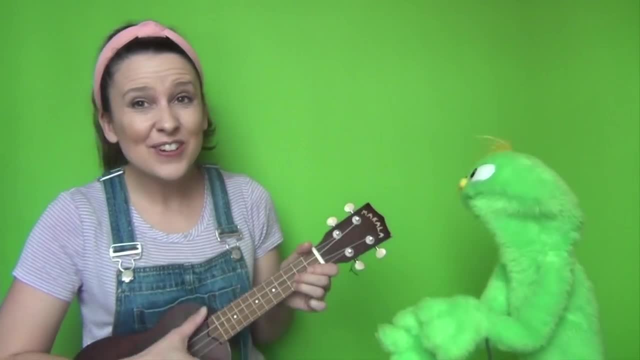 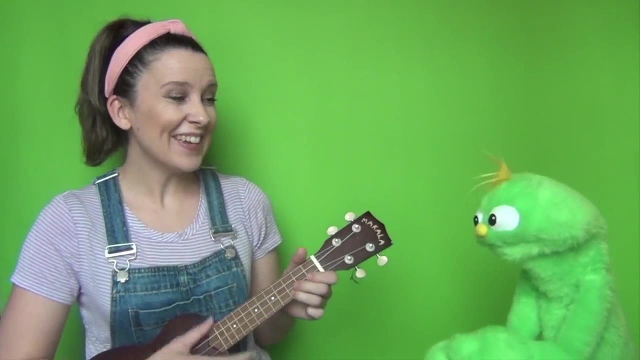 Oh, what a snow that would be. I love your idea. You know what next let's do? bubblegum and ice cream. Those are two of my favorite things. Okay, If all the sunbeams were bubblegum and ice cream. 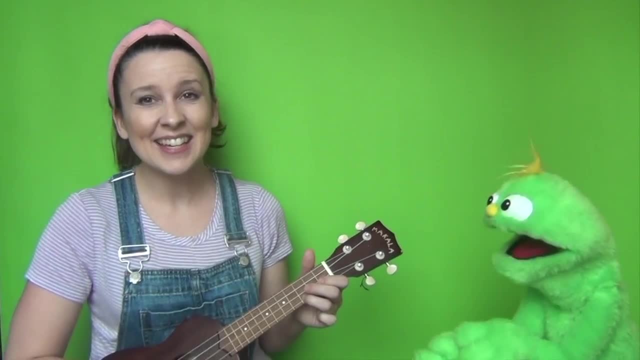 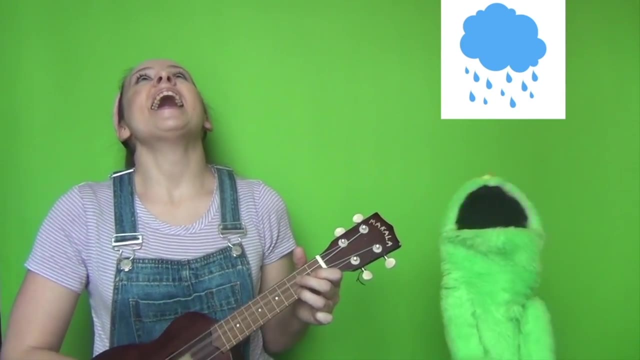 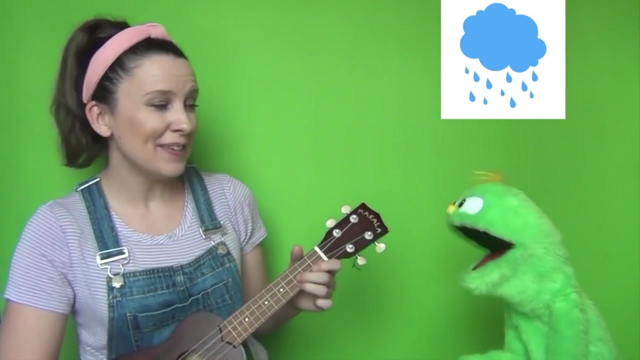 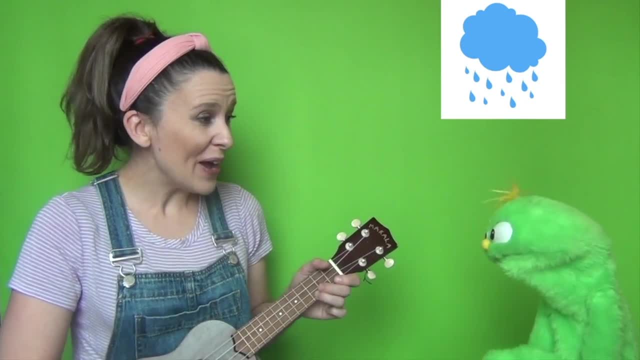 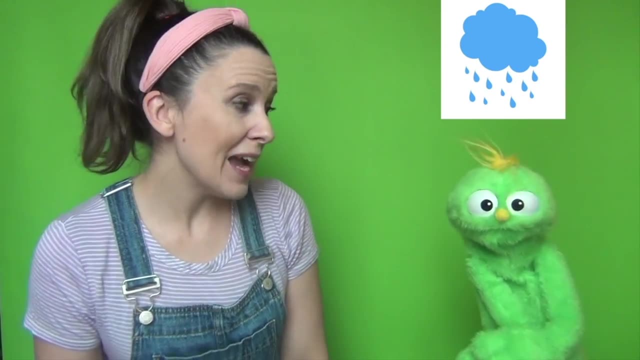 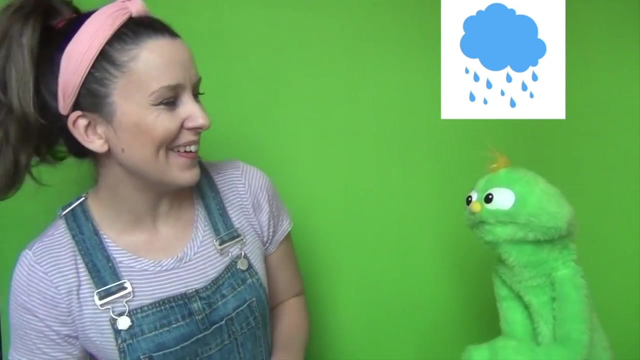 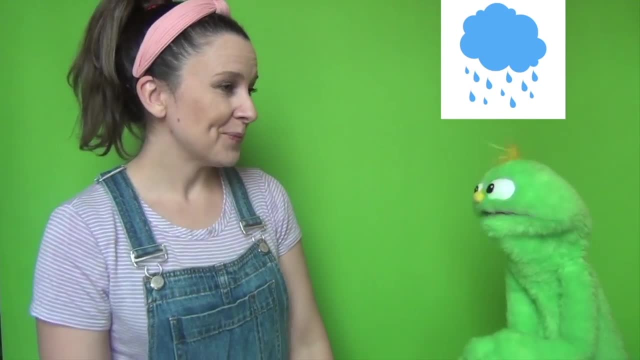 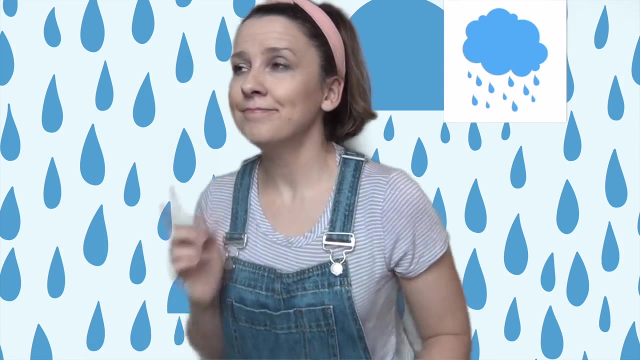 that would be. I'd love to hear what you would choose. Yummy, I like raspberries. Mmm, those are good too. No, it's still raining because we sang the rain song. Hmm, what can we sing to make it go away? 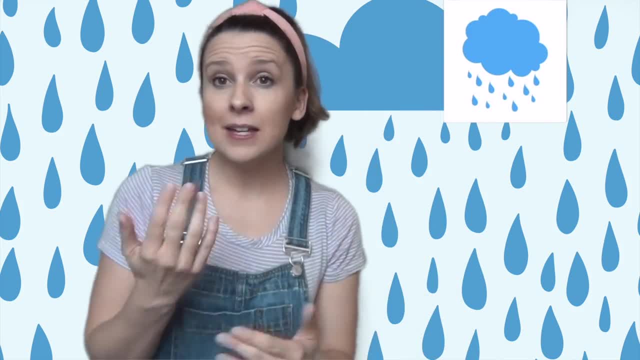 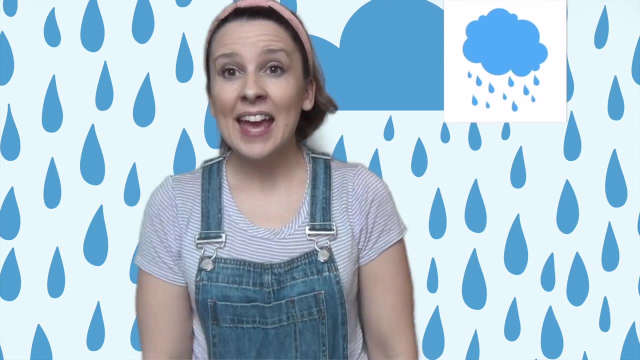 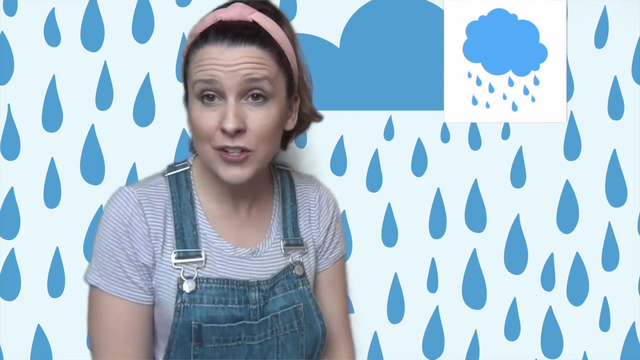 I know Rain, rain, go away. Come again another day. Rachel wants to play Rain, rain, go away. Now let's put your name in, because it's still raining and we need that rain to go away. Let's try it with your name. 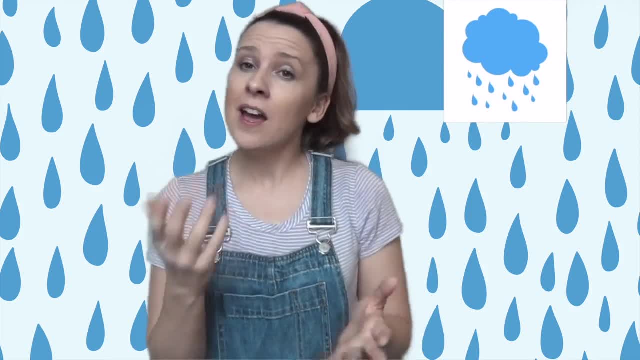 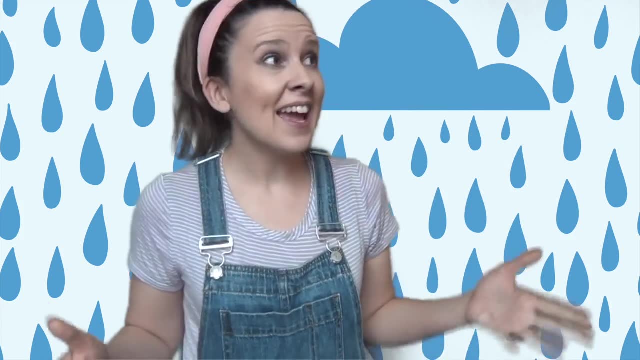 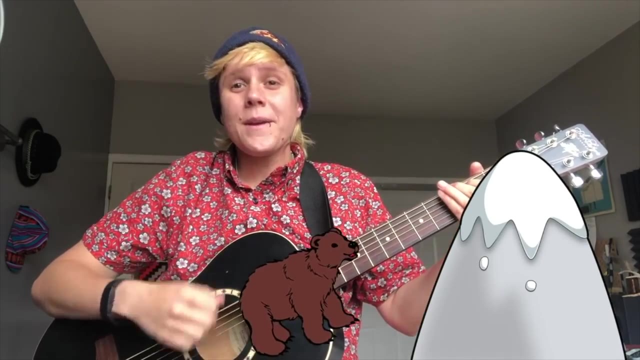 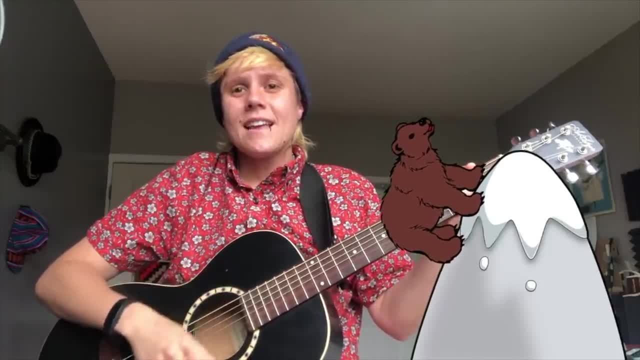 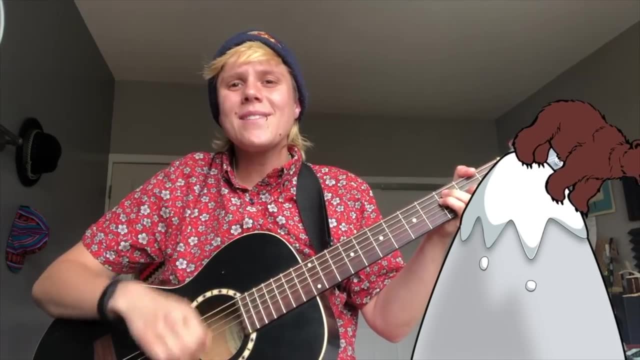 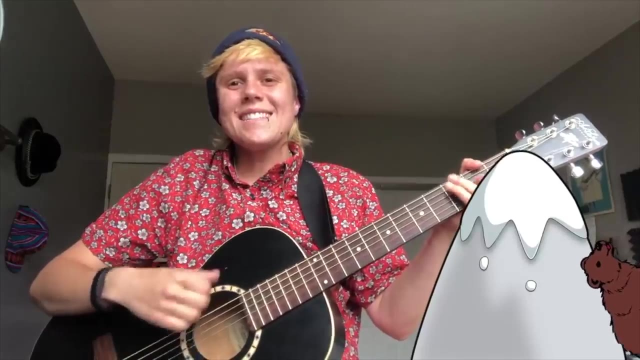 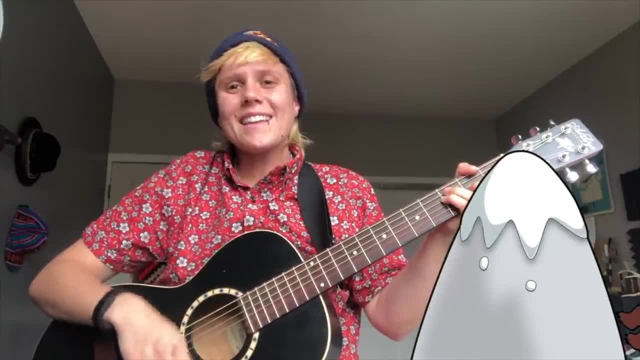 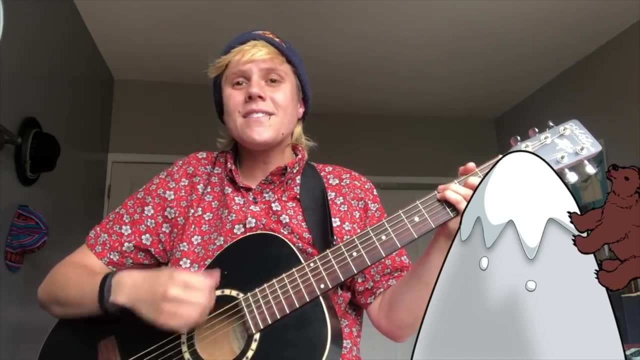 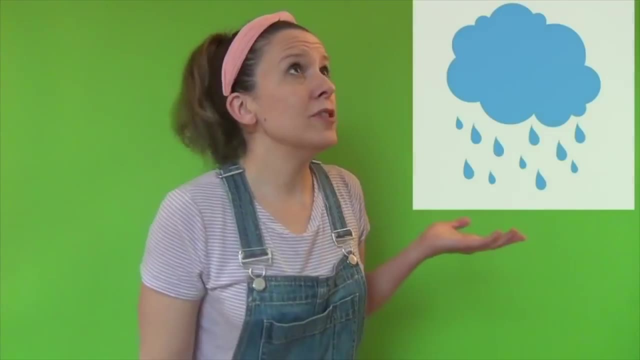 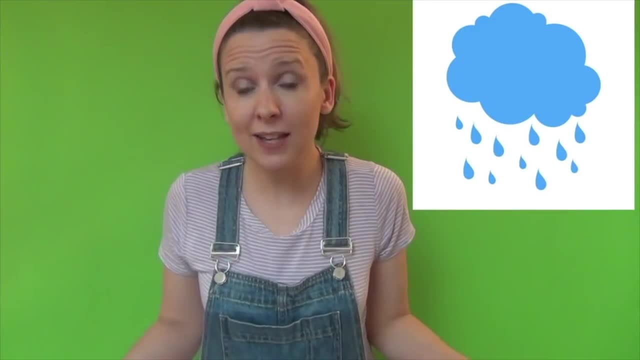 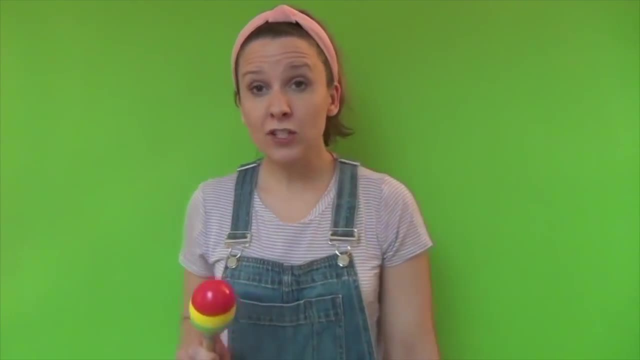 Can you help me sing, Mr Golden Sun, so the sun will come back out. If you have a shaker at home, it's time to get out your shaker. Oh, Mr Sun Sun, Mr Golden Sun, Please shine down on me. 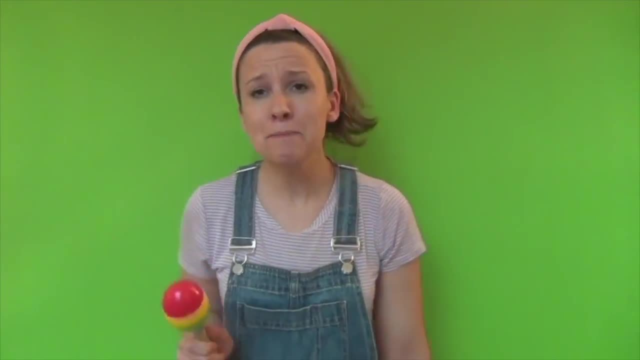 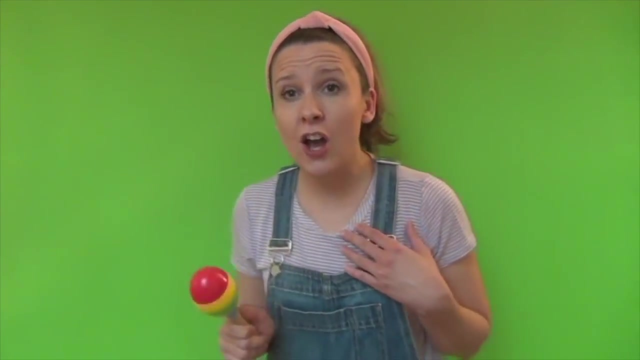 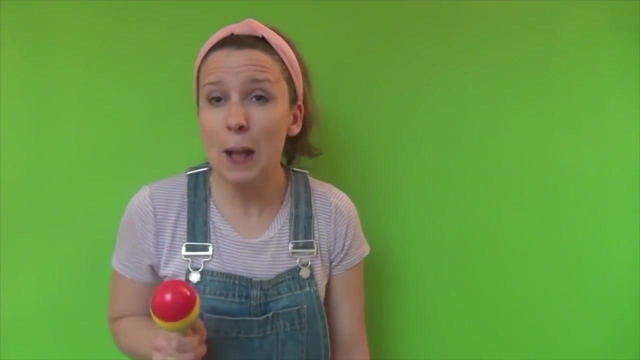 Oh, Mr Sun Sun, Mr Golden Sun, Mr Golden Sun, Hiding behind a tree. These little children are asking you to please come out so we can play with you. Oh, Mr Sun Sun, Mr Golden Sun, Please shine down on me. 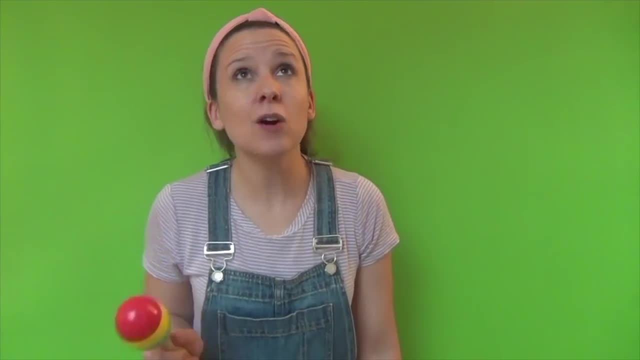 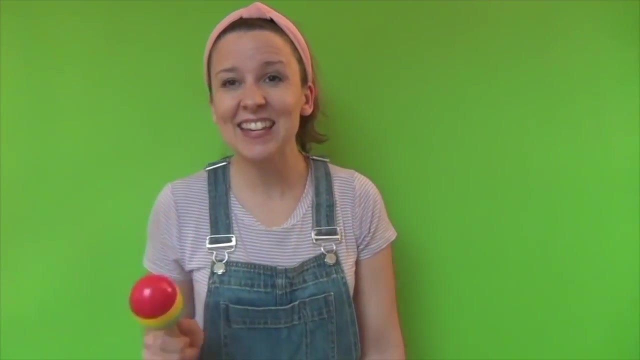 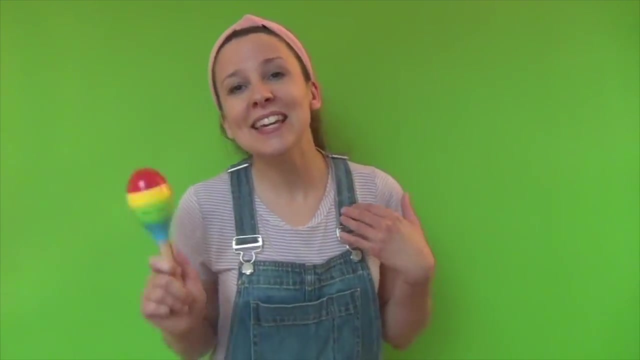 Wow, The sun is coming out, but it's still a little cloudy. Let's sing it again and see if the sun comes out. Are you ready? Oh Mr Sun Sun, Mr Golden Sun, Please shine down on me. Oh, Mr Sun Sun. 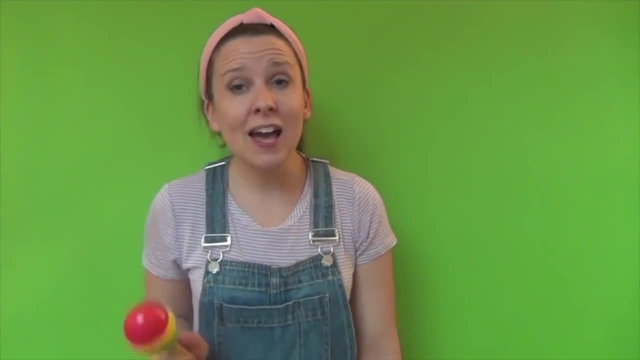 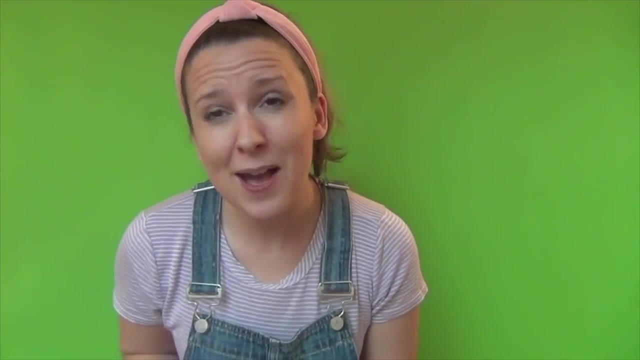 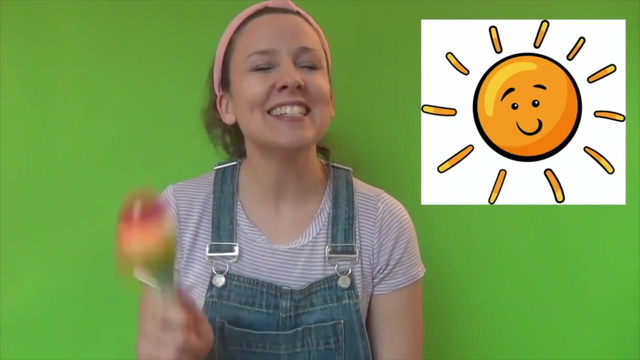 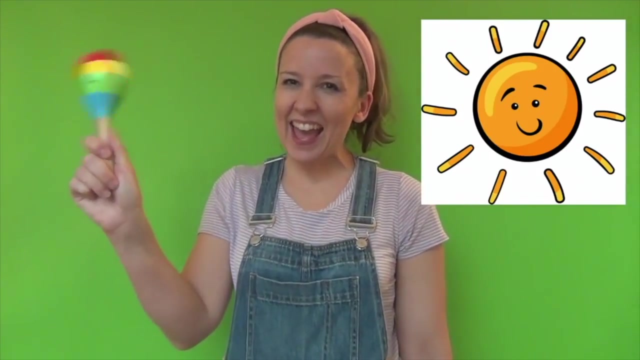 Mr Golden Sun Hiding behind a tree. These little children are asking you to please come out so we can play with you. Oh, Mr Sun Sun, Mr Golden Sun, Please shine down on me. Oh, Mr Sun Sun, Please shine down on me. 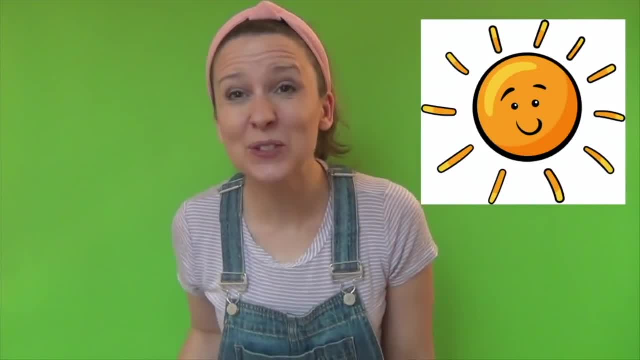 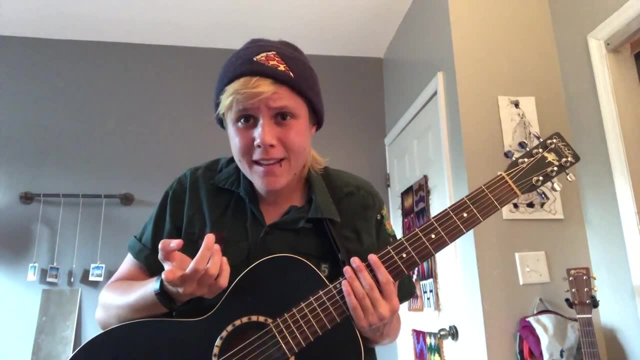 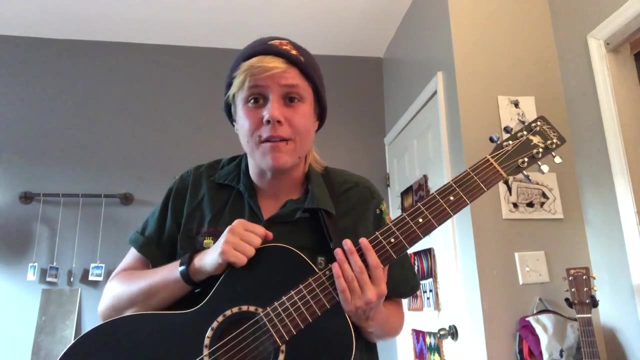 Oh, the sun came out. It's so warm now. thank you so much. Hey everyone, We're gonna do a song with dynamics. did you learn about dynamics already? so what are they? that's right. soft and loud. it's how soft or loud music is. 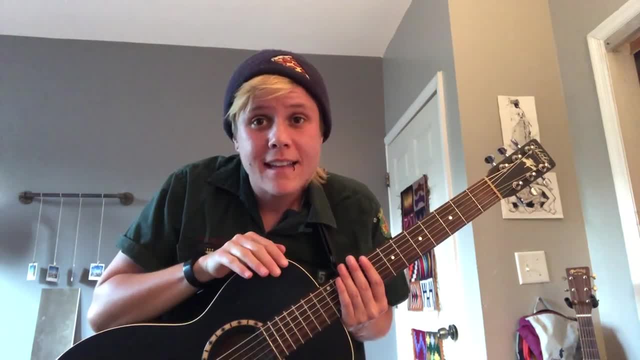 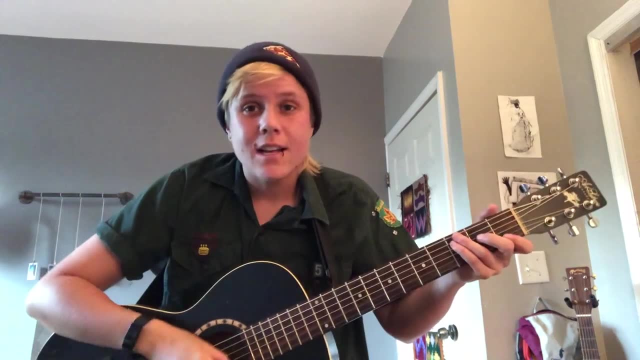 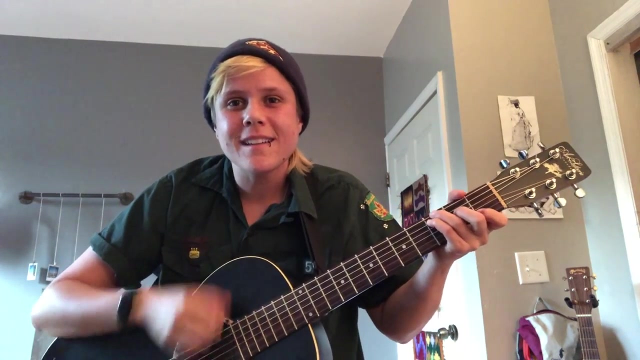 so let's do a song and soft and get really, really loud whenever you hear the word shout. so it's gonna be like this: John Jacob Jingle Heimer Schmidt- his name is my name too. whenever we go out, the people always shout: there goes. John Jacob Jingle Heimer Schmidt. 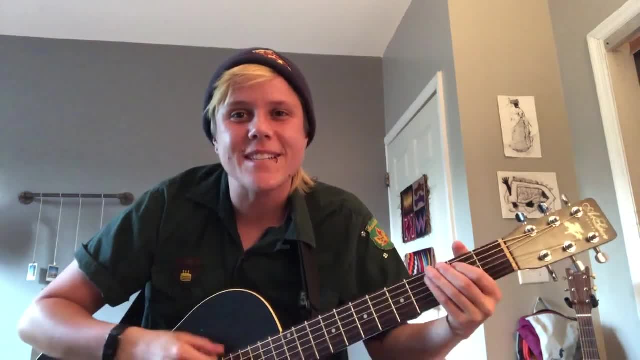 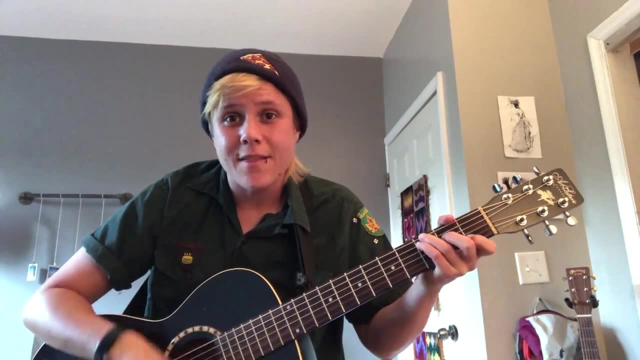 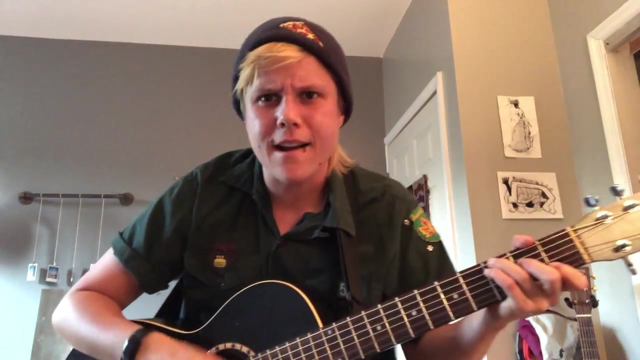 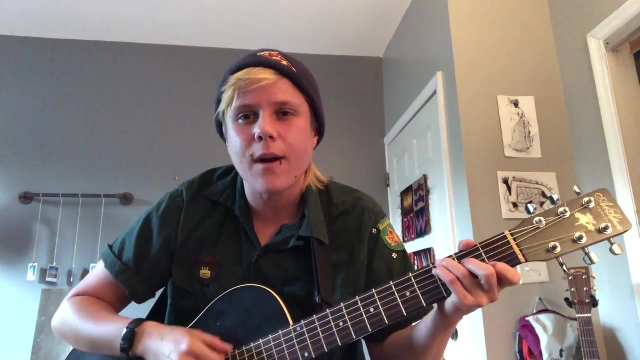 John Jacob Jingle Heimer Schmidt. his name is my name too. whenever we go out, the people always shout: there goes John Jacob Jingle Heimer Schmidt. oh my gosh, y'all sound so good. can we do it again this time? be really loud in the loud parts and really quiet in the soft parts. let's try to be. 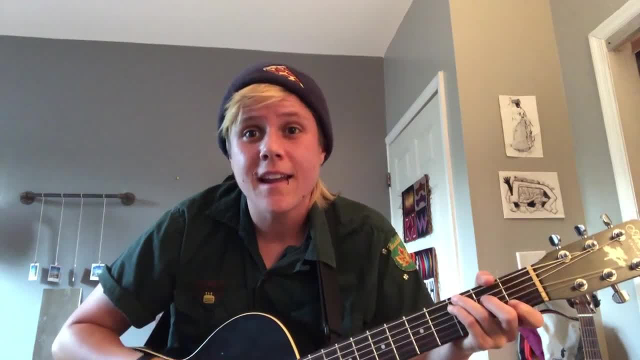 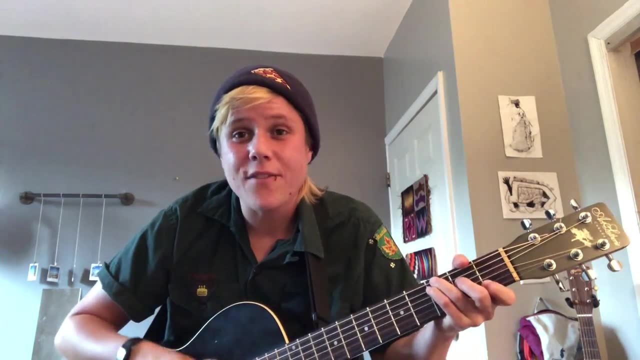 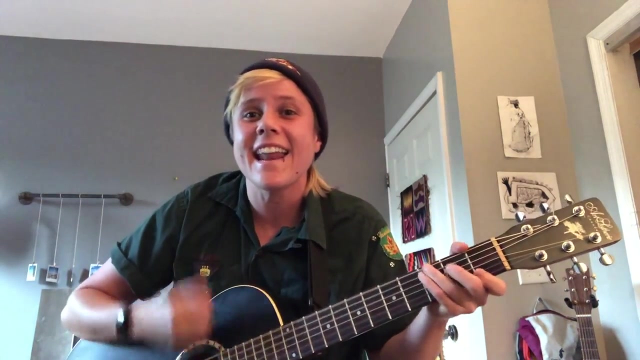 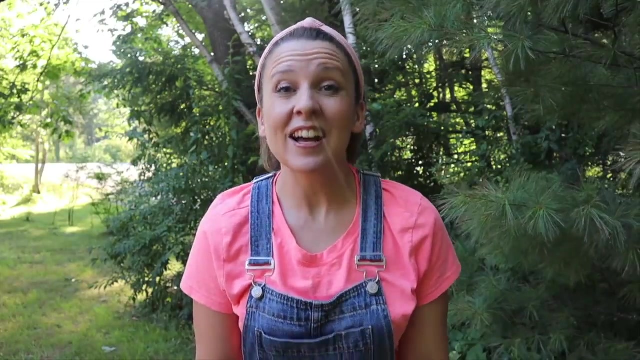 really really quiet, ready, here we go. John Jacob Jingle Heimer Schmidt- his name is my name too. whenever we go out, the people always shout: there goes, John Jacob Jingle Heimer Schmidt. good job, everybody. using those dynamics, now back to Rachel, the next song. I'm going to dance around. 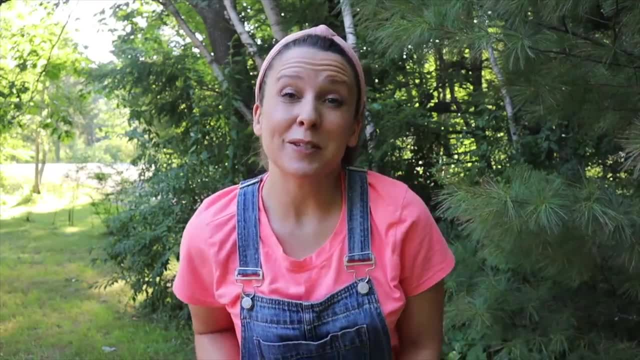 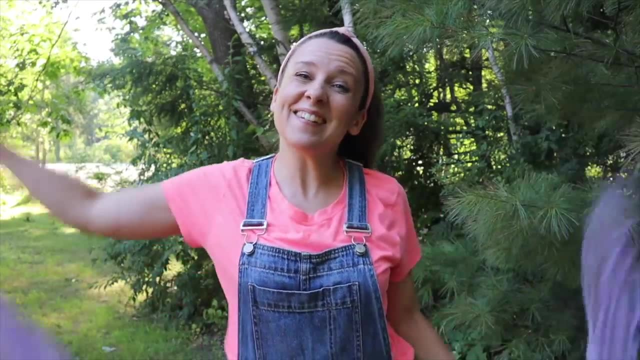 with these pieces of fabric, you could get out some scarves or some little dish towels. you could get out some scarves or some little dish towels. you could get out some scarves or some little dish towels or anything. you have old fabric and let's dance around. it's gonna be so much fun. 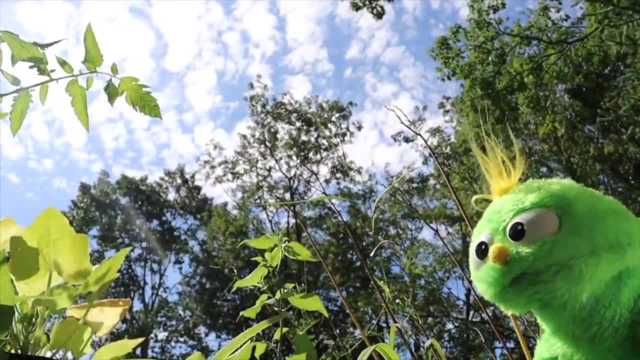 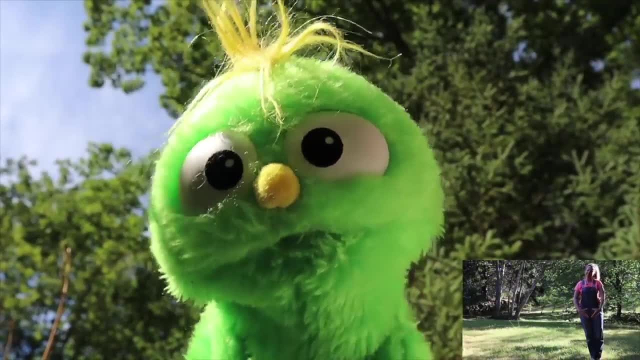 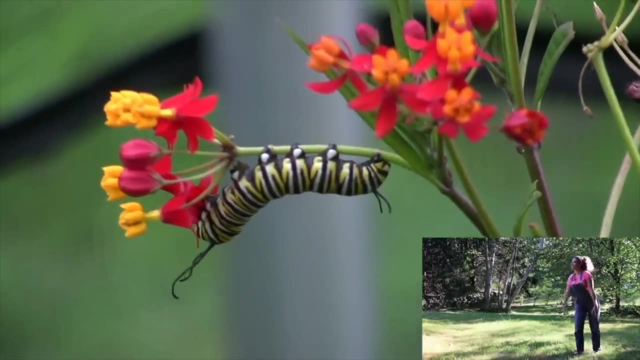 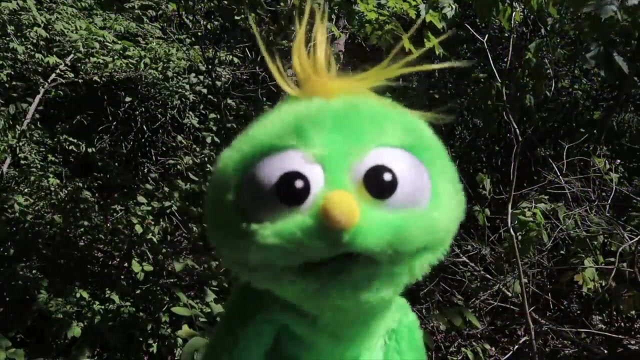 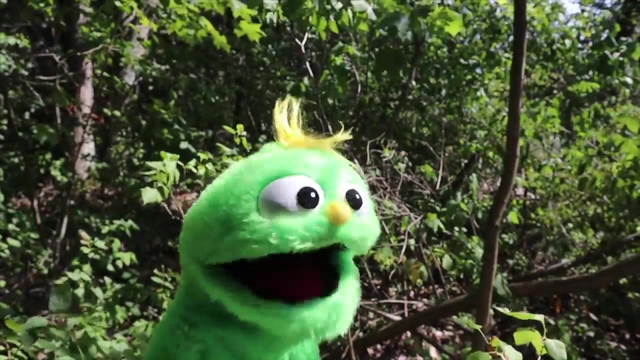 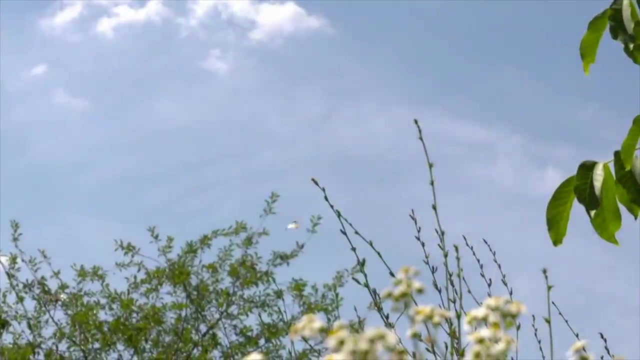 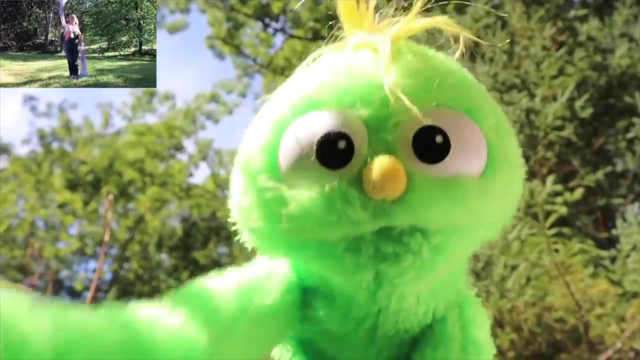 caterpillar, caterpillar moving, oh so slow. caterpillar, caterpillar munching as you go. caterpillar, caterpillar, munching as you go. that you're a problem. some people might call you strange, but caterpillar, hang in there, cause things are gonna change. caterpillar, caterpillar climbing up your plant. 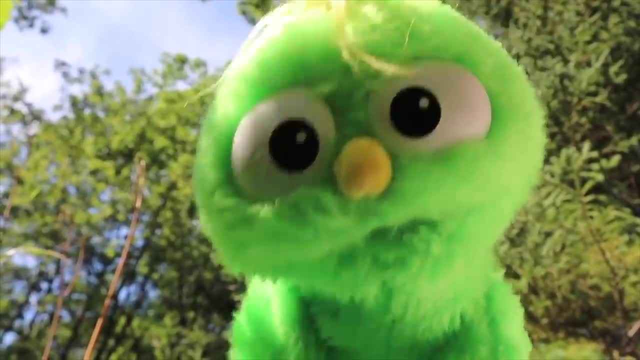 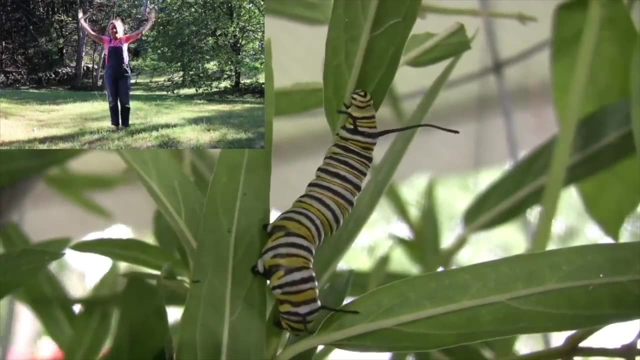 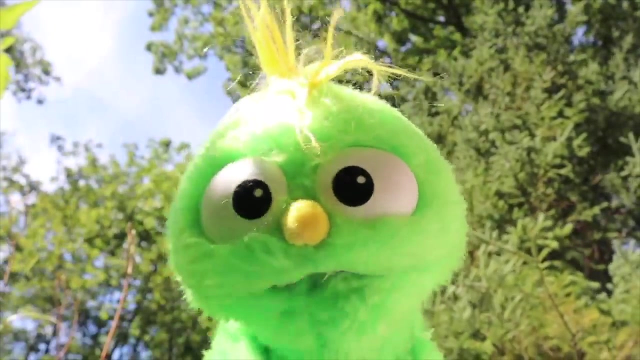 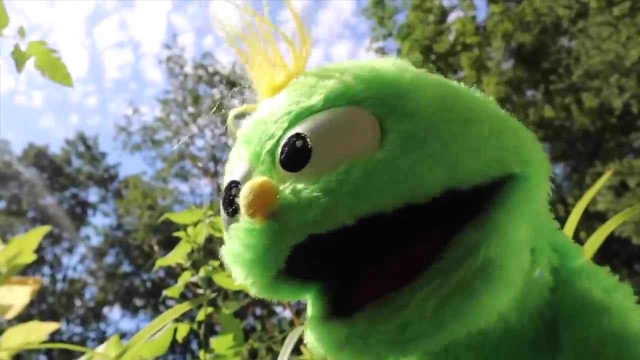 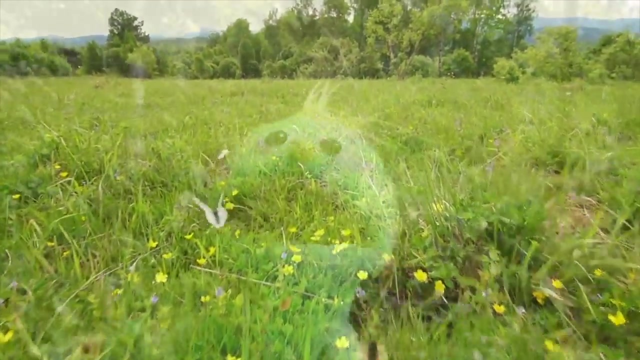 whoa, quiet little caterpillar never saying caterpillar, caterpillar climbing up your plant, but caterpillar, caterpillar, climbing up your plant, can't. no, every day you're growing bigger. you once were a little guy and caterpillar, caterpillar, soon you're gonna fly. where you'll go? 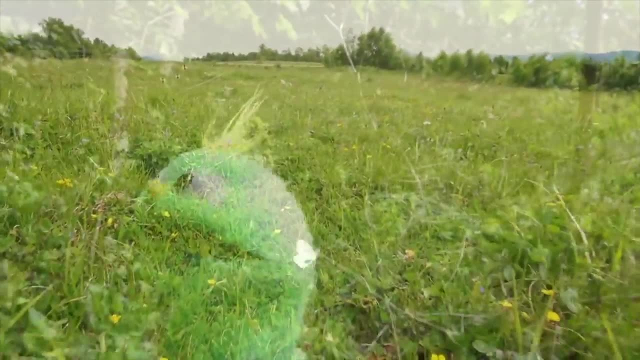 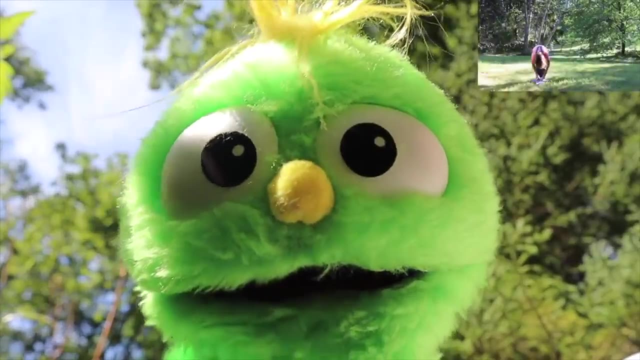 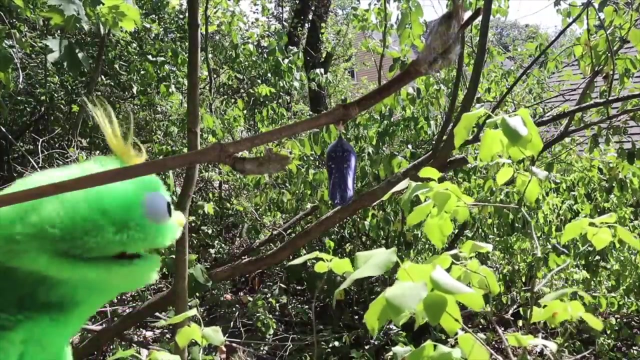 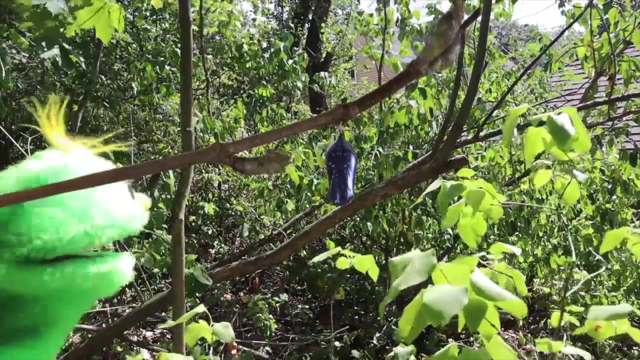 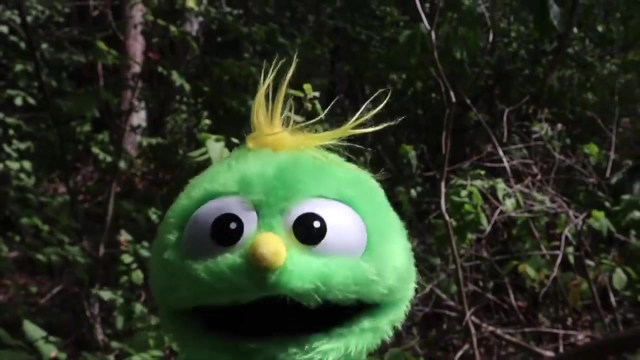 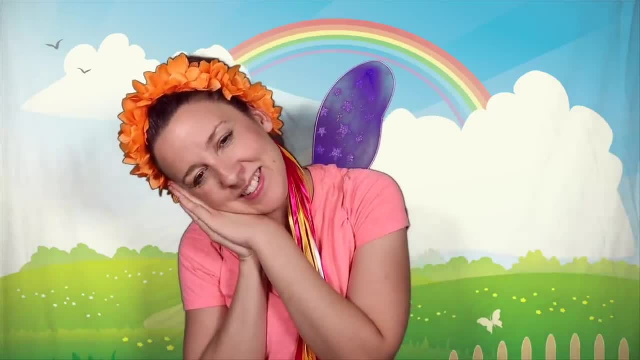 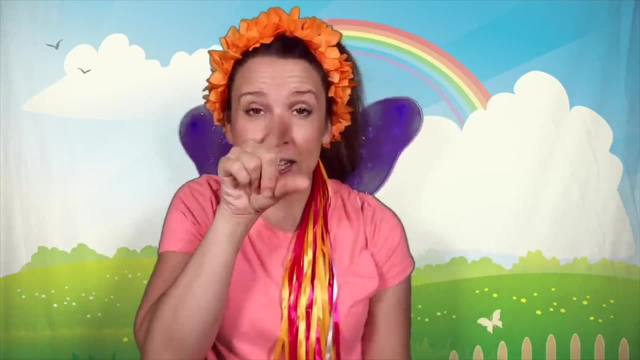 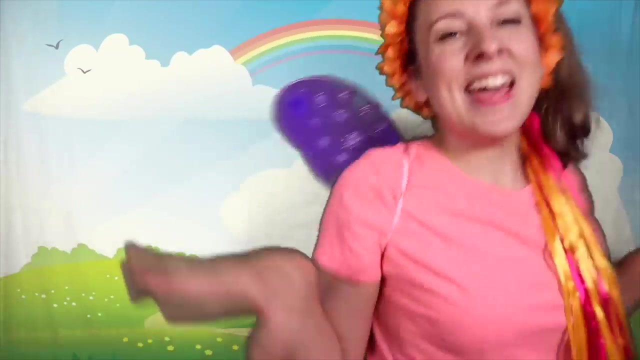 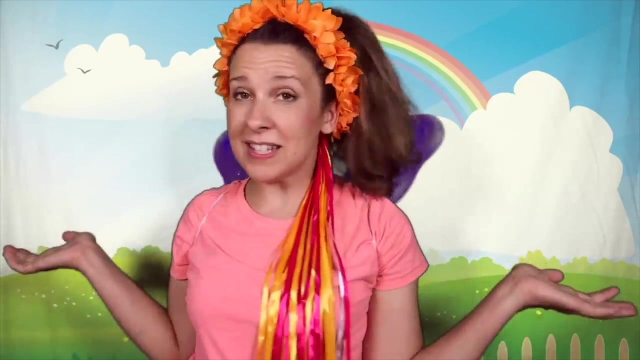 Here I am, here I am. how do you do? That was so much fun. What do you think this is? It's a bird, Little bird, little bird. where are you? Here? I am, here I am. how do you do? 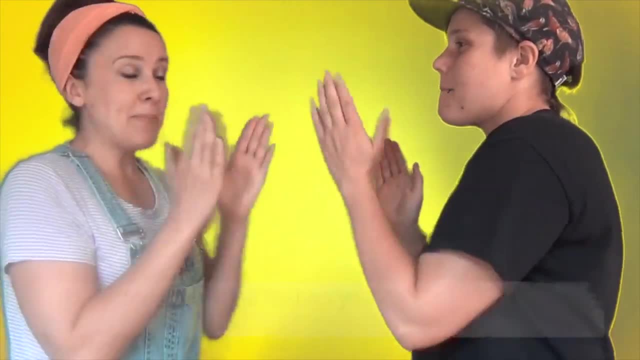 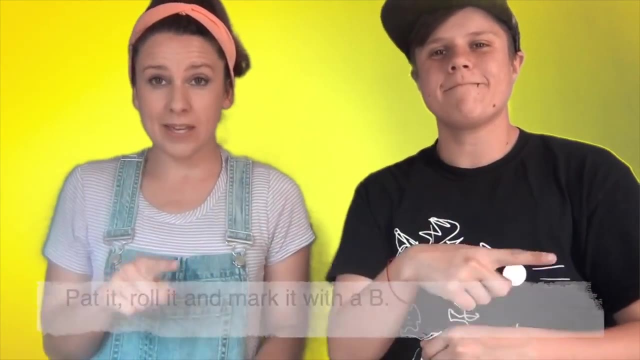 That was so much fun. Great job pretending to be animals and insects that we see outside. Patty cake. patty cake baker's man, Bake me a cake as fast as you can, Pat it, roll it and mark it with a- B. 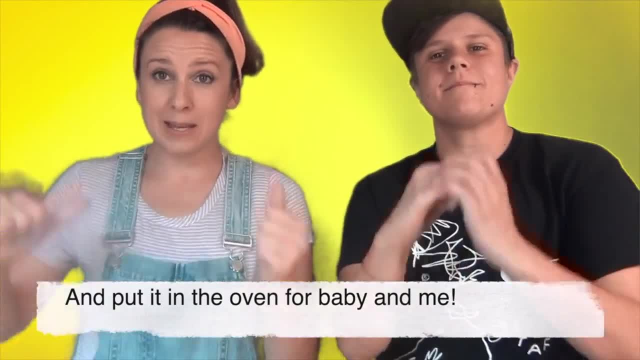 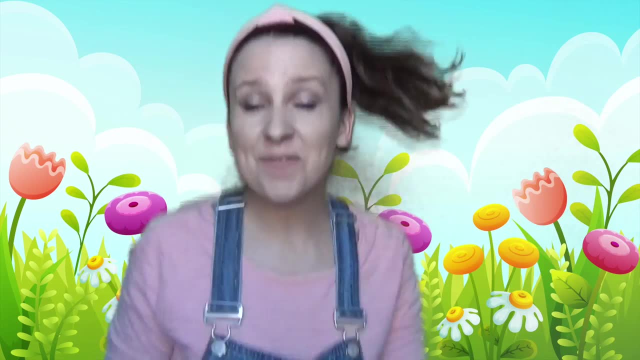 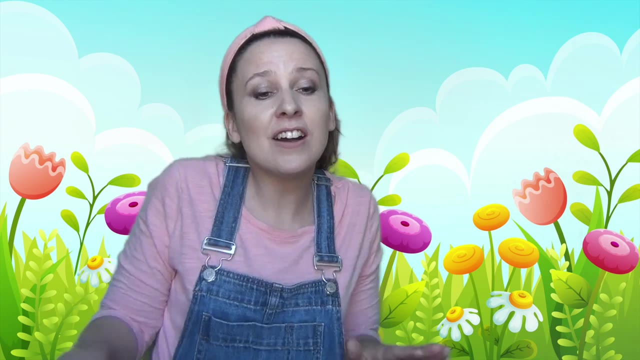 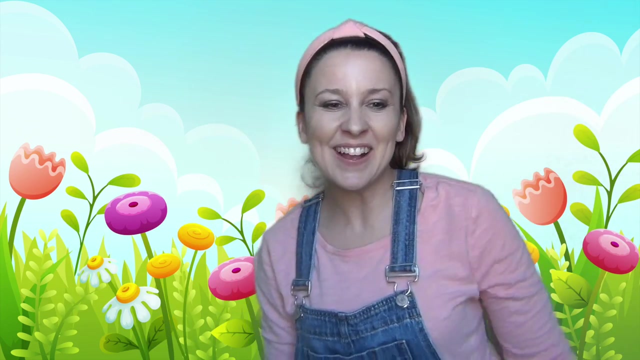 And put it in the oven for baby and me. Jump like a froggy Jump, jump jump. Jump like a froggy Jump, jump jump A little green froggy in a pond. Jump like a froggy Jump jump jump. Fly like a birdie. 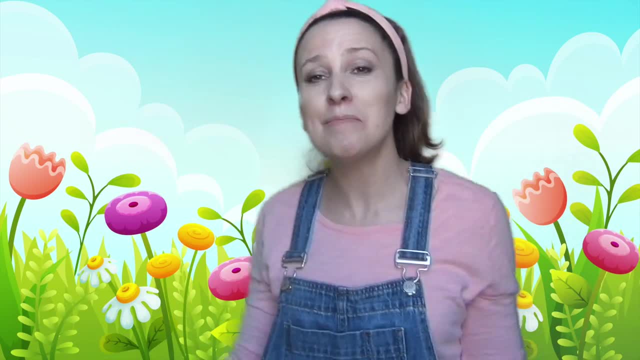 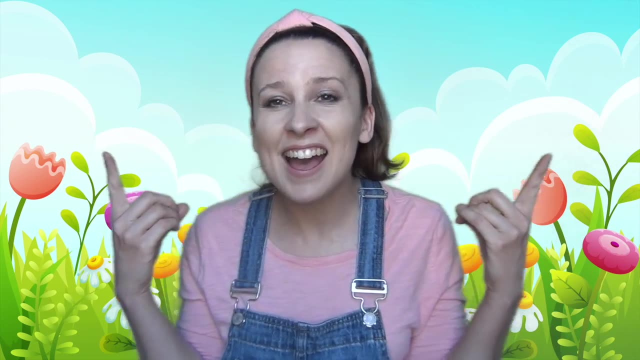 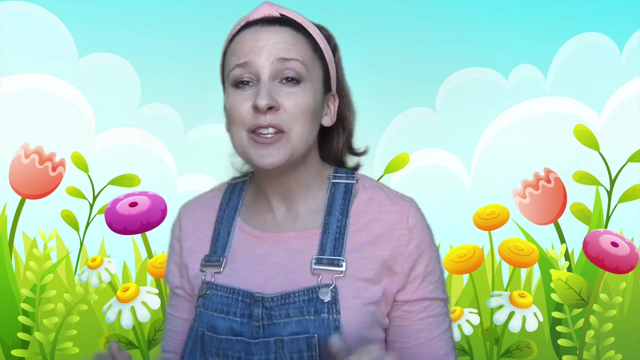 Fly, fly, fly, Fly like a birdie, Fly, fly, fly A little blue birdie in the sky. Fly like a birdie, Fly, fly, fly. You can be anything you wanna be. Da-da-da-da, Ba-da-da-da-da, Da-da-da-da-da. 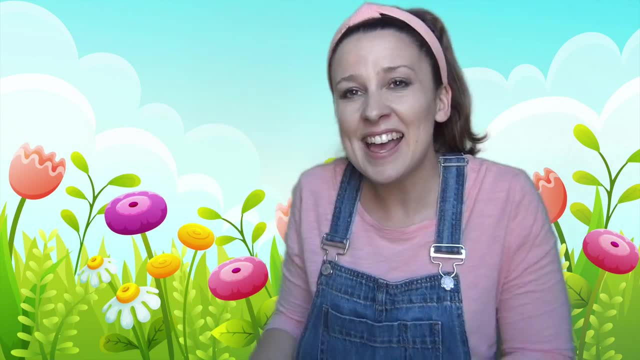 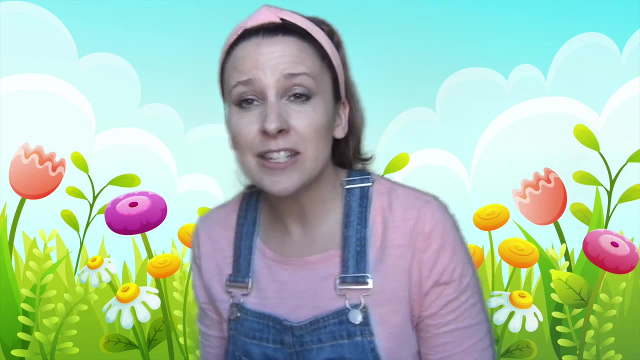 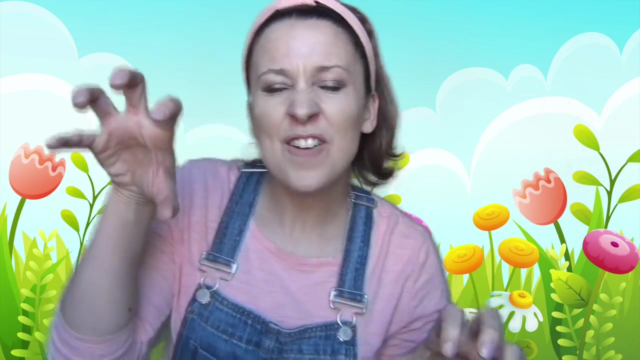 Da-da-da-da-da, Ba-ba-da-da-da. Stomp like a dinosaur, Stomp, stomp, stomp. Good job. Stomp like a dinosaur, Stomp, stomp, stomp. A big green dinosaur on the ground. Stomp like a dinosaur. 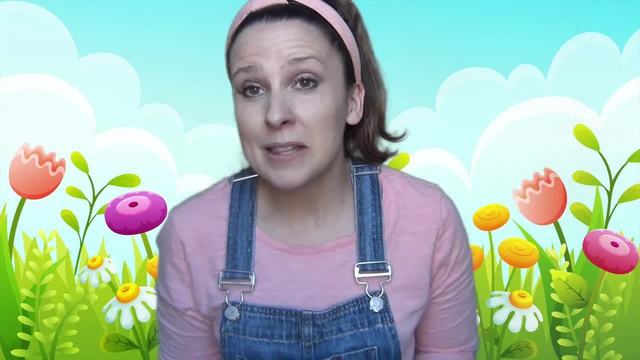 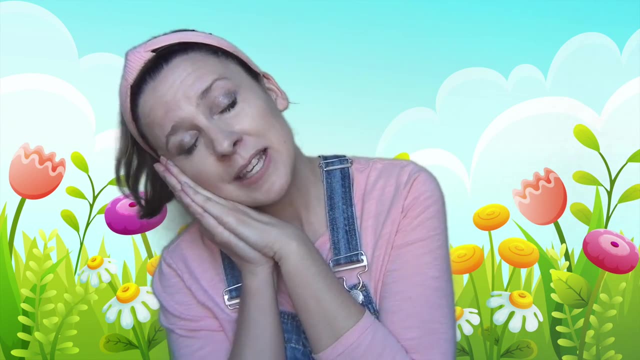 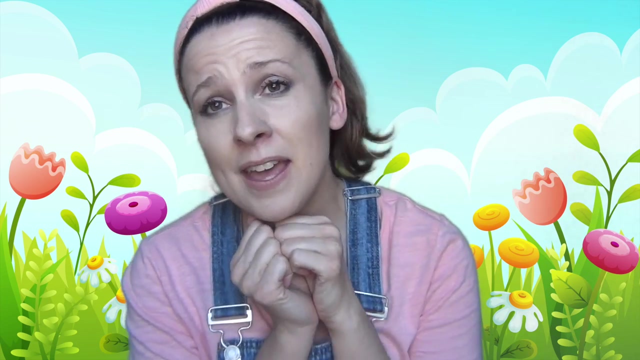 Stomp, stomp, stomp. Now we're gonna sleep like a baby. Can you fall asleep? Sleep like a baby? Sleep like a baby. Sleep, sleep, sleep, Sleep like a baby, Sleep, sleep, sleep. An itty bitty baby in a crib. 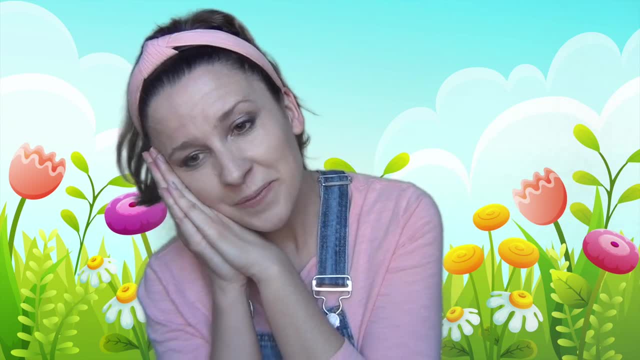 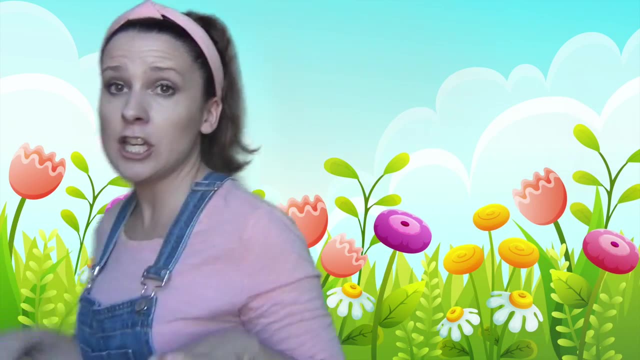 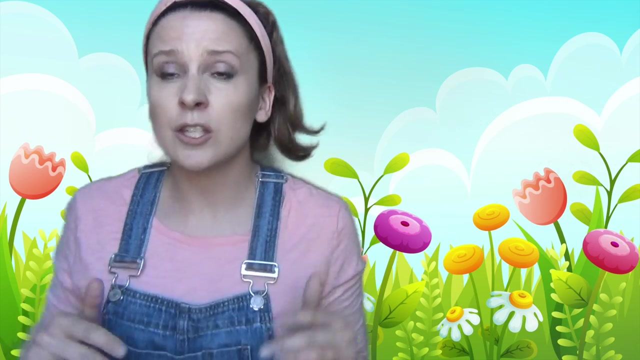 Sleep like a baby. Sleep, sleep, sleep. Swim like a fishy Swim swim, swim. Let me see you swim. Swim like a fishy Swim swim swim A slippery fishy in a lake. Swim like a fishy Swim swim, swim. 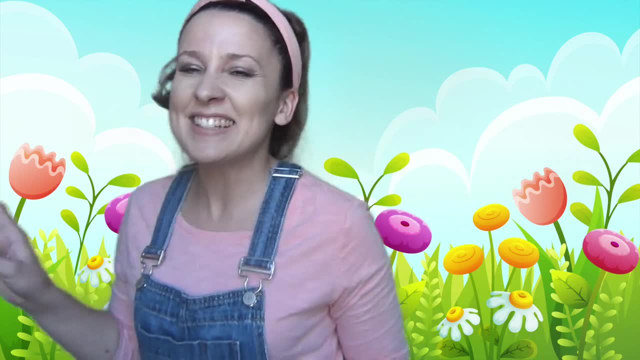 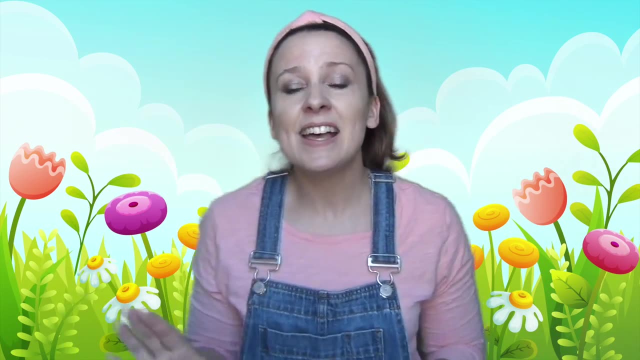 You can be anything you wanna be: Da-da-da-da, Ba-da-da-da-da, Da-da-da-da, Ba-ba-dee-da-da, Sweep-a-dee-da-da, That's called skedding. I'm just saying any syllables that come to mind.